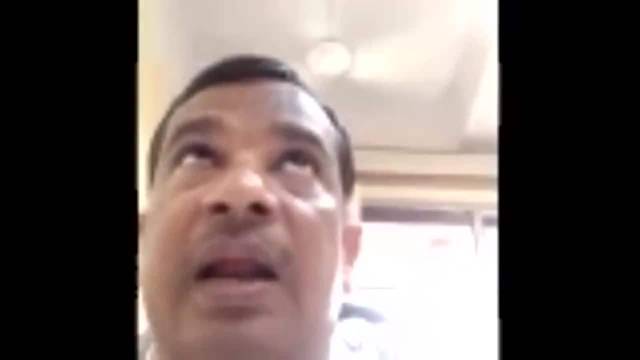 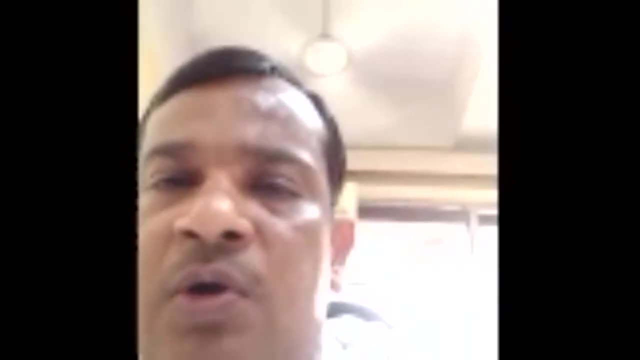 Today also there will be There will be a 15-minute time break at around 11.15 to 11.30.. So in that all participants are not required to leave this meeting. However, they can take rest or something like that. 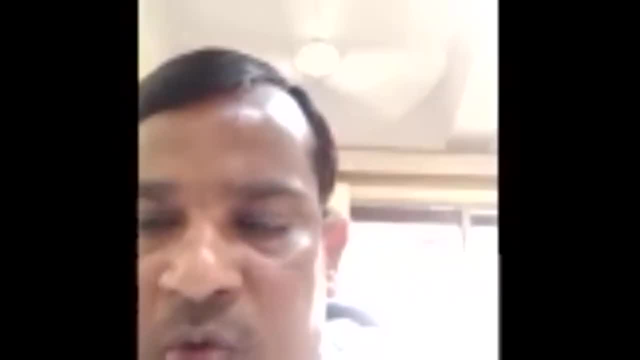 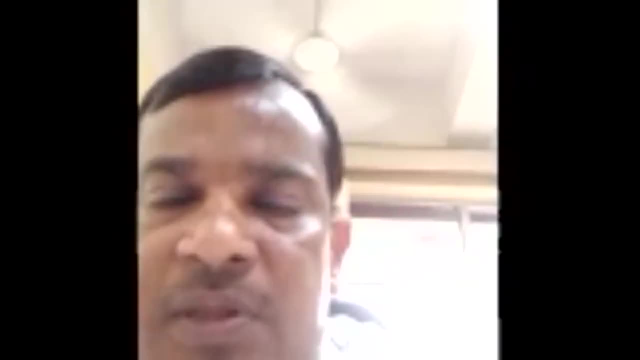 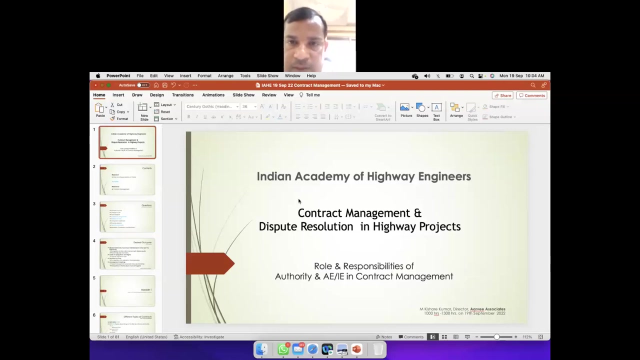 So I will not take much more time. I request Sri M Kishore to start his presentation, as well as his experience with the participants, Thanking you. Thank you very much, sir. Good morning everyone. I see that some policy makers, decision makers and officers across the country are there watching this program. 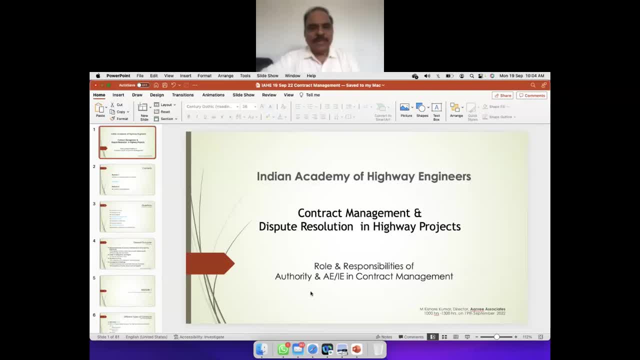 And, basically, many of you might be already implementing the contracts and you know the problems and other things already. But consider this as an orientation program if you are already into it, And what I request you is that you might be having some problems, some issues, some questions in your contracts. 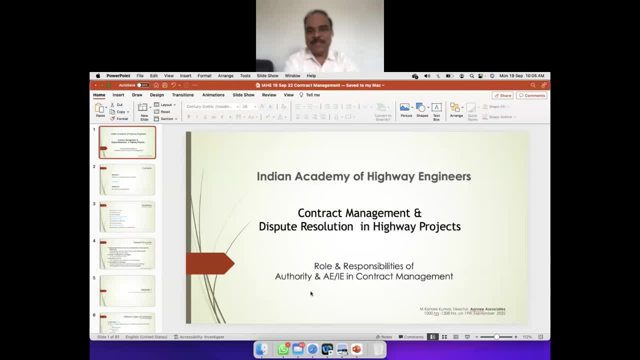 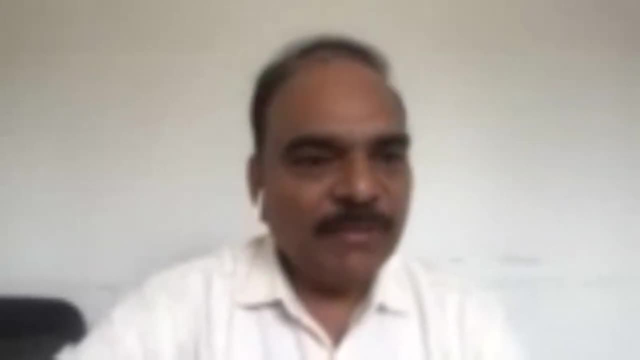 Because nobody is perfect. So we always have doubts and questions, And there must be some areas where you have stopped Means. I don't know what to do. Whom do I ask? So such kind of things Kindly note down and ask me whenever you. 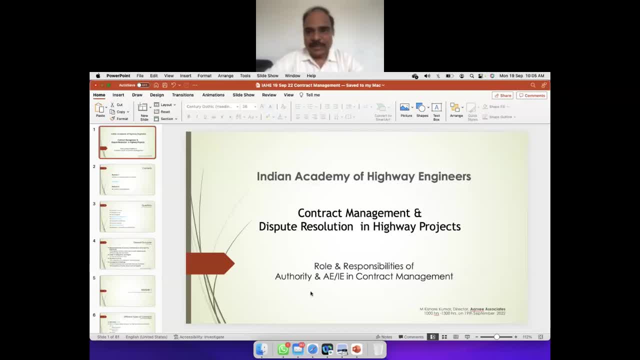 past 24 years And I'll be completing 25 next year. Before that, I was working with one company called Afcons, Asian Foundation Constructions for 13 years. So these are the two companies where I have worked. So I have a stable career and we have around 50-60 projects across the country, only in highways. 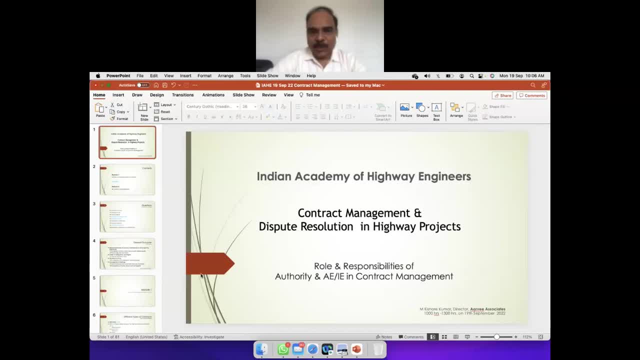 But rest of the sectors are also there And I look after all these design projects and supervision projects, quality contract everything. So I will be able to answer your problem, answer your queries, if at all you ask any, Okay. 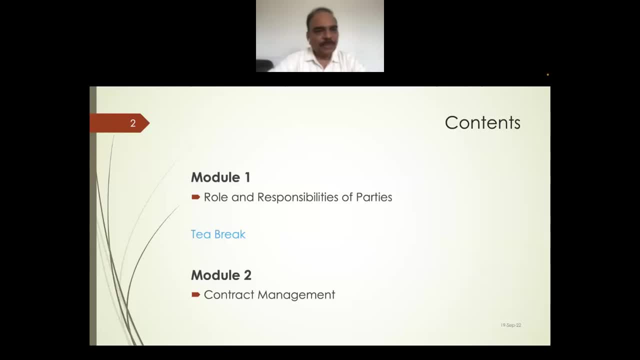 With that I'll go to the presentation And what I'm going to do. there are two modules. One is module one, the role and responsibilities of parties. So these parties are all three: authority, AI, contractor, concessionaire, all the parties. 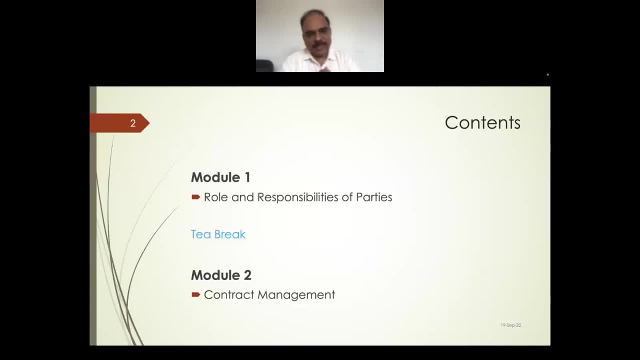 So that is module one, And module two is contract management. So there will be a tea break in between, But I may cover one or two aspects of module two Before tea break, because module two requires attention And I may take more time. 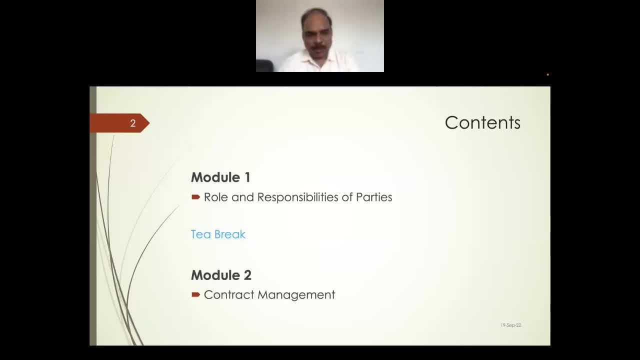 Though number of slides in module two are less, the content may be more, So I may take one or two aspects of module two before tea break and leave you. Otherwise, general organization is like this And what I request. these are the aspects that I'll be covering in the contract administration part. 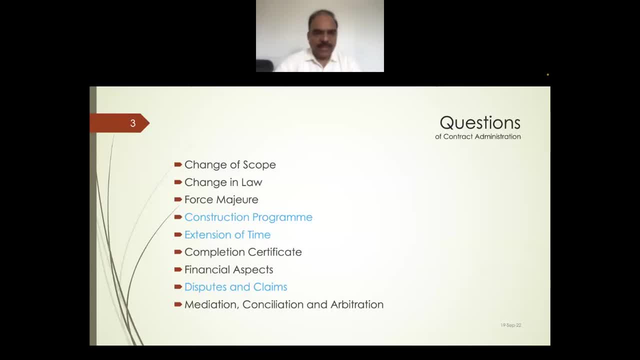 Okay, If you have any question on this, Any issue on your ongoing projects, kindly note down on this And you can ask me questions at the end of the session or whenever you want to, When I am covering it or even otherwise. also. 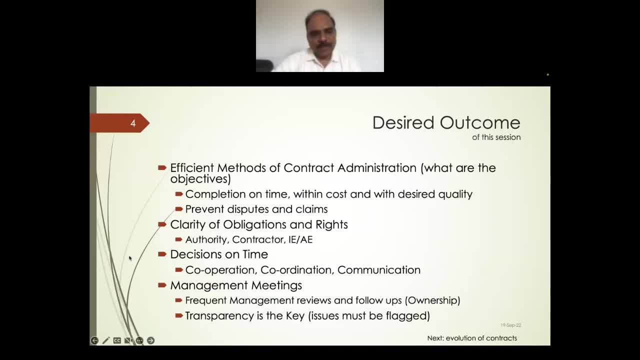 So these are the issues that you can look at Now. the desired outcome of this session, as it is written under that, is efficient methods of contract administration. So this depends On what are our objectives. So the objectives, main objectives of anyone, any client- is complete on time and within cost and with the desired quality. 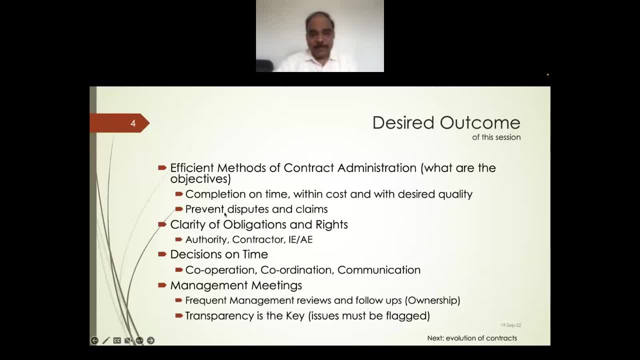 So these are the three important things, So how to achieve them. So, with a view to doing that, we will discuss on efficient methods. Then the most important thing that we should concentrate on is prevention of disputes and claims, So we will discuss on cost overrun, time overrun. these are the two main things. 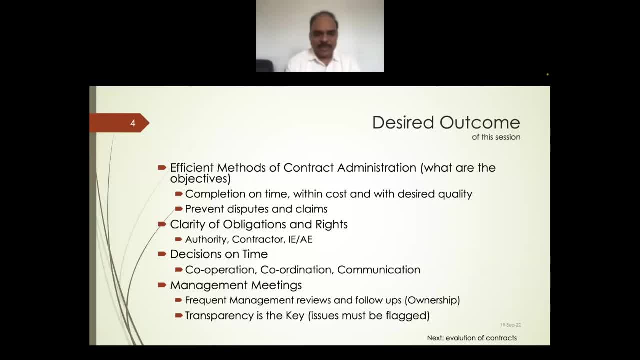 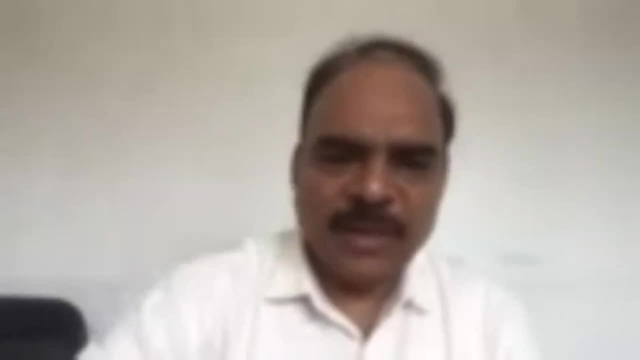 So I have written a paper on this in 2022.. I will ask the organizers to circulate that paper also. It is just six pages, I think, but it has some idea to prevent disputes and claims which you can implement. 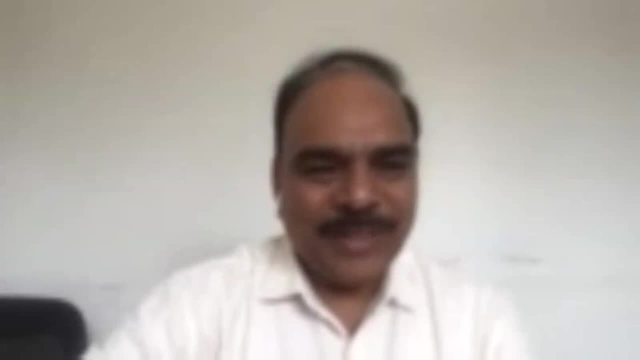 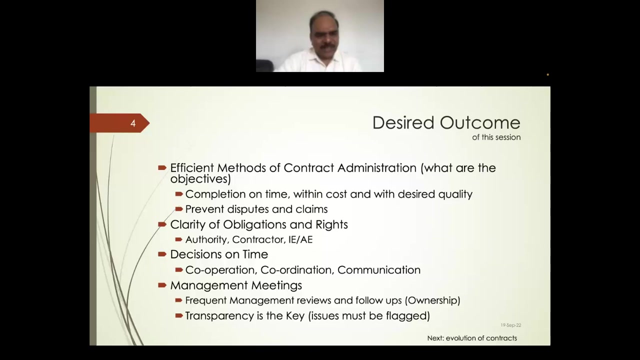 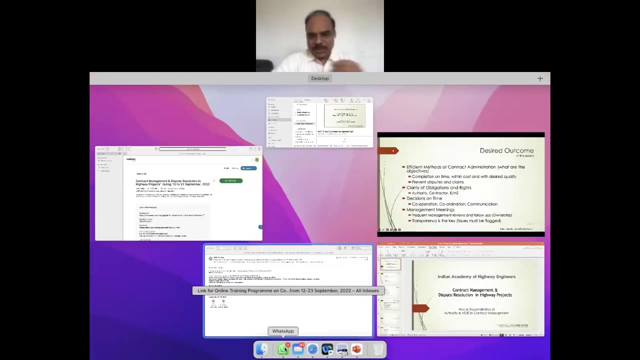 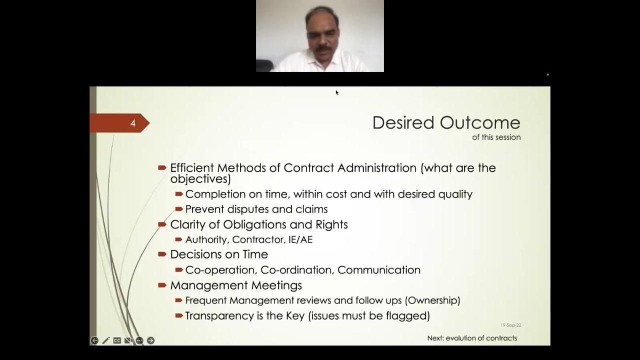 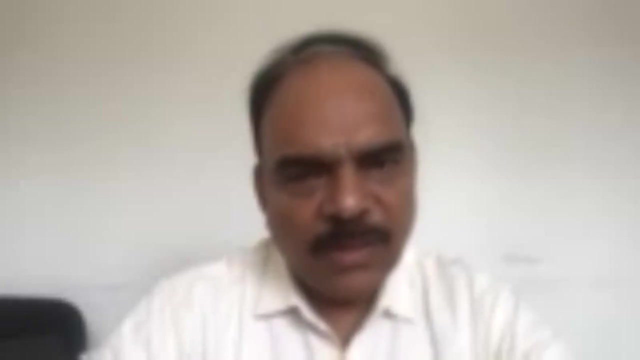 Not easily, but certainly, Okay, Certainly, you can try to implement them. Union Minister Sri Gatkariji, nowadays is cooperation, coordination and communication. So just a moment, I have some funny things coming over. I have some pop-ups coming and I want to close all the other windows so that they don't disturb us in the next…. 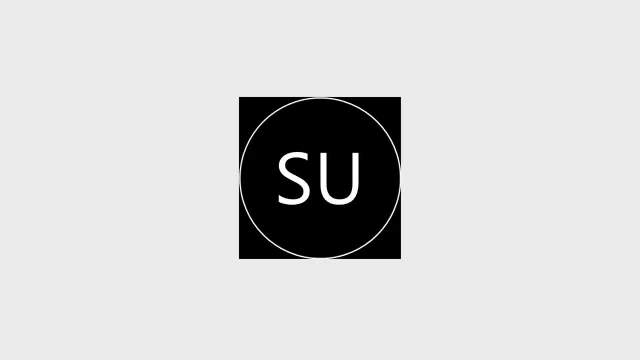 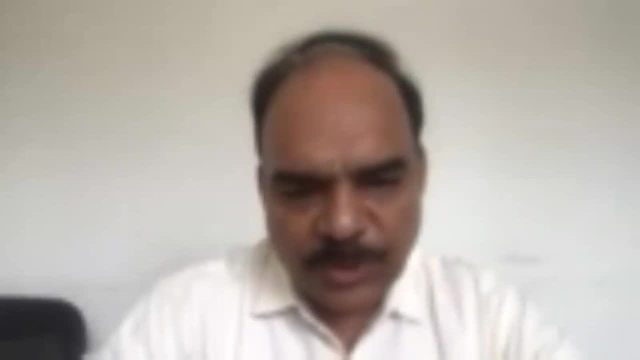 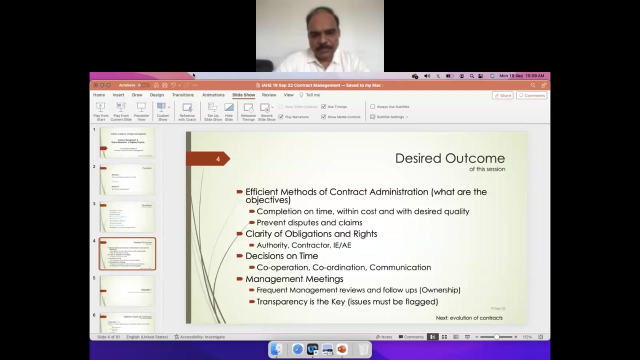 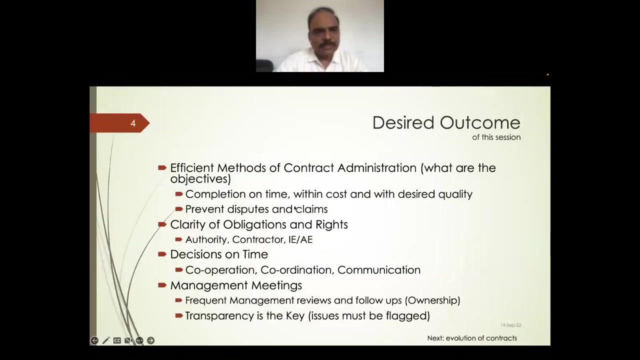 Yeah, Just a moment. just a moment. I have some pop-ups coming and I want to close all the other windows so that they don't disturb us in the next…. Yeah, Okay, Ready, Yeah. So these three words: cooperation, coordination and communication. 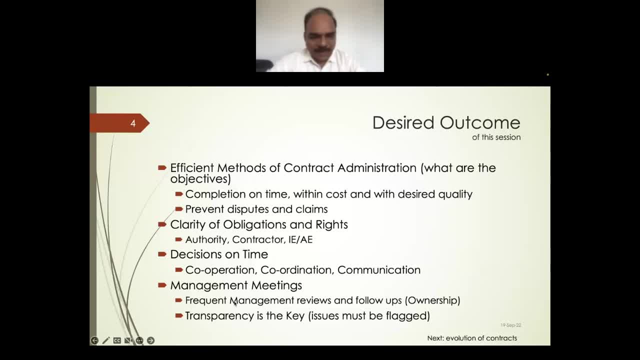 Yeah, these are very, very important, very important. so if these are there among the parties, and then the decisions also can be on time management meetings- management, of course, is the owner, so frequent management reviews and follow-ups- they go a long way wherever the chairman or the managing director. 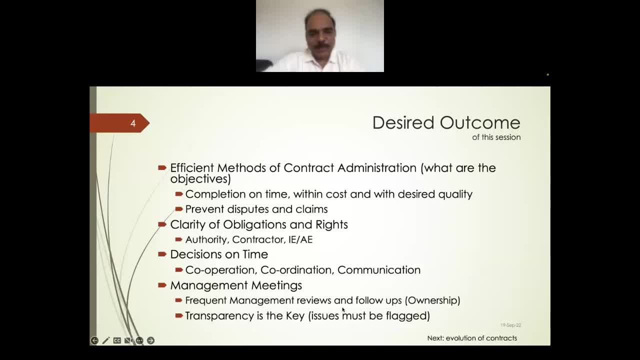 or the secretaries or anybody, adg, dg, depending upon the chief engineer, when whoever is the head of the institution, if they take reviews and there's a follow-up, it goes a long way. and, of course, transparency is the key when the top man is reviewing. if you don't flag. 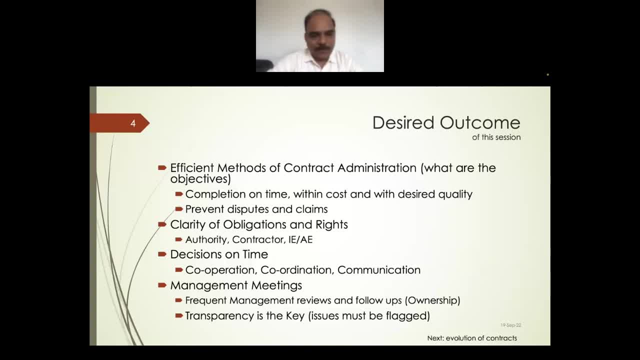 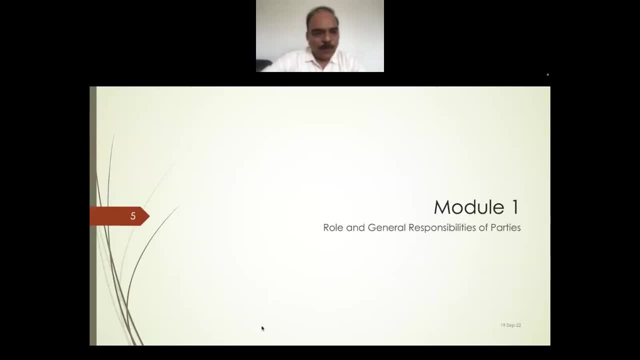 the issues and if you don't tell them properly, you want to hide them. then it becomes difficult. so transparency is the key in management meetings. so these are the four heads that the organizers has given me to cover. i hope these things will be covered without heading. now. module one: role and responsibilities of the parties. now, how these contracts have. 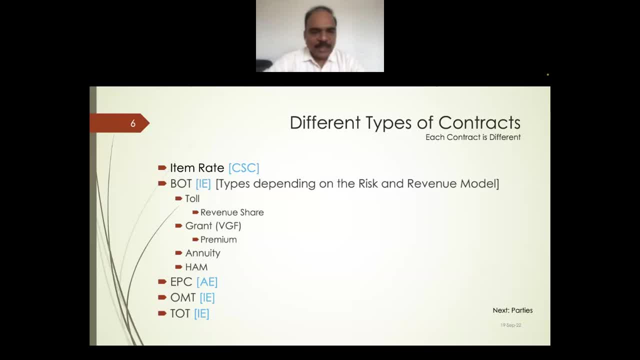 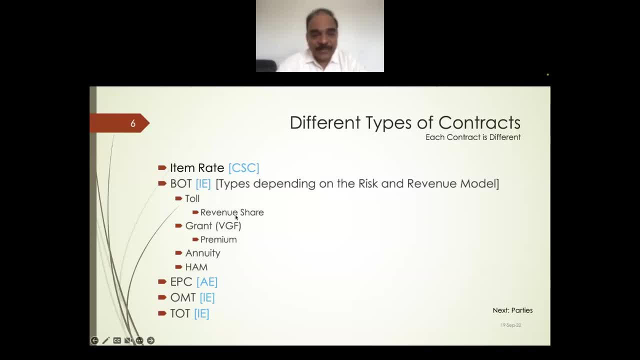 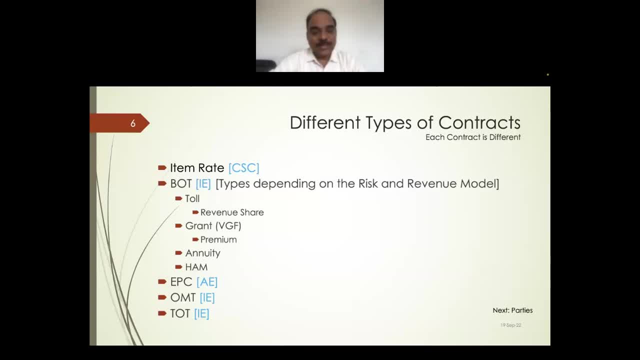 가. helping for准备 means two thousand. you have to add this to the balance. so price of another is there are three villages. you have to select that. the big parameter is which is which, where you know, is it a small or big? that are one, or if two papers and a small. 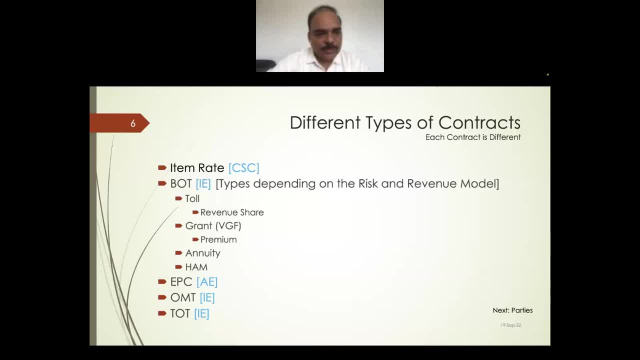 son and давай and tol. there are still people as i can coloured. if this is an example, that much grant do you want? the total project cost was being given and how much grant do you want? and when it crossed 40 percent it becomes difficult. so generally five percent, ten percent. 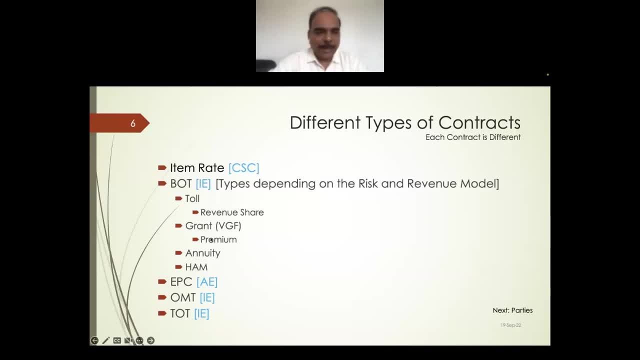 up to 40 percent. the grant was allowed viability gap funding. as you know, then if the toll is more, that is when the toll is less. if the toll is more, then, like revenue share, the concessionaires were offering premium. so premium was the big parameter with the fixed concession period. 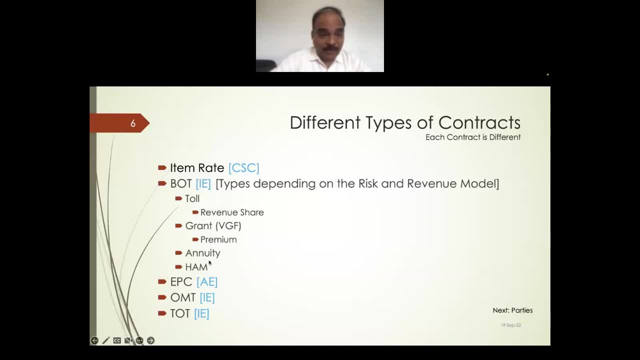 then there was another thing: when all of these things fail, toll, pure toll fails, grant fails- then we were giving annuity. annuity is the payment that we give every six months after completion of the constructions. so then, and for annuity also, concessionaires were not coming. 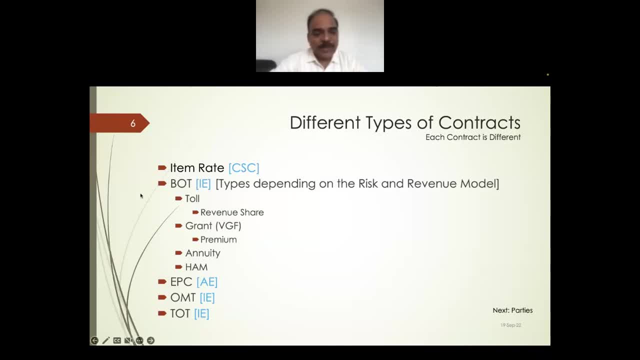 because during the construction period all the money was supposed to be put by, invested, by incurred by the operator. so he doesn't have money, banks were not giving. so then came the ham model, hybrid annuity model. that means 40 percent of the cost of the project will be given during the construction and 60 percent of the cost of the project. 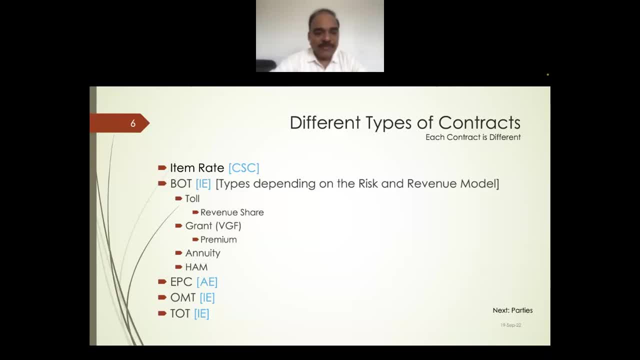 was being given as annuity for 15 years. so that is how these models have evolved. when that is also not viable, then these people are not able to get that- also loans and other things. then we had come up with the epc contract where epc means 100 percent will be. 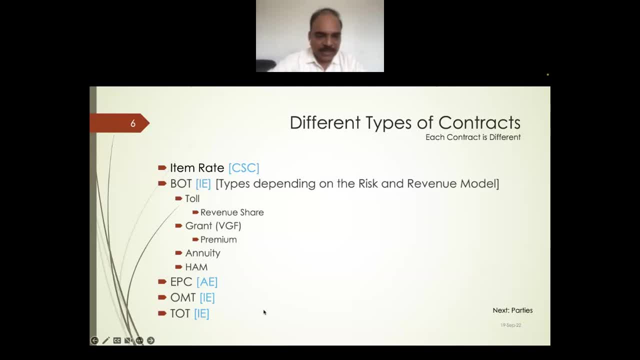 provided by the company client itself, the authority itself. so all the money will be. but there the risk of design, the risk of certain things like earth work, profile corrective course and all those things, these risks are still with the contractor. then the other two modes are omt and tot. so 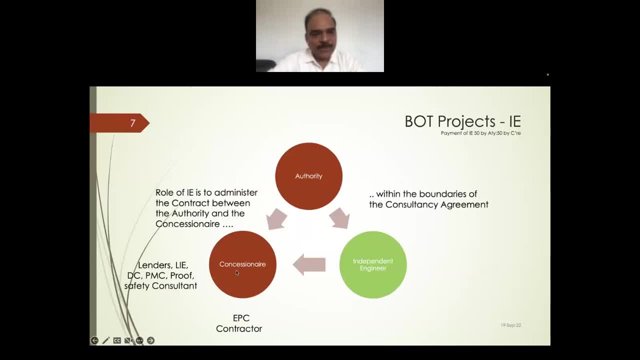 now, even when it is called a bot, then ie comes into picture and when it is epc, ae comes into picture. of course, the contract is always between authority and the concessionaire and independent engineer. he actually administers the contract between these two. that is the role of independent engineer and there will be various other parties. concessionaire will 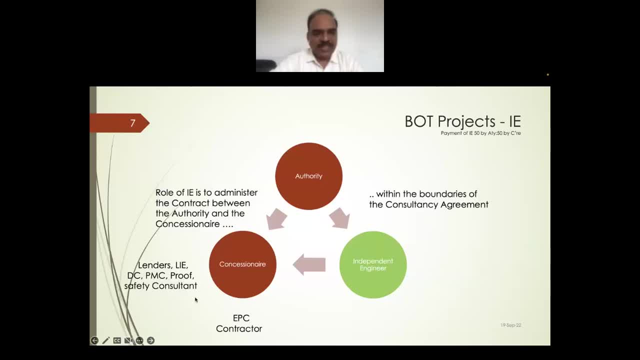 have an epc contractor and so many parties will be there: lender, lenders, independent engineer, design consultant, pmc consultant, project management consultant, proof consultant, safety consultant. so many people are involved in one pot project, in epc project. again, the role is role of otheriki need to administer the contract between these two people and there will be a design consultant. 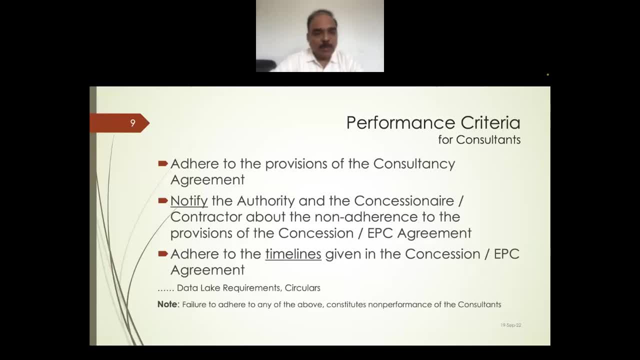 project management consultant and, by agreement, proof and safety consultants are also there now. Now, when we are talking about the consultants, I am sure the main idea is to understand what is the role of independent engineer and authority engineer in this section. So what do we look at as performance criteria of the consultants? 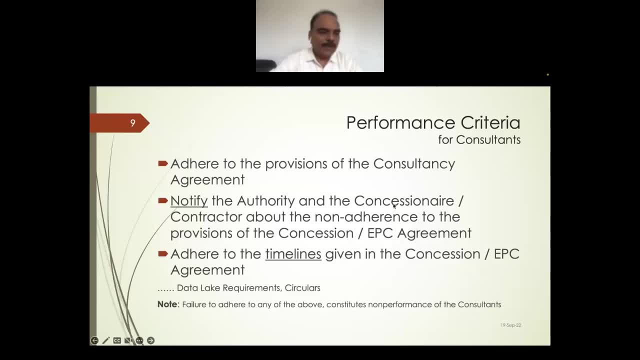 The first thing is they have to adhere to the provision of the consultancy agreement. Whatever is written in the consultancy agreement that they have to follow anyway. The second thing is they have to notify the authority and the concessionaire whenever there is a non-adherence to the provisions of the concessionary agreement. 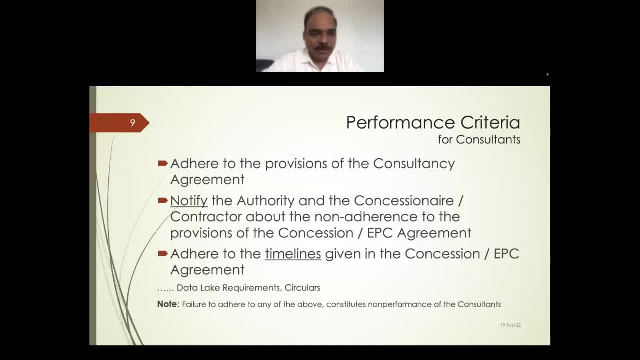 They can't keep quiet, They can't say: Mr Contractor, you know everything what you are supposed to do. Mr Authority, you also know everything that is there in the agreement. Why should I tell you? Both of you are aware. 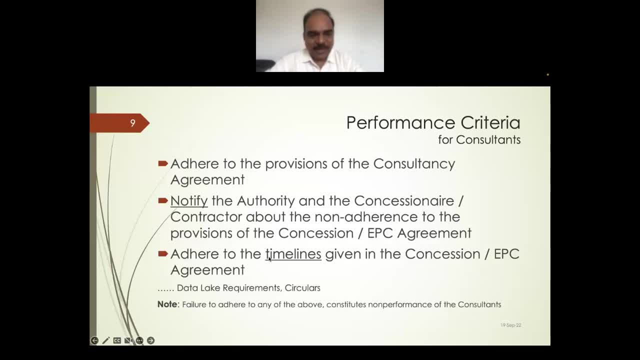 It's not like that. Independent consultant- I mean IE or AE- has to notify the authority on time. That is the second thing. And he has to adhere to the provisions of the consultancy agreement. He has to adhere to the timelines given in the concessionary agreement or EPC agreement. 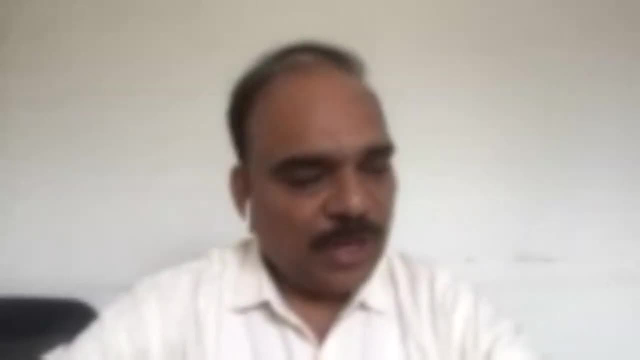 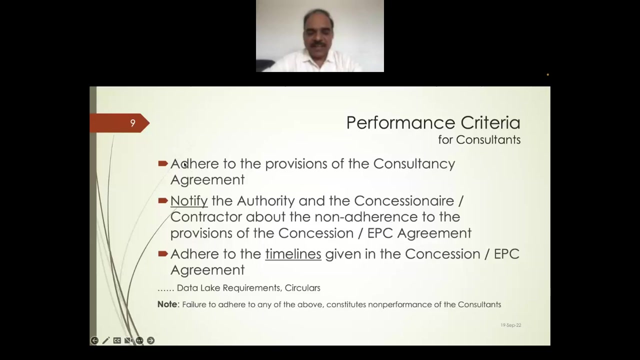 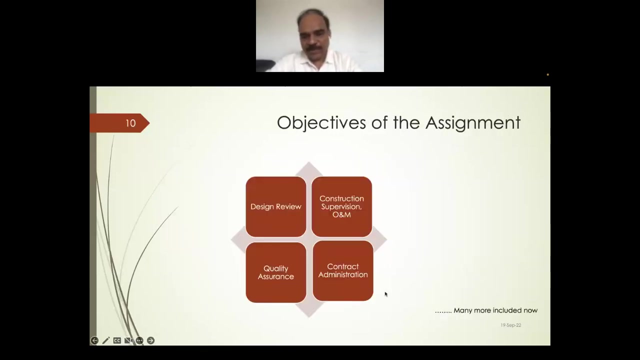 for whatever say design, reviews or notifying whatever timeline is given in the agreement, that has to be followed. Any of these things, if he is not following that is a non-performance. Failure to adhere to any of the above constitute non-performance of the consultancy. 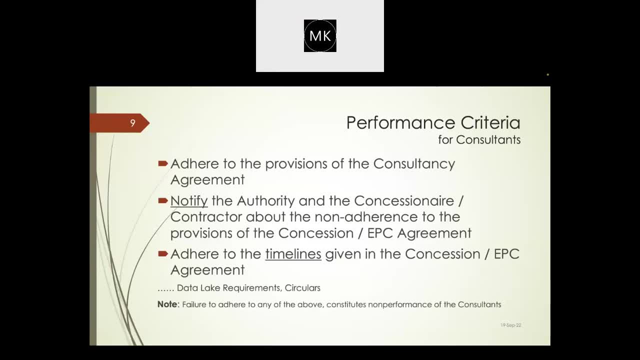 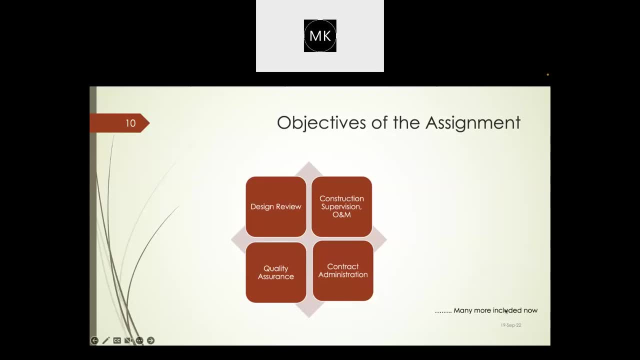 So this is So. that is the first thing that we have to understand. So when, as a consultant, they have to follow this. So as authority, we have to see that, whether this fellow with the gentleman is following this or not, The main objectives of the consultant during the thing is design review, because in BOT, 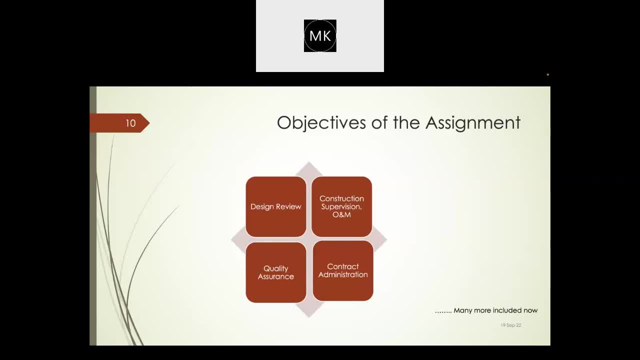 contracts or EPC contract, the design responsibility is with them. So the first part is to do the design review, Then of course construction supervision And also on them during the construction. I mean maintenance during the construction and one in the operation, then quality assurance. 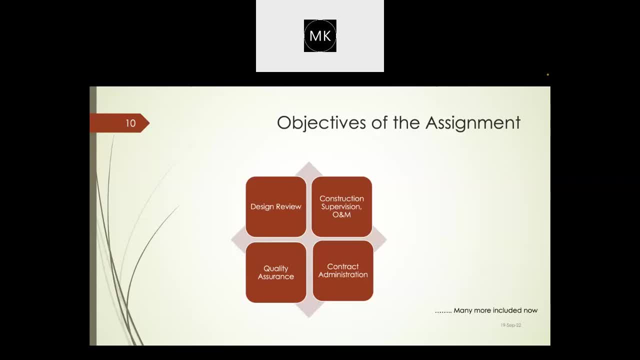 So it's. the difference is it is not quality control. Quality control will be done by the person who is executing the work. Quality control means carrying out tests at the frequencies Those are specified in the contract or in the manuals and codes, but quality assurances 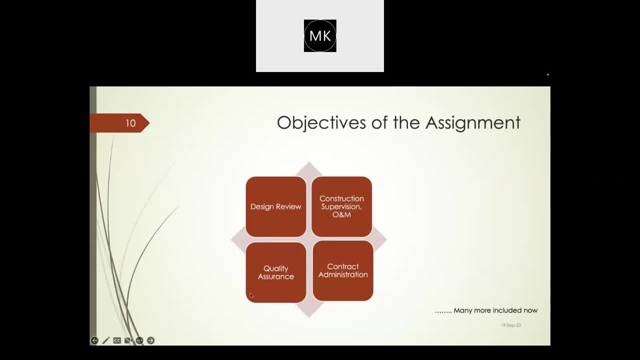 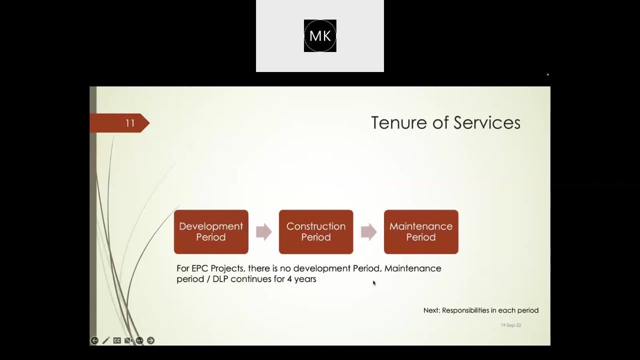 making those plans as to when it has to be done. And then quality assurance. So we have to be tested by whom at what frequency, and that is basically we have quality plans. So that document is called quality assurance document. So we have to see that the arrangements are made and planning is done. 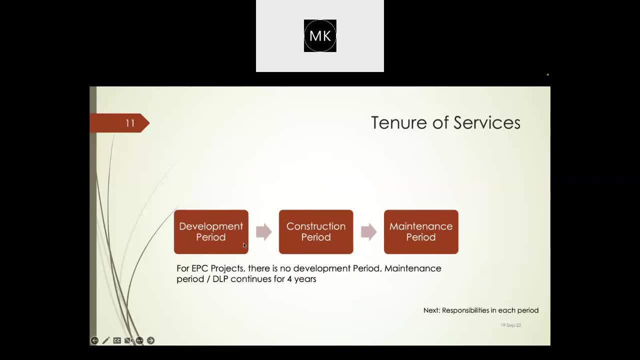 That is quality assurance, as IE and AE Contract administration is the subject of the session anyway. There are three periods: development period, construction period and maintenance period. Of course, development period will not be there in EPC. By definition it will not be there. 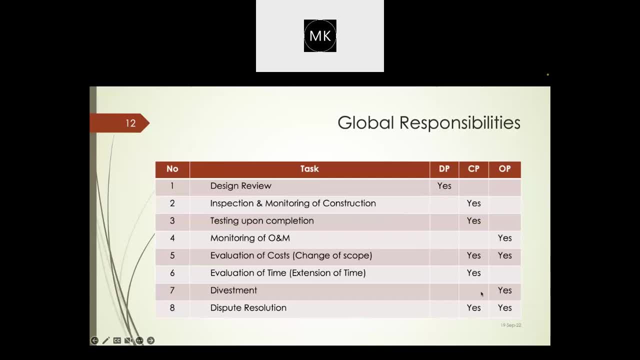 During the development period there are certain responsibilities of the concessionaire. We will see in the next slide. Now, generally, these are various responsibilities, as I said. So in development period, design review is done and in construction period so many responsibilities are there. 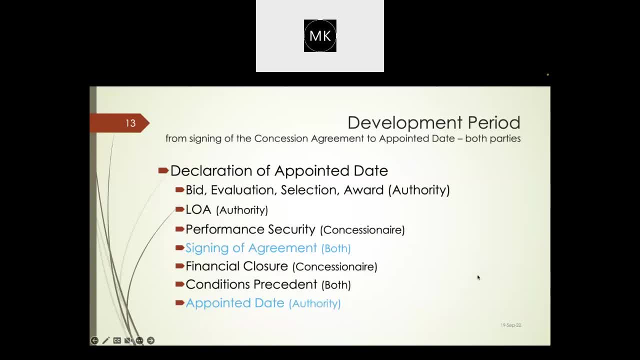 In operation period: monitoring of O and M, then evaluation of cost divestment, divestment with closing of the contract. Dispute resolution will be there in any way, in any. Now let us come to the role in development period. 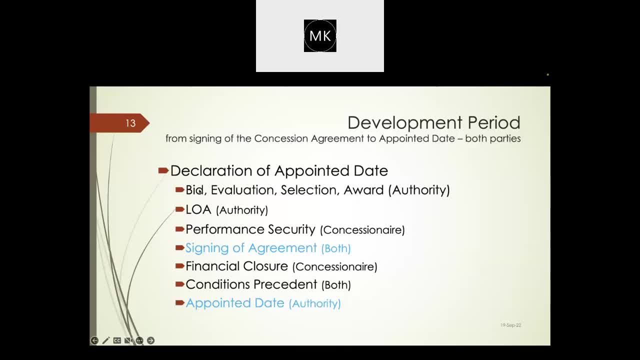 Now, what is development period From signing of the concession agreement to declaration of appointed date? Of course, both the parties are responsible for doing this job Now. first, of course, you know that, bidding, then evaluation, selection of the person, and then we award. 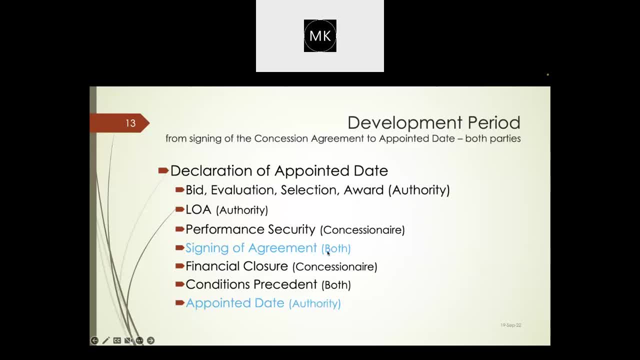 Who awards Authority awards? It is the responsibility of the authority. They give the LOA, Then performance security is submitted by the concessionaire and they sign the agreement. After signing the agreement, they give the agreement. Okay, And two things are there. 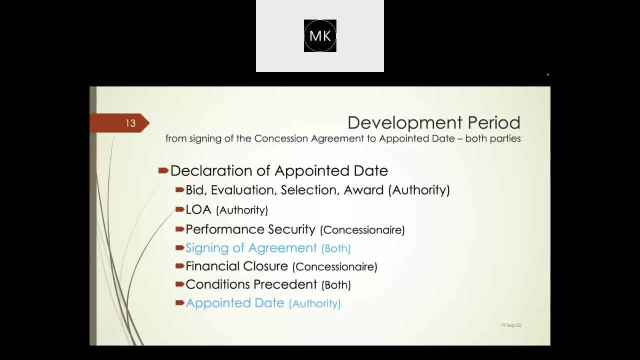 One is financial closure. It is true even for the HAM, also the hybrid annuity model, not only VOT. So financial closure means tying in the funds. whatever funds are required, they have to approach a bank. There may be a lead bank. 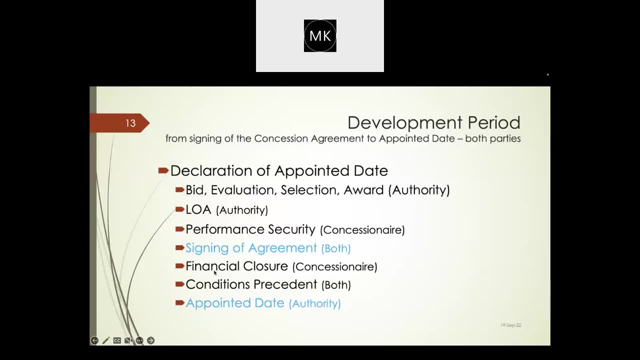 Nowadays there are consortiums. So many banks will be there in one consortium and that loan agreement has to be signed and that has to be brought to the client and then they have to submit it. This is our financial plan. So much is our equity and so much is going to be the debt that is to be provided by the 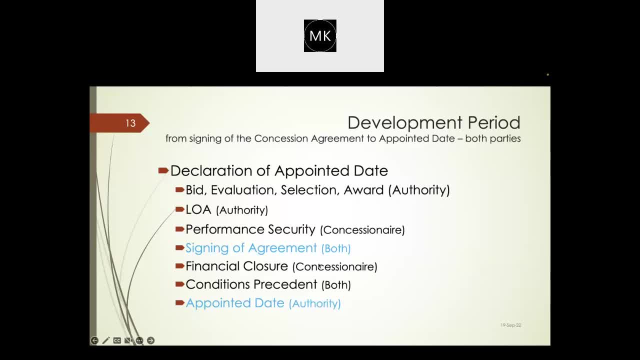 lenders And, if at all, there is any grant or anything- equity support, they call it. those things also will be mentioned. So this financial closure has to be achieved on the part of concessionaire Condition precedents they are. that means precedent to declaration of appointed date. 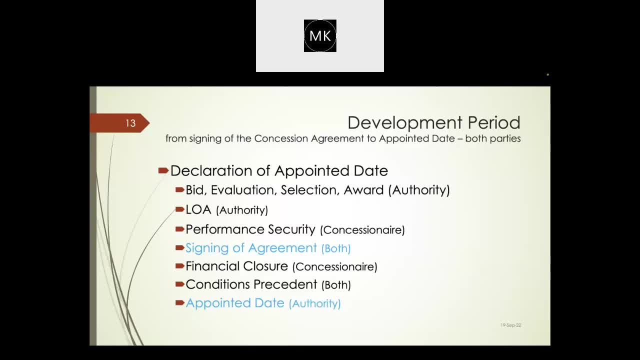 They are the responsibilities of both the parties. From the client side They have to. they have to procure the clearance, environmental clearance. If there are any ROBs, those ROBs have to be cleared. The general arrangement rights have to be cleared, like that. 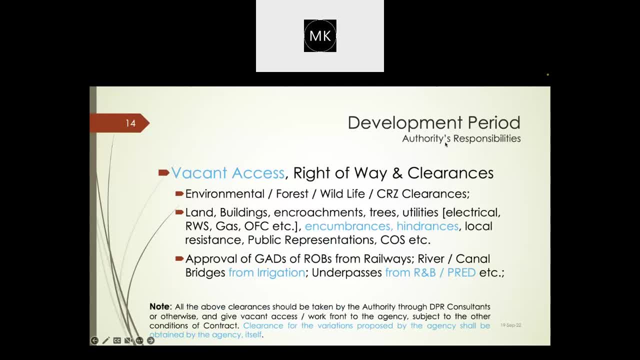 Then concessionaire, of course. basically he has to achieve the financial closure, but he also will have some other responsibilities, and then the appointed date is declared. Then now, once it is- of course we are still in the development period- the primary responsibility. 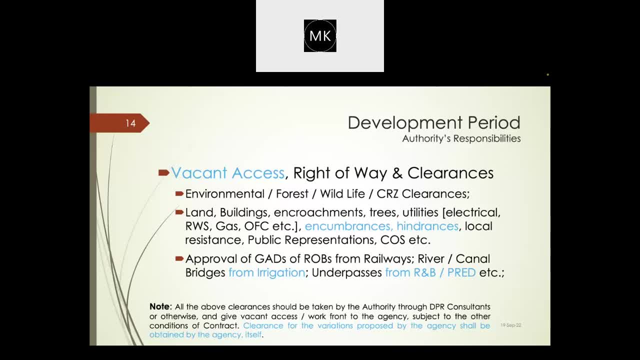 of authority During the development period is providing vacant taxes. Vacant taxes should be understood properly. It is not just a declaration of 3A, 3D, 3D, something like that It is. there should not be any hindrance in the site. 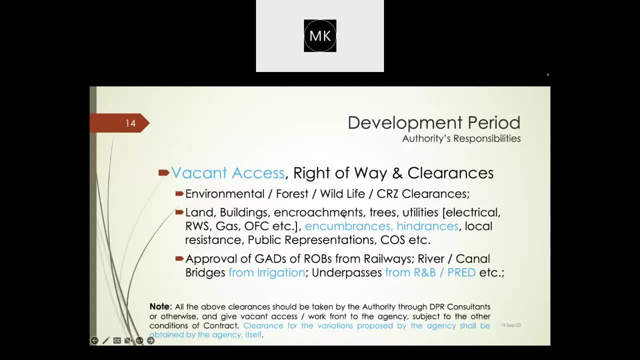 The contractor should be able to put his machinery and start working. There comes that is called vacant taxes. There comes the difference between these two words, encumbrances and hindrances. Encumbrance is a legal one That means that is. 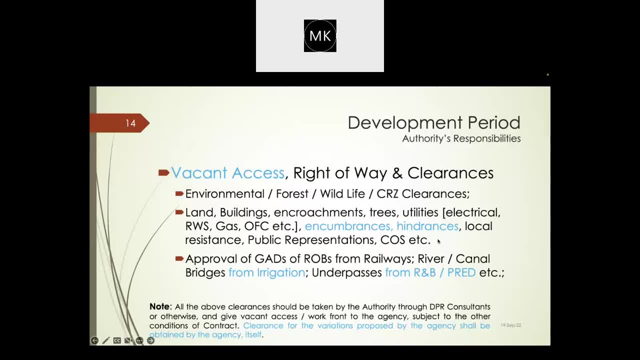 There is a court case attached to that and you are not able to enter. legally That is called an encumbrance. Encumbrance may be removed but there could be some hindrance over there. It can be an electrical pole, water pipeline, tree, anything. 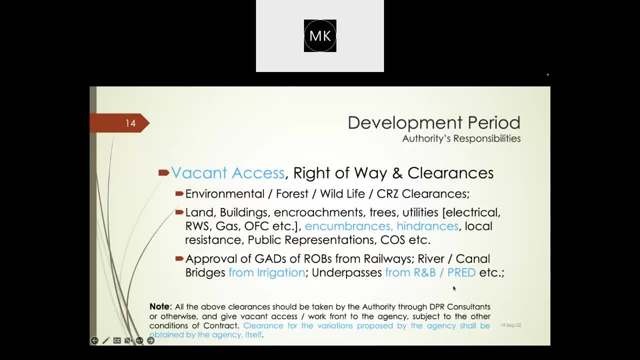 So all these things have to be removed. That is called vacant taxes. That is what we have to understand. During the development period. the authority also has to get clearances from irrigation, clearances from R&B, PRED for the underpasses and other structures. 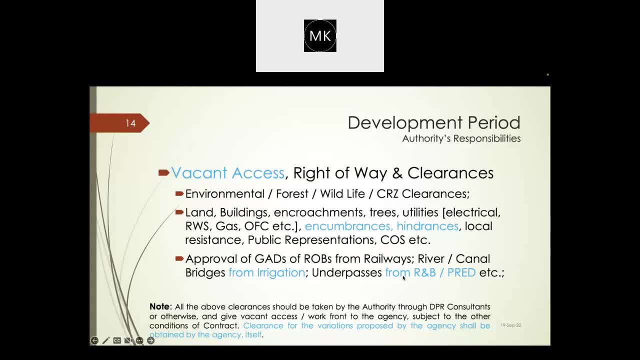 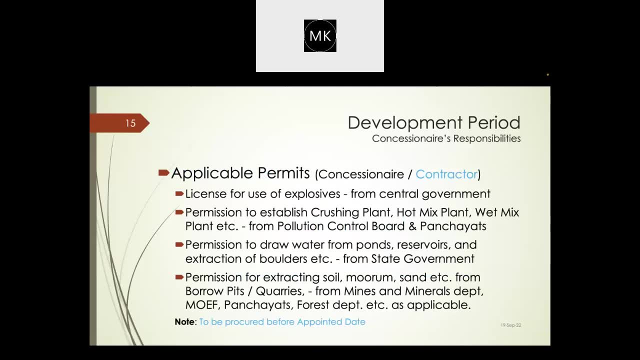 If we are having anything on the minor roads, okay, whether we do it through DPR consultants or we do it ourselves, but this responsibility is with us, it is not with the concessionaire. This presentation- copy of this presentation will be provided to you, so the details can. 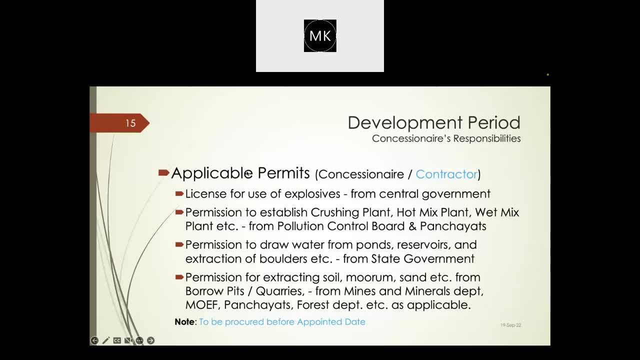 be read Now: during the development period, what does concessionaire do? He has to procure applicable permits. Whether it is contractor or concessionaire, These permits are necessary Whether a development period is there or not. even contractor has to secure these permits. 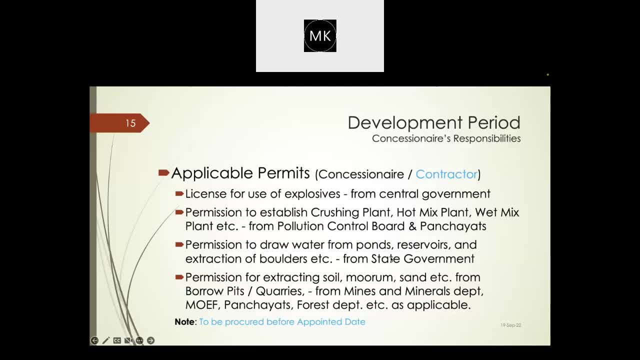 Explosives. then for establishing plants, pull it from Pollution Control Board or panchayats. we have to get clearances, Their permission to draw water from ponds, and we have to get it from state government Permission for extracting soil. whatever material that is going to be incorporated into the project, 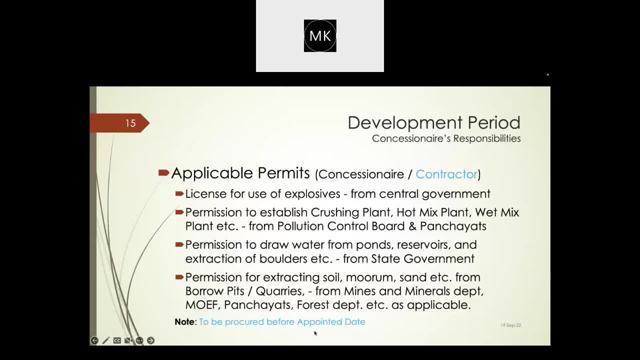 It may be from MOEF, depending upon the area: The 5 hectares, 10 hectares depending upon the area. we need to even get clearance from MOEF, panchayats, forest departments etc. But, mind you, these have to be procured before appointed date. 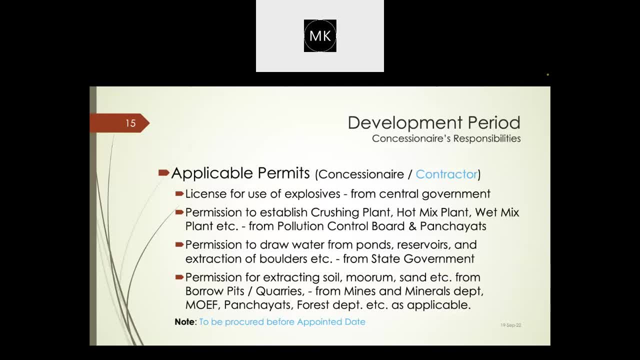 This is very, very important in the sense that tomorrow, when he is going for a claim in one of the projects, it so happened that after the appointed date, there were certain changes in the procedures for securing the MOEF clearance or permission for this. 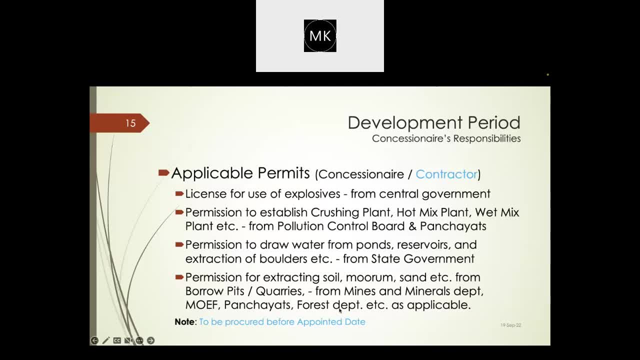 So this is very important. So they started putting it on us, on the authority, that this is not attributable to me. I could not get it because they changed the procedures and all, but they changed it after the appointed date. So when it is after the appointed date, we told that we can't give you any extension. 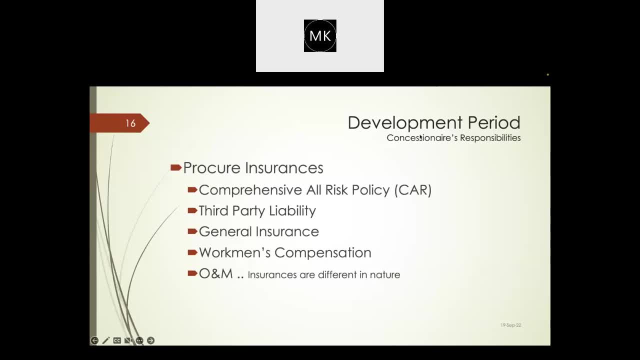 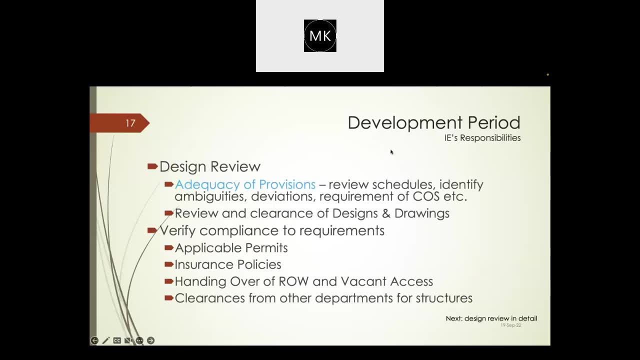 of time. You could have done it before the appointed date. Now, after procurement of permits, they are also supposed to procure the insurances. Various insurances will be there. we can see in the document. This is also concessionaire's responsibility. 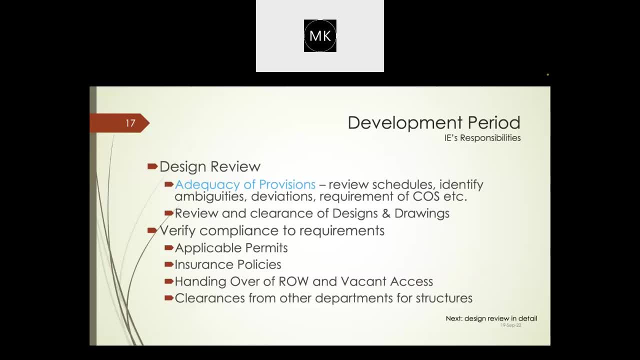 Then, during the development period itself, the concessionaire is supposed to do the topography surveys, prepare the designs, drawings and everything and then submit it to the authority And of course the independent engineer or authority if he is there. So then the role of IE during the development period is do the design review. 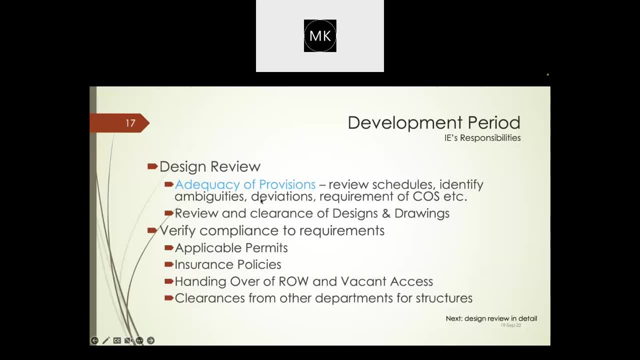 The most important thing is people think that it is only review of designs and drawings. No. First of all, design review starts with the adequacy of provisions. So we have to review the schedules, identify the ambiguities, deviations and, if any, COS. 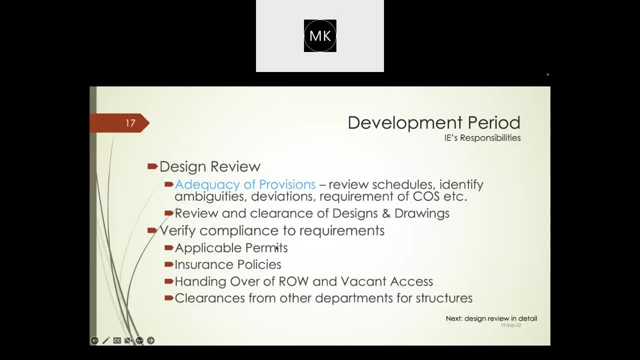 is required or not. This is very, very important. This is a part of design review. We will go in detail Then verify compliance to the requirements. I told you about permits. So did he take policies? insurance policies did he take? 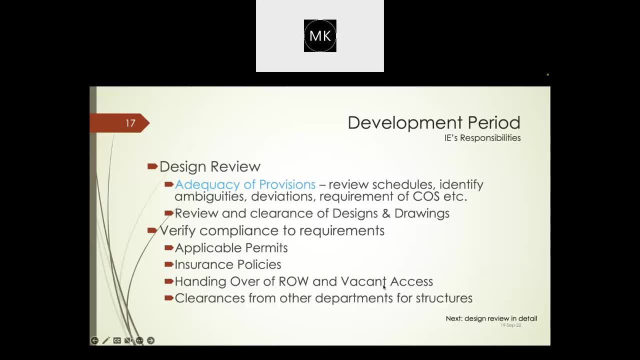 Then also IE has to verify whether the ROV and vacant taxes have been provided by the authority. So from the concessionaire side and also the authority side, So is it given He has to maintain records, not that he will go and get the ROV cleared and clearances. 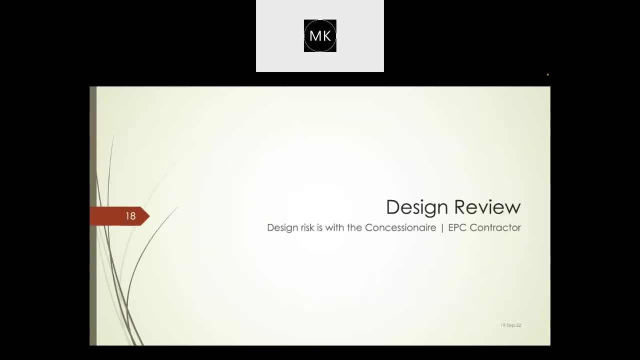 from other departments, whether they are there or not, like for irrigation structures, If there are big bridges, Ganga and all that, whether there are clearances available, Then now design review. So here the most important thing is design. the risk is with the concessionaire or APC. 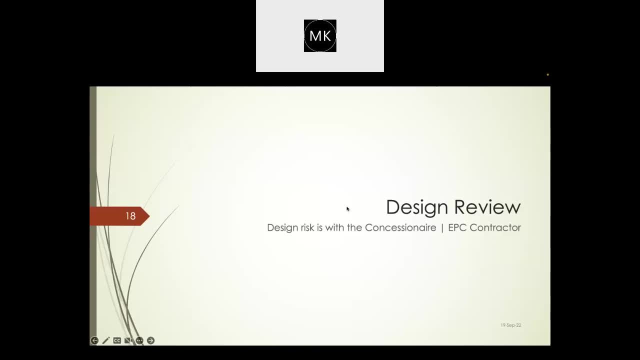 contractor. They may be redesigning the whole thing. The drawings that we give may be from feasibility or maybe from DPR, but they will be redesigning And so the design risk is with them. So what we do when the risk is with them? we only declare some things that it is within. 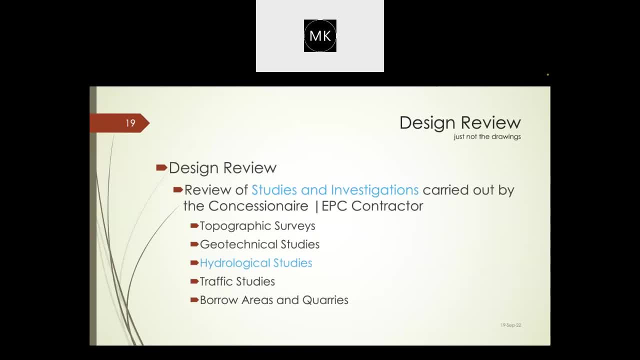 the scope and it complies with the specifications and standards, something like that. Now, design review: As I told you, it is not only the drawing. So, and first of all, adequacy of the provisions in the contract that we have seen in the earlier. 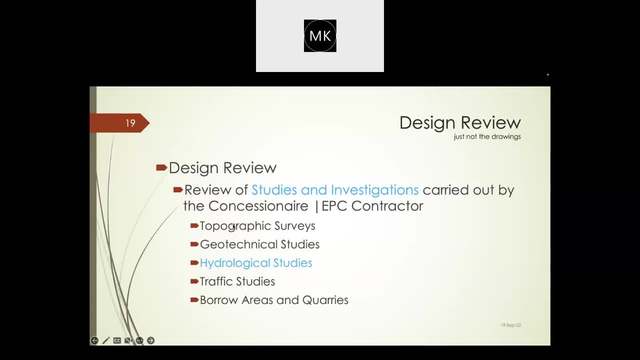 slide. Now, here it is: studies and investigations. These reviews also have to be done. We should not say that, no, no, no, it's not my responsibility, It's, of course, it is his responsibility. Now, what are the various things? topo, geotechnical, hydrological, traffic studies and barriers. 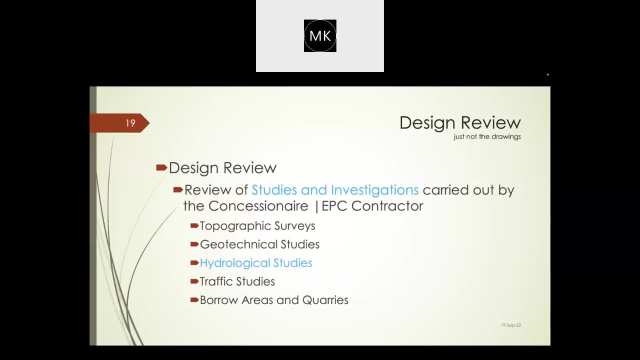 Why I have highlighted this in one of the projects, somewhere in Arkanth or in Bihar, I don't remember exactly. So after one year, After one year of executing around 22 well foundations, then the authority engineer was appointed. When the authority engineer came to site he told he was reviewing hydrological studies. 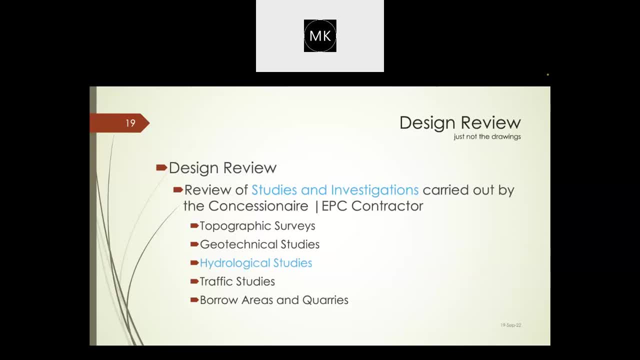 and hydraulic studies. And then he said that the discharge that was considered is less and the scar depth is also less than the foundations are above the actual requirement. So that was the first step, Then the second step, Then the third step, Then the fourth step. 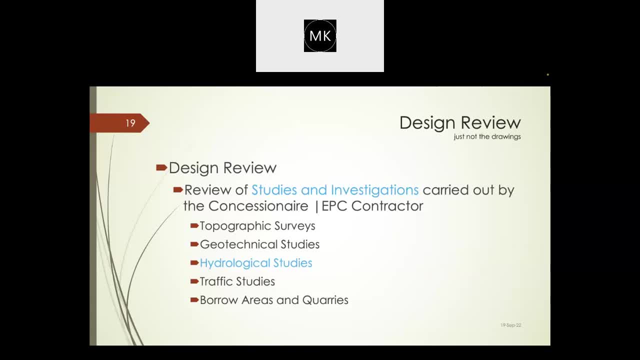 Then the fifth step, So all that he has found. So appointment of the authority engineer or independent engineer at the right time is very, very important. But of course the DPR consultant could justify that: the hydrology, the HFL and discharge. 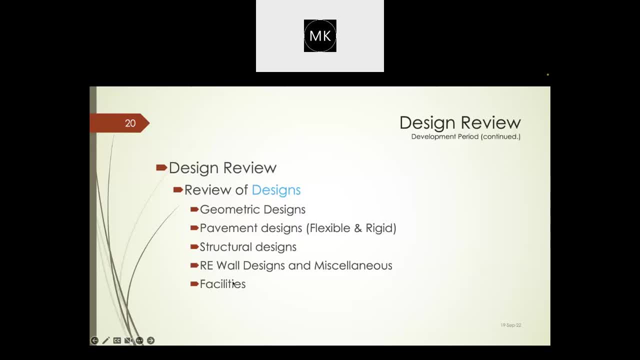 whatever they have considered is appropriate. So they went ahead. So it's very important. Everything has to be seen Now. review of design: of course there are various designs, It's not only structural designs. So geometry design, pavements, structure, RU, wall, facilities. 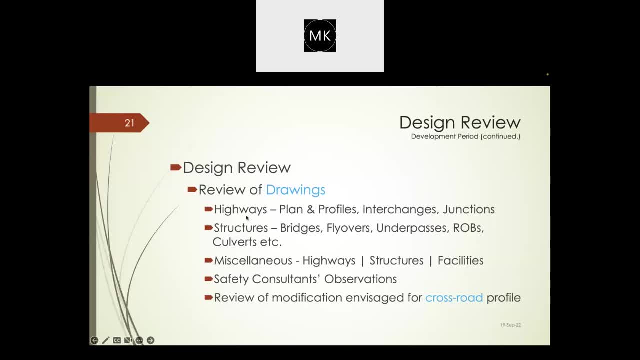 All these things have to be Reviewed And quickly going through because you might be already knowing them. Then review of drawings. Drawings are not only structural drawings but highway plans, profiles, and there will be junction drawings also. These people generally the concessionaires or the contractors- they put this to the end. 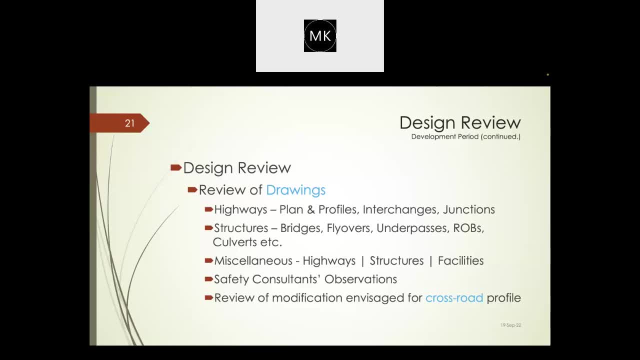 of the contract, So they are never ready. So it should not be like that. All the components should be designed together in the beginning of the project And during the development period more so, So that designs are in place and is in place and the contractor can simply go ahead. 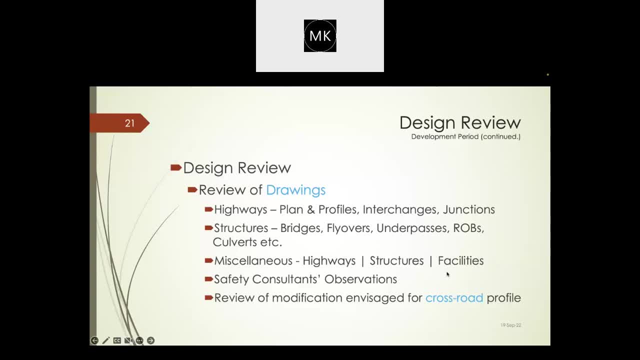 The structures, of course: bridges, flyovers, underpasses, all this stuff. miscellaneous facility designs also are important. Bus bay design cannot be left to the end, and any other, like rest areas, safety consultants And another thing is the crossroad profile is also important. 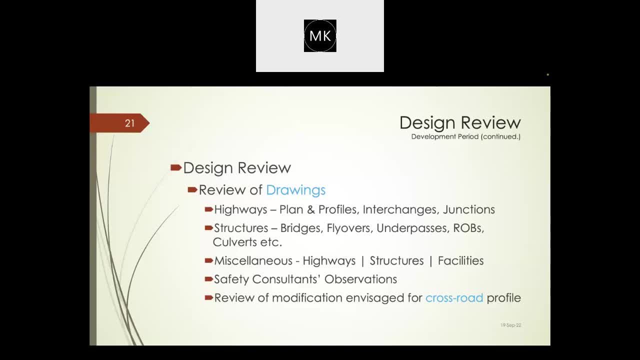 Some of you are from the state departments And you might be having Some plans for development of the crossroad. But the main highway, when we are doing the crossroad development, if it is not considered, then we may be providing too little clearance. 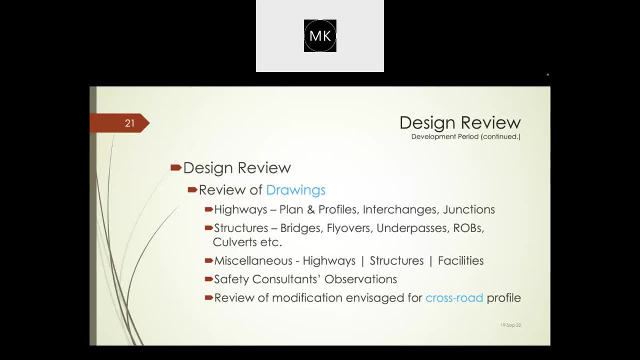 Suppose 5.5 meter is required. We have provided 5.5 meter, But there is a 1 meter increase in the crossroad profile and the clearance will get reduced to 4.5.. So it is very important. In one of the cases in Andhra Pradesh, when we were doing this, the State Department has. 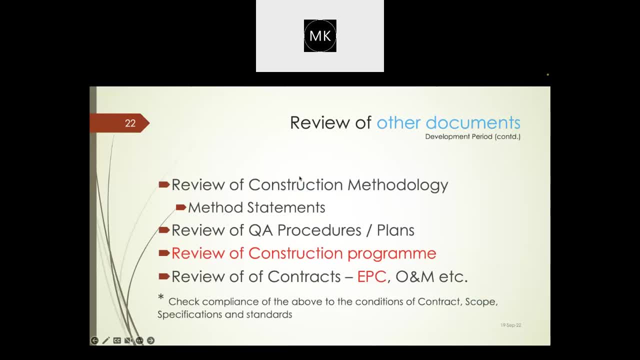 put around 35 lakhs of penalty on NHI for wrongly designing this. Then review of other documents. This is also to be done in development period. We have to see that this gentleman submits all these things during the development period And as authority, we have to see that IE is in place first of all during the development. 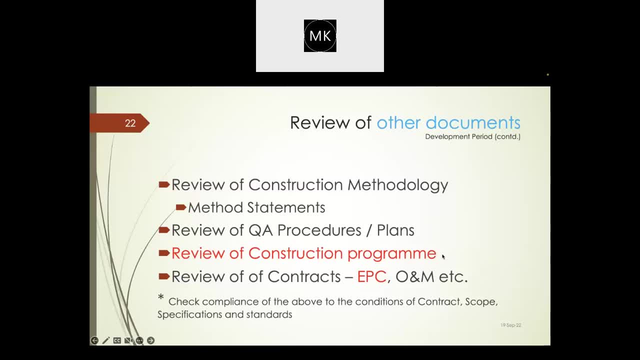 period. So construction methodology, method statements, QA procedures, What there is to be done, So this is also to be done in development period, What they are going to do, And the most important thing is review of construction program. If you take even this one idea from this session to your life, I will be very, very happy and 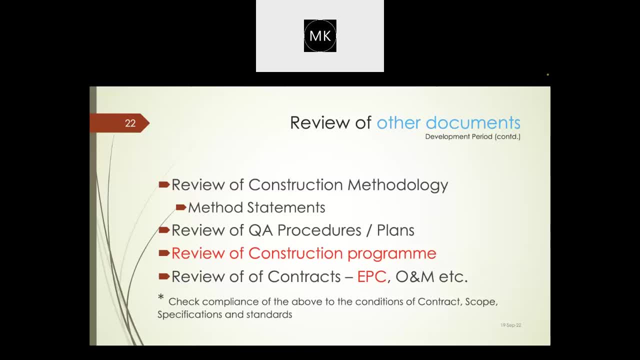 I will feel that, yes, my new purpose is served. We have to review the construction program And I will discuss in detail as to how to review it. what are the qualities of the construction program, how it will be useful in the course of the construction. 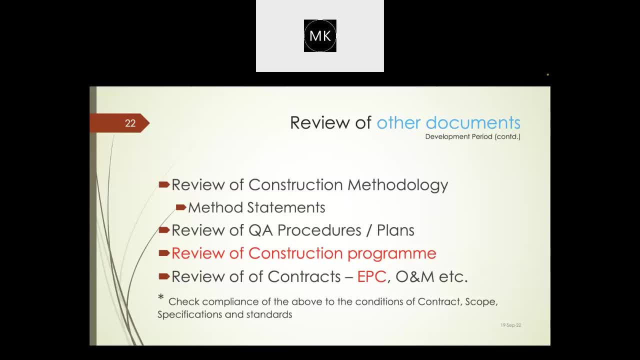 That we will discuss. Then review of contracts- EPC contract, O&M contract, like that- See what happens. you know, these people are very notorious, Sorry to say so. I'm talking about concessionaires. So they actually say 70, 30 or 80,, 20,, 80% debt and then 20% equity, like that, if it. 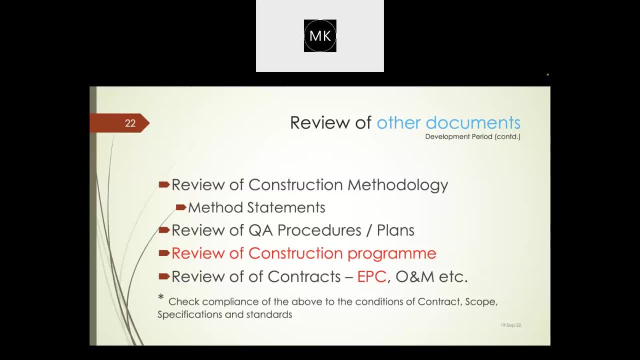 is there. They structure the financial in such a manner that the 20% amount they draw in the beginning of the project itself, the equity they draw in the beginning of the project itself. So whatever they have put, they got it. Now: the debt servicing and toll. 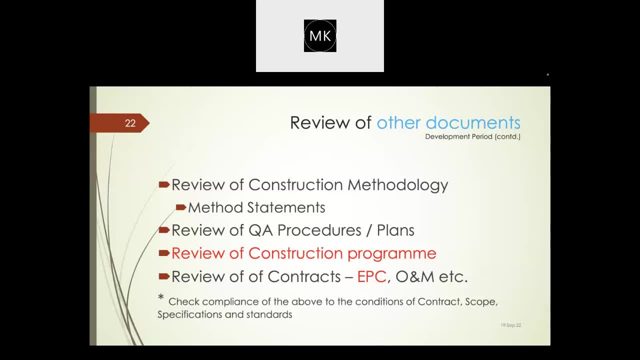 So they have nothing to do with the project. seriously speaking, The debt servicing will be done by the toll or any other revenue that is going to come. It may be annuities and all. So now, the way they do this is through EPC contracts. 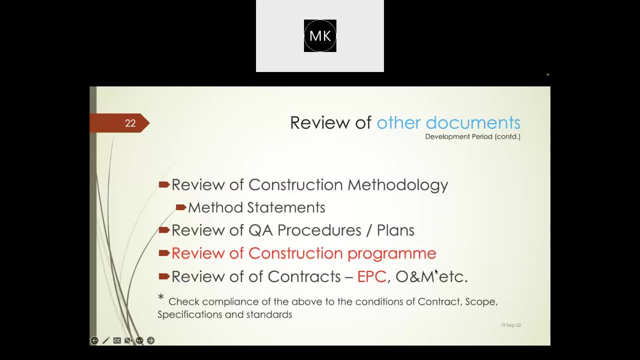 Generally the concessionaire and the EPC contractor are same. In fact, two people come together and make an SPV And the SPV Gives the EPC contract to themselves. So we have to review this EPC contract very much and they load them up front. 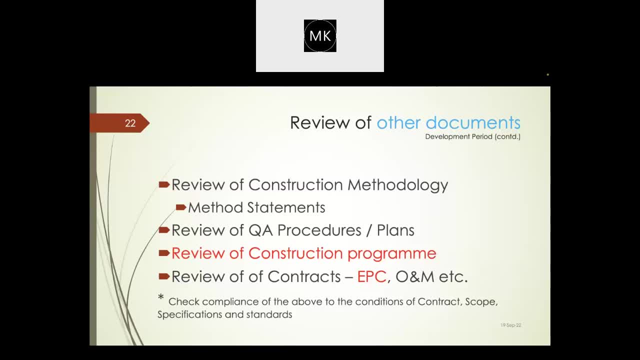 Say the varying course constitutes around 45% of the contract. They put earthwork as 45% so that they will be able to give that money to the EPC contractor. They will be able to take out the money through EPC contractor early. 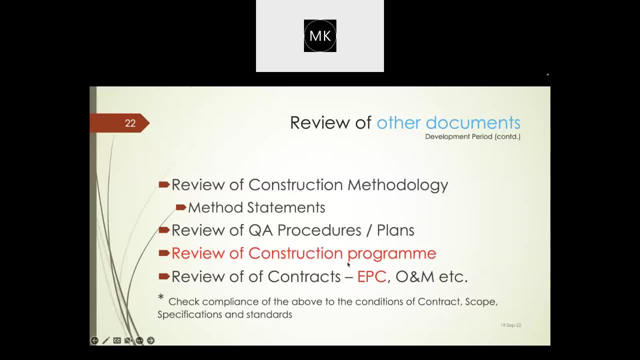 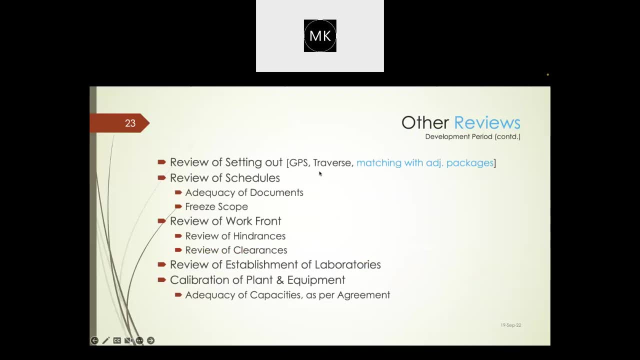 So these things are very important. So we have to focus on the review of the EPC contract. These things come into our help when we are doing termination payments and other things. Then other reviews setting out: We have to go and see exactly whether the GPS pillars are there, traverse pillars are. 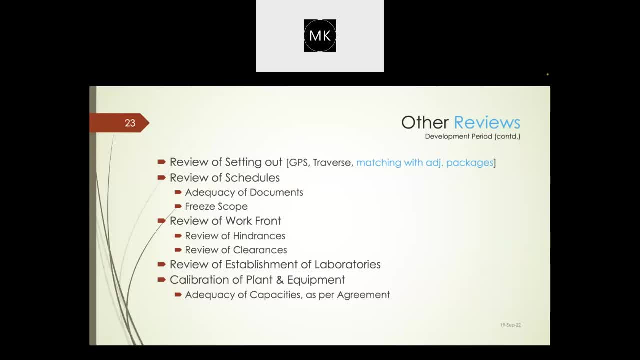 there and TBMs are there every 250 meters And the most important thing that I have seen is that we don't check actually the addition packages In a very important expressway project where we were doing, of course. see, I can only 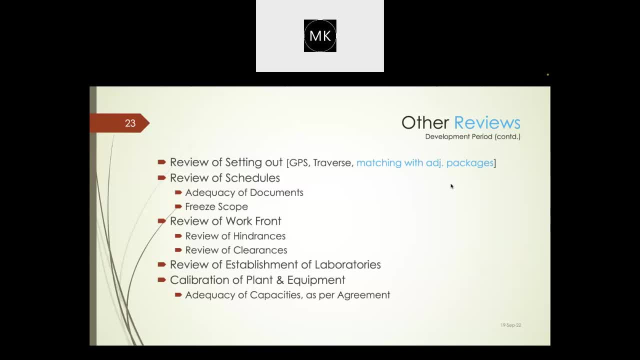 give examples from my own projects. So if I'm telling something generally, it is from my projects. So we found that those people they did not check what is happening in the junction. So it was there was a mismatch. So you can, you can understand what can happen. if it is a simple road, it was okay. 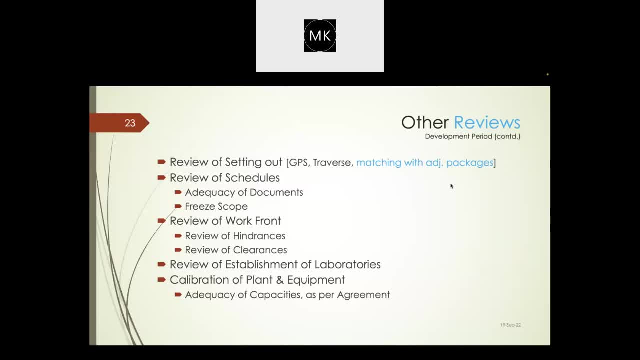 But it was exactly split at the structure, So One structure was in one package and the approach was in another package and it was so difficult for me to correct it. So it is very important initially to understand whether the levels are okay and the alignment. 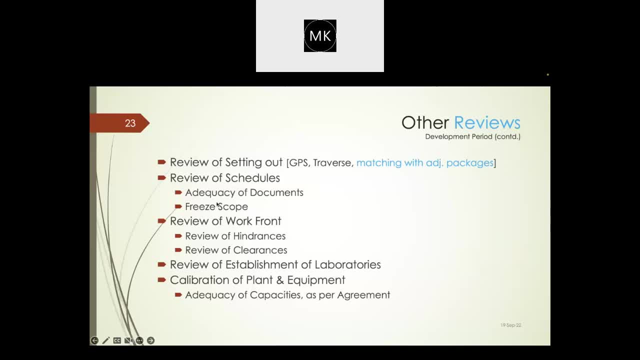 are matching. Alignment is matching at the packages, at the joining of the packages. Then we have to do the review of schedules for adequacy of the documents And we have to freeze the scope. See, this is freezing The scope. is very important in avoiding time overrun. 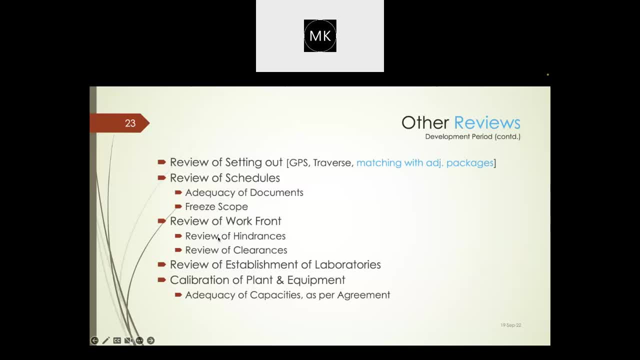 This is how we tell you towards the end of the project: Okay, Thank you. So we have to review the schedules and we have to review this. we have to freeze the scope Parallely. we have to review the work front also. 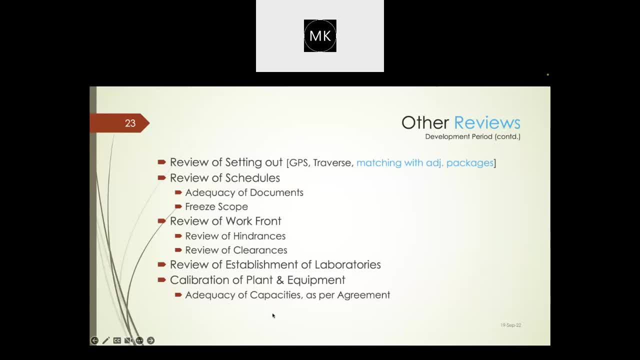 This is very, very important. We focus on something else instead of giving work front to him: Review of establishment of laboratories, calibration plant and equipment, And also we have to see the labor establishments, labor camps and all whether he's having facilities. 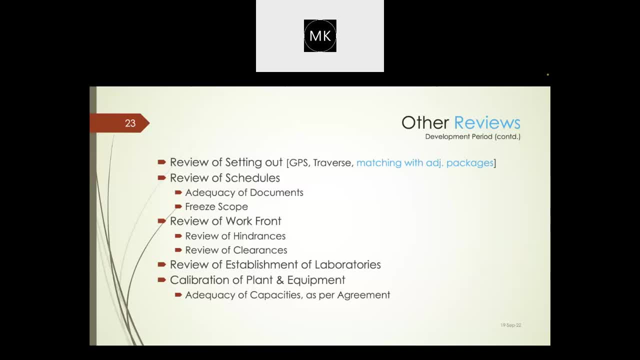 or things. That is also very, very important- The people who have seen the entire cycle of the projects. And if you have gone through the claims of the contractors, then you would understand why we should see the labor camps and why we should see exactly where the plants are. 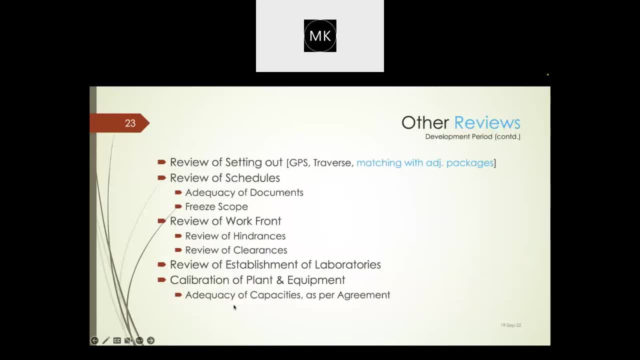 and whether they're in working condition. They are just dumped because they don't have scope elsewhere. They have just dumped them. Ultimately, you know, they will charge the idling and other things on us. Another important thing is we have to check whether they are having adequate capacities. 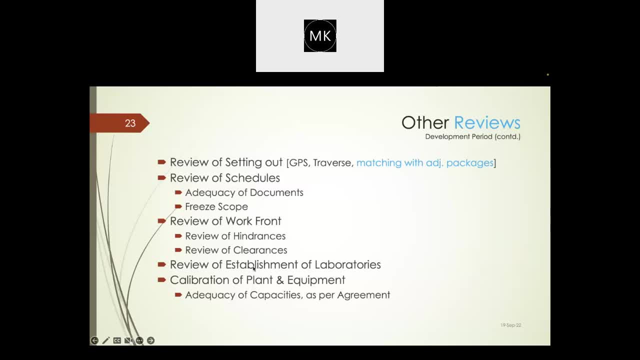 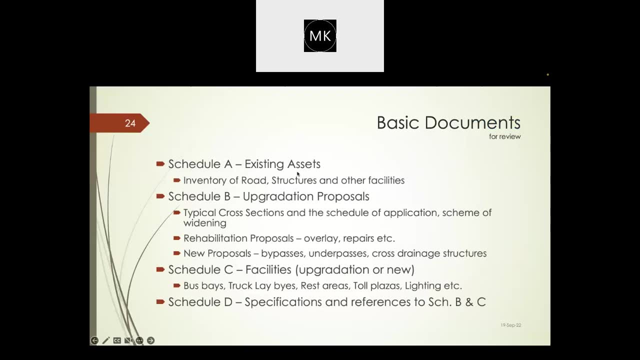 as per agreement. Agreement says 200 tons per hour and they might have provided 100 tons per hour. Those things are required to be checked. Each line, whatever I have provided in the slide, is important. It will be useful if you go over these slides after the program and even afterwards. 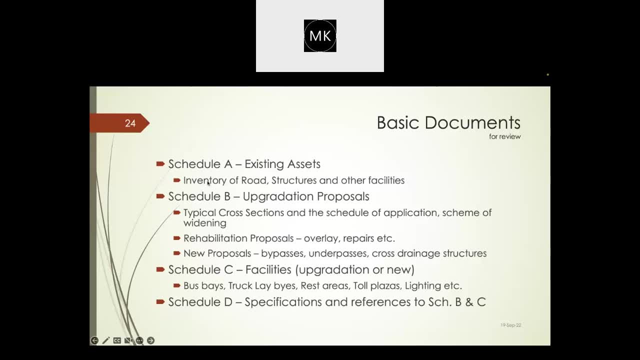 Now you know that Schedule A either it is in, either in concession agreement or EPC contract agreement. Schedule A tells about existing assets, So we have to review them, review the inventory of road. These are the things. anyway, This will be there in Schedule A, and Schedule B consists of upgradation proposals. 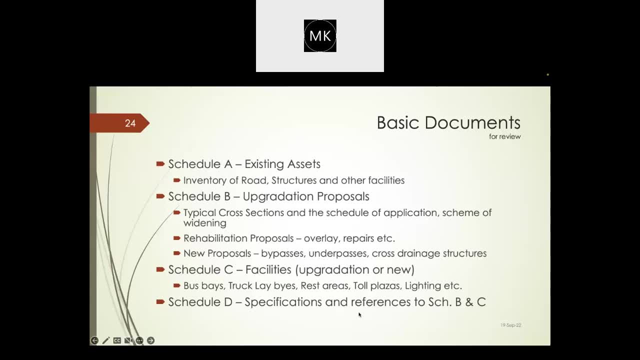 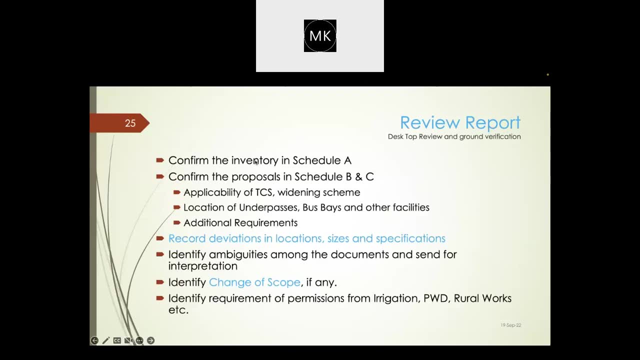 It may be road and it may be structures. So then, Schedule C: it gives facilities, whether it is upgradation or new, and Schedule D is specifications and references. So these things, these are the documents for review, And what are we supposed to do with the review? 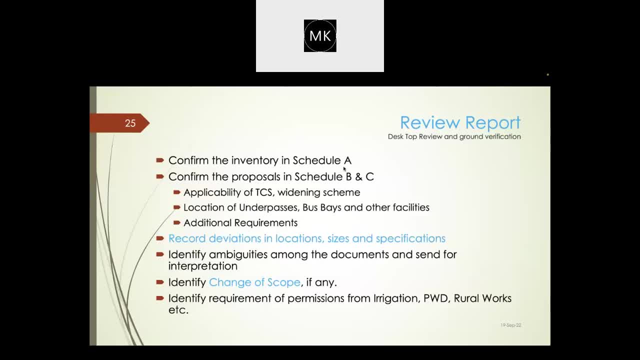 The first thing consultant has to confirm the inventory in Schedule A. Whatever the information is given in Schedule A, it is correct, sir. no missing, no wrong interpretation When we are telling that it is two-meter culvert. it is only one meter. instead of slab it is. 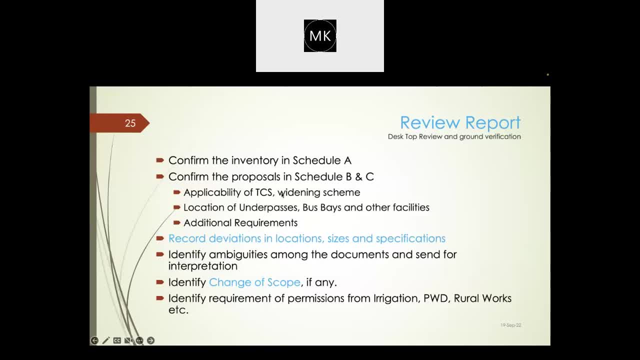 only pipe, whatever. we have to confirm the inventory in Schedule A. We have to confirm the proposals in Schedule B and C also whether TCS it is correct. TCS has been applied, widening scheme left, right and concentric, whatever. whether it is proper, whether it. 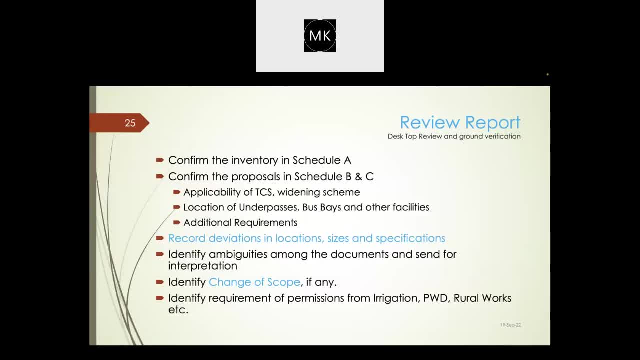 is correct, Whether it is properly given or not. So exact scheme we have to confirm. If location of underpasses it could be plus minus one kilometer, half kilometer, 10 meters, whatever then bus base and other facilities, bus base, they are provided at a place where 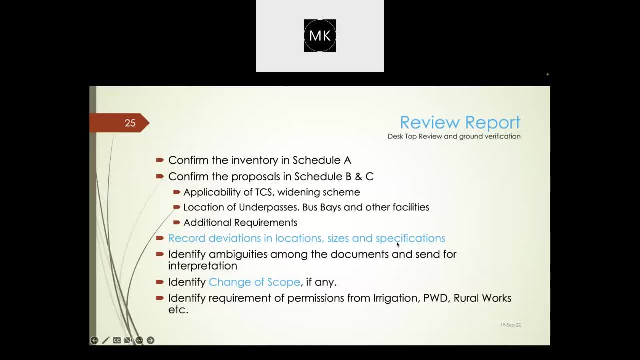 they will not be used at all. We have to put the bus base and bus shelters at a place where they will be useful. Then additional requirements, if there are any, that also. So ultimately, we have to record the deviations in location, sizes and specification during. 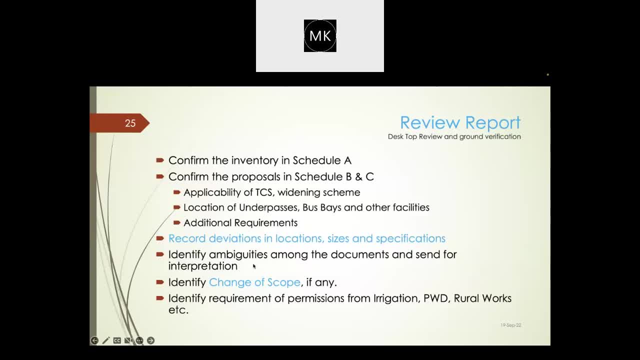 the review. If we don't do this, But if we keep it, if we defer it to some other time, then we are only going to suffer as authority and also the contractor. Identify ambiguities, if there are any ambiguities, and identify the change of scope. 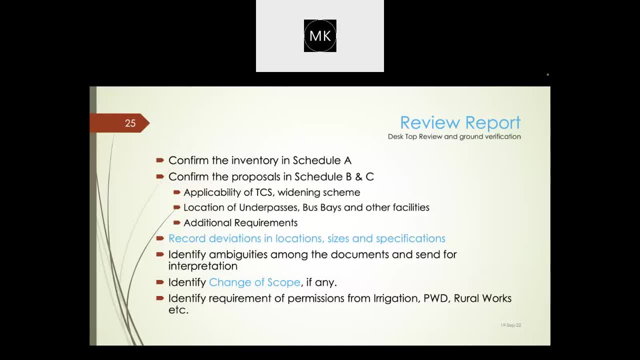 This should be done during the development period itself- That is what I am trying to say- even before the appointed date, or at least within three months of appointed date or commencement date. then the project will be in shape A lot of them, So we need to keep it in mind. 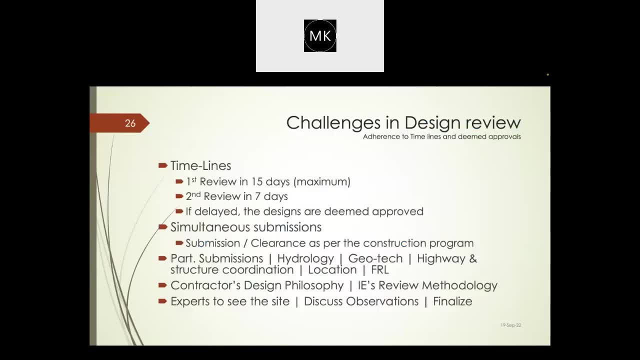 I just think that whatever I want to dump, I will just dump, and it is. I is responsible, he is responsible to do, You are also responsible to do. Yeah, Okay, Thank you very much, Thank you very much. 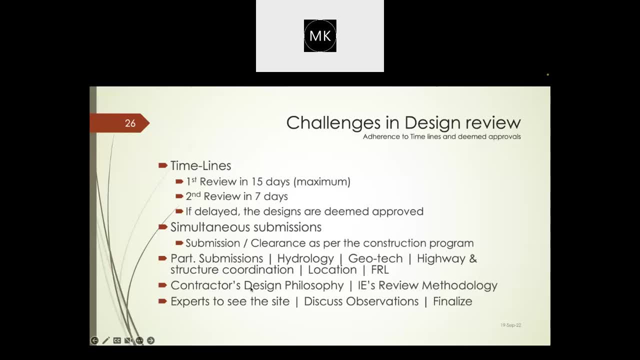 you to review, and if they don't review, if you don't, if they don't approve, i'll go ahead with the construction. this kind of a thing should not happen, so people should sit together and agree on their design philosophy and the review methodology. experts must see the site and discuss observations. 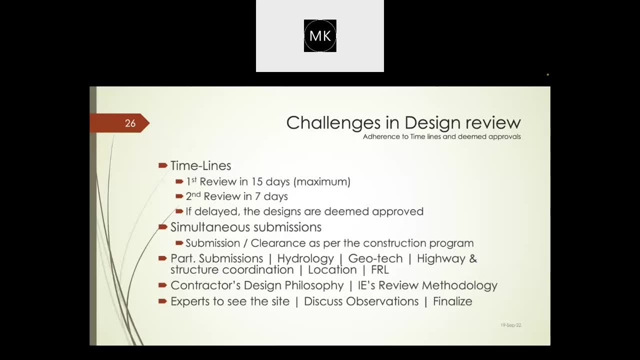 and finalize, because with every site is different. vup may not be vup, a simple vup. everywhere it might be having drainage problems. the crossroad may have different issues. all the water might be coming over there, only we have to check whether it is below the existing ground or above the. 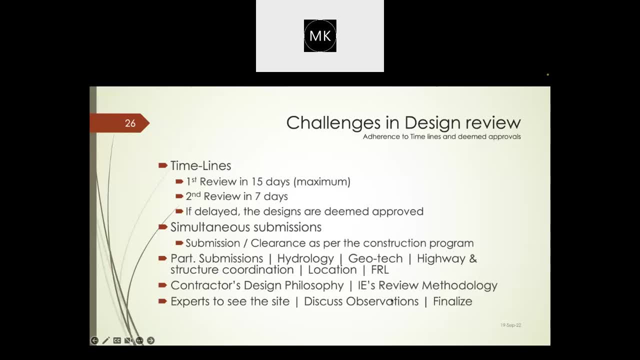 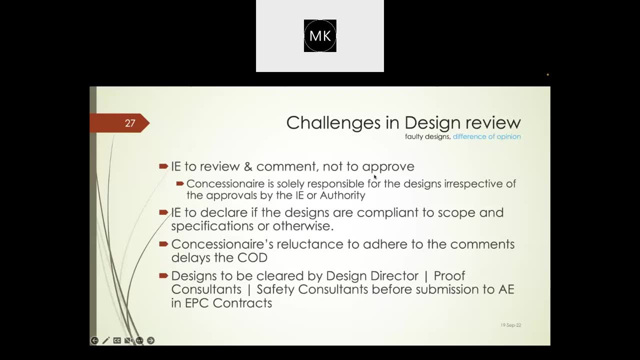 ground, whether it is on crust, whether the location is proper or not, anything. ultimately, it is important that experts should see the site and then only review the submissions. the most important thing is that ie has to review and comment, not to approve, even in the case of you. 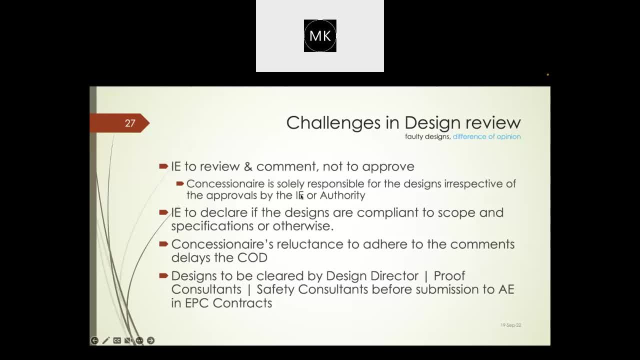 also they are not supposed to approve. there could be places where he has to approve, but generally it is so because concessionaire is solely responsible for the designs, irrespective of the approvals by the year authority. you might have might be already knowing: even if the authority approves the drawings designs, even if the ie approves the drawings designs, it is the responsibility. 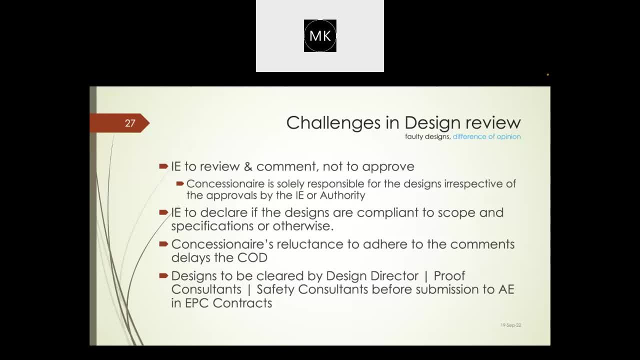 of the concessionaire and epc contractor to see that they comply with the specification, standards and codes, all that. so that is the reason why ie has to only review and comment and not to approve and what he is supposed to put. the stamp he is supposed to put there is designs are compliant. 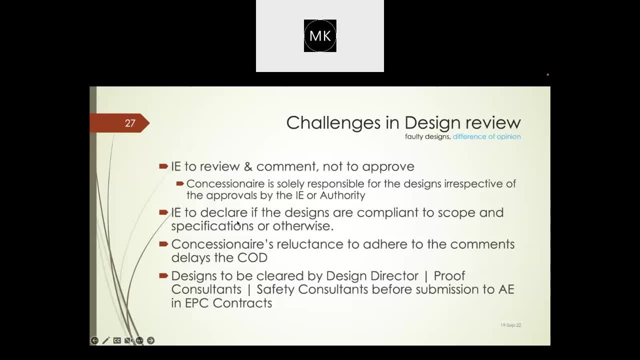 to scope and specifications or designs are not compliant to scope and specifications. that is what is he, what is the certification that he is supposed to give? and one most important caution that i would like to give is: there are failures in the structures, quality and collapses and all. so the important thing is in epc, there is a design director there. 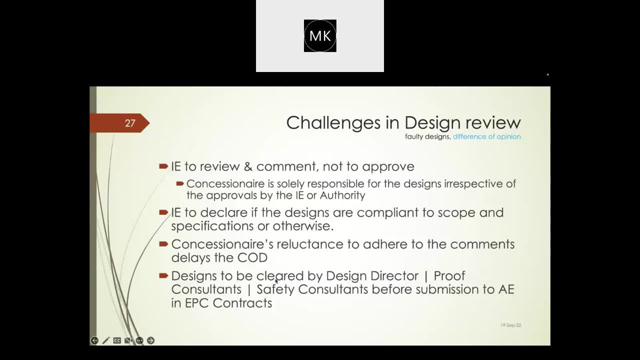 is a proof consultant, there is a safety consultant and after that it comes to the ae why there could be any design problem when it passes through so many. because they really don't do the thing. they simply dump the designs on ae, on ae, and ae is supposed to clear and 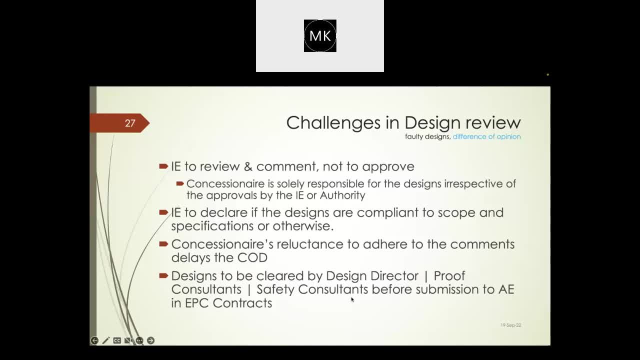 when he clears, all these people sign. so as authority, we have to ensure that these people are in place. all these people are in place and they do their, and they are different. you may be surprised. even one. only one person may be discharging all these responsibilities for namesake. only they are there, so we have to see that they are. 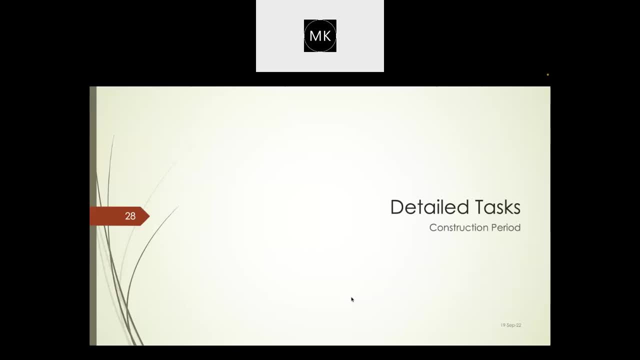 different from each other and they discharge their obligations, and proof of such discharge should be verified by us. yeah, so that is so far as a design stage, development stage, is concerned. we, if we quickly go to construction period, construction period- of course- we have got quality monitoring. that is very, very important, whether ie is having only two people or four. 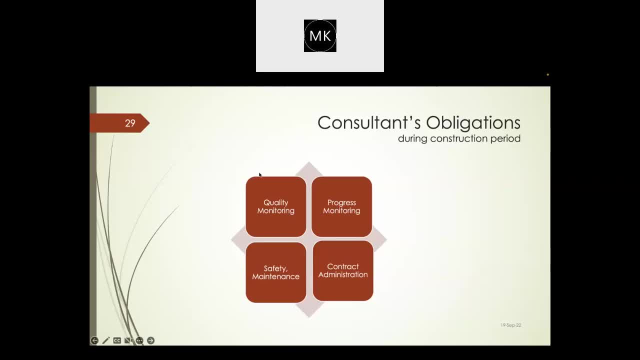 people. he is responsible for 100 percent of quality. whether he checks only 10 percent or 20 percent or 50 percent, he is responsible for 100 percent of quality. those things are there which are very, very you important and in fact after one, after the bot and apc, when they have come in, the quality has. 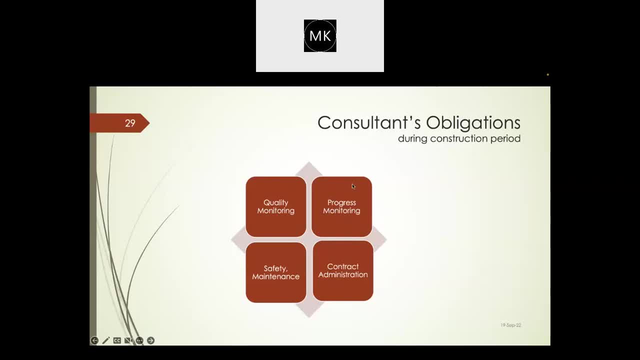 deteriorated. only for that reason- this is my view. then progress monitoring is the next responsibility. we can't keep quiet. this is where we have to compare it with construction program continuously and see whether we are going as per the program. then safety and maintenance of the existing road. 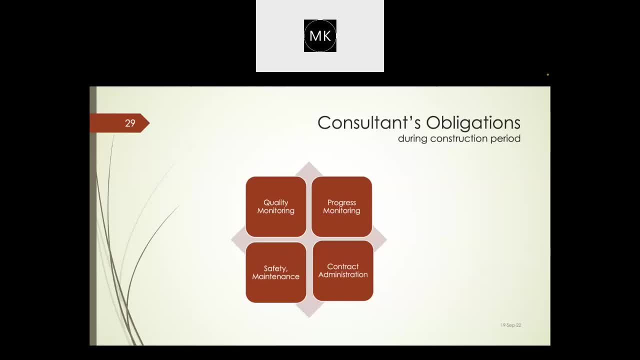 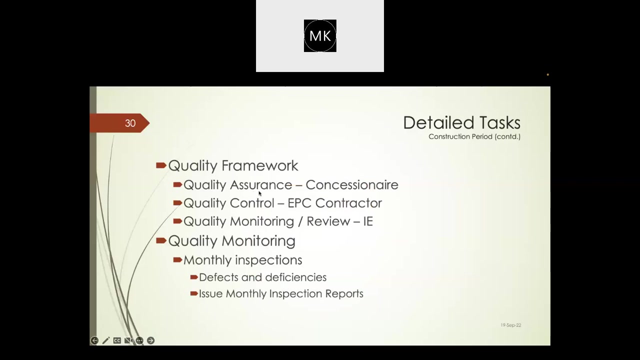 whatever is that is important and, of course, are what safety and maintenance means. when construction is done in those têmolo long, too long and it's a little bit switching off, or during construction also, the safety is very, very important. then contract administration. so these are the four responsibilities now: quality framework, quality assurance- who does it? 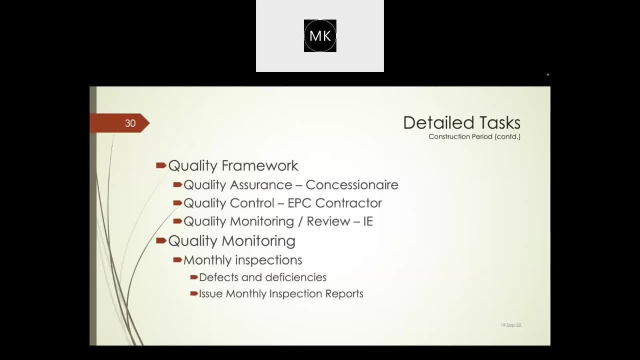 concessionaire: quality control. that is testing and all who does it. vpc contractor: what does ie or ae do? quality monitoring? he reviews the results. of course he also participate in testing- 10 or 25 percent as per the agreements. he does that so, but 100 program will be given to him. 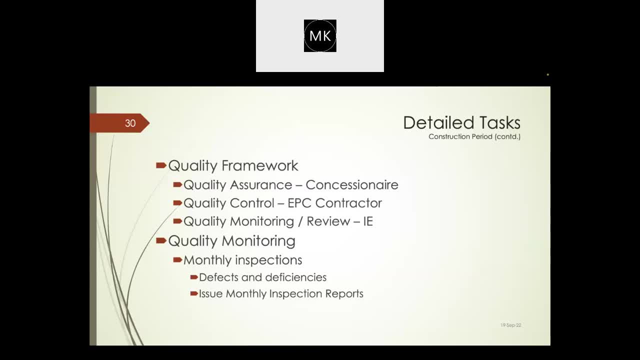 he chooses 10 or 25 percent, whatever, and then he attends to them and those must be held for his review. the contractor cannot go ahead all by himself without waiting for ie and there are monthly inspections. see, unfortunately, if you go through the documents, it says you. 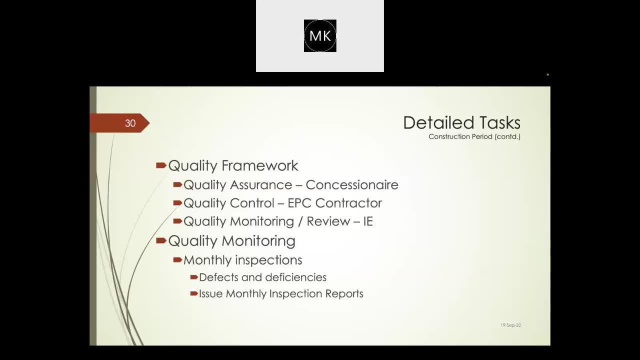 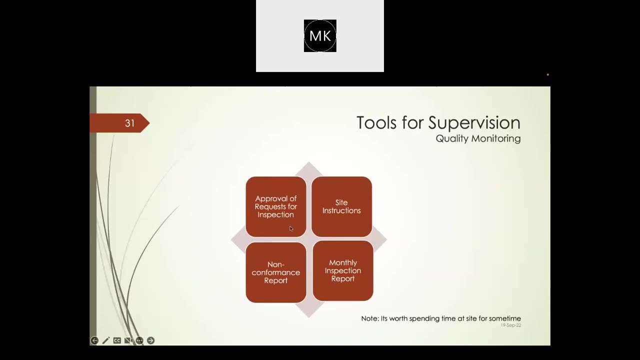 have to do an inspection at least once in a month. that kind of a language is there. so at least once in a month. you can understand it's only an audit. it is not a daily inspection. now, defects and deficiencies have to be identified and we have to issue monthly. 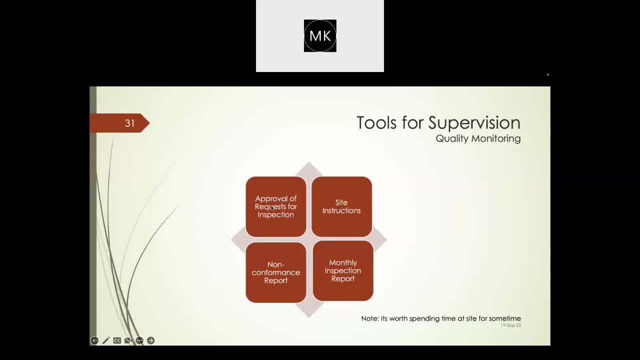 inspection reports. but there are four tools for monitoring, important tools in quality monitoring. one, as you know, is rfis. these have to be approved. the ones which we have to do are the ones which we have to do are. the ones which we have to do are the. 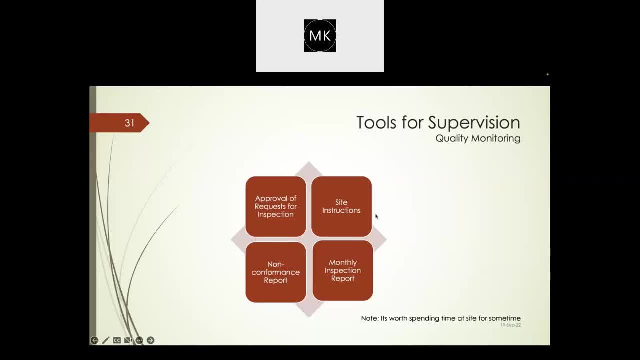 ones which we do not witness, they need not be approved. only those things which have been witnessed shall be approved. then that is not the only tool. you go, we go to site and we see that that rfa is not given to us. we are not supposed to see that, but something wrong is going on. so 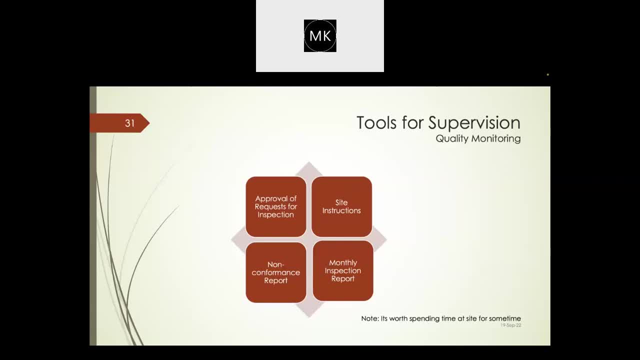 we have to give a site instruction. we can give you a site instruction over there. it can be in the form of a letter, it can be we can write in the register there so that all the instructions given are there in one book. so we can go to the camp simply write our instruction and come back. 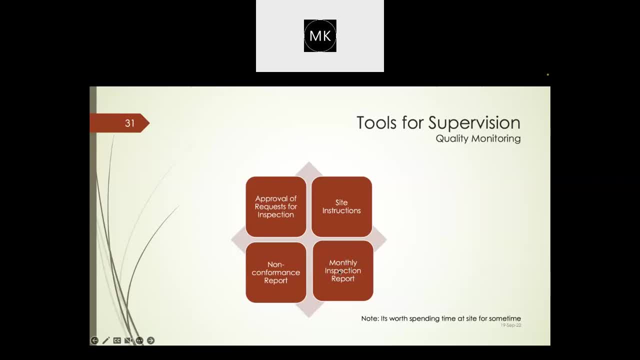 so that you can, we can refer back also letters. they are filed and you may know where they are and all. so that is one way of doing the site instructions. then you have got monthly inspection report. that we have. we are supposed to deliver as per the agreement. but the most important thing is: 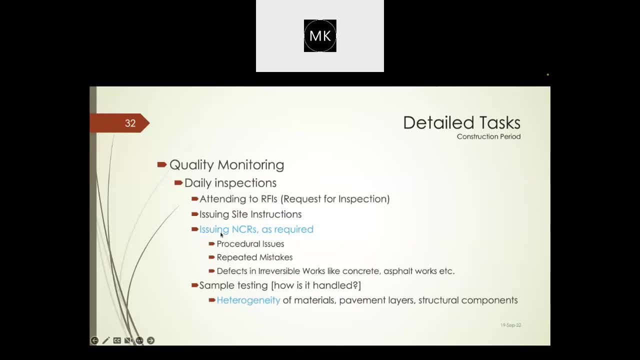 the ncr, now ncrs being indiscriminately used. so when to issue this and how to dispose this is very important. now, when are we supposed to give ncrs? when there is a problem of procedures, procedural issues are there. it may be say, a paver is supposed to be used, but whereas a grader is. 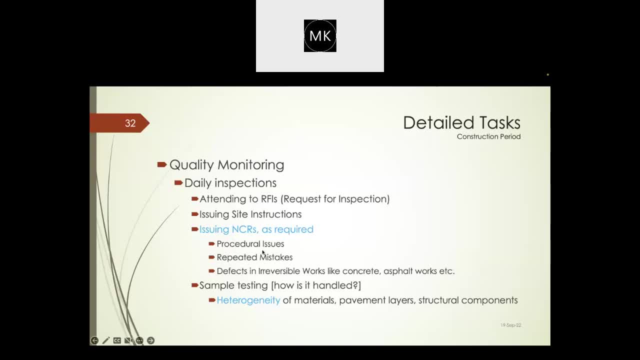 being used. a batching plant is supposed to be used but a drum mixing plant. a drum mix plant is being used like that. so at that point of time you have to correct it. even for curing, suppose he is supposed to use as in cloth and watering and all, but he is using a curing compound. 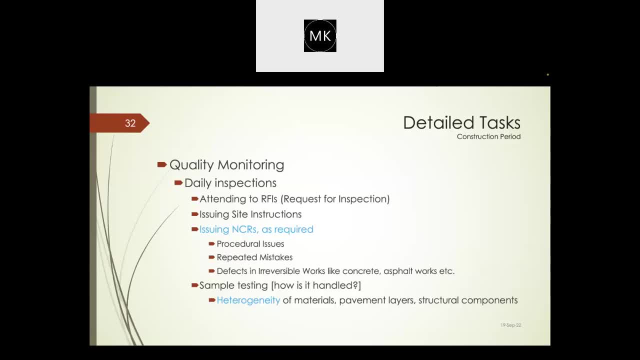 or vice versa, or he doesn't do anything whatever. there are procedural issues, so we will be, we'll have to give that. then repeated mistakes: he is doing same mistake on and all every time. so it can be anything in any procedure. so then also we should be able to issue, we should issue ncrs. 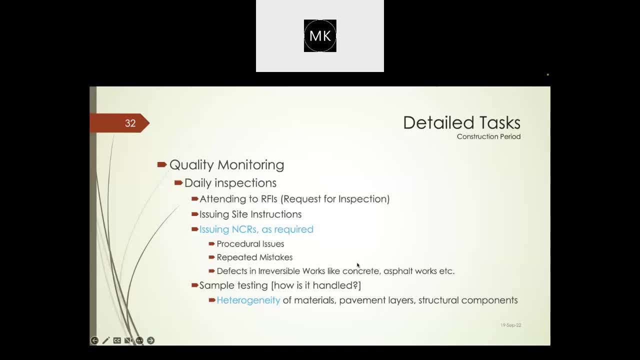 but the most important thing is defects in irreversible works like concrete, asphalt, like that. so, because you can't do anything about it, honeycombing has come, or after the casting of the concrete, the levels, the workmanship that is wrong, or it fails in compressive strength. so at that time it has to be put on record by way of an ncr and it must be. 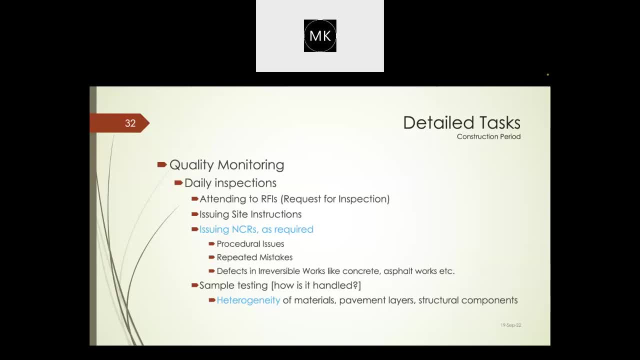 maintained separately. similarly, asphalt works. asphalt has been done and after that we see that there is segregation, raveling or crushing of aggregates, or the density itself is found to be deficient. it is deficient in density. so those are the times, so we should not give on small, small things. now. one important thing i want. 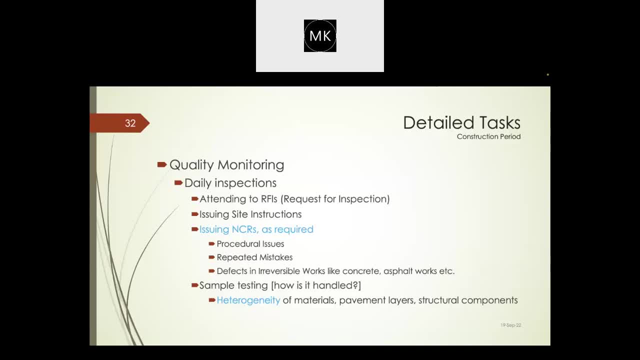 to mention to you here is: so uh, in most of the works where vigilance goes and resilience tests, what does it test? uh, there's a hundred kilometer project and they take uh two or three cores and those cores are deficient in either thickness or uh in gradation, or in bitumen content or intensity. okay, so they will say simply after: 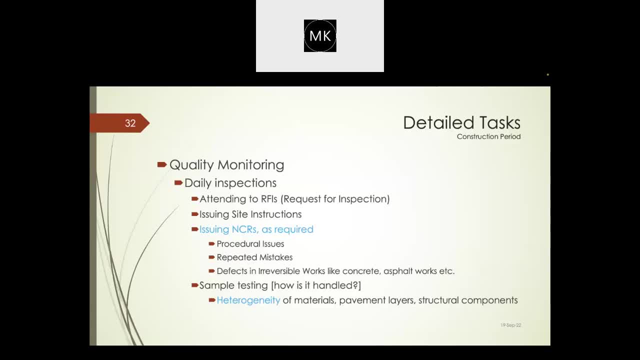 that if they're deficient, they'll say that yep, this project was not done properly and uh, he must be taken to task. and it becomes very, very difficult to discharge, dispose those, uh, vigilance observations. now try to understand the heterogeneity of materials. it may be in pavement layers or structural 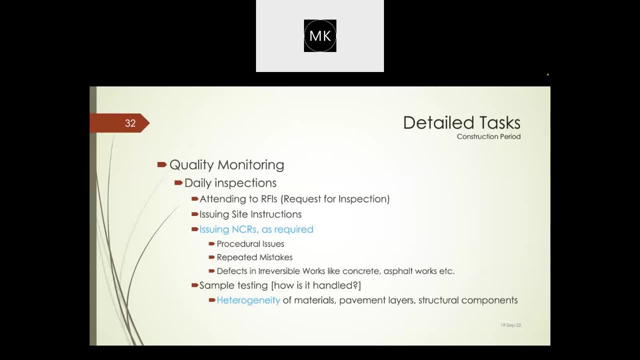 or you can display them in a very uniform way. uh, if you are going to use uh a, uh, uh a do, but you will see it, uh gets aggregated, we can, so in the with so much. is it really possible that you have a uniformity of all the properties? 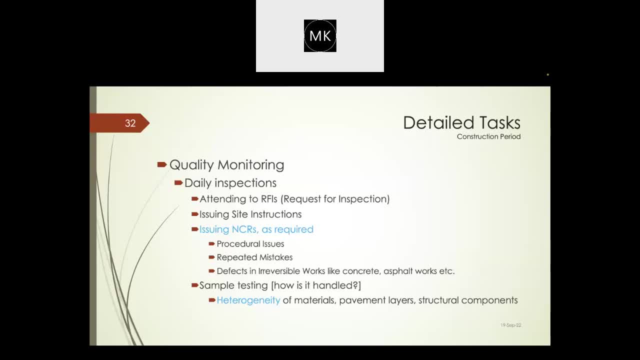 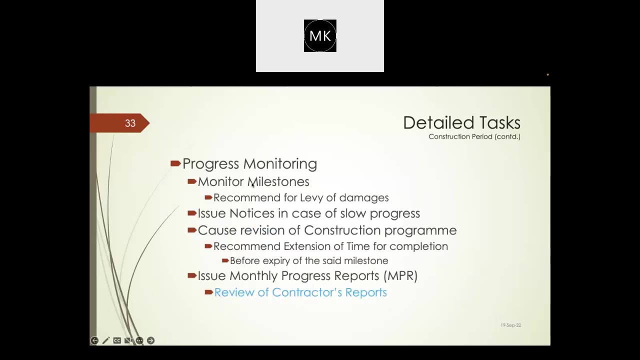 maybe thickness, all that? is it possible? let us take one meter, just for the sake of it, and in one meter square you, you take some eight to ten samples. all ten samples will be will be exhibiting different properties. you can check for the sake of it and understand so this. 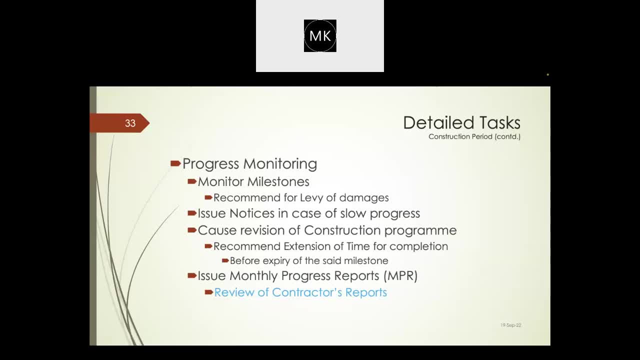 is very, very important how sampling has to be done. there are codes, progress monitoring. it's very, very important that we monitor the progress and monitor the milestones when exactly it is happening and then whether this fellow will be able to achieve the milestone or not. we have to be very watchful. we should not think that it is kind of contractor's responsibility. 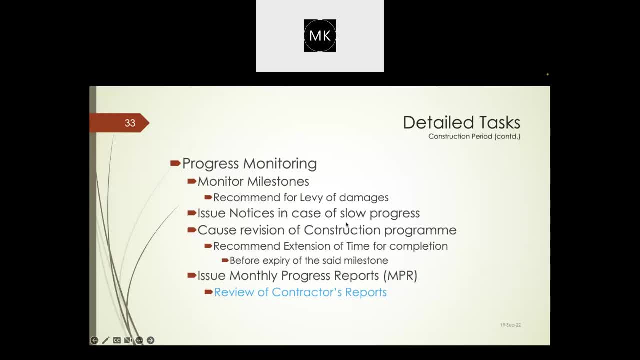 we have to be very watchful in this. either i, as ie or even authority, also you- and then issue notices of slow progress, then cause a revision of the construction program and recommend extension of time for completion before expiry of the said milestone. this is very, very important. we should not keep processing the thing. we should not initiate it first, after the. 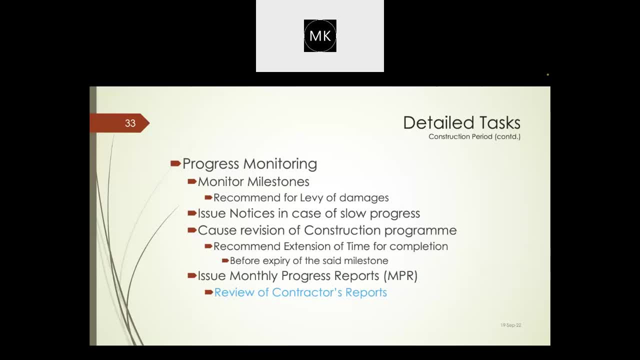 expiry first, at least one to two months before we have to process and see that it is approved before the set milestone. that is a healthy way of handling extension of times. monthly progress reports have to be issued, uh, but contractor, he will be submitting because he is mandated to submit. 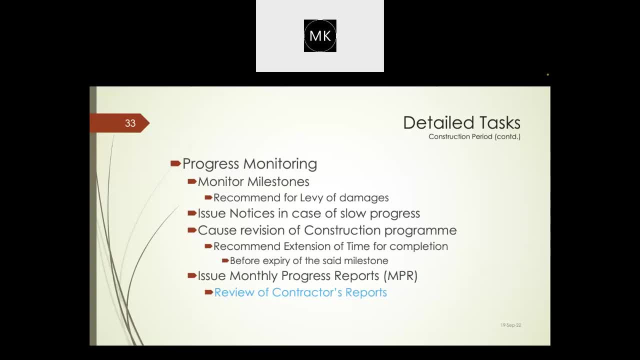 contractor, mprs. if we don't read, if we don't review, you know what will happen. he will be stating wrong status of hindrances. he will be stating, uh, giving a different account of his equipment and manpower and we don't see it, we don't verify it, and at the end of the project, if he has to claim, then he will. 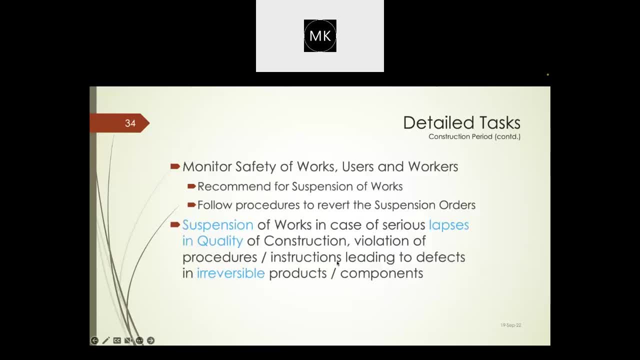 use these reports as support, if we don't deny them, if we don't review them. and deny them, we stand we, we lose, we stand to lose. so that is very, very important. we have to review the mprs submitted by the contractor and concessionaire now monitoring the safety of works. username workers. 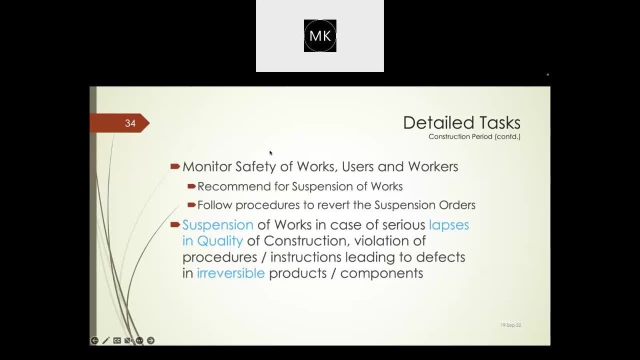 here: suspension. this is a very, very important thing that i wanted to tell you. suspension of work is generally when the safety of works is threatened. so if at all there is a quality lapse, we are not able to suspend the works. we should be able to suspend the works even when there is a quality lapse. 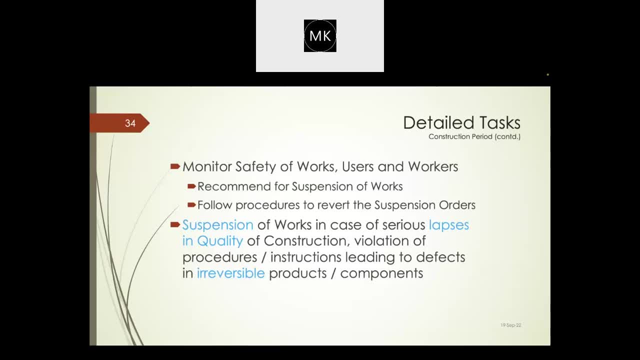 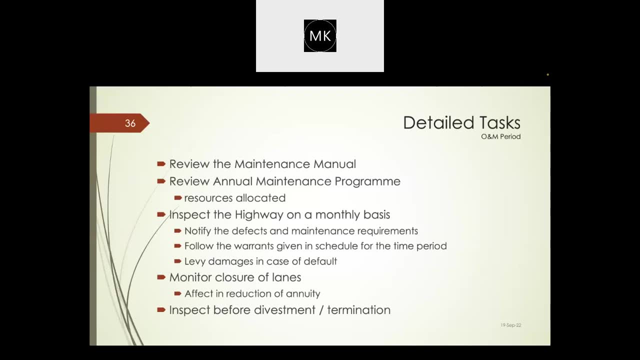 and that too when there is a problem in irreversible products. so when we suspend the project, then, no, we can control them properly. now it is o and m period, because we are dealing with the responsibility of the ie and ae, so i just wanted to cover all the periods. so we 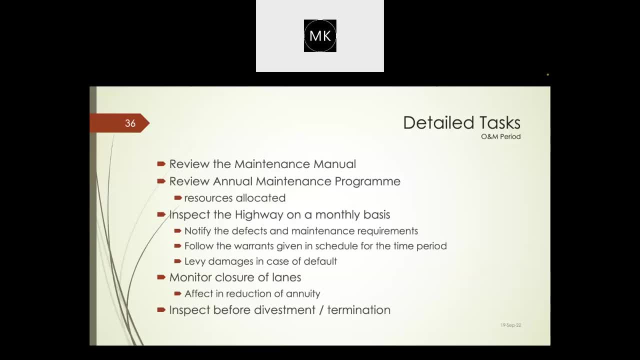 have seen the development period, then we have seen the construction period. now we are coming to the o and m period, that is, after the construction, after cod is issued or after provision completion certificate is issued. now the first thing that we have to see is maintenance man, what is the maintenance manual in the sense? what kind of defect, what kind of 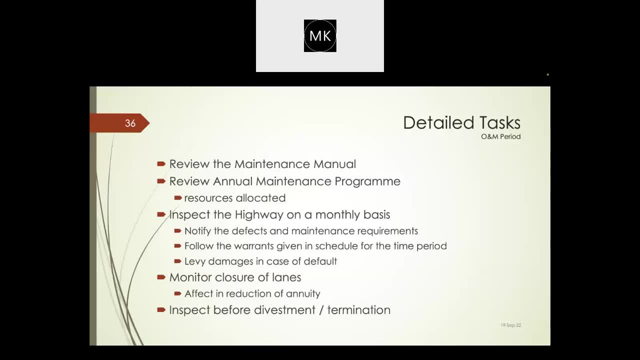 mitigation measure he is going to propose and what is the kind of timeline he is committing to us? there is a schedule, the schedule of maintenance, schedule for maintenance. whether he is doing it like that or not, every pothole has to be closed within 24 hours. 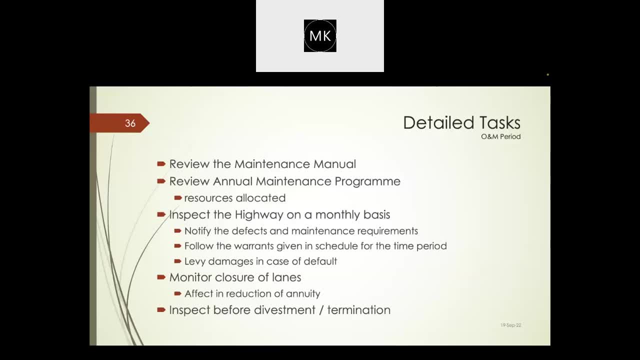 but if it is important and of safety consideration, then it has to be immediately done. so, like that, there will be many clauses in the agreement. those have to be properly incorporated in the maintenance manual. so what is the defect, what is the mitigation measure and what is the? 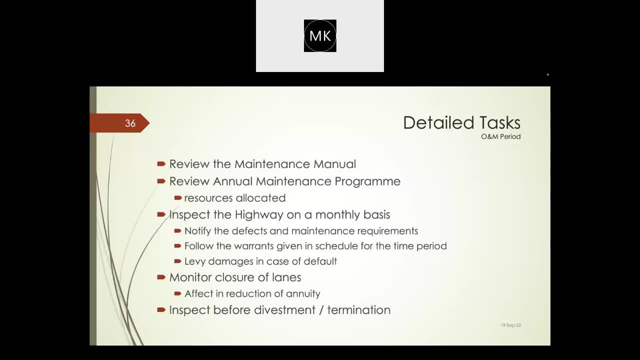 timeline and then how it will be verified and all that. i think there is a app now. i forgot the name of the app when i attended the month and program in bangalore. they have released that app where even the public probably is able to take a snap of that and then post it and when it is rectified, the 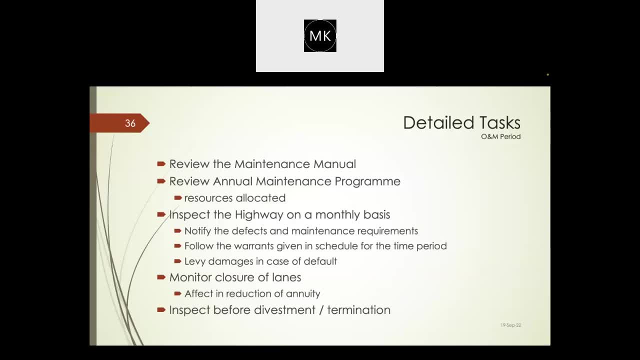 contractor is supposed to host the same thing. post the photograph of that against that. so this we have been doing the isolated level, project level, but now this has become a national level monitoring system. after that we have to- this is the first thing- whether he has a maintenance manual and 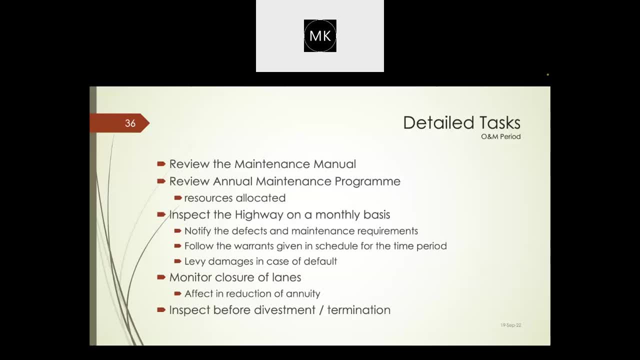 whether it is as for the requirements of the agreement. second thing is annual maintenance program. now what i am trying to say here. see, you might be thinking why he is spending time this line on the road. you sometimes see that it is a good maintenance. sometimes it is bad maintenance. 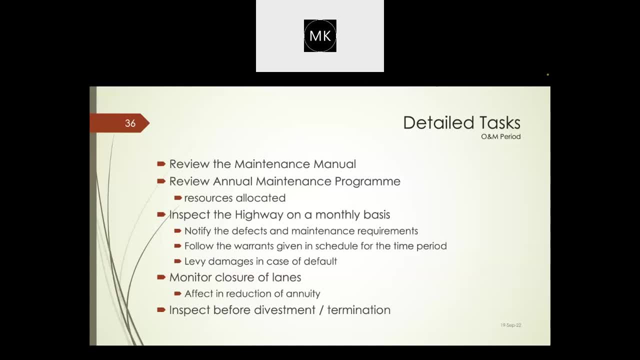 sometimes you see people on the road and sometimes you do not see anybody on the road, right? so now what is he committing? suppose if there is a pothole, then he will attend, if there is rutting he will attend, if there is a crack he will attend. but what about the median plantation? 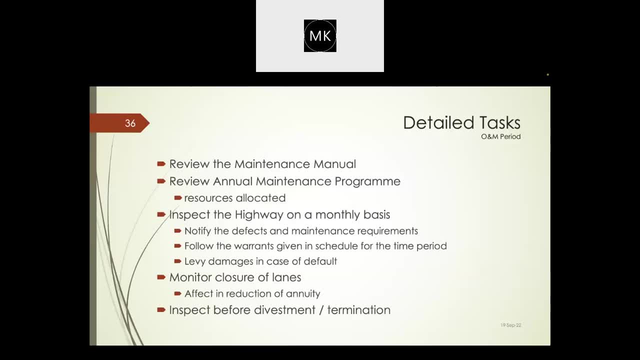 maintenance of the median plantation and any problem with the shoulders slopes, cutting of the wild growth in the slopes and removal of the garbage in drains, or removal of the openings of the clearing, the openings of the culverts and all so there should be a regular way of doing this. so 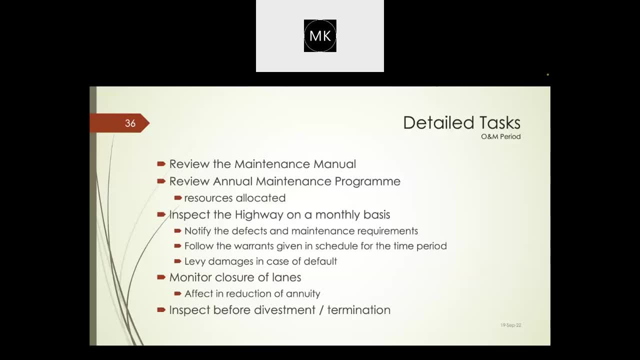 he should have a plan. he should say that in six months, i will be visiting the entire road once, so so i have 20 people on this, 20 people on this. they are actually. they are spread over like this, so he should have some resource allocation and we should be able to see them. 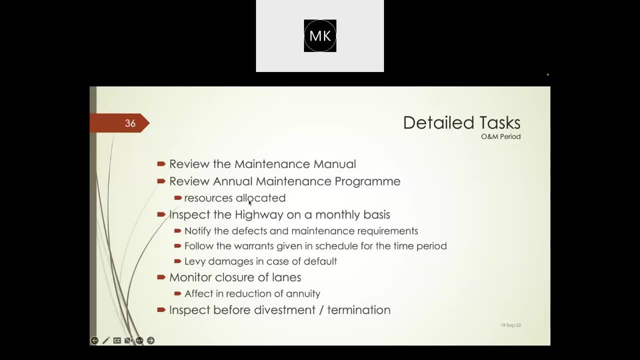 every day: cutting of the median plantation, trimming of the median plantation, like that. so it is very, very important to see what he has and what are the resources. so whenever we go to the site, we should be able to see those resources. they cannot be only on the paper. right then we? 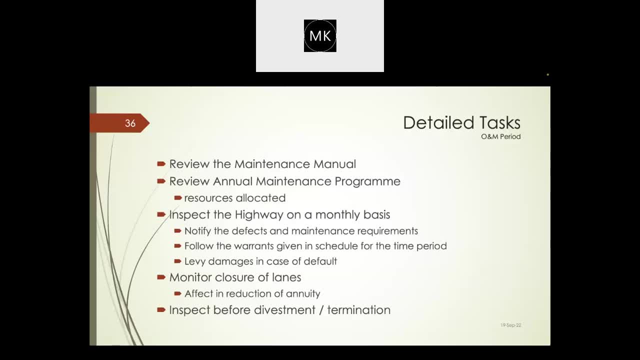 have to visit on a monthly basis and identify defects and deficiencies, and it should be as for the warrants given in the schedule. so far as the time period concerned, if there is a functional requirement, it can be done in six months. whatever reason, then we have to leave damages in case of 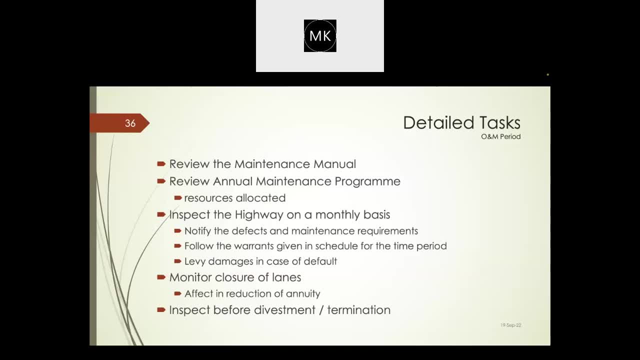 default, so we should not be light on them. these damages have to be levied on a monthly basis. at the end of the month we have to visit the site and then we have to tell him these are the damages, then closure of lanes: if there is a closure, there is a reduction. 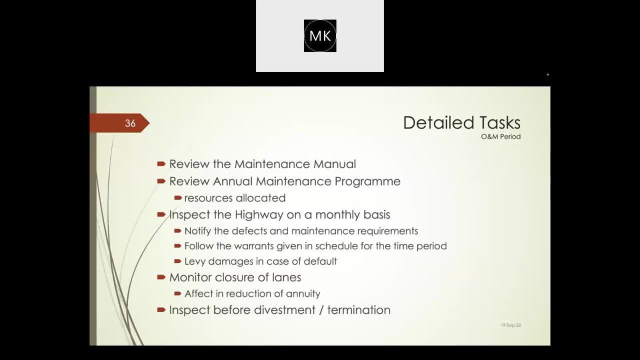 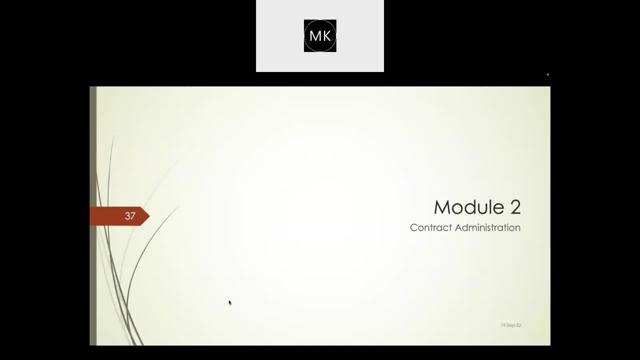 in annuity or something. so wherever this is applicable, we have to see that these are monitored. and then inspection before divestment or termination is also a task. now comes the module 2.. it is 10, 52 and 11- 15. we have the break, so 7 plus 15. around 20 minutes will be there, so we will. 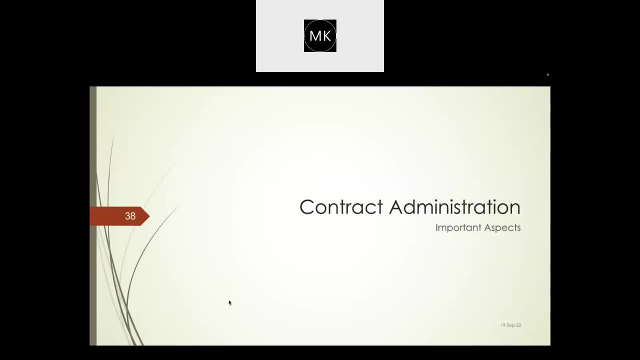 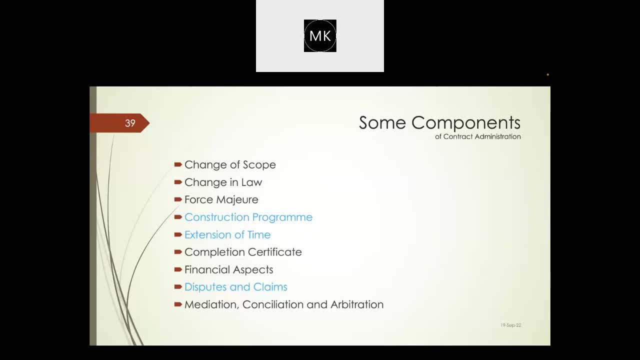 see, most of you know what they are, but most of you face problems also in dealing with them. so in what areas you face problems, we have to see, and i am trying to save some time for the questions and answers in the last 10, 15 minutes, so don't disappoint me by being silent at the end. 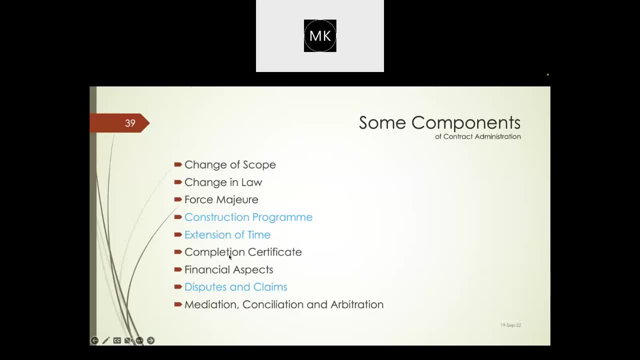 i'm trying to chase time, so now: change of score, change in law force measure, construction program, extension of time. we will try to spend a lot of time on these aspects: competition, certificate, financial aspects. don't think that it is only auditors who are supposed to do. we have to see the financial. 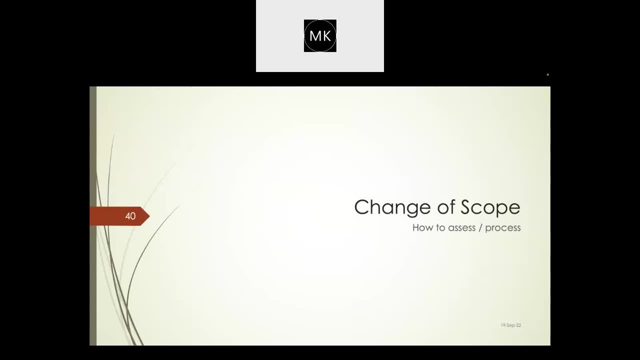 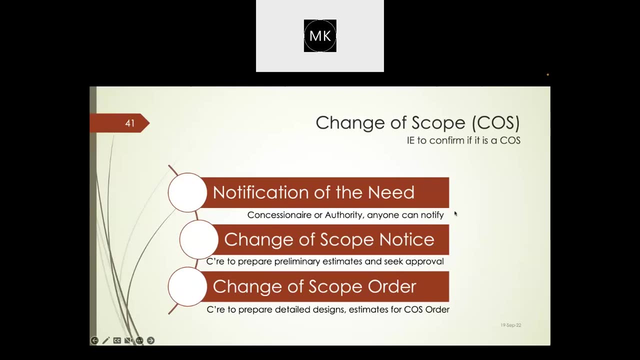 aspect: disputes and claims. we will see three types of claims and three reasons, basically, and how to avoid them. then now change of scope. we will deal change of scope and change in law. before now, change of scope: first of all, ie has to confirm or ae has to confirm if it is a cos. 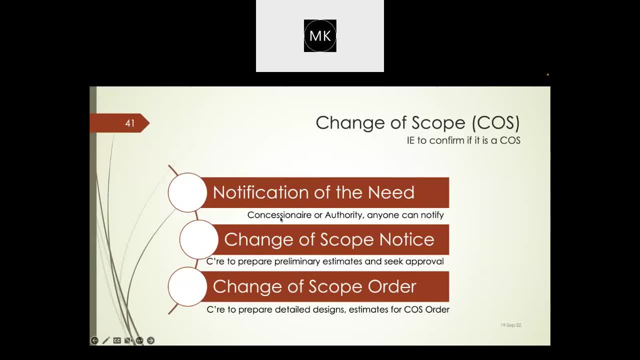 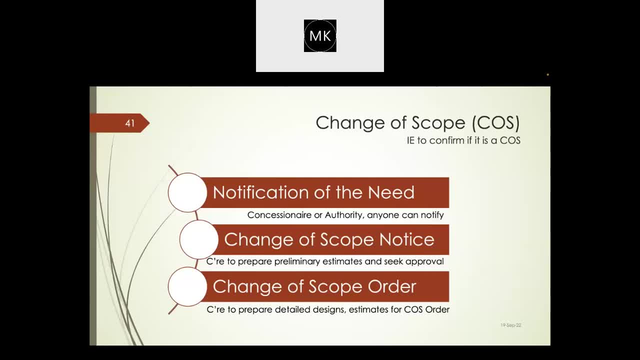 Yes, so notification can be done by anybody. then change of scope notice has to be given, see in NHGI, in Ministry, in various places. this word is forgotten, this word, in fact, they don't care about it in the sense in principal approval, some sort of those works are confused, but 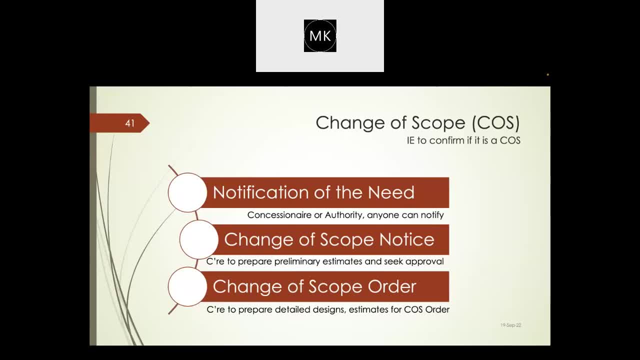 we should use the proper words. so finally, the change of scope notice has to be given. then who has to give? also important: authority is supposed to give, but what authority does? it says so, you can give, you can give. i think it should not be the case now, when notification is notified, i mean when the 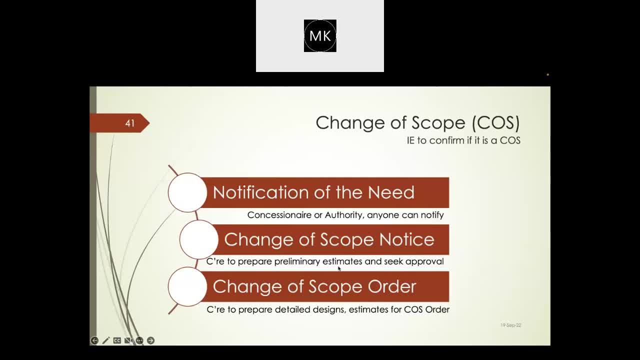 need is notified. change of scope notice is supposed to be given by preparing preliminary estimates and then we seek approval. without estimates there cannot be a change of scope notice. that is important, but at the time of change of scope notice, drawings may not be there. detailed designs may not be there. 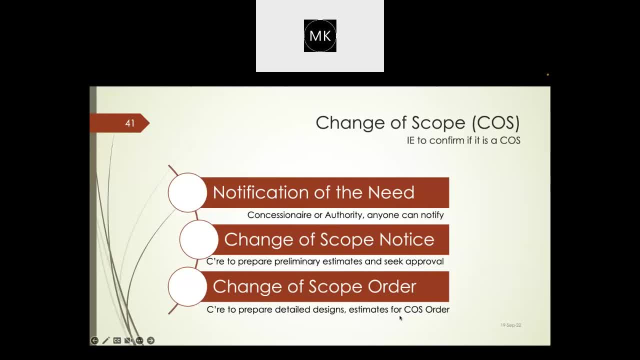 but still we have to do some preliminary estimates and then seek approval of the authority. then, once change of scope notice is issued, then we have to prepare detailed designs, drawings and then prepare estimates and then we should issue the say we should submit for approval of the cos. 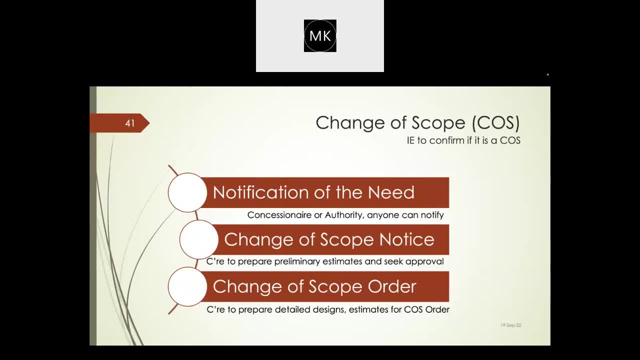 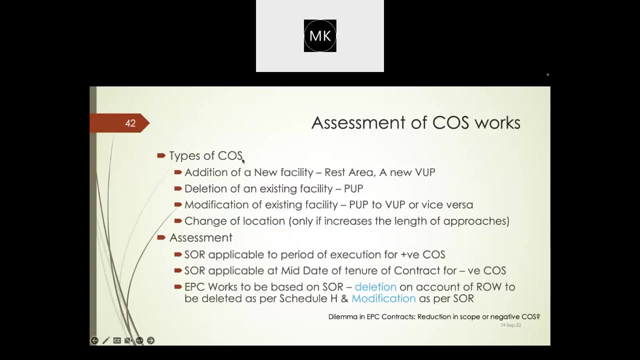 order now. if there is a difference between preliminary estimate and detailed estimate, then you are going to have problem. so it is good it. we should always see that more or less things are done in detail at change of scope notice so that there is minimum change. so this is how it is going to be now. what is a cos? what are different? 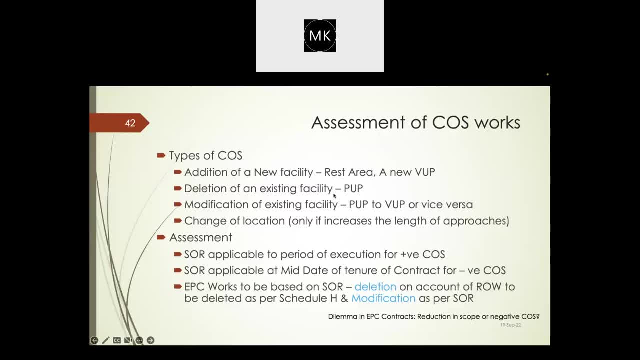 types of cos. one is addition of a new facility. when there is a new facility, it's a change of cos which is not there in either schedule b or schedule c. then deletion of an existing facility. suppose the pup is there and we don't want the pup there. we only want a plain rule that is also a cos, negative cos, modification of an. 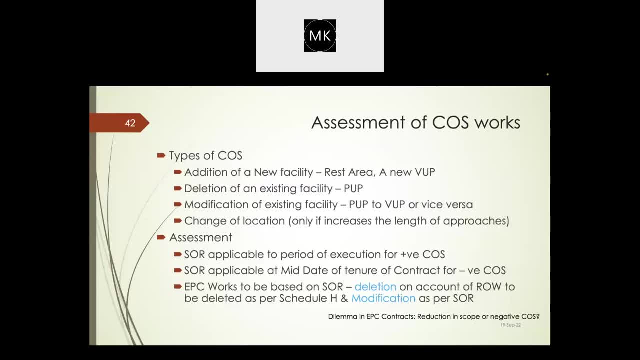 existing facility pup is upgraded to a vup or a vup is reduced to pup or whatever change of location. now this is a very popular thing. so even if there is a change of location, people are trying to issue change of scope notice. the whole problem is how they are doing it. so if there are, there is a negative change of scope, say. 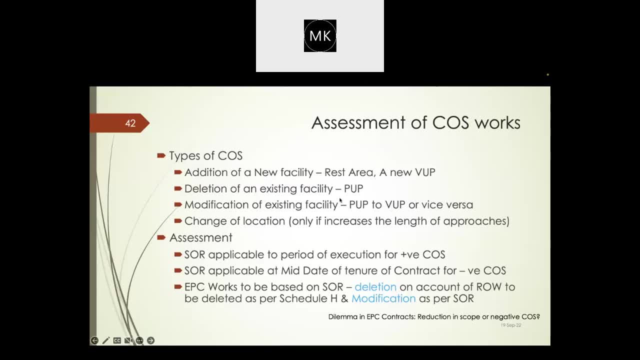 this one: pup to vup or vup to pup. what they are doing is negative change of scope will be done by using schedule h and the positive cos will be done using current s4, and they are creating problems and creating disputes. so there should be clarity. so, in change of location, 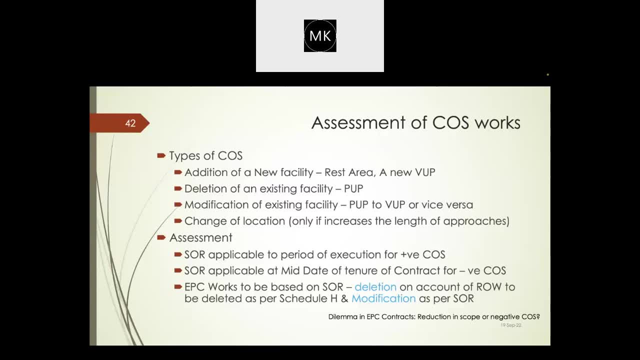 only if it increases the length of approaches or area of re wall, and that too grossly, there may be a chance of giving a cos for change of location. otherwise till now i have not given anything. only now somebody during conciliation, they are asking where you check this. i told it is too much. 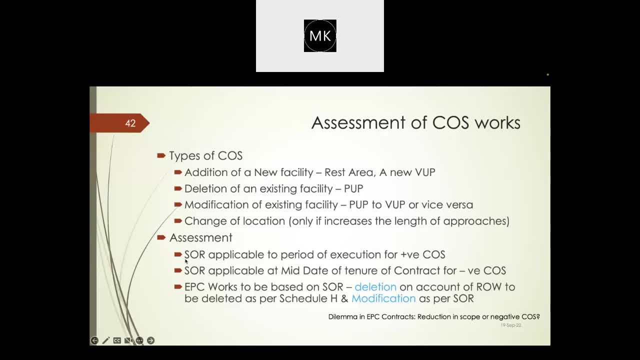 sir, change of location in a plain terrain, whether it is here or whether there anywhere it should not be possible because of the change of scope, will be pushed fly, caused by the change of location. equally, i will go further. i think you were considering prototypes. perfect, that's something. 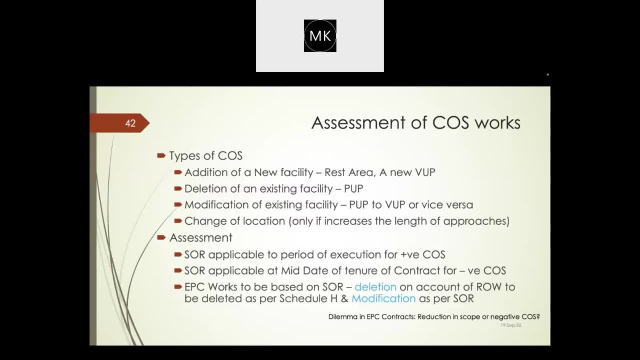 that we need to not justsstił. take a look, it is very important. that is when we were Prim Scotate. where is it able to be reflective of? of course it should be. LCD went to know that, but something may have taken shape. we should it so 완성 toward what you just saw now. assessment now: 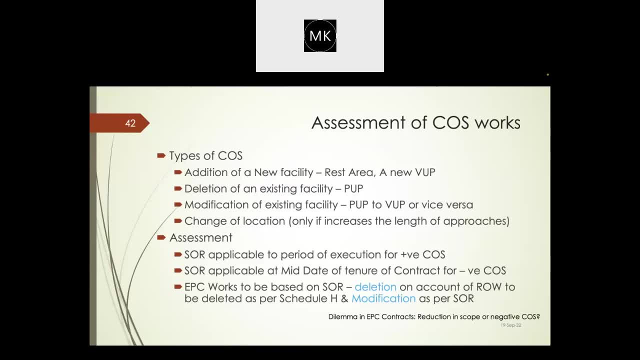 assessment. now this is where we have actually considered and that SOR should be applied on the positive COS, But that SOR is not in place today. Whatever is in place today is a past SOR, So, in fact, it is good that there should be a. 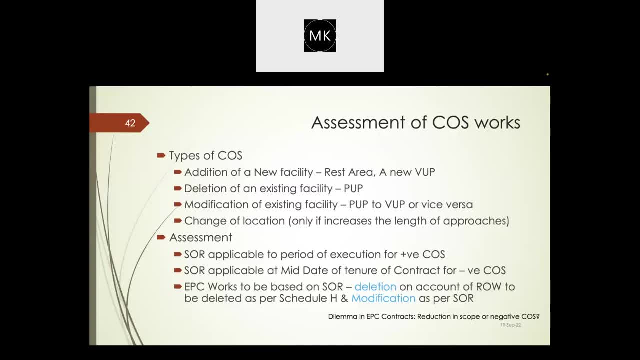 price multiple for this and there should be a correction for a positive COS depending upon the midpoint and the SOR applicable at the midpoint- midpoint of the execution, period of execution, But otherwise current SOR is in practice We just apply current SOR, SOR applicable at mid-date. 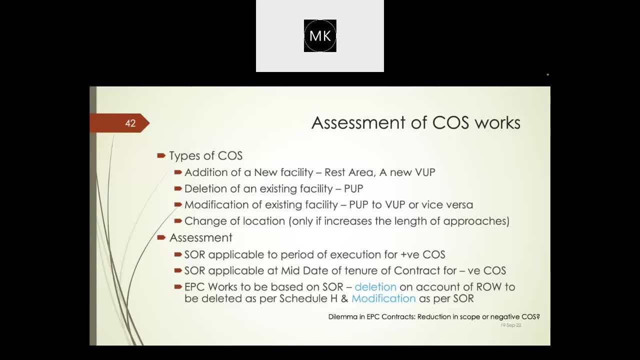 of tenure of contract for negative COS. Suppose there is a three-year contract, Scheduled date is, say, 2020 and the completion date is 2023. So we get to 2021 and whatever SOR is applicable in 2021. 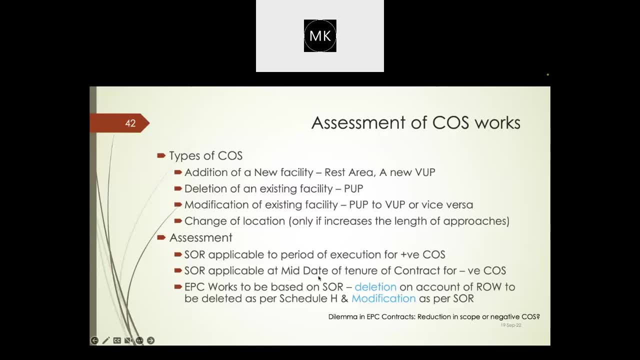 apply it to all the negative COS items, because they are applicable to all the negative COS items. So that is the way he might have structured the contract So we can do this. So I have applied this in many projects and they have. there was a dispute but ultimately they have accepted that. 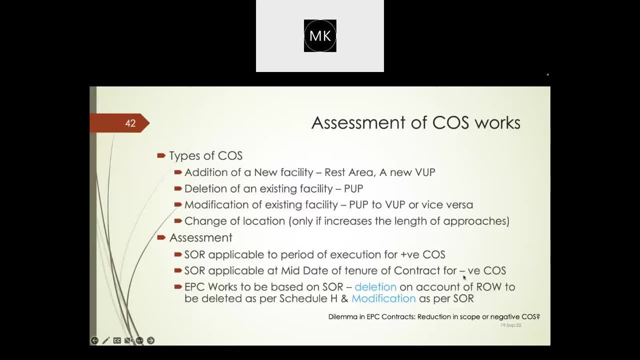 that would be that way. But otherwise they are telling, in NHIA at least, that both for positive SOR, positive COS and negative COS it should be current. Then EPC works to be based on the current SOR. So that is the way he might have structured the. 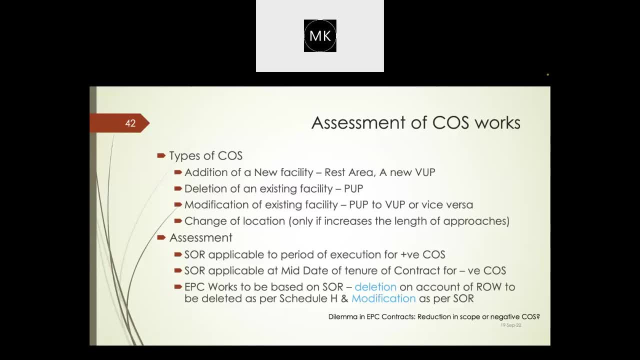 contract based on SOR and deletion on account of ROW to be deleted as per Schedule H, in the sense, if we are not able to give right-of-way to him and because of that we have to delete something, At that point of time we have to use the percentages given in Schedule H for deletion. 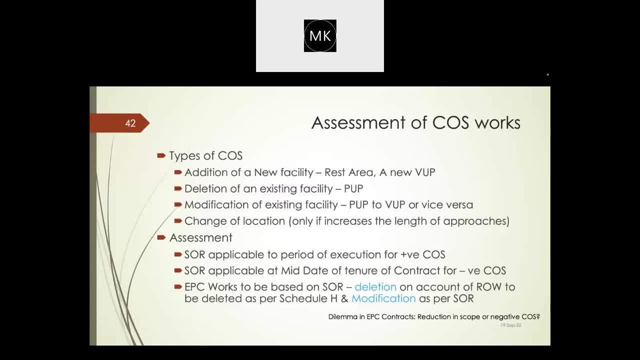 That is the idea for this Schedule H. But if there is a problem we have to use the percentages given in Schedule H for deletion. But if there is a modification as per, that should be done as per. SOR. Suppose a PUP is. 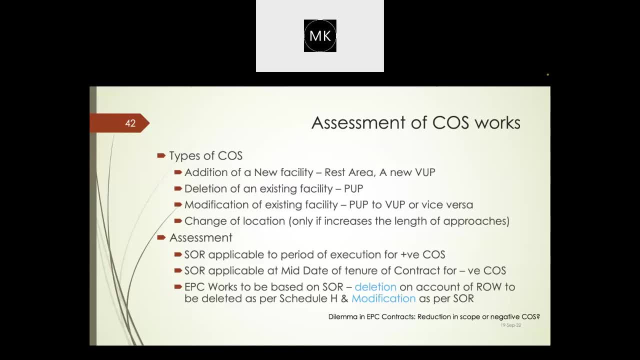 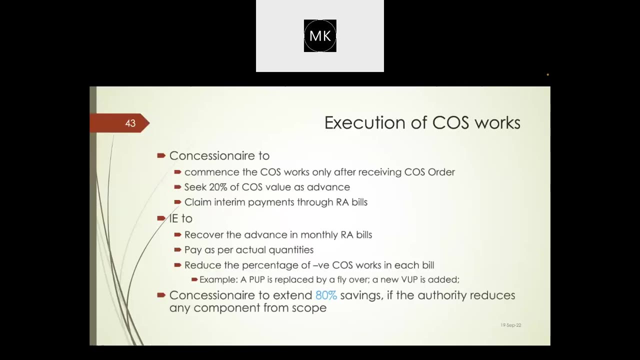 converted into VUP. So we estimate the PUP as per SOR, we estimate as per VUP as per SOR and we find the difference and that will be the change of score. So this is the main dilemma in COS works. Now how to. 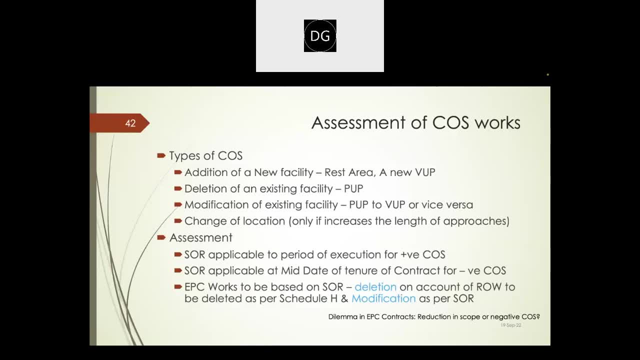 Sir, I have a doubt, sir. Yeah, please, Sir. VUP is converted into PUP, then this has to be calculated based on SOR. You are right. I am also telling the same thing: modification as per SOR. 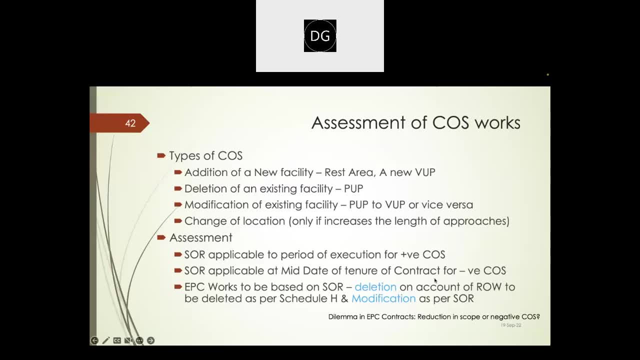 Sir, in any case, if any PUP is removed and in place of PUP ROW is constructed, this is a modification or deletion, sir, It's a deletion, But in any case we do it as modification. But if it's a simple deletion, we can go as. 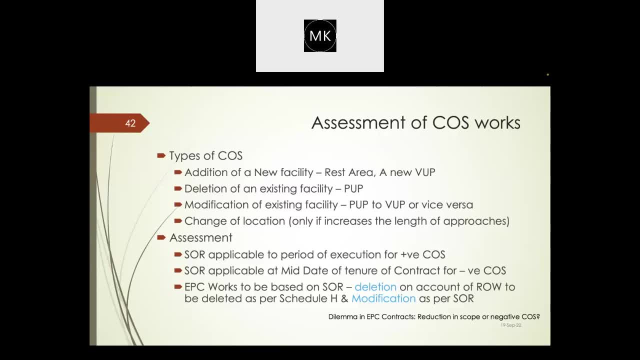 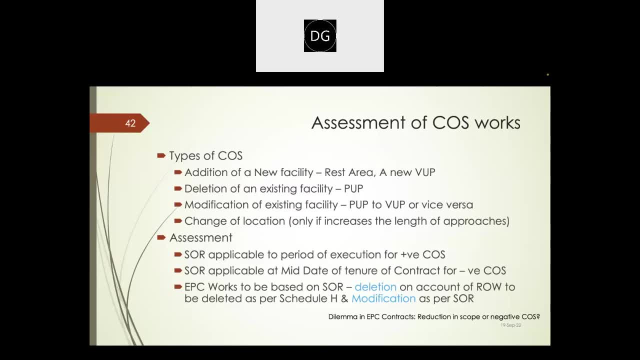 Yes, Yes, Yes, Yes, Yes, Yes, Yes. Anyway, bridge cannot be removed simply because bridge has a stream bridge has, unless the DPR is done badly. See, generally, what we do is if there is a simple deletion and 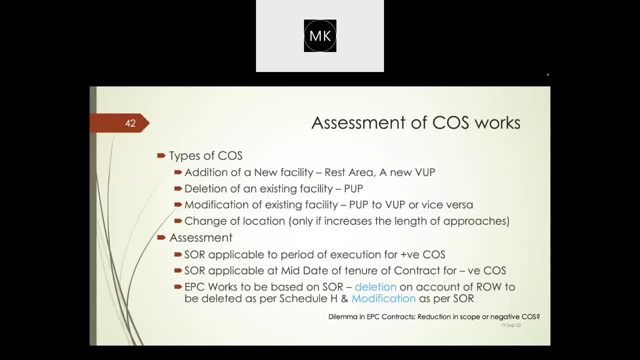 if it is due to ROW, it is good. then we do it as per schedule h. so in your case, a bridge is being deleted because of because of a problem with the authority or because of a problem with the site, then it should be deleted as per schedule h, only in case of modification. modification, as i told you. 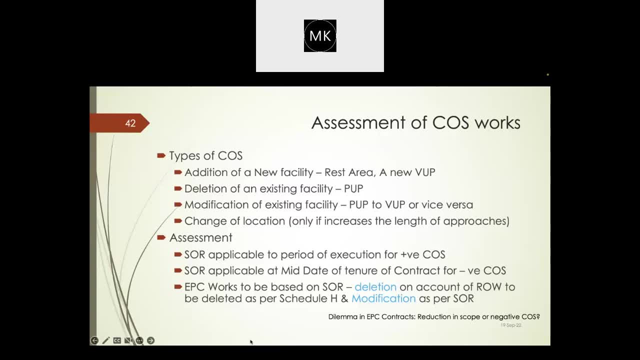 pup to eup, vup to pup are, with this being, it is being widened, it is being the height is being increased, or whatever. in case of modification, only we go go as per so on. let this be, uh, like this clear deletion on account of authority schedule h. there is a modification. it will be. 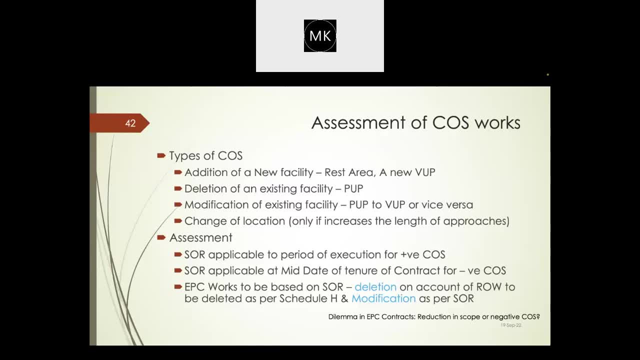 sor pup to where pup is there, that pup is removed and road is there. now you try to understand this. road was there when pup is there, also, over the approaches. road was there you? so it's actually like that. it's not a modification as such, so there, we simply use. 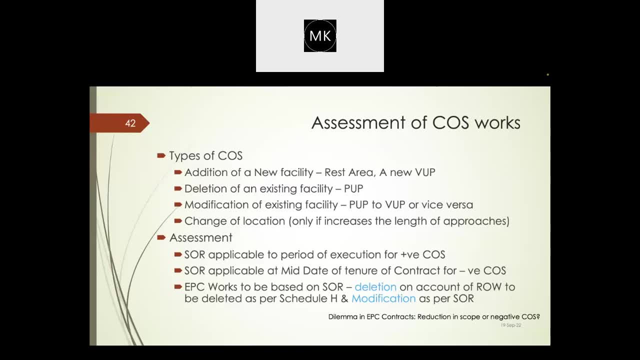 but on top of pup we are only giving somewhat bituminous layer and in place of road we are constructing, we are giving earthwork, gsb, wmm, dvm, bc contactor. saying is that this is a modification. it's only a small width pup seven meters, so if it is a vup 12 meters. but whereas the approach is 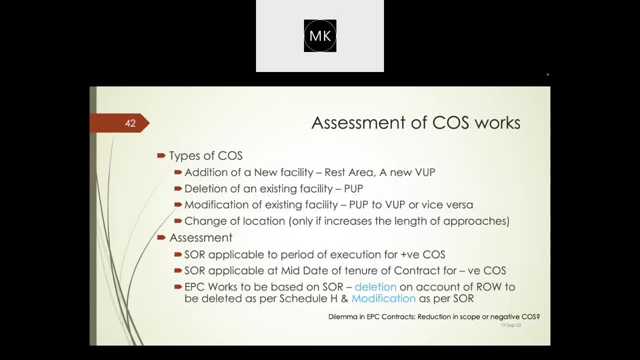 200 meters, 300 meters, where the road work is same, more or less. so, anyway, this is, uh, this is how i am following everywhere, and it is going on like that, so we can go go to specific issues. uh, if at all you have some, can we say like that, if any scope is, 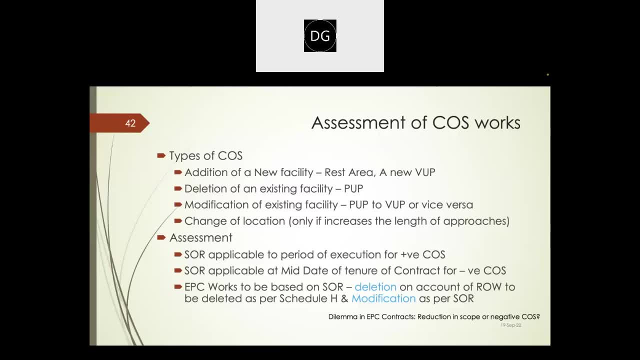 deleted due to only of row, then we will go for schedulers and any other reason. we will go from sor no more. other other reason means what is saying that these culverts are not required at this location because there is no water flow Right? So that is not the problem of the contractor. 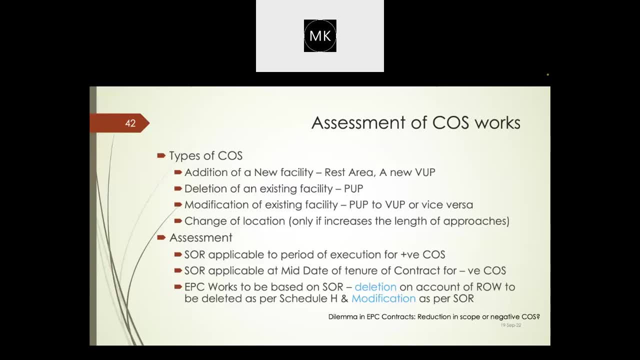 That is the problem of the authority. So whenever there is a problem of the authority and there is a Schedule H, it should be done as per Schedule H, Sir, but at site we are deleting. actually on site there are 10 culverts of 2x2 and 10. 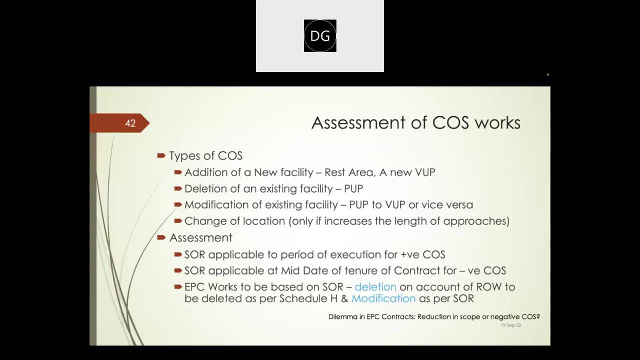 culverts of 3x3. On Schedule H all the culverts are having same rate, but we are deleting culverts of 3x3. Then the bigger size of culverts are deleting and the smaller size culverts has been constructed. 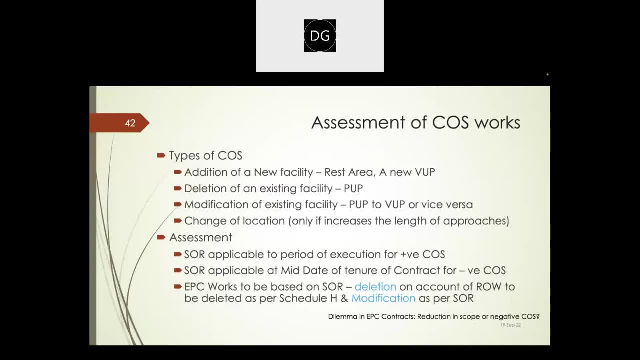 Then how can we take the same rates for all the culverts? See, when bigger culverts are being deleted and smaller culverts are being constructed? it is a modification. Okay, sir. Okay, So let us try to understand it that way. 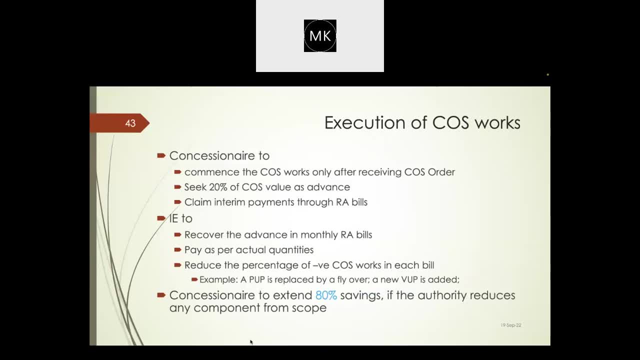 We can go to specifics. Okay, If your project has something, we can interact, and then we will do that. Okay, sir, Yeah, Thank you, Thank you, sir. Thank you for that question Then. execution of COS work. It is 11.05 and we have 10 more minutes. 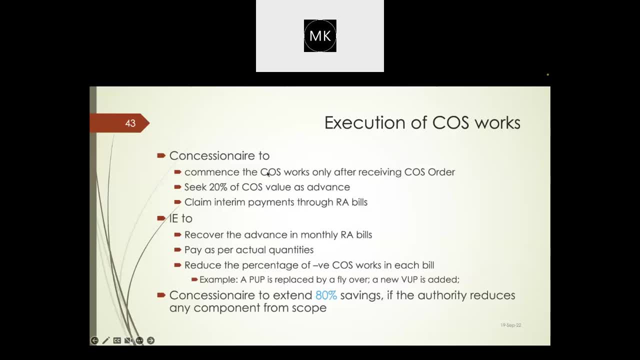 First of all, when COS should be commenced only after receiving COS order, we have problems. He starts, he commences work before and then afterwards authority does the work, Authority does not give COS order and he goes into disputes. Then 20% advance is given. that you know. 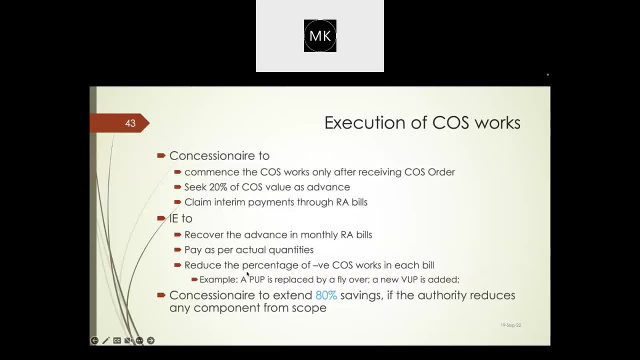 Then interim payments are claimed through RA bills and IE has to recover advance in monthly RA bills and they have to pay as per actual quantities. But the most important thing is reduce the percentage of negative COS works in each bill. Suppose a PUP is replaced by a VUP and the result is, you know, reverse. 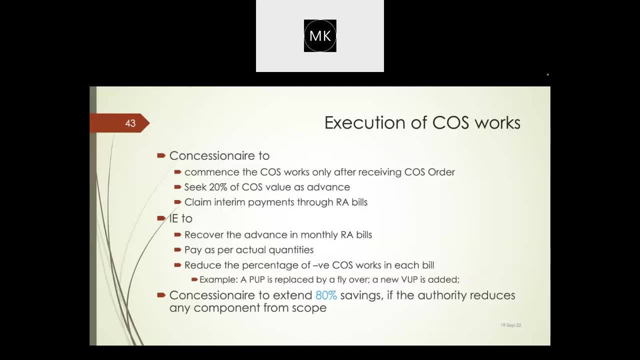 A VUP is there is a negative component and there is a positive component in the same location and that negative component is, say, 20%. So each bill we have to see that that 20% is directed so that we are consistent with the COS order given. 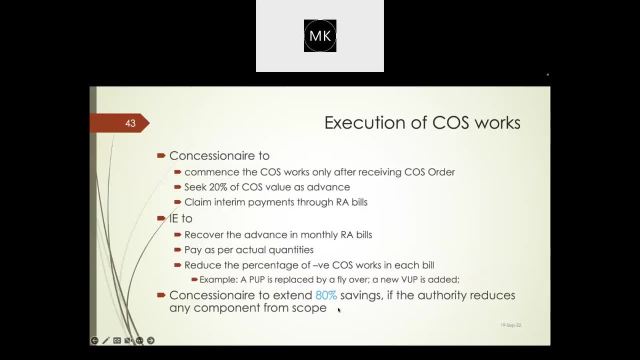 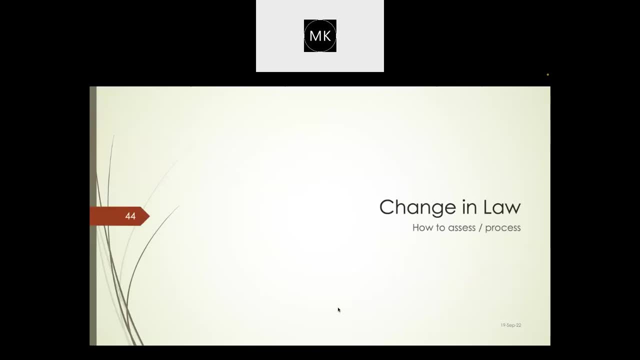 And there is savings if we are deleting. if the authority reduces any component from scopes, the concessionaire need not give 100% savings. He can give lesser savings, as per the agreement. It may be 80%, it may be 90%, as per the agreement. 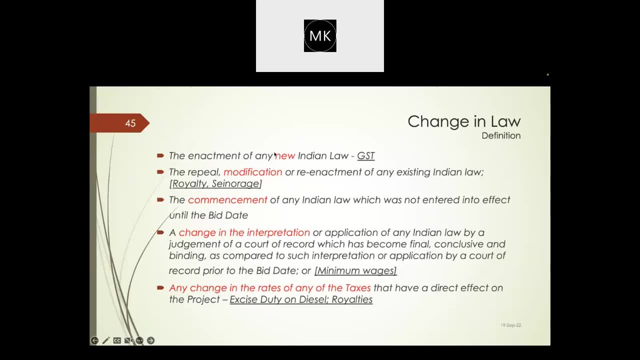 Then the last item before T is change in law. Now, what is change in law? These are various situations. One is a new enactment of a new Indian law, So GST, that is a new modification, Royalty or scenery, These, When there is a modification of rate and other things, it becomes even some somewhere. 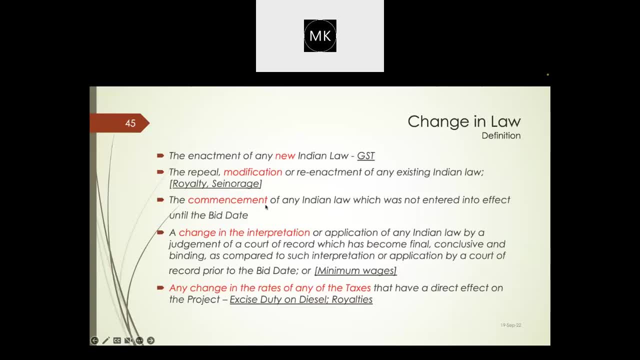 in the methods have been changed, So much percentage over royalty will be paid as scenery, something like that. So there's a modification. Then commencement of any Indian law. This is the way it is written in the contract, But this is as good as the new Indian law in my view. 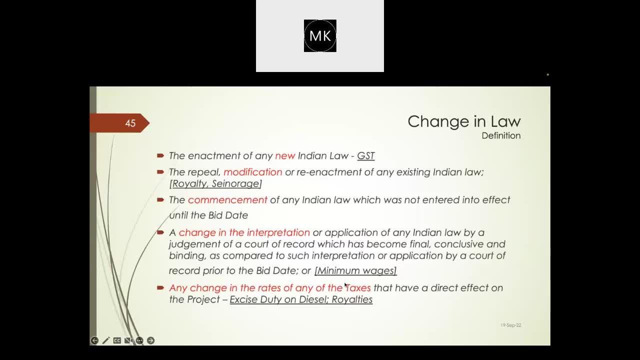 Change in the interpretation, If at all. a court has given a judgment on a specific thing, If that also can be taken. Now, minimum wages: I'm facing one specific case in one project where they told: Sir, minimum wages have abnormally increased in my project of, say, three years or four years. 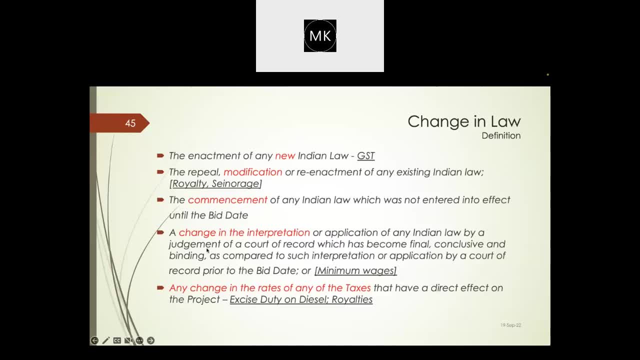 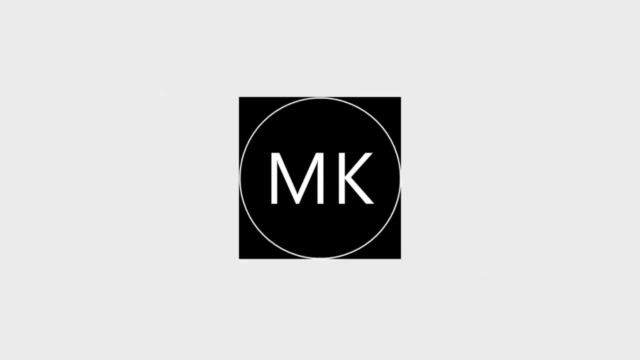 And you have to give me change in law And I'm in actually a dilemma. But he brought some interpretations, He bought some judgments. Even if judgment is there, It should be expressed and explicitly given that minimum wage. That's the question. 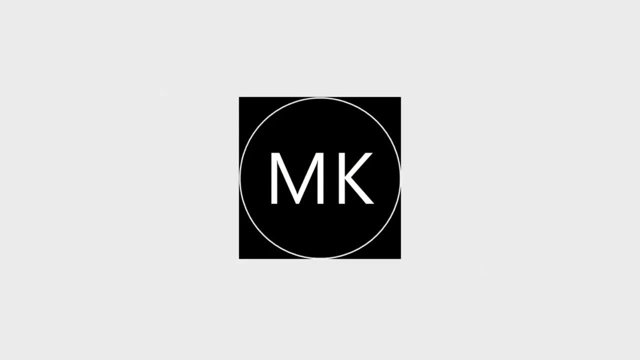 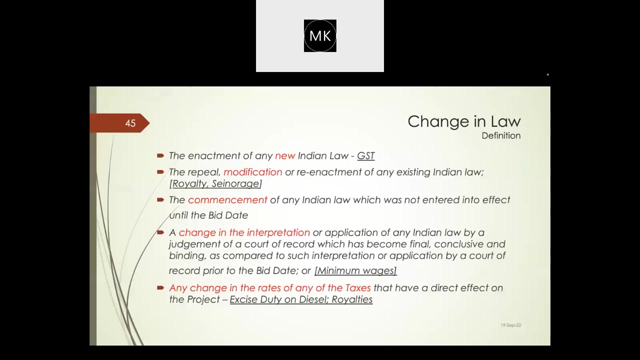 So that's pretty much it with it. Thank you, I appreciate it And thank you. Thanks, Tim. Have a good day. Have a good day. Thank you, they won't Thank you you. if it is increasing, it may decrease. So there is no correspondence between. 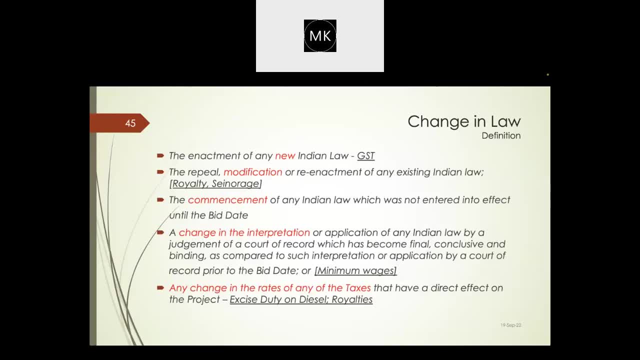 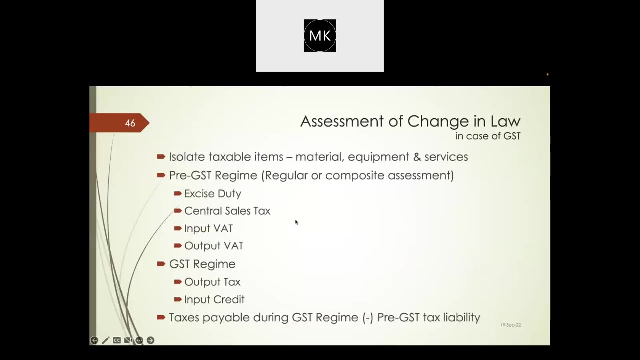 the actual retail rate in the site to change in the SI duty. So with that condition of course, I have denied it, but there is a problem like this. So this is how the change in law is considered. Now, royalties: changing in royalty also is a change in law and we have been giving 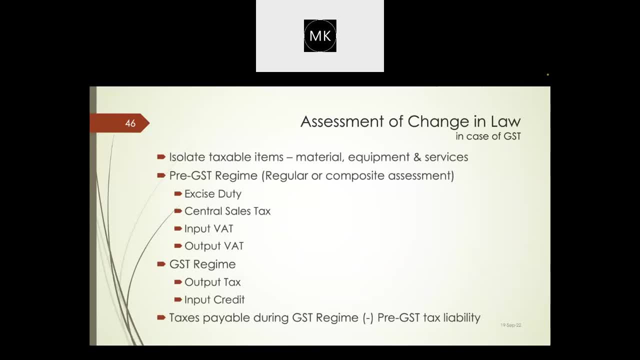 and GST. of course we have dealt it Now. I just want to have this one slide before the tea break. You may be seeing that GST is not my lookout. some auditor will see. but we need to understand the basics. We have to take the total contract and from that 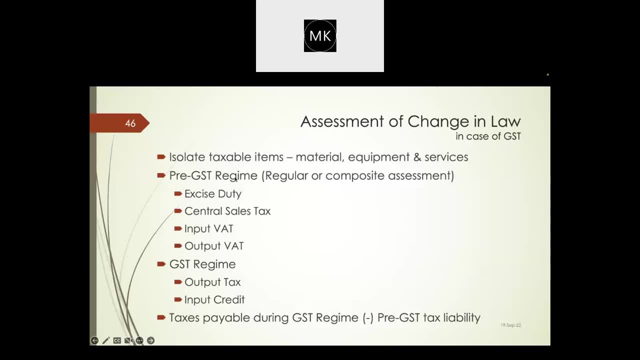 we have to isolate taxable items, particularly material equipment, services. whatever is there, we have to isolate them. Taxable items in the sense in pre-GST regime, some of these materials, equipments and all they were levied with these taxes. 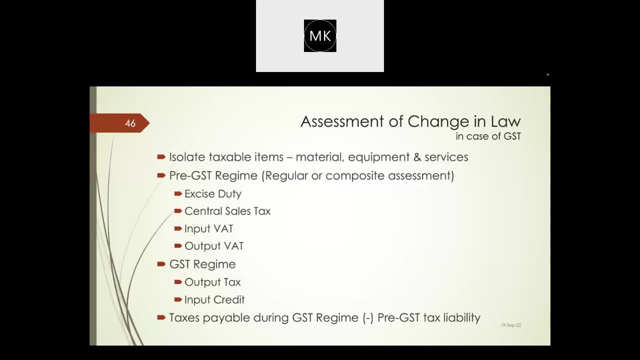 these taxes were levied: Excise duty, central sales tax. central sales tax is levied on the materials procured from other states. Suppose I am working in Andhra, Andhra and I am getting. I am working in Telangana, but I am getting steel from Andhra. 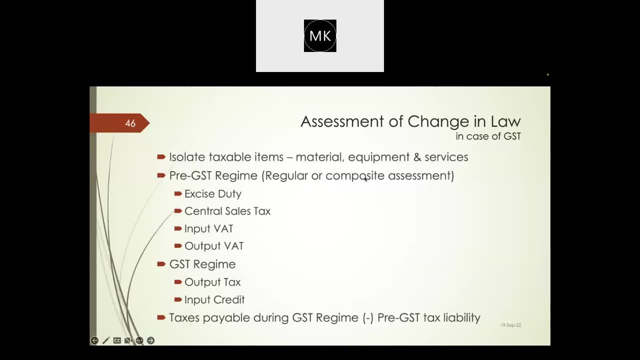 So I have to pay central sales tax. In the earlier regime, input VAT and output VAT- these things are also were there in previous regime. So there was a regular assessment and there was a composite assessment. What is meant by composite assessment? 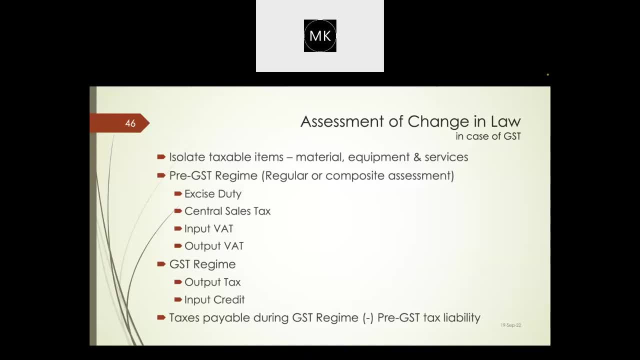 They don't want to go into all these things. Contractor doesn't want to go into all these things, So at that time he can pay 4% of the whole project as taxes. So that was a composite. It can be 1% whatever. 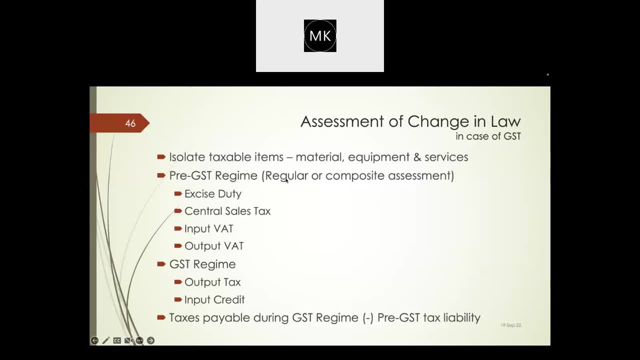 Regular means now: what are the materials used, What should be the tax of all these things? And then, what is the output tax? What is the difference Then? what I have to pay all that? So NHI has given different formats for these two, for regular and composite assessment. 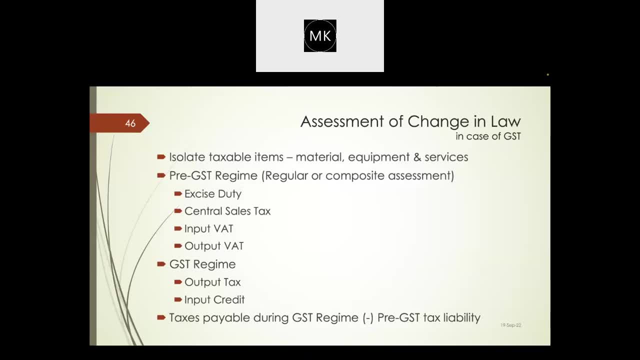 Now in GST regime, What is happening? Most of you might know what is happening in GST regime, but still I would tell you. If there is a EPC contract and it is say 1000 crores, straight away on 1000 crores he is. 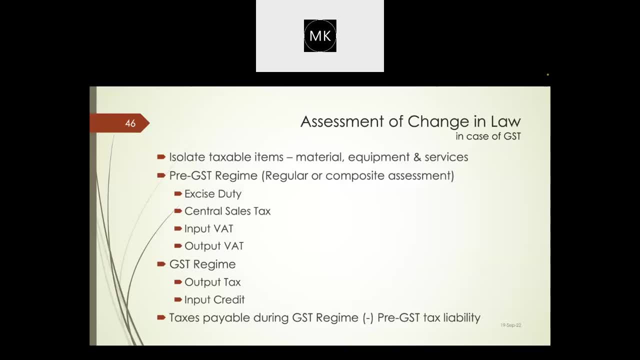 supposed to pay 12% as output GST on that in earlier regime. So earlier regime in the sense up to some date in 2022.. 12% way of paying: That means 120 crores. he has to straight away pay to the department 120 crores. 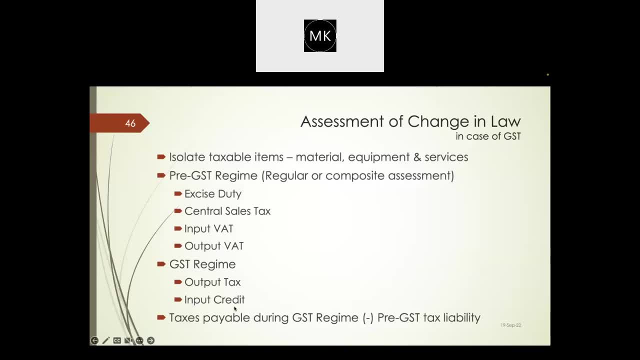 Now it has increased to 18%. So now he is supposed to pay 180 crores without talking. but that is called output tax. What is input credit? He is going to a steel factory, a steel outlet, and he is procuring steel. 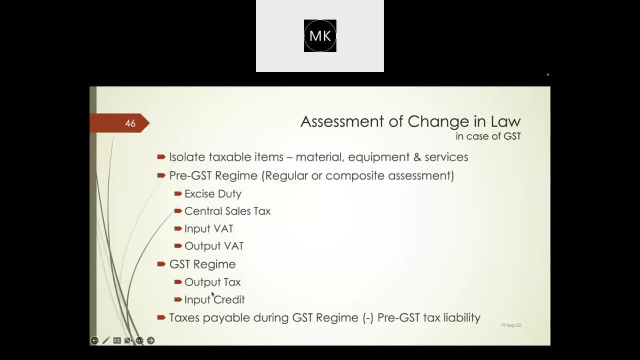 He's getting cement, He's getting various other materials- expansion joints, bearings and various other materials- And then he is paying GST to those people. whatever GST he is paying to them, He can actually claim it, as I don't have to pay 120.. 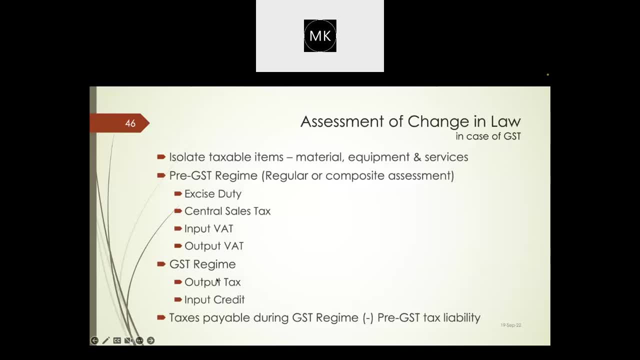 I don't have to pay 180.. I have already paid some 50 crores of tax GST to these people in securing these materials. That is input credit And he pays the balance. That is input credit And he pays the balance as output tax. 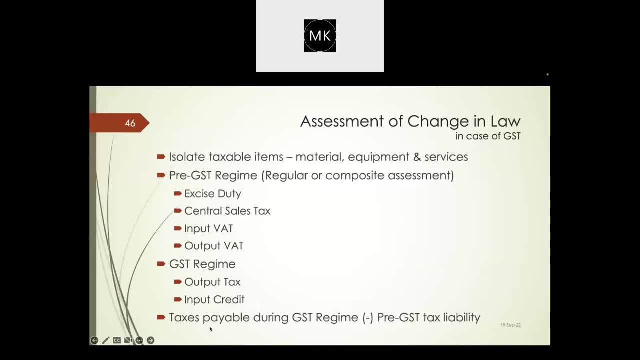 That is called paying in credit and paying in cash. So we assess all these things And then we say taxes payable during GST regime minus pre GST tax liability. This is the change in law. If anybody has specific questions, you can ask me after the break on this. 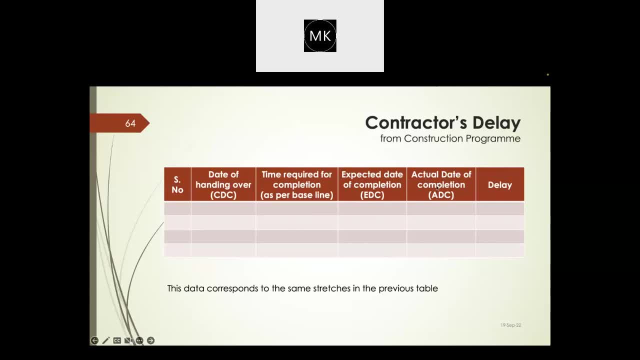 Thank you, Thank you, Thank you. You can have any time. Thank you, kilometer. there should there should be a program for such lengths then culverts in that should have a different one then for each structure. it may be a bridge or underpass or toll, plaza or any. 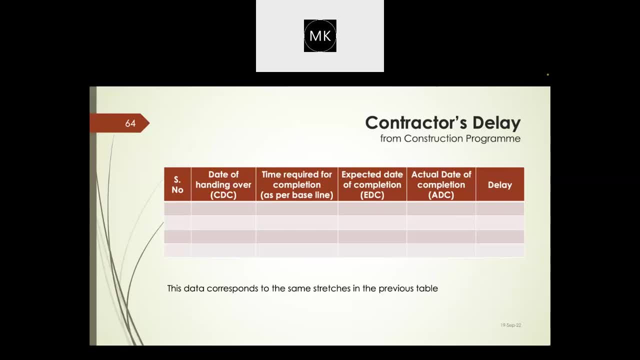 facilities for each of them there should be a separate program. suppose we are not able to give time land for toll plaza, then that particular bar itself we should be able to move. we are supposed to give here but we have given here, so it affected the program. like this. we should be able. 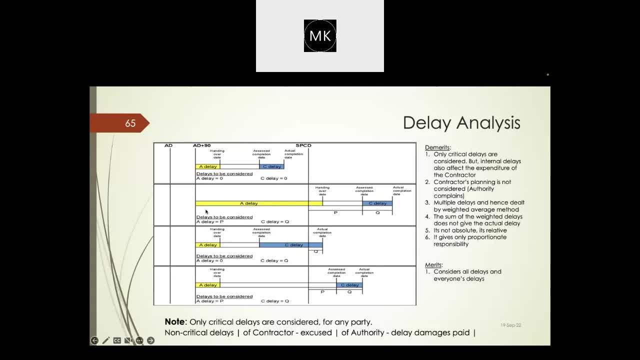 to assess for that each structure. there should be a different timeline then for the hindered works, when you are very clear on, say, 80 plus 180 or whatever particular day or time on that day, if such and such works are hindered and they are delinked for the purpose of completion. 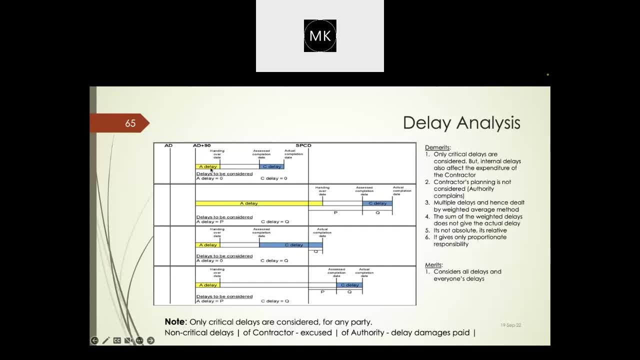 those things should be separately shown in the program, so then you will be able to monitor those works. third, that is called micro level. the third one is responsive. responsive in the sense it should be responsive in the sense all activity should be properly linked so that the effect of delay 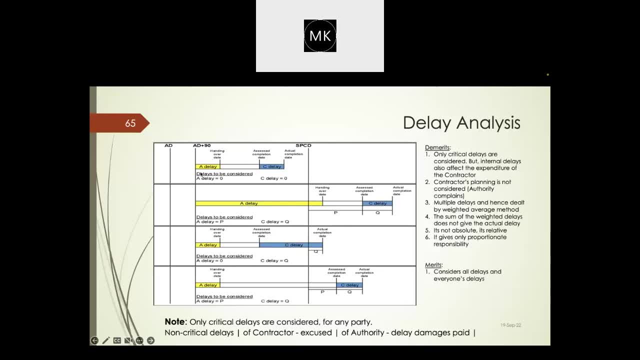 in any activity is instantly reflected in the date of completion. suppose one particular bar. you pick and you move that bar and see what is happening to the time of date of completion. there should be change in the date of completion. why, if there is no change? there are two reasons. one is there. 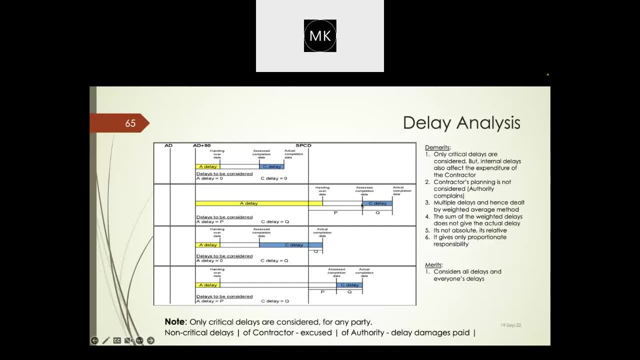 is a float in that activity or second, it is not linked to the main program. you can touch the program at various places and see whether it is responsive. then it will be resource based with the actual number of plants and equipment. if 100 kilometer is divided into three packages, four packages: 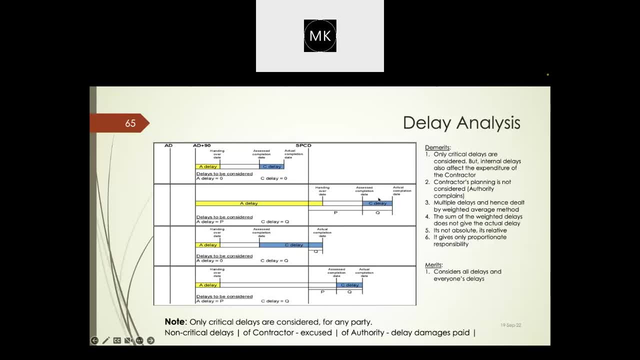 and separate plants and equipment are allocated for such packages, then accordingly their numbers and other things have to be incorporated in the program. that so it should be based on resources. it cannot be just ad hoc. then it can be tracked and kept live by updating the progress. this is where i am telling you that microsoft project is deficient, though. 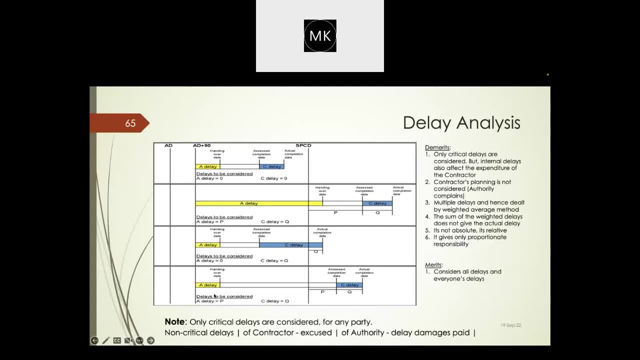 they say that they can update the progress on that, but it can be manipulated also. that is what i have seen. but whereas primavera, we'll be able to catch if something is happening, but so it can be tracked and kept live. if it cannot be tracked, so we will be able to even track it daily, at least weekly or 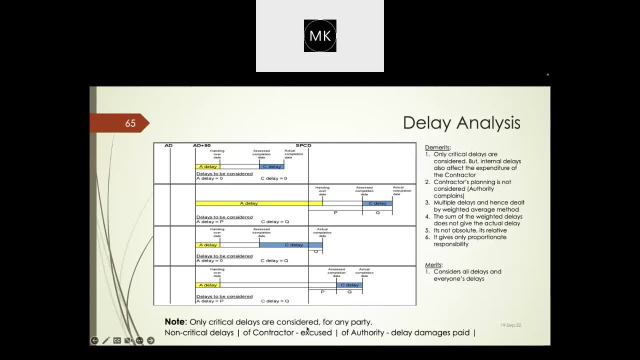 100 monthly to see whether the actual date of completion, whether it is changing from our target. then it should be linked to boqs raw materials, plant and equipment and cash flow. what is happening? they develop a excel sheet separately but when we change the program, this doesn't change. we should be. 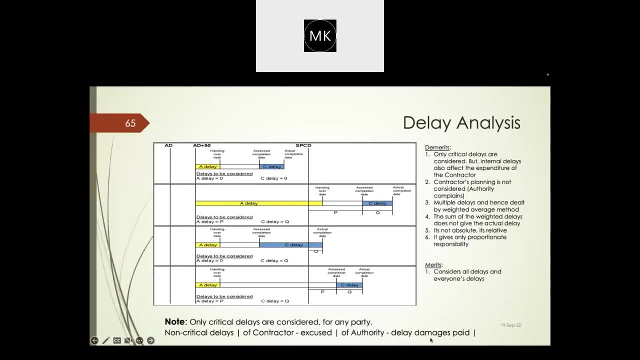 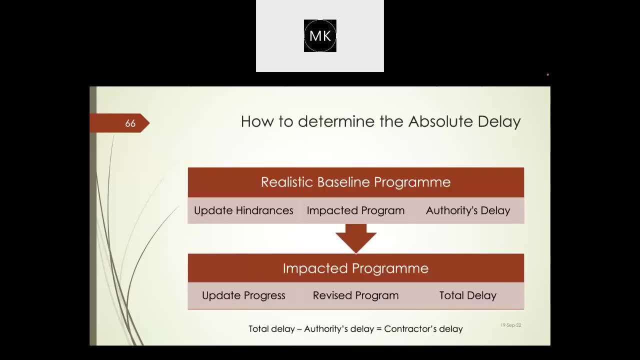 able to know what is happening to the percentage progress. you know, the most important thing, we should be able to see what is happening to the milestones. that is the reason why we want the percentage progress: 10, 35, 70. so when we change the event, then what will happen to the percentage progress? 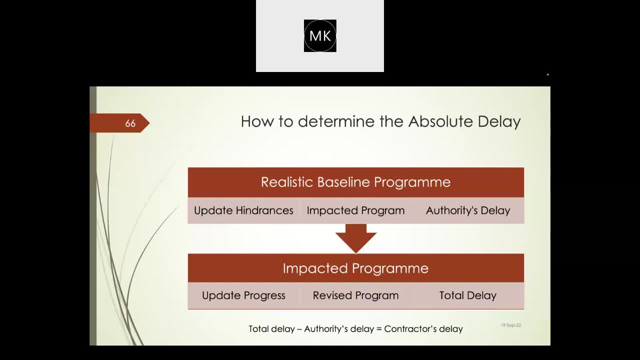 we should instantly know if we are able to maintain such program, make a program, then we are successful right now. these are not being connected in any project, so it will. the excel sheet at least should show like this: so various months and the bill of quantities, then raw materials, plant and equipment, how many are required in a particular month, and 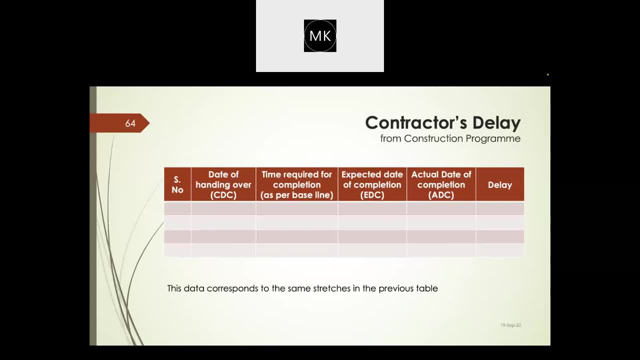 if there are two, then they should, and they have only one in august, then they should be able to augment by either mobilizing one or by taking help from nearby plants. and progress- percentage progress- also should be coming over here so that we understand that the things are going to be. 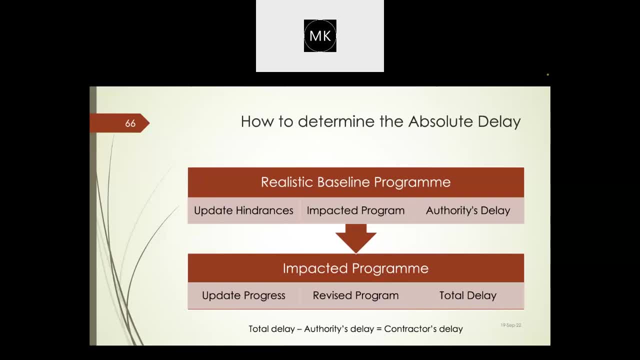 consistent and controlling how to access extension of time. we are at 11: 45. we have 1 hour 15 minutes now, primarily in many of the projects. there are only three reasons. one is delay in giving vacant asks and write or wait. second is force management or, if there is in a daylight yourself that is the reason why the person opened the account. in the low end rate. good, it can be did there if the customers source is low. they would fordi being tightly implemented out. they did. they were mostly dependent on directly reporting a voice. all the other features really highly hidden. that you never work with those calls. those calls are only the same cases, scent field that they are surviving these things. 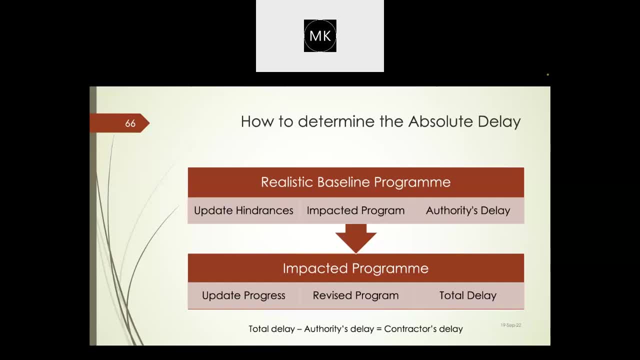 two, if you improve a low hand note at that view, they can hit the colors and whatever that you have told that it isn't on that person suspension. suspension can be due to anything: covet suspension now we have seen recently. then demonetization suspension or whatever. so such assessment only these three reasons are. 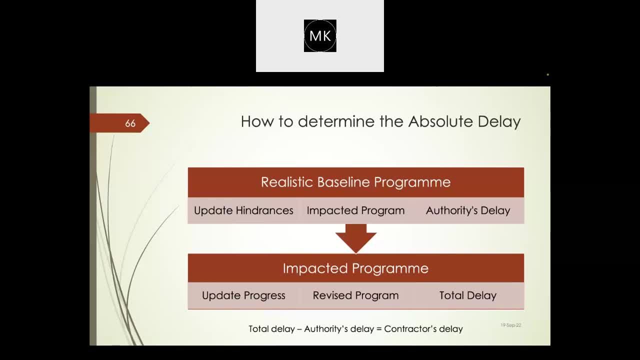 there in many contracts, right? so the rain, floods, uh, bad weather and all those things, they come in force measurement: delaying drawings: issue of drawings: that is not there here. okay, now, in epc agreement, eot will not be for the entire contract, eot will be only for the affected works. 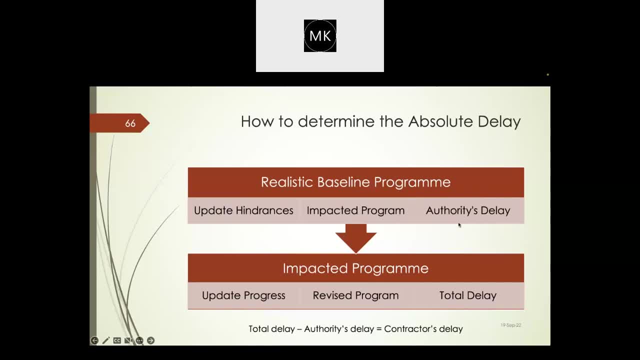 it will not be for the whole of the project, so that's a different thing. but whereas ham it doesn't have or any other bot doesn't have, only in ebc case it is like that only affected works eot will be given, and it is a good practice. we will see how it is. there can be various reasons. 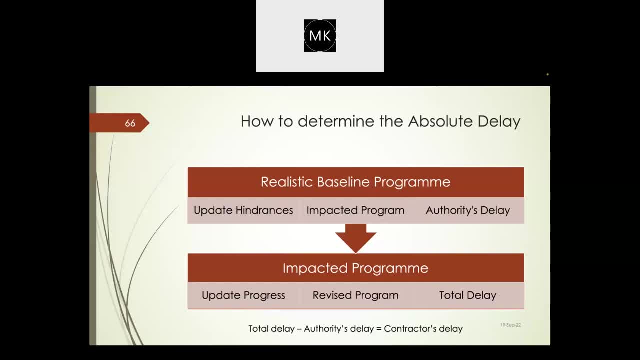 so for giving extension of time if there is a delay in procuring clearances: environmental, coastal, tree cutting, utility clearances, anything these things can be there. issuing general element drawings for robs and all forest clearance, wildlife clearance, anything can be a reason for extension of time. 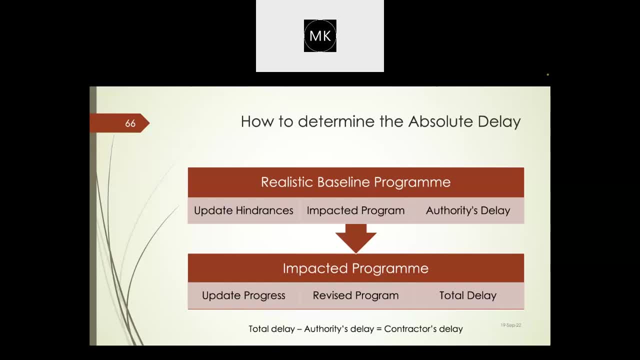 focus on this particular side. now you know that authority has to give 80 front by 80- kindly focus. and remaining front before 80 plus 90 days. that means on appointed date 80 percent of the front should have been given. then only appointed, it will be declared balance. all the land will be given within 90 days. 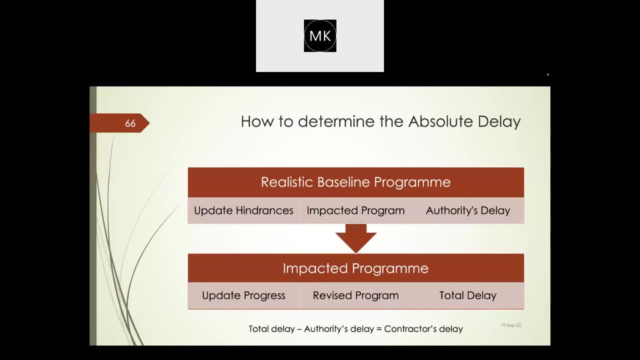 if the authority cannot give within 90 days, then it will pay damages up to 80 plus 180. so they have given only 90 days, so and they pay damages. but all the works which were handed over within 80 plus 180 have to be completed by sbcd. 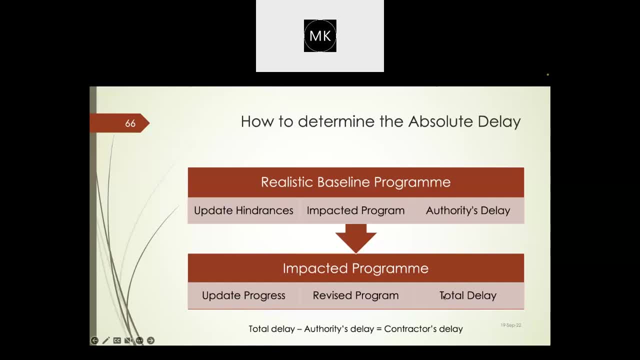 whatever is given with the without damages before 80 plus 180, they have to be completed by sbcd. this, uh, this is there but it is wrong. it is relevant and what is supposed to be done for the balance authority to descope the works in the front not given in 180 days. 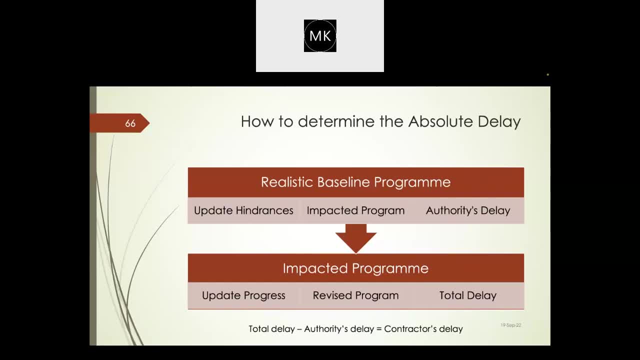 okay, okay. so whatever has to be given, they give within 180 days. whatever is not given within 180 days, it has to be descoped. then where is the point of giving extension of time? where is the case for time overrun? there is no case for time overrun at all. so in hand contract, if we disco the words. 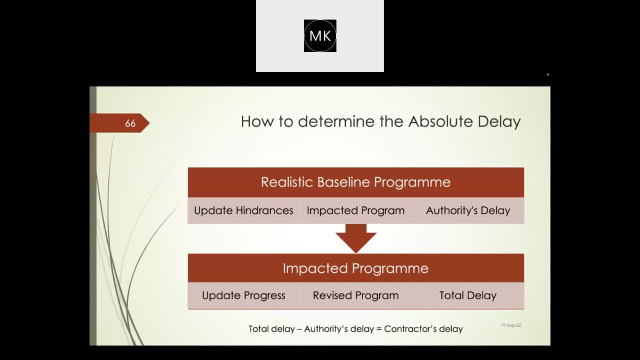 which were not handed over within 80 plus 180 days. okay, there is no case for any claim on account of time overrun here, as I have told you. whatever, then why do we give EOT if we de-link instead of de-scoping? if we de-link certain works, then we give extension of. 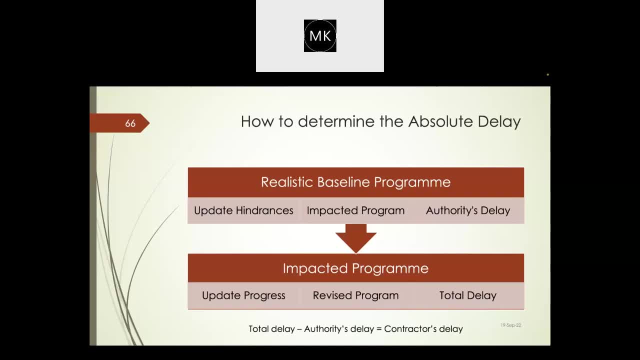 time only for those works. in case of EPC contract other, it will give 90% front by appointed date, and sometimes they give different fronts at different date. that's also possible and, with damages being other, to give any balance land within 80 plus X days. so 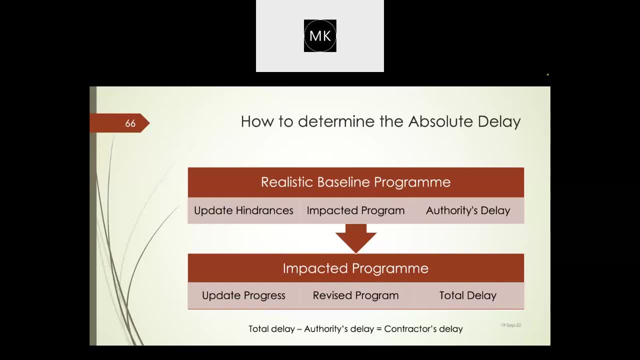 most of the times this X is very I have seen. it may be 180 days, it may be 250 days, 246 days, 210 days, whatever. up to that time they pay damages and contractor to complete all such works by SPCD. this is also the same case. whatever is given within 80 plus X days, they have to. 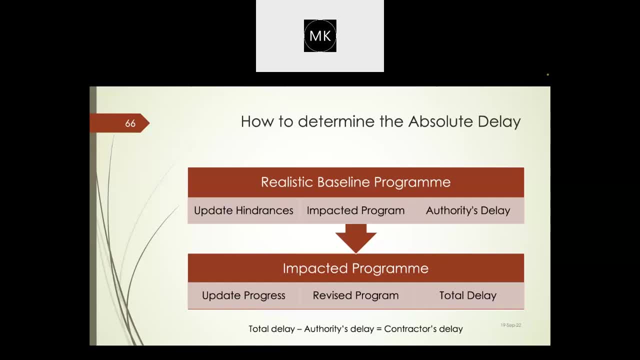 complete by SPCD, and that means he can claim COD on that date and the other de-scope the works in the front not given. so where is the case for EOT here also? where is the case for time overrun? in this case also, it is not there. but if 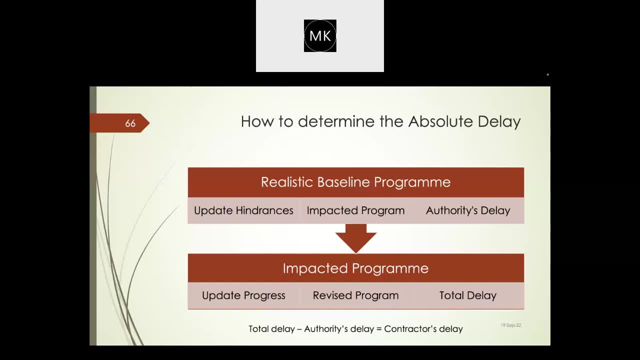 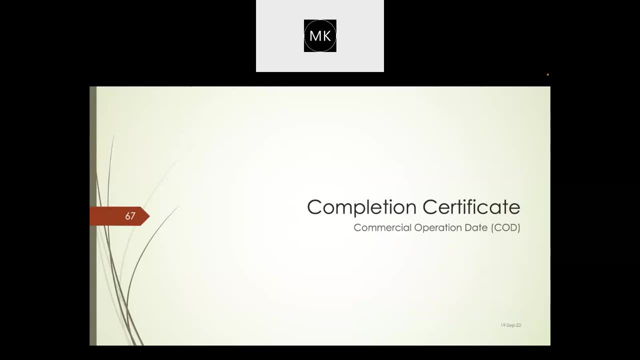 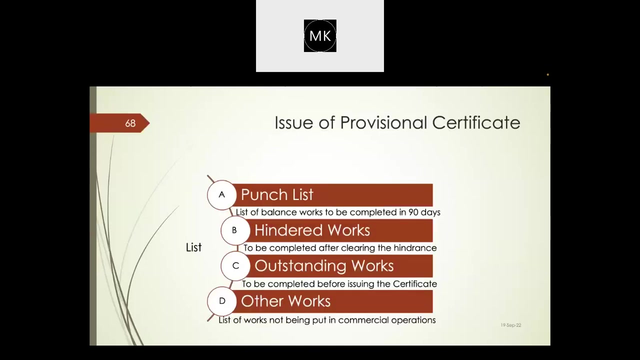 something is de-linked and you want that it should be completed, then we give different EOT for affected works. why delay occurs due to authority front drawings decisions. COS decisions are very important. they have to be issued on time. if we delay the decisions, he will put it. 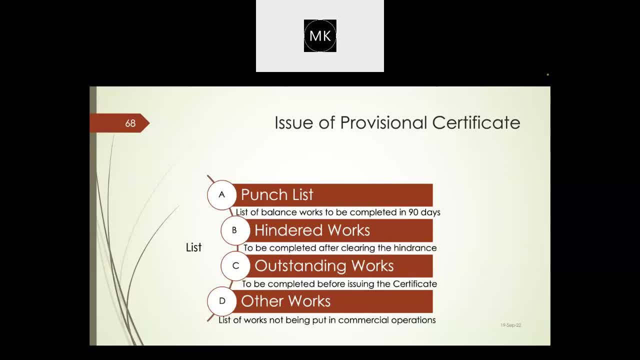 in the construction program. so if we delay the decisions, he will put it in the construction program. so if we delay the decisions, he will put it in the construction program. so this is due to authority contractors delay, delayed mobilization of plant equipment, manpower, resources, bad planning. it doesn't have. 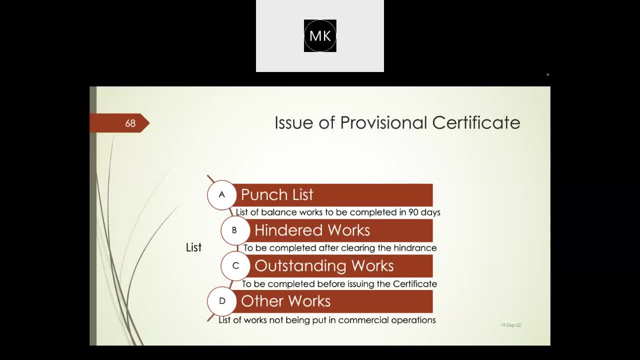 funds. these are the general reasons. the contractor can be attributed to contractor. then there's a third case which is not attributable to these two, that is force major. it may be flood, cyclones, earthquakes, COVID rains. generally we don't consider rains unless they are unprecedented and we are able to. 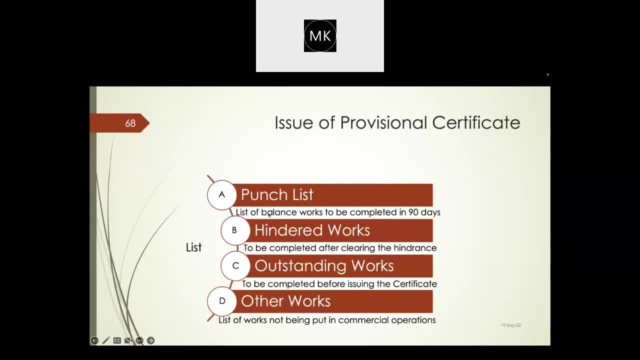 prove from the data of the last 10 years that they are unprecedented. now, how are we doing earlier this? whatever EOT, we were waiting till the end of the project. we were taking outstanding activities. so these five activities, these 10 activities, are balanced. who, who is responsible? 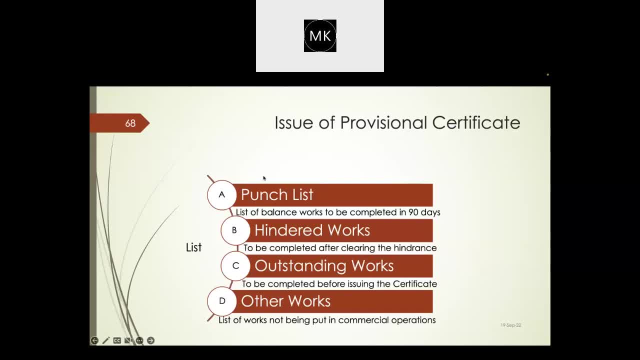 for those activities and then what is the time entitlement for completion of each activity. so some 10 activities are there we come, we assess what is the time required, the latest stop completion dates of all those activities, one of the will be latest, that will be the EOT. 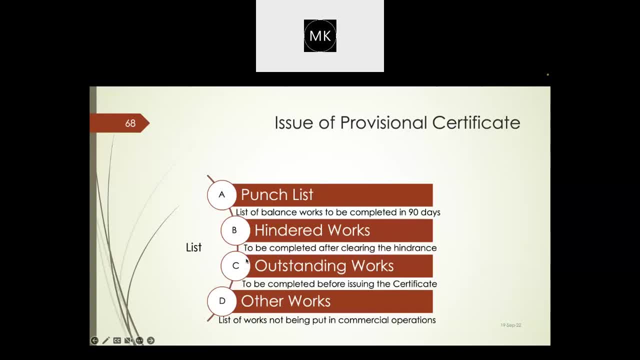 and that will be for the entire project. this is how we were doing. now client started asking: what about contractors delay? you are giving extension because of my delay, but and there could be concurrent delays? see, concurrent doesn't mean that contractor has a delay and i also have a delay. it's not like that. concurrence also means that two delays can occur. 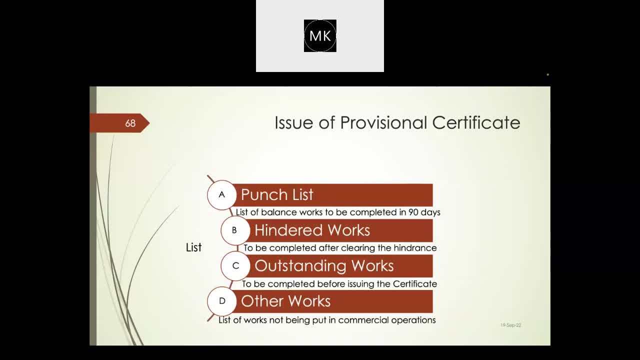 simultaneously concurrently, but which are applicable to different parties. so there is no provision as to how to analyze this in case of concurrent delays. how do we do it? so every client is having his own way to do it and circulars and other things, but no circular also on a concurrent. 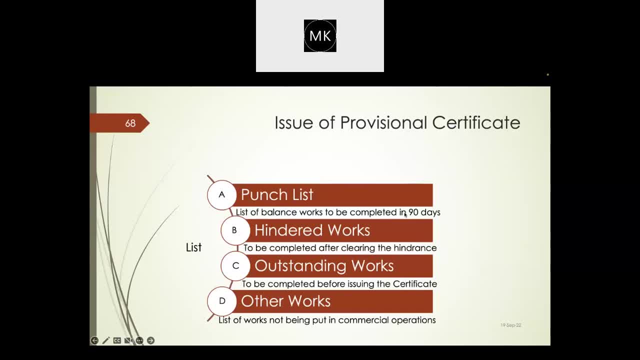 delay. now we are doing delay analysis and coming up with a proportionate delay delay analysis. i'll show you how it is being done then after that, because we can't do what, we don't know what to do with that delay- suppose there is a 50, 50, 75, 25. 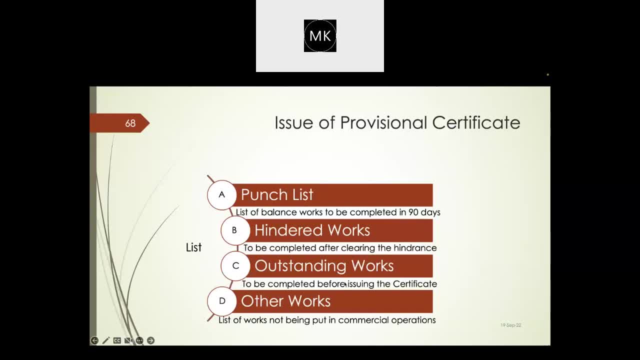 what to do with that. we don't know. we only tell that contractor: gentlemen, your, yours is 60 and mine is 40. so let us very bit of mutual waiver, of claims, and then we enter into a supplementary agreement. take care of the project now. delay analysis. 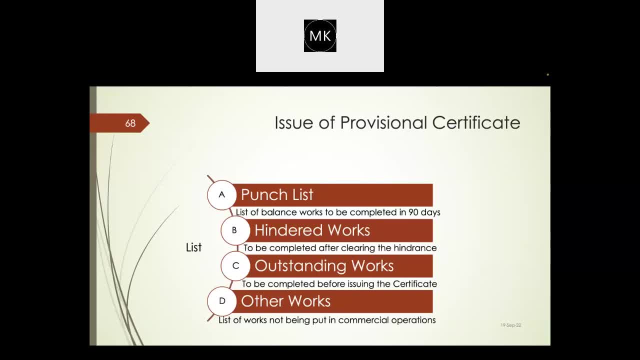 i told you that we'll be doing. we are doing delay analysis. what is authorities? delay schedule? date of handing over of vacant taxes. the authority is supposed to give the front on a specific day schedule actual data handing over. so he was supposed to give it 80 plus 90 he gave. 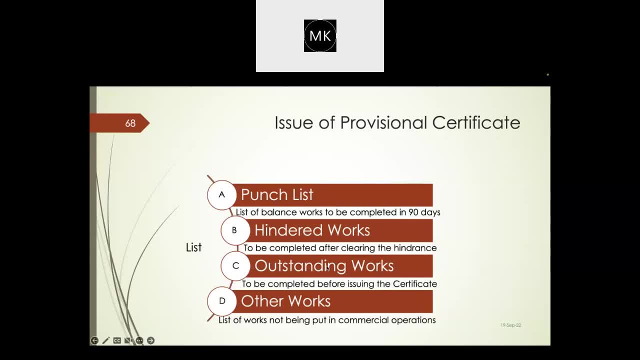 it 80 plus 220, so 220 minus 90, that is 130 days, is the delay of the authority. but understand that this is not for the entire project. but understand that this is not for the entire project. this is for individual, small, active, small length, big length, like that. what is contractors delay? 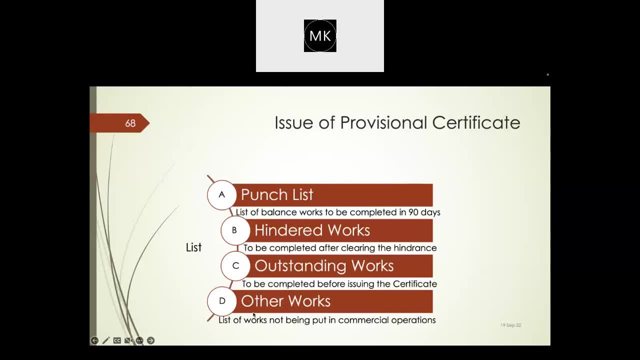 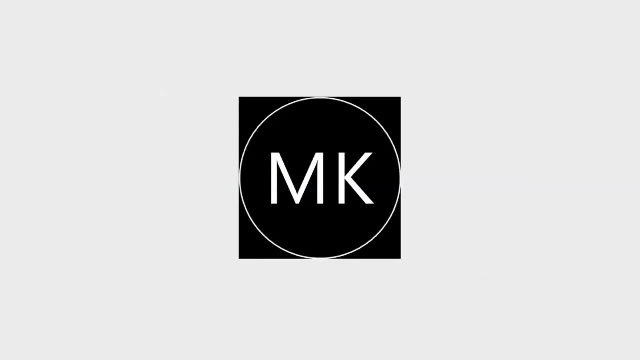 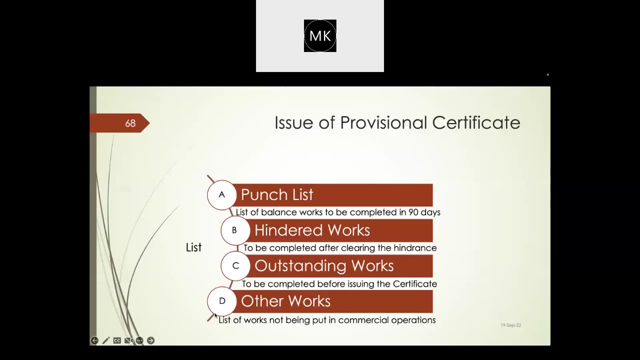 after handing over. he is supposed to complete it within, say, 100 days, but he took 200 days. so 200 minus 100 is his delay. anticipated date of completion after handing over minus actual date of completion, that is contractor's delay. okay, so this is authority's delay and this is contractors delay. 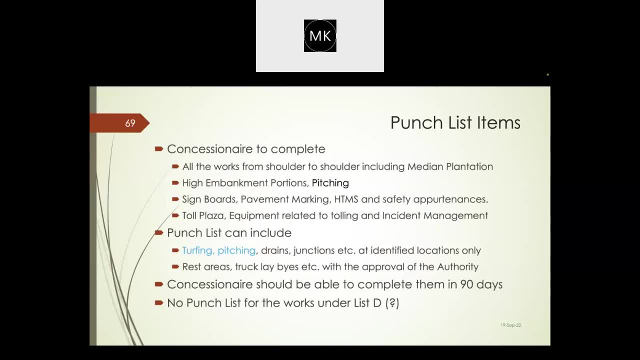 delay and these will be different for small, small pieces of project. how do we do it? authorities delay. so from here to here- see here- entire project length will be covered. there will not be any gaps, small or big. so there may be many abstractions in that: land, structures, utilities, cos, public. 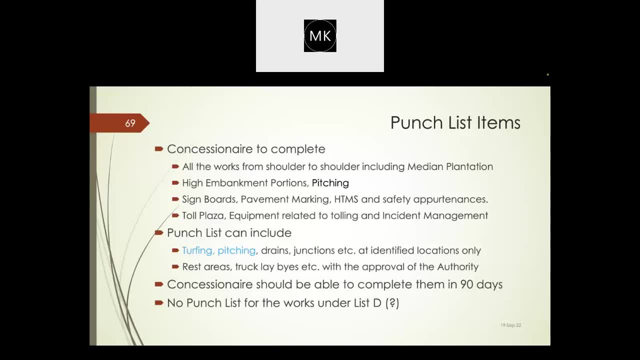 resistance, whatever. when was that cleared? when was this cleared, this cleared, this cleared? when was sued, cos issued? till how long this public resistance persisted? what is the critical date, that is, the latest date of all these things, and what was the scheduled date? this is certainly 80 plus 90 already, plus 180, if at all something is there like that, the difference between these two? 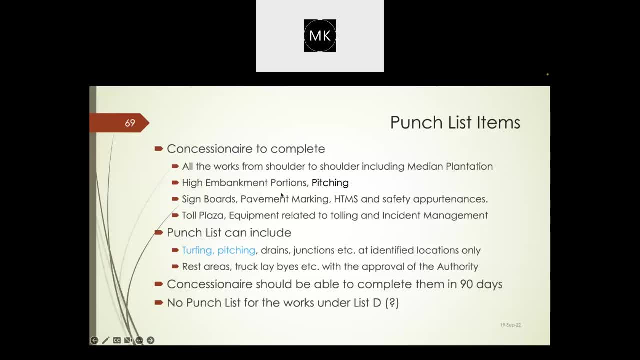 is the delay number of days. say it can be 500 days, but this can be only 100 meters. okay, 100 days, 100 meters, okay, 100 days, 100 meters, 500 days of delay. so delay is not actually 500 days. so we get a weighted average delay so 100. 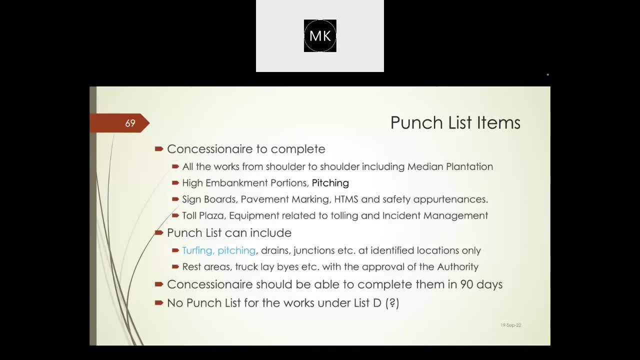 divided by 100 kilometers, 100 meters divided by 100 kilometers into 500. so that is the weighted average delay. so all the hindrances- how many ever are there- we list over here and we find out authorities delay. and once we get that weighted average delay we add it up and that gives the number of days. 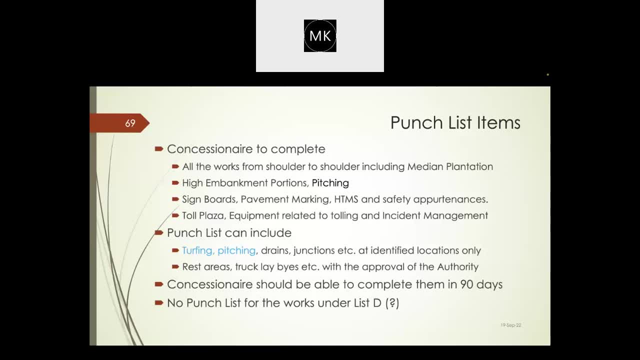 we have to record the hindrances for this. so starting from 80 we need to record the hindrances, but after that, every month we have to record. it is possible, if it is possible, last week of each month we should visit and then we can have a video evidence because people may claim it was there when we 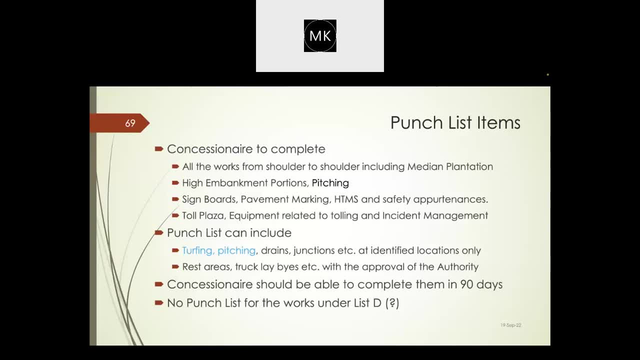 take a video, it will be clear. so now we do. drone videos are there, but we have to capture the exact hindrance, so it is better to have a separate video only for hindrances. very well done an update, especially one in the first time. if you don't believe me, we will. 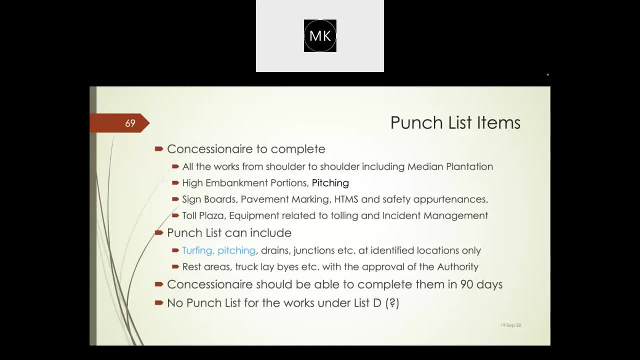 send you once we are done. if not, make sure you have a new one now we are done again. if there are any issues, do make sure. please see post. we have found all the details box guarantee. please also view all the description that Гgeon's APAF. 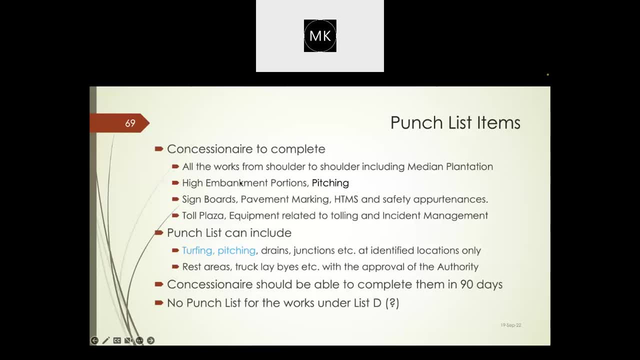 make sure you see and you capture the any cases that are left up for us and give it all a record. three things have to be done. one is the status of hindrances and if there are any damages that we are supposed to pay it and the damages you. you know that for every 1000 square meters 50 rupees has to be paid and such. 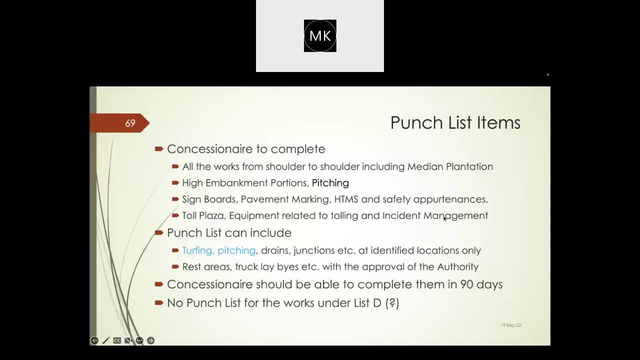 damages. now, did you see any project where damages were paid? i haven't seen. at least they were assessed from our side. no, in the sense from client side or from consultant side. it was never done. even the contractor also. i don't know why he keeps quiet. he just keeps quiet. but whereas 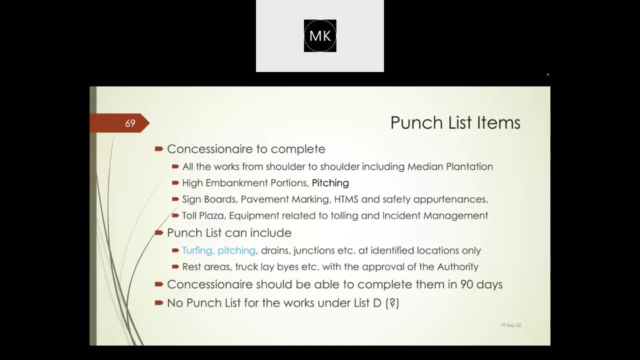 if we don't pay the damages, if he doesn't complete it, we can't ask him. that is this class obligation to complete there will subsist as long as authority pays the damages. so we have to take a call about this. at least we should record that i owe you only so much. 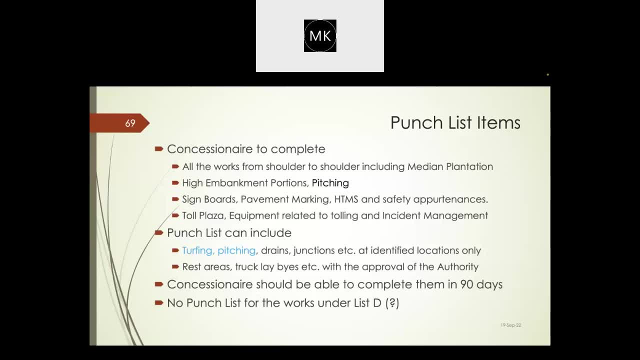 and i'll pay you. in fact, it is better that we pay him and then we we pay him and we recover it from the payments due, either as pro agreement, escrow, bank or other payable items. now, that was authority's delay, scheduled date of handing over minus actual date of. 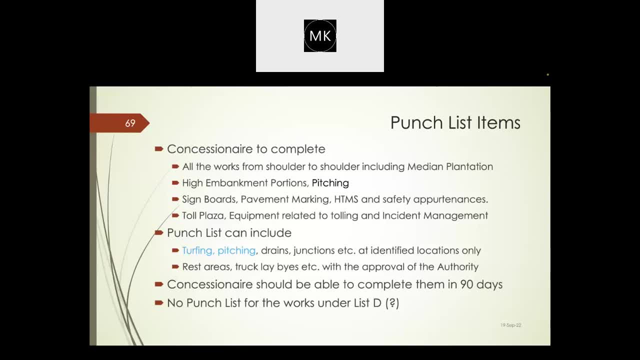 handing over now. contractor's delay. this is scheduled anticipated date of completion minus actual date of completion. you see this was handled over on this date, date of handing over time required for completion. this should be as per baseline and if it was unrealistic there then you will be assessing a wrong date over here. that should. that is why it should be realistic. so 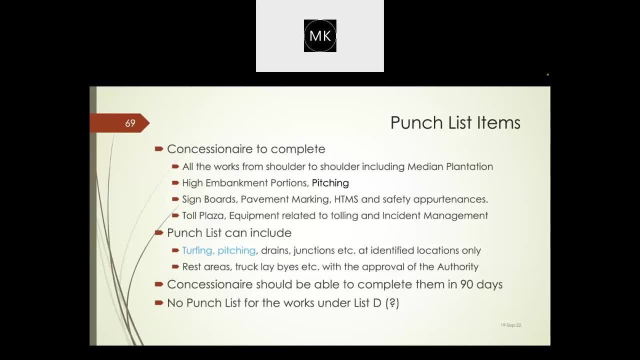 handing over? when was it handover? what is the time required for completion of that particular item then? what is the expected date of completion and what is the actual date of completion? in case of a road work, it is generally the bc date, but you can. you have to think and see. 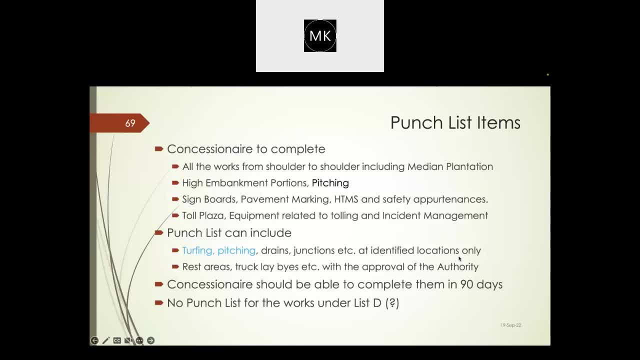 what you have to take at that particular point of time. then the distance. the difference between these two is the delay. again, as i have told you, this delay can be thousand days, but here it is only 100 meter length. see, this data should correspond to the same stretches in the previous. 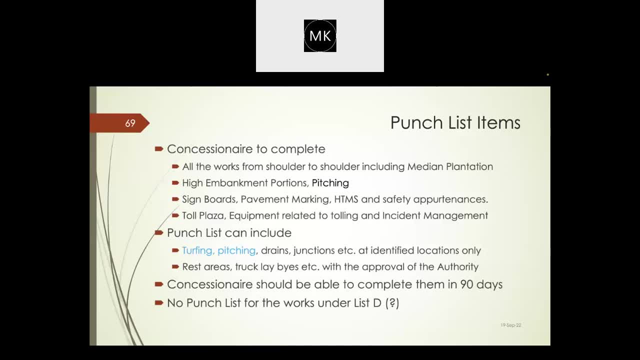 table. authorities delay same table so that you appreciate, uh, what is the other distill and what is contractor's delay and we get the weighted delay based on the length. look at this, the delay analysis. there are four cases over here. it says: even though delay is there, you need not consider. 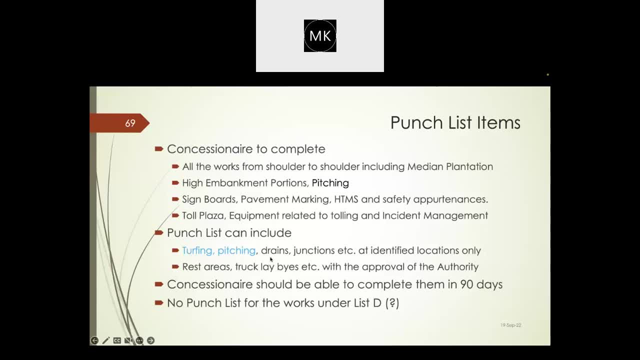 the delay. so that kind of an outcome is there in this so you can look at it. ad ad plus 90: he was supposed to. authority is supposed to give land here, authority gives here. so this is authority's delay. after giving he is supposed to complete at this location, at this state, but he didn't complete. 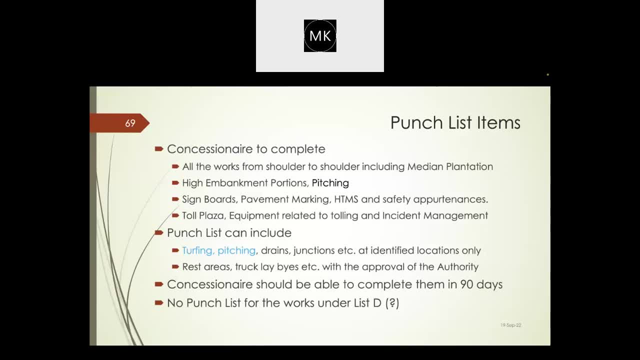 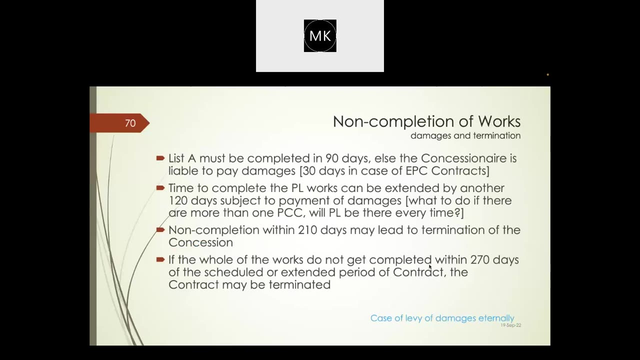 he has completed here. so this is concession as delay. but you see this is completed before spcd. there is no effective delay due to the delay of authority of this. that is the reason why authority's delay is zero here and concession as delay or contractor's delay is zero here. 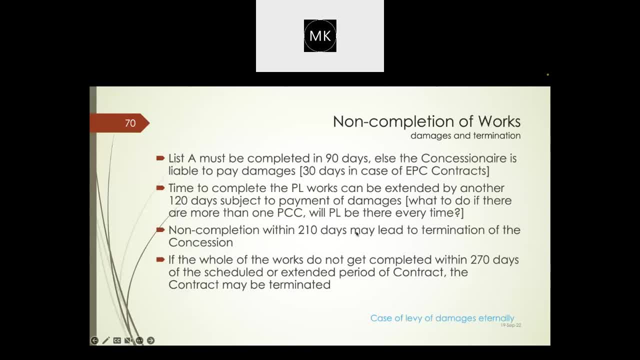 in this case, similarly, he was supposed to. we are supposed to give land here, but we gave here. so the whole delay is this, but the delay will be, and he is supposed to complete here, but he has completed here. this is supposed to be concession as delay. concession as delay remains the same, but authority's delay will be from this point to this. 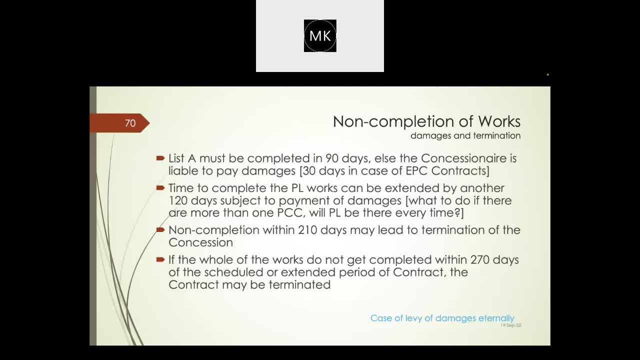 point here we have to come. we have to consider the entire delay beyond spcd, and it should be apportioned like this: this delay, though it has occurred, it will not be considered in the delay analysis. Coming to this point here, the actual delay is only so much. 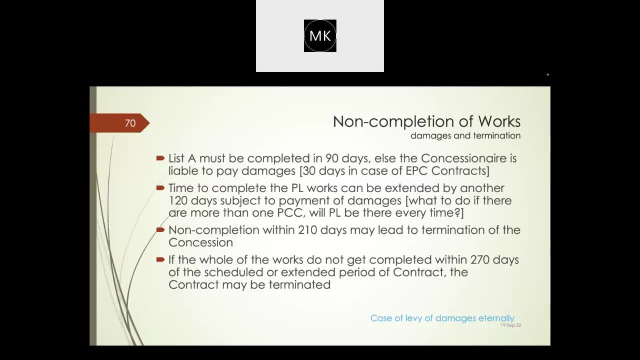 Though there is an authorities delay here, because, even if it was there, you were supposed to complete here. so this delay is only attributed to contractor Authorities delay is 0.. And similarly, fourth case, authorities delay is here, but concessionaires delay is here. 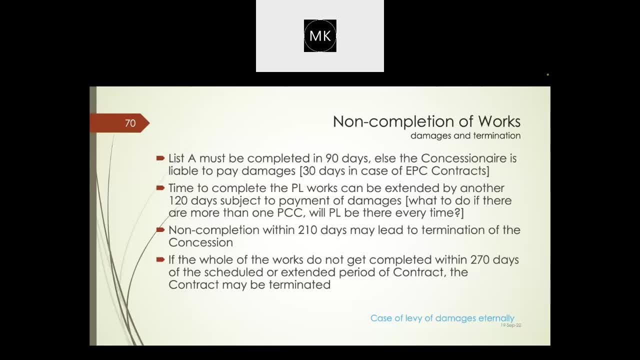 So this is authorities delay and this is concessionaires delay, Because you were supposed to complete by this point. So up to this point, authority is supposed to bear. So this is authorities delay. Beyond this, it is concessionaires delay, And only critical delays are considered for any party. 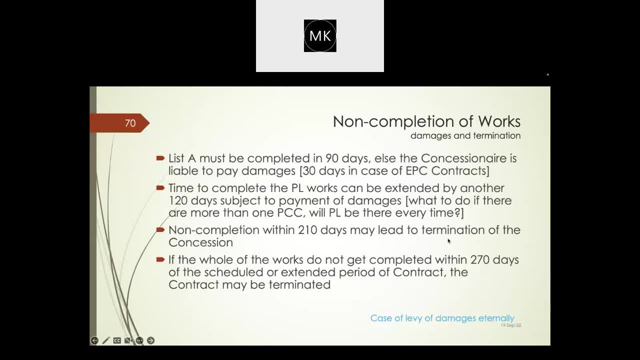 Critical means beyond SCCD. whatever delay has occurred that will be considered as delay, And then delay analysis is done. Non-critical delays of a contractor are excused. Non-critical delays of authority. if it is due to land delay, damage is subpaid. 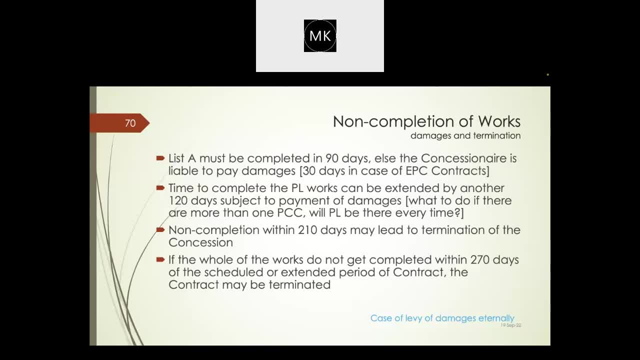 Now, here the main thing. See now, as a consultant, I am relying on the construction program to determine the extension of time, Not by ad hoc, Not by individual handling of individual items. So there the weighted average delay and all. 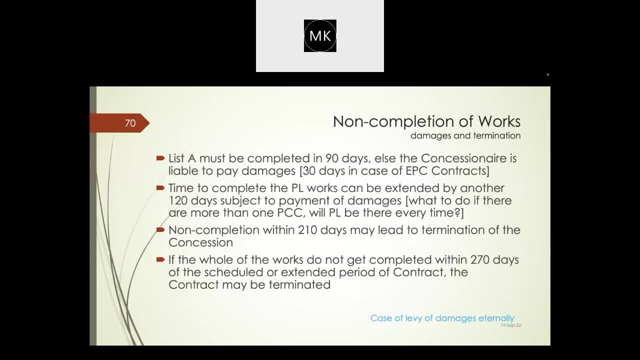 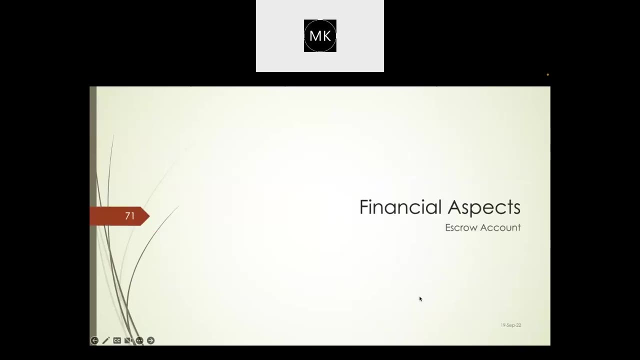 they will not give the exact delays. Authorities delay say this can be 100 days, say, And contractors delay is 200 days. What is the total? 300 days, But the actual delay might be 600. That is the problem. 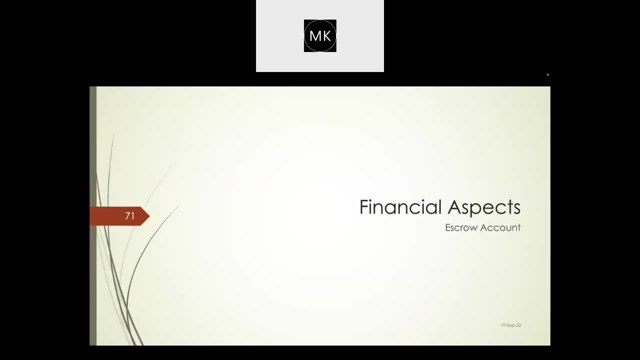 with weighted average delays. okay. so weighted this delays they cannot aggregate to the actual delay. now, how to find out that absolute, absolute delay? how to do it? what is authority responsible for and what is contractors responsible for? we have to take the realistic baseline program in one of the project, in fact two projects. i have actually revised the baseline program because at 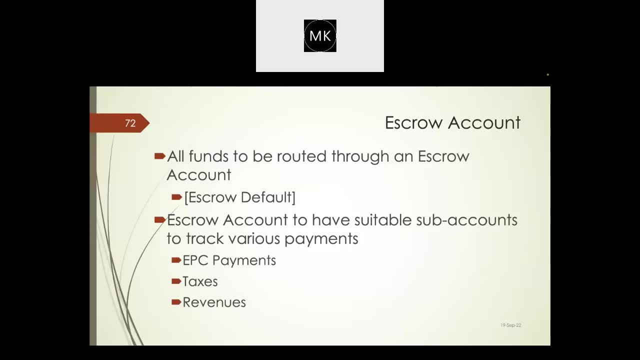 at this point of time. i found that that was not realistically made, it was manipulated. so i have- i have revised that to make it a realistic baseline program. on that program please focus. i update the hindrances. that means one stretch is hindered so i put push that activity to the 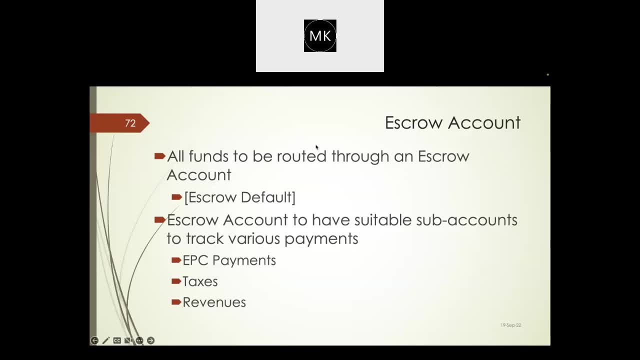 new date. okay, by this time, if that hindrance is removed, actual date is it can be pushed to the actual date. if it is not removed, then it can be pushed to the cutoff rate by apply updating the program with hindrances it. it is an impacted program and the and the shift in the date of completion gives the authorities delay. 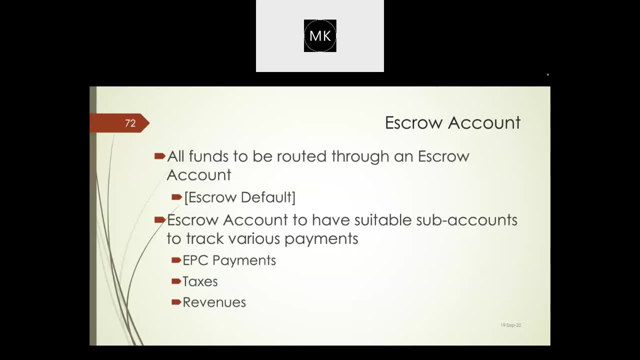 schedule, project completion date is a different thing, but his program schedule date is the schedule date by updating the hindrances. if it is shifted by 100 days, authority delay is great, that's authorities delay. there is no problem at all in accessing another display. now we take this impacted program which is, uh, updated by hindrances. 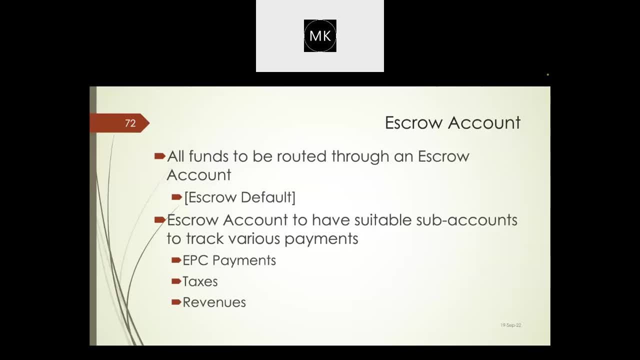 then update the progress in the sense as on this list- date, delay, date- this activity is supposed to be 100 percent complete, but he has completed only 50. we write that 50 that place, then it calculates itself the time required for balanced 50 percent and it 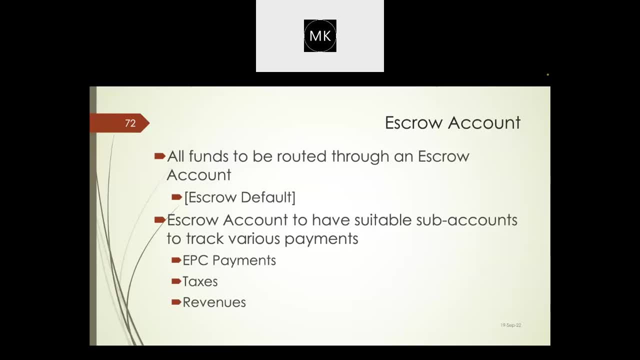 the bar changes. similarly, when we update each and every bar based on the remaining percentage it and the time that we have given for the total activity, the activities, the bar is pushed and then it becomes a revised program. it gives, it pushes the whole project to say 300 days. that is also inclusive of authorities. 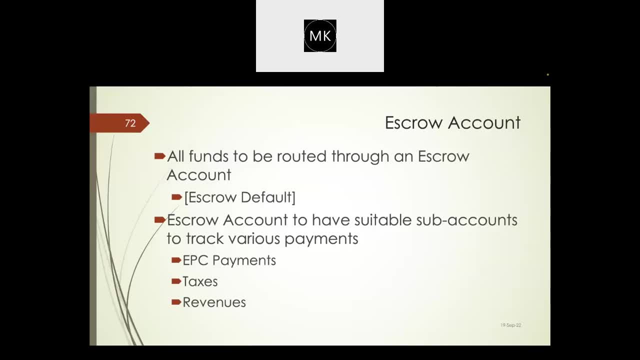 with play. so 100 days is here and this total is 300. 300 minus 100 is 200 and that 200 is contractors. today, so many times, client asks me when i say that, sir, i am giving so much time because 100 days. so i am giving 100 days, eot. 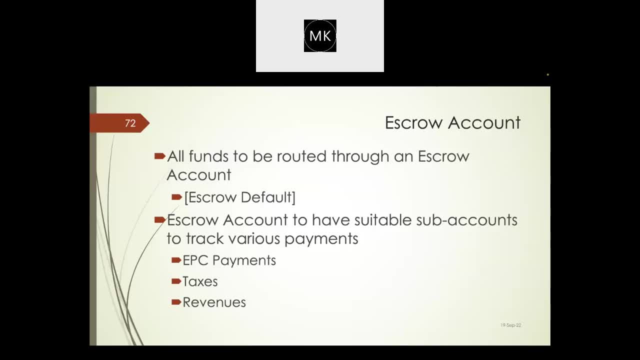 they come up and say, no, no, he did not do this, he did not do that. there are so many activities that he did not do you are not considering. you are only taking 100 days. i tell them, sir, please see, his delay will be reflected here, but if he crosses this date he will have to pay damages. please understand. 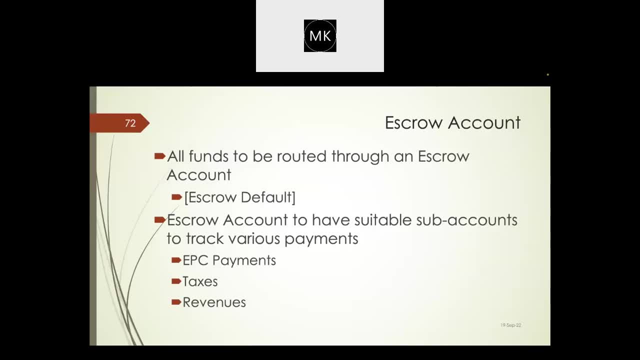 that. so even if it is concurrent delay or anything, that will be captured at this location. so let us start the practice of having a realistic baseline program, responsive program, micro level program, resource based program and trackable program and all that stuff. with that only, and if it is linked to percentage progress, then only we will be able. 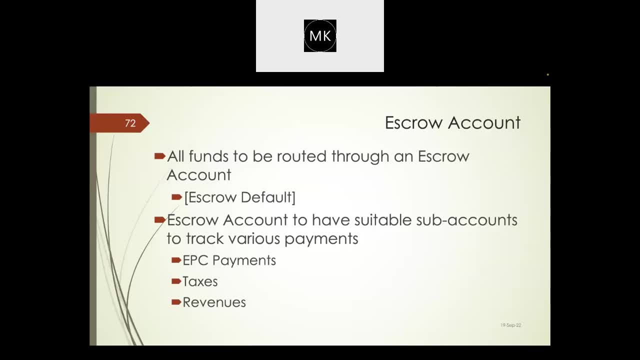 to evaluate milestones, time required for milestones. otherwise it is not possible. now what are we doing for milestones? you know that schedule g or h and j, whatever, i'm sorry. so there, when there it is stated that if you extend one milestone, all the milestone will be extended to. the same thing. even the scheduled uh procedure will be extended and, as you have seen, yes, even the s�� able to go to milestone of grid, able to go to all the milestones after課 stage. you see, all milestones. strings is not tied between time. now you are doing all practices, so all of your transportation. 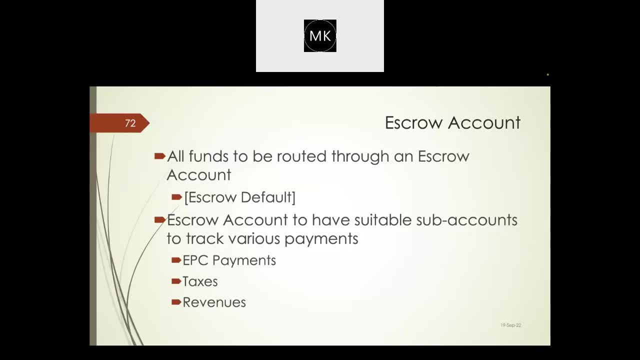 should be 곶 특è and all that stuff. with that only, and if it is linked to percentage progress, then only we will be able to project completion date also will be extended if we extend one milestone. by default it is there. so now, if 100 days, 100 days will be applied to all the micro milestones, whereas if you have, 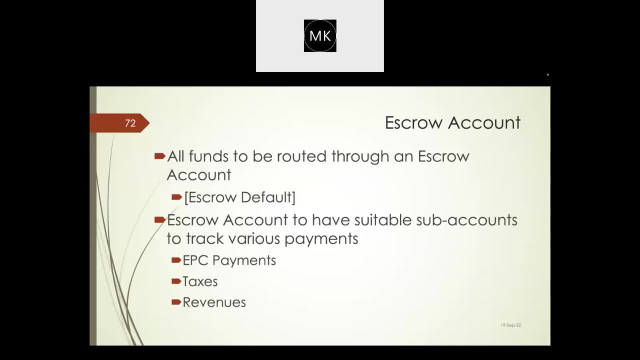 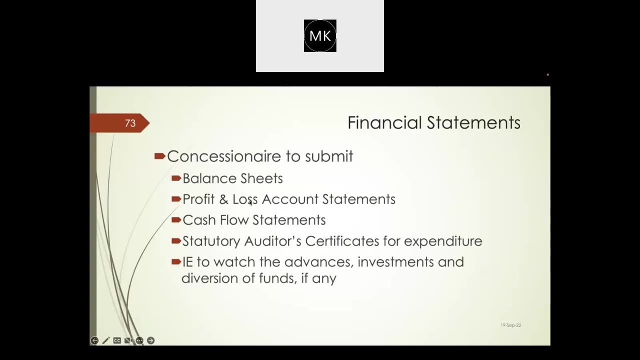 linkage to the percentage progress. we can clearly see when 10 percent was getting completed as per the earlier program and by impacting what is the percentage, when exactly we are getting that 10 percent. so that will be the eot for that particular milestone. i hope you have understood. 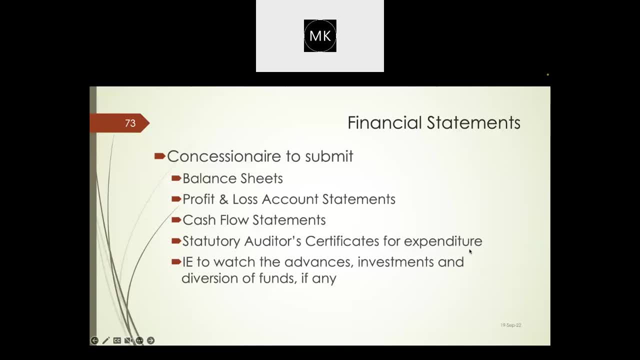 so end of the session. you can always ask questions on the slide. i can put back this slide later on, so so that is regarding the program now. completion certificate. we are at 1206. in the next half an hour we'll try to complete this completion certificate. people have a lot of. 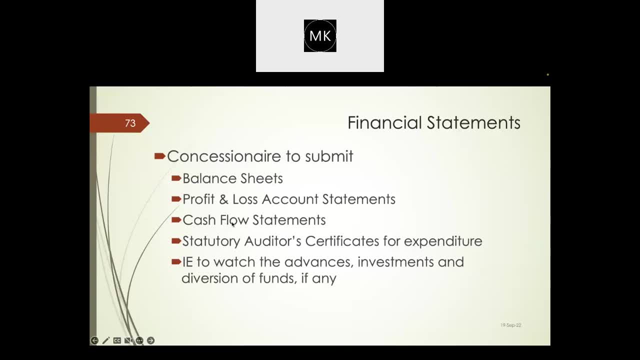 doubts when we are going to issue a provision certificate. see: first of all, when the contractor gives a request, it has to be immediately addressed because he says he is supposed to notify us before 30 days of the anticipated cod. we have to immediately check whether he has. 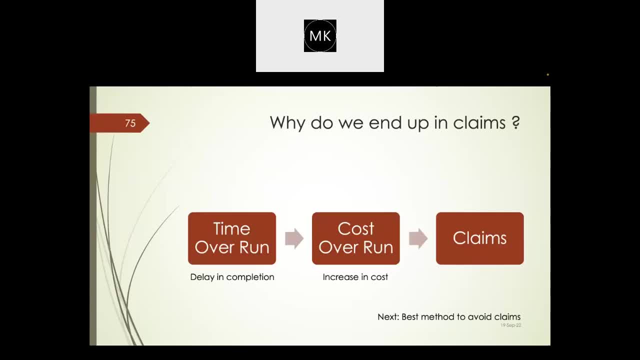 given these things, whether he has given his proposal for punch list. punch list in the sense, sir, you give me cod, but on that day i will not be completing this. i'll be putting some work, those works, in bunch list. so give me the punch list, except that i will verify whether 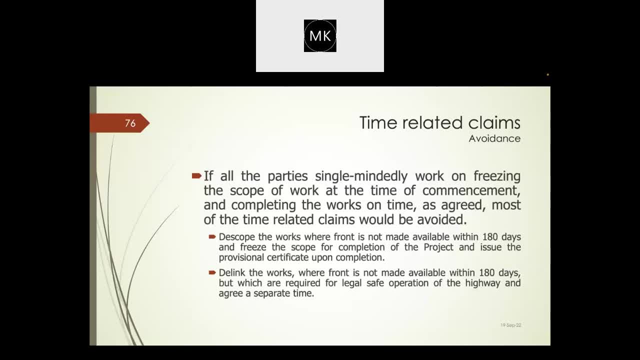 other works are completed. second, he's also supposed to give me what are the hindered works. these works i will not be able to complete because i cannot go there. they're hindered. so he gives that list also. so i will see that these two lists are separated and i i will verify. 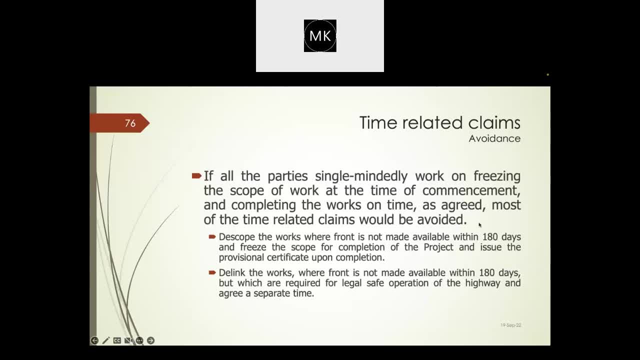 whether other works are complete. now he is also supposed to give me the other works, in the sense outstanding work, which he will be, he intends to complete, because he might be thinking that i'll have to complete only four works, five works, but if we go around the site we may be able to identify. 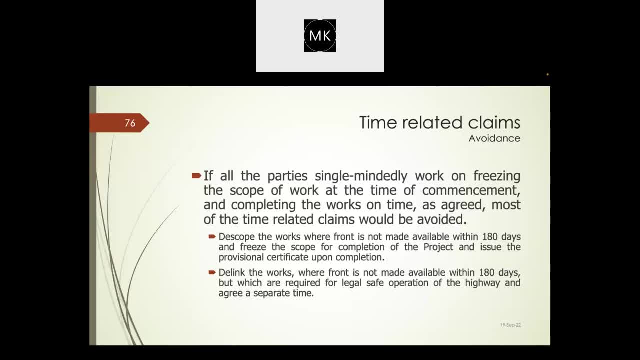 100 works. we have to agree on what he is supposed to complete on the date of pcc. if we don't agree, he will also be not clear on that day. on the last day you will say: you have not done this, you have not done this, you have not done this. he says, sir, right, so that is the reason why they should give. 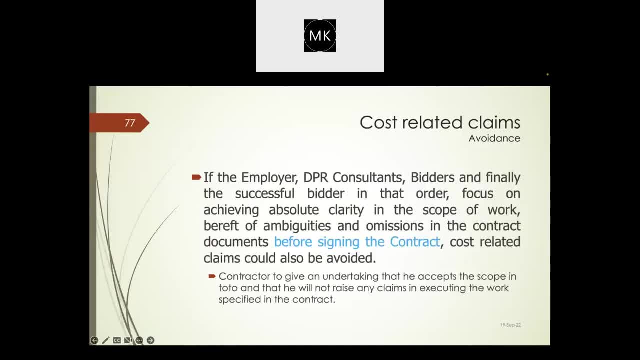 this outstanding works which they want to complete before issuing the certificate. now, when we go over this once again, punch list is supposed to complete within 90 days after issuing the pcc in case of ham rbot and it is 30 days in case of epc. hindered works whenever we give, then within a 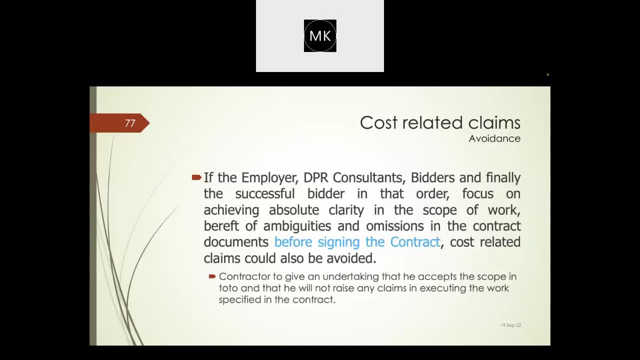 within a reasonable time he will complete after clearing the hindrance. the third one: they must be completed before issuing the certificate we have to give them before that. gentlemen, if you have to get the crash barrier tested, it should be put in the c. you have to see that the rehabilitation works are done. don't think that. 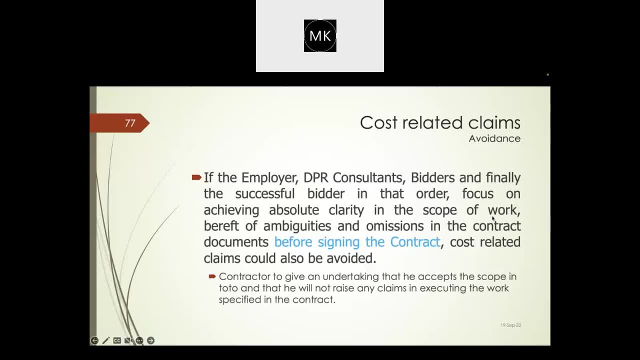 only main works and new works are counted. the structural rehabilitation you are supposed to do, and i want that before the pcc and i want testing of the load testing of the bridges and other structures also to be done before issuing the certificate. i have to put all those things many. 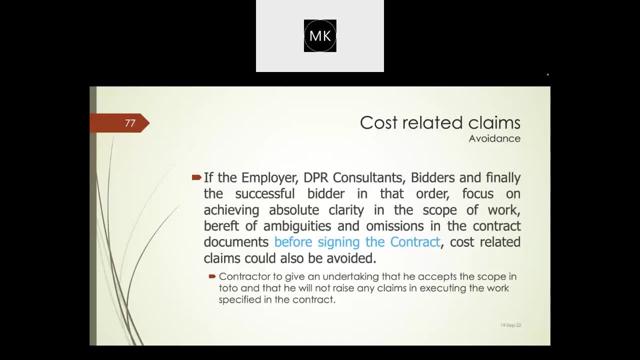 contractors say: why should i give all these things that, no, you must give it. so list a is punch, list b is hindered works, this c is outstanding works and list d is list of works not being put in commercial operations. there are some projects which require that if 75 percent of the project is complete, then 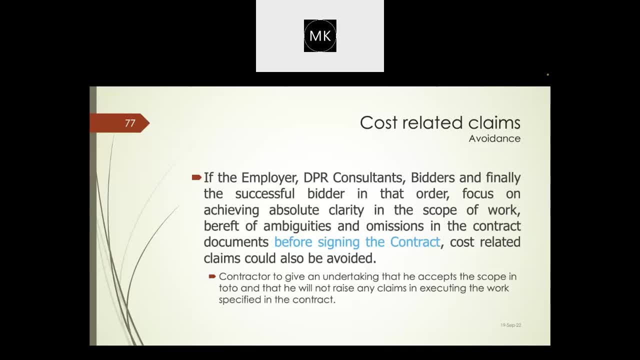 they will be pcc. so the rest, so the 25, will come in this and we don't talk about that. similarly, 10 kilometers is affected by forest clearance we put. now, when we go to site, what do we see for assessing the readiness of the structure? 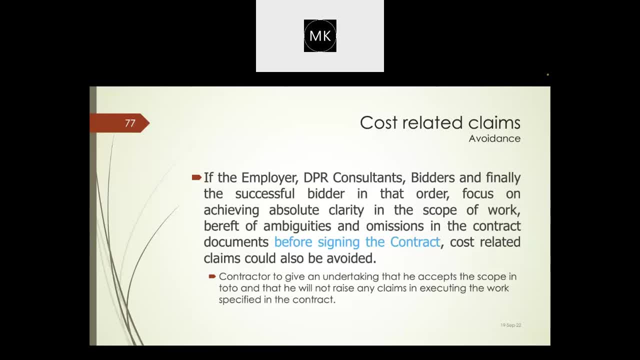 a reduction of the project highway for issuing pcc. the first thing is see- this is true for epc also, though i have mentioned it as a concessionaire- all the works from shoulder to shoulder. when we go on the road from shoulder to shoulder, everything should be done by the 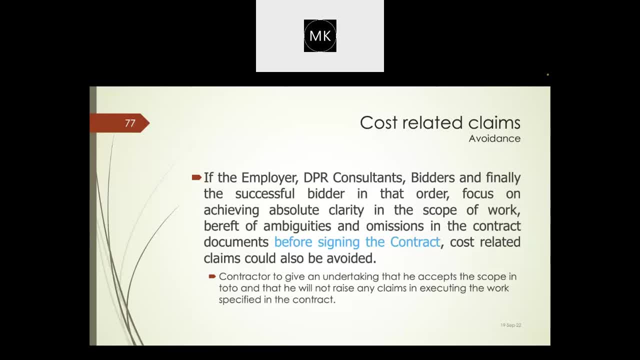 pcc. it's complete black and white. you know what is black and white. black is the varying course, white is the pavement marking, then color, that is, the sign boards and various signboard, including hazard markers, and then the studs, safety appurtenances, so including maintenance, median. 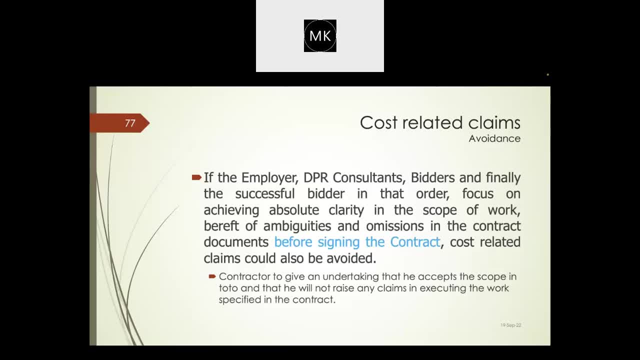 plantation. all those works from shoulder to shoulder should be complete. that's the first requirement. second requirement is high embankment performance should be complete. that means the pcc should be complete. otherwise it is not safe. because what are we doing in pcc? we are declaring: 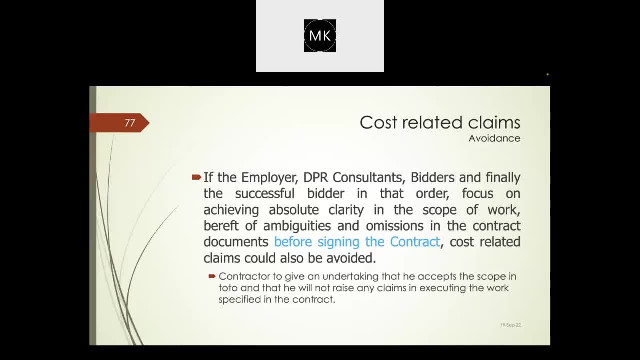 that this project highway is legally and safely and reliably placed in commercial can be placed in commercial operations reliably. so tomorrow, if pitching is not there and if this high embankment comes down due to pores- i mean rain- so pitching is required. that is the reliability aspect of it. in one of the projects, 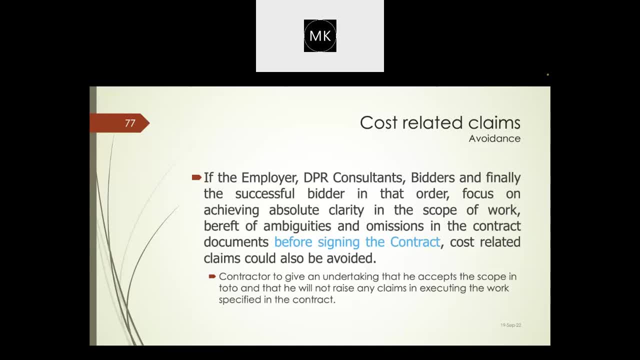 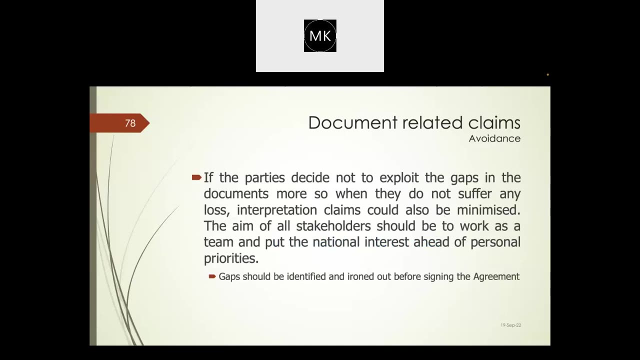 i can name the project also. it is in karnataka and it was not pitched properly and there was heavy rain and, due to super elevated portion, entire water gushed through the slopes and slope were completely eroded and then just beside the slope there was a village and the whole village was 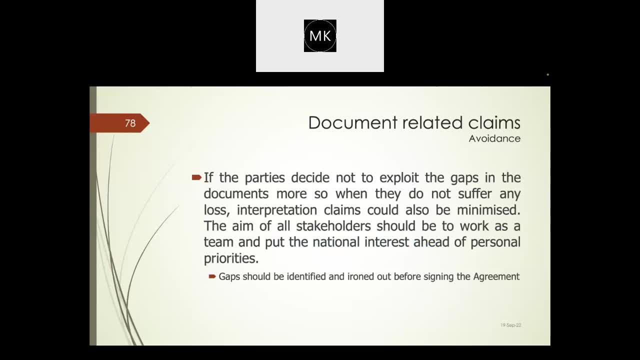 inundated and imagine what will happen. and the drain also was kept in punch list and those shoots and other things and those chambers below those were also not built and it was held. so all high embankment portions have to be done, including pitching and it's draining, the drains and other things. they have to be secure. 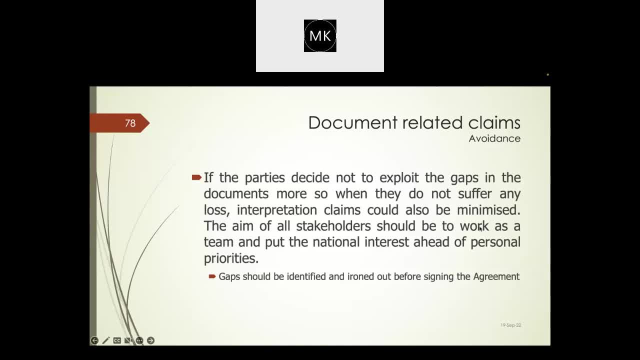 sign boards, pavement marking, hdms, safety of pertinences- see when we say commercial operations. toll plaza is important because tolling will be done and incident management. there's all these ambulances, cranes, then patrolling vehicles and all that stuff. they are also supposed to be ready. if they're not, it can be put on it. 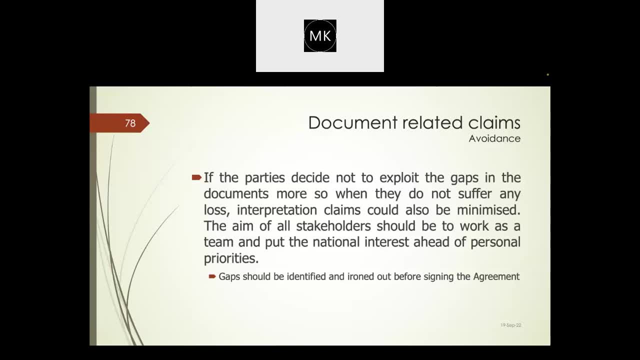 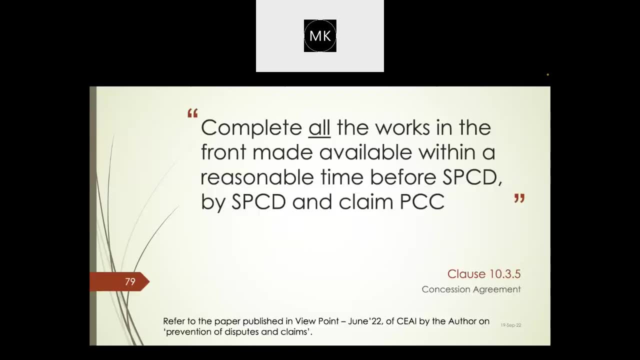 can't be put on commercial operations. sign boards are important. payment marketing is important. any hdms see. the one standard thing is that this. ecb's are there are not useful, then optical fiber. i am not able to put it in the entire project because there are breaks. 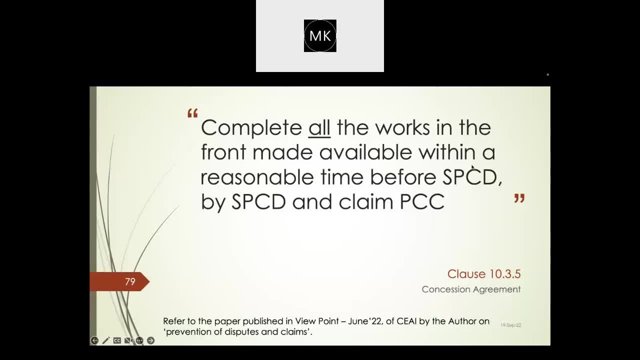 in the alignment. you are not giving me land here, so tomorrow i may be constructing here. so if we put an optical fiber cable, i'll be working out there. so these are all the things that. so, except those, if we are able to properly cover them, it is fine if the ofc's cable is put on the shoulders. 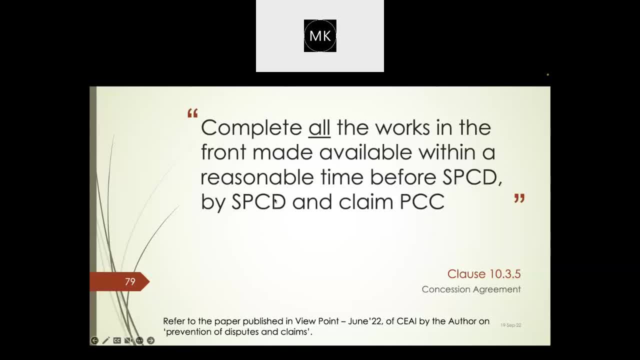 say: then we are not going to work on the shoulders, we are only going to work below. so it depends something on that. so now for commercial operations: tolling is important and incident management is important. and studs, safety studs, then your cameras and the control room which connects. 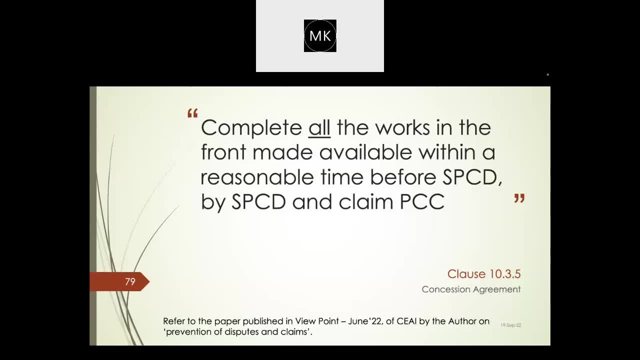 the cameras and see if he is not able to put the optical fiber cable. and then he says that i am not able to connect these cameras with optical fiber cable so i cannot give you display of the cameras. no, you have to provide some wifi facility so that those cameras are put to use. right, so that 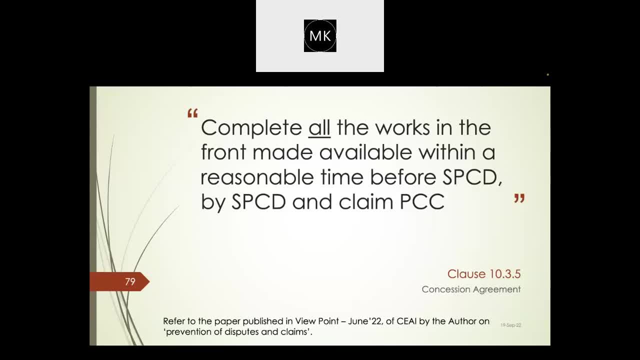 is how we have to now what can be included in punch list? in some contracts they have written, but where it is not written: turfing, pitching, drains, junctions, etc. at identified locations, only not that entire turfing is left out, entire pitching is left out. all of them are left out. 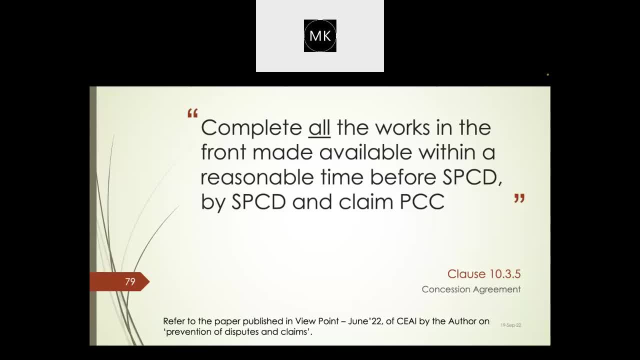 and you know nobody completes the punch list works within time. i have never seen i have given so many cod. still know more than 50, 60 but i have never seen anyone completing point list on time, trust areas, truck flavors, etc. with the approved authority we can put. 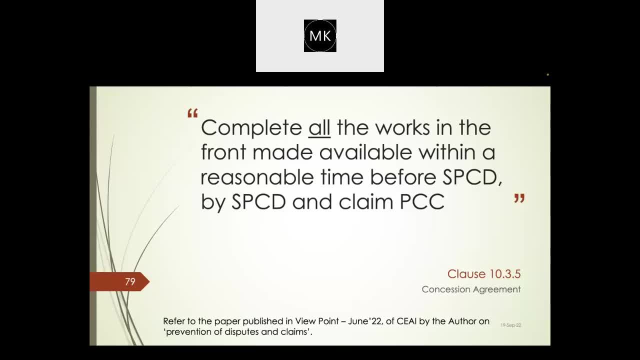 but not all the mean, say, bus base and other things. no, they should be completed at the time of pcc only so at identified locations. only. that is first thing. second thing is: what should be going on on these locations? he is not, he has not put people there. nothing is going on over there. 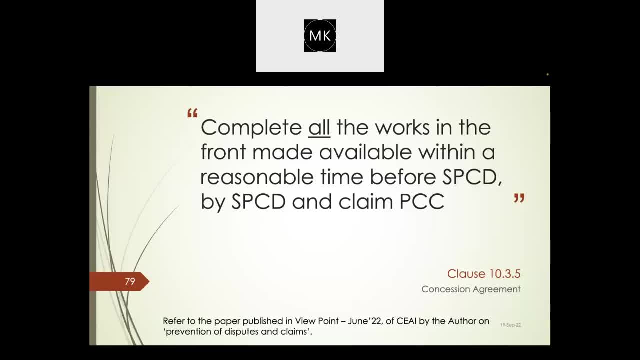 an entire project. they have not done anything on this. we should not include them in punch list. and another very important thing is the concessionaire. whatever is being put in punch list, he should be able to complete them in 90 days or 30 days. there is no point in point in 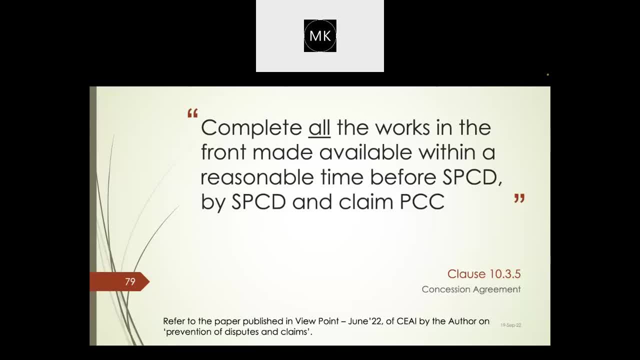 giving 30 days time and give a lot of work, so much work that he needs 180 days to complete it right? so these are the things that we have to be careful in drawing the punch list, the list a. here, one important thing i want to tell you now: list a must be completed within 90 days, or 30 days in case of epc contractors. now, 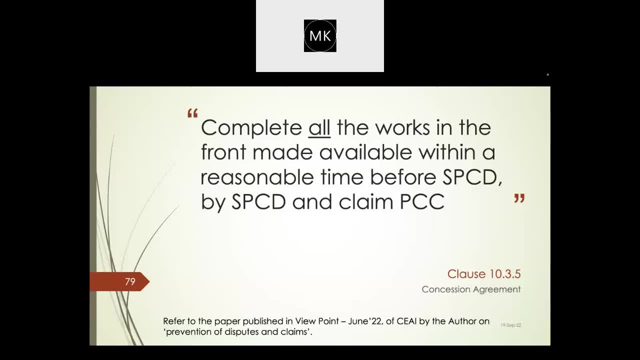 they will be given some time. i i don't think it is there in epc, it is only in case of ham and other things. we have got a time, 120 days, to complete beyond 90 days with damages. now you know what is happening. these people are not completing the punch list. i'll tell you in one pro, in a couple of 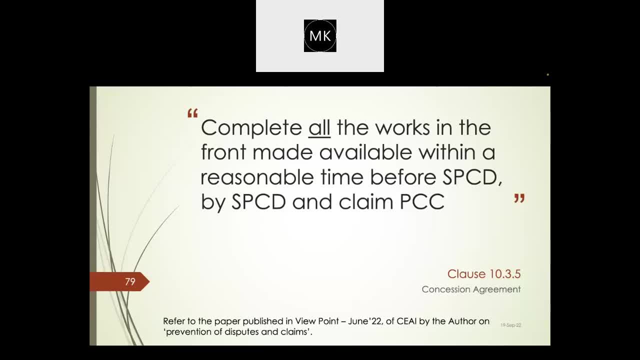 projects in telangana we have given provisional completion certificates 10 years back ourselves. then after 10 years we have come as a own dam consultant on the same project and completion certificate was not given and punch list items were still removed. now we have given a proposal for giving the punch list. 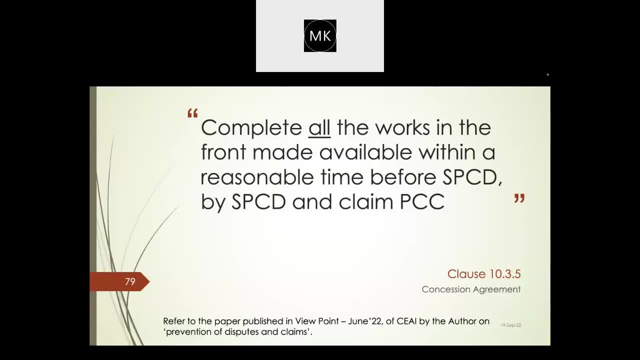 items. meanwhile, all the consultants, they have listed the damages. the damages have been given. the damages are in terms of a few crores, not one, two. it is more than 50 crores, 60 crores, something like that. now the question is: can you really levy damages for so long? 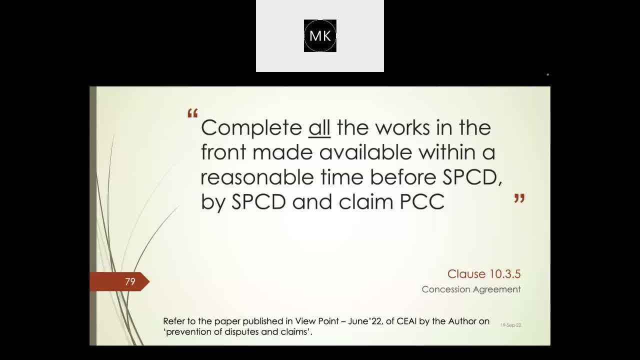 90 to 120 days. 90 plus 120 it is 210 days. so non-completion within 210 days may lead to termination of the concession. Rozido terminating- why did you keep him? you should have terminated. Blazement for lesser pock. we don't get 20 to complete within 200 days because at least 145 day. of his life in a duration may lead to termination of the concession Loading to terminate him. why did you keep him, Lee, anti- breach 100 days to complete it. we don't want nobody to complete it in 12 days to complete this case. why did you keep him? there should Spider wheel door back now because there is constant data saving. 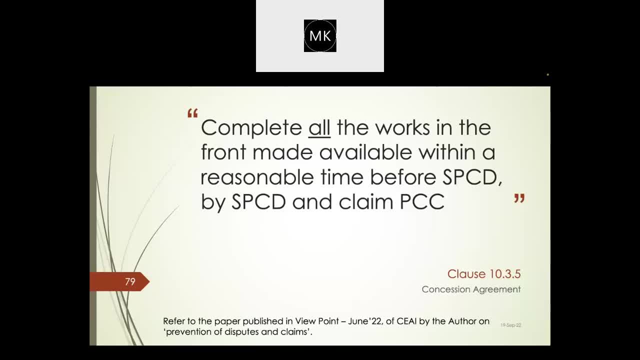 of contribution that is anywhere, because we have to create warehouse. 그것 estavam genau in this paper. the damage is, this is not the same amount, threebacks. We should have terminated, Or at least we should have got it done by a third party. if those things are important, We have not got them done, So it was our own problem. as an authority, I should have either terminated or I should have got them done through a third party. 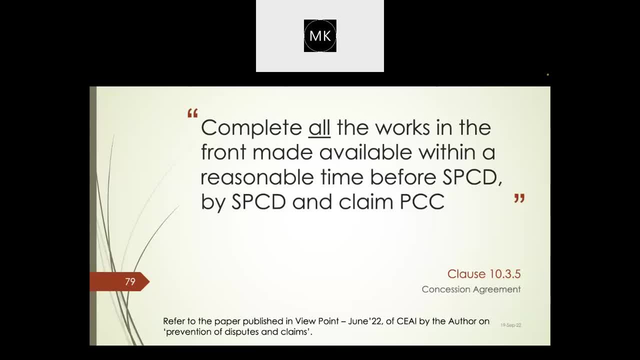 I didn't do anything And I kept on letting punch list damages. To give you a corollary, it's something like the batsman in cricket: he hits the ball and the ball goes out of the stadium, And then the people they are running between the wickets. 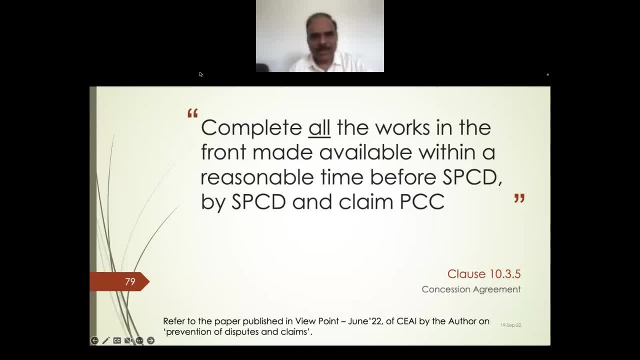 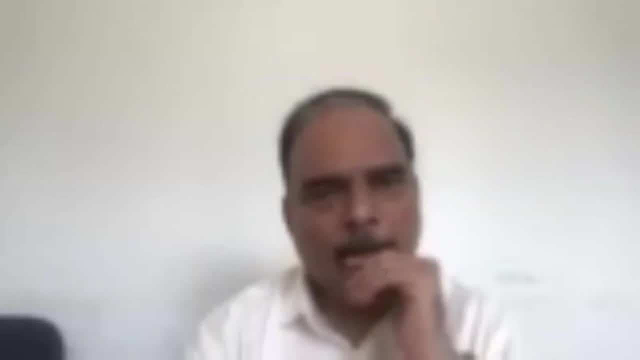 He is not getting the ball, He is running and running. So this is what is the corollary to this: He is not completing, You are not getting him to complete, And then you are still letting damages. So in conciliation I am clearly ready. 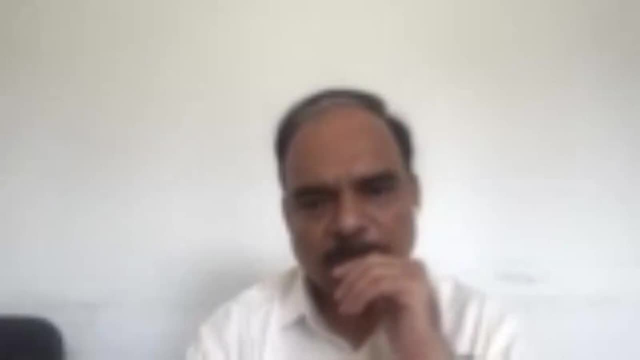 I am recommending to people that you cannot levy damages beyond 120 days. Case of levy of damages eternally: You can't levy damages eternally. Yeah, Time is 12.18.. Financial aspects. Now, let us not think that these financial aspects are not ours. It's very much ours. 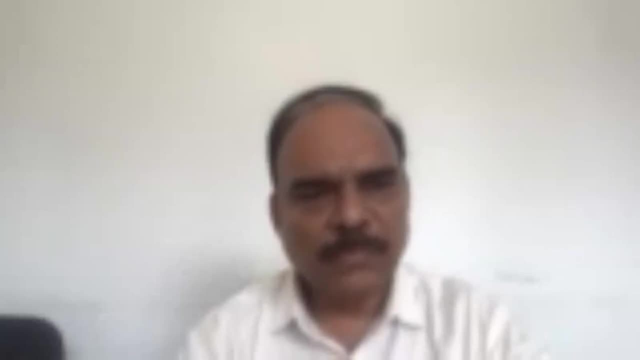 It is important that they open an escrow account And all funds should be routed through escrow account. What kind of funds come? Number one: equity from the parties in the SPV. Equity has to come Debt from the lenders- Lenders directly. put them in the escrow account. 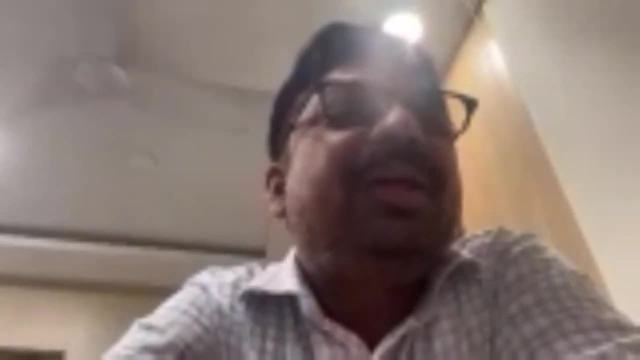 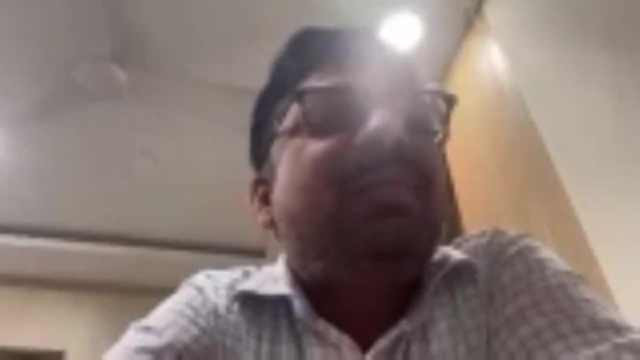 Then there could be a grant that comes from client And there could be a toll. where four-lane to six-lane projects are there, People are allowed to toll them, So toll also comes. So anything that comes into the project should be routed through escrow. 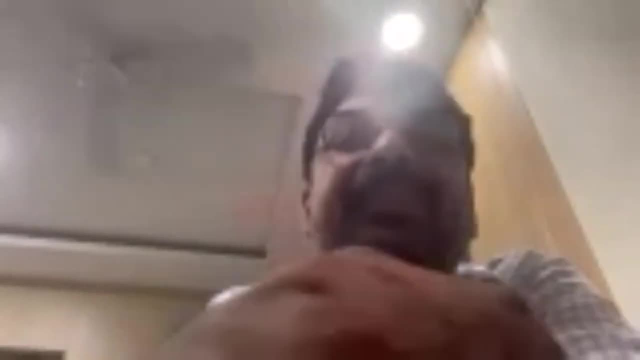 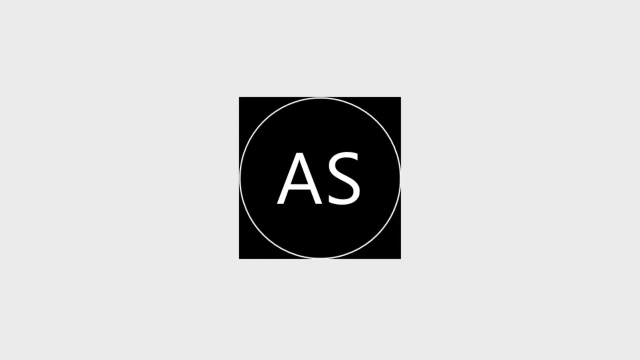 They should be put in escrow only, Otherwise it is called escrow default. If they operate any other account and if the money is put into that account, then it is called escrow default And all the money should be removed from this account only. 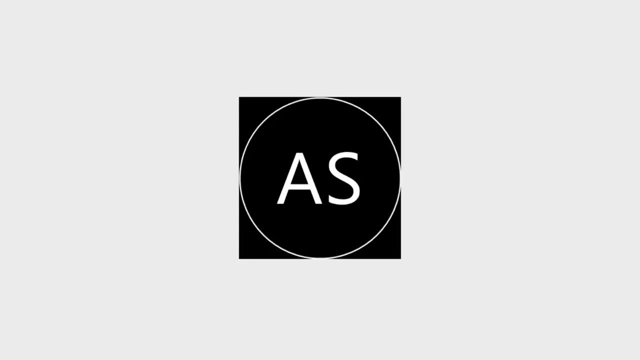 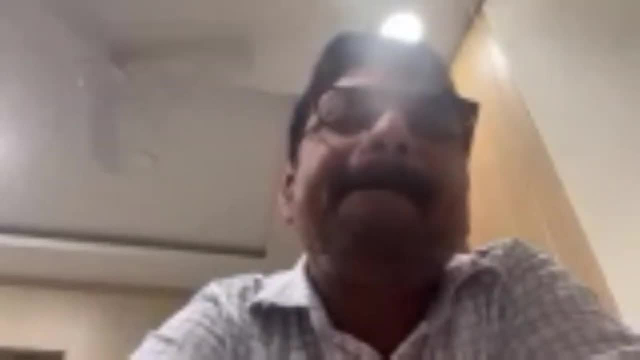 And then they should be put into various sub-accounts. So say they want to pay EPC contractors, There should be EPC sub-account to this escrow account, Taxes, Revenue And in many projects there are more than 15 sub-accounts, so that all the things are properly routed. 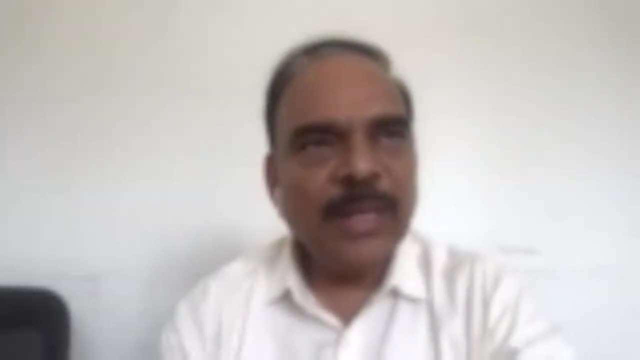 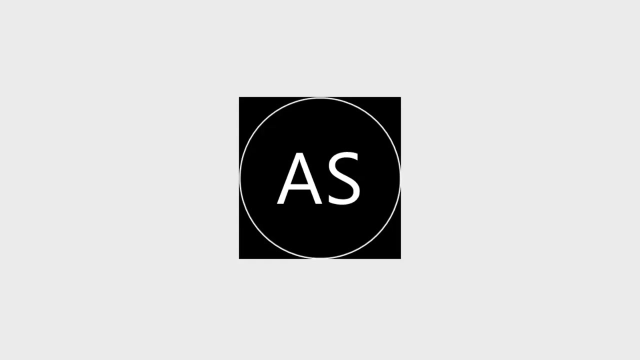 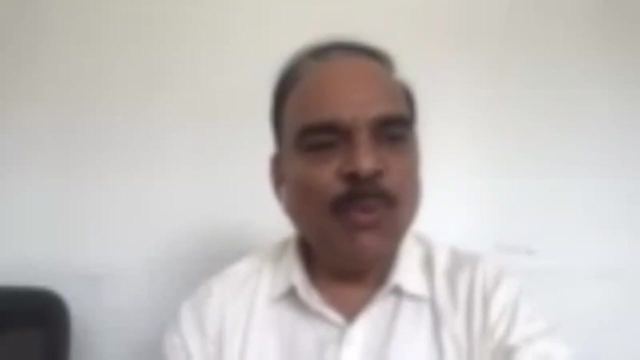 So there can be an O&M account, There can be a maintenance account, There can be maintenance reserve account, So that we clearly identify what is going where. It is not only important for the contractor or concessionaire, It is also important for us to understand how much toll has come till now since PCC or since appointed date. 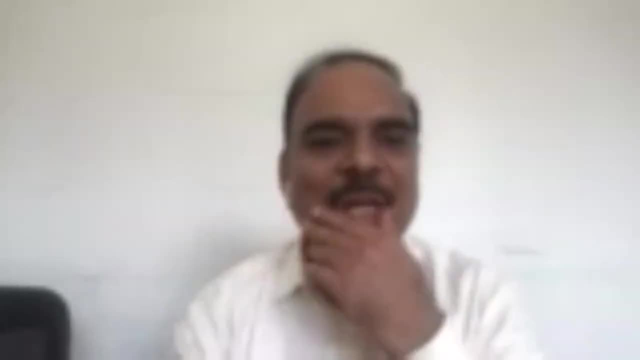 Straight away. open the escrow account of that sub-account of that EPC toll revenue, Then you will understand How much taxes have been paid. Did he pay any taxes or not? You know people even invest. So now it is a question whether these concessionaires can invest their funds, if at all something is remaining. 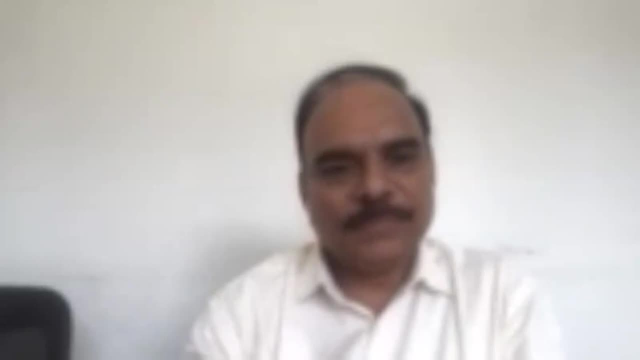 Funds have come From the lenders, But these people are not able to do the construction for whatever reason, Due to the pace of construction or due to non-availability of this thing. So funds are still there. So now they can't park the funds eternally, because they are paying interest to the lenders also. 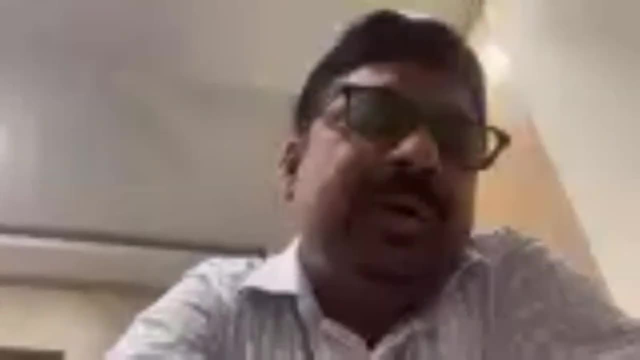 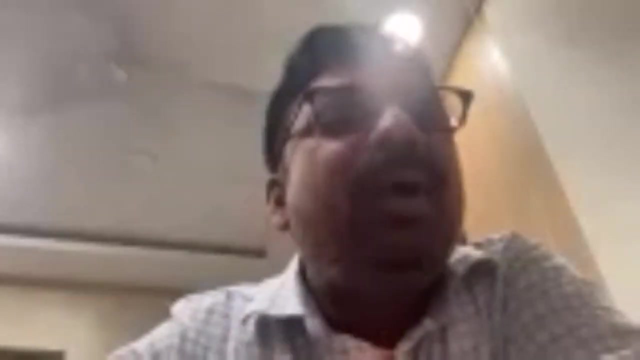 So they can always invest in some place- mutual funds or something- But the auditors come and they say that this fellow is using public money for his own purposes, Whereas in my opinion it is allowed to invest, But project cannot suffer. 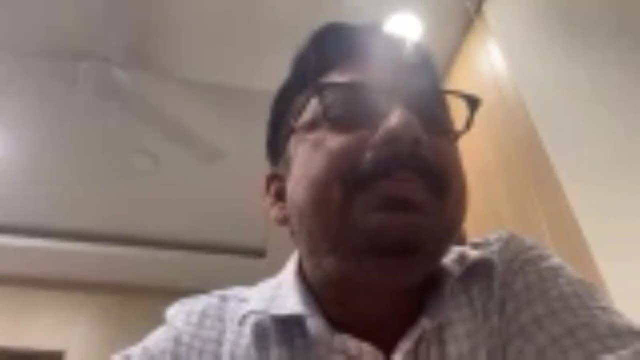 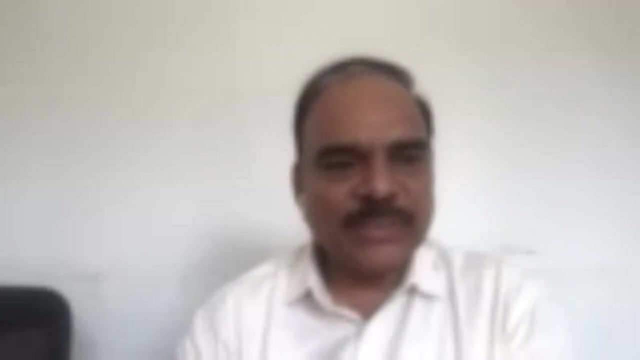 Project cannot suffer. Project should go on. So we have to be cautious about that. So now there is one chance of escrow default. Why it comes, You remember, when they sign the agreement, the development period starts And appointed date will be declared only when the financial closure is done. 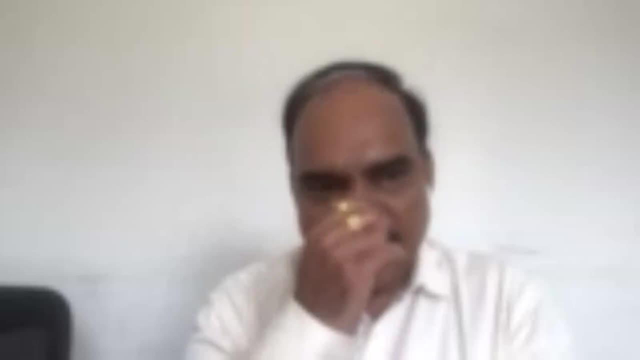 That means escrow account will be opened on appointed date. Within those six months he is supposed to do surveys, He is supposed to do designs And he has to expand many things during that period. Where will he put, Because escrow account will be opened only upon signing the agreement? 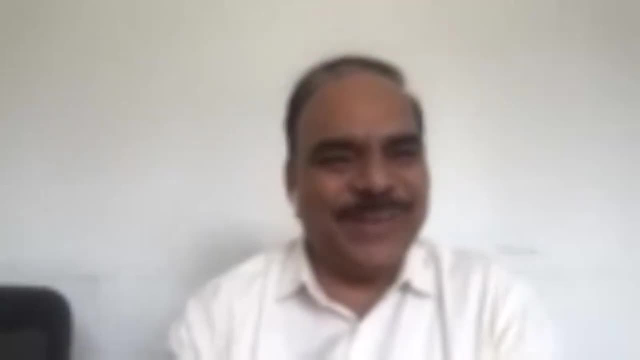 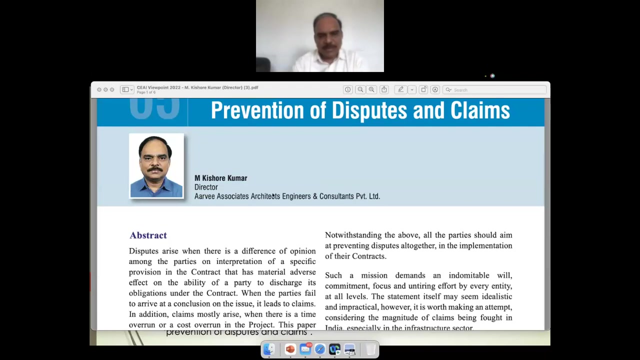 Yeah, Yeah. If we signed sorry, escrow account will be opened only upon financial closure, That is, on appointed date, Then so much of expenditure is happening during the development period. Where will he put it? He is supposed to put money in a different account. 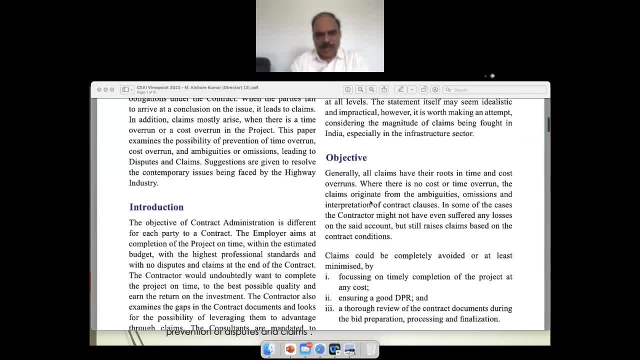 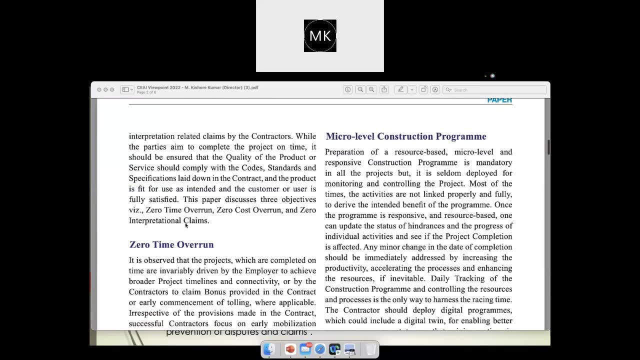 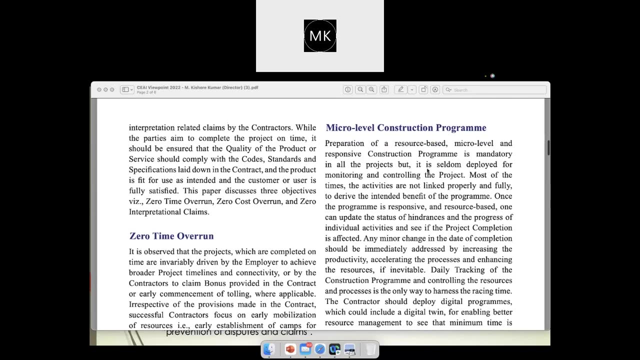 So now, what will happen to that money? So it is always important that the concessionaire chooses the right escrow bank for his first account And he opens the account in that bank And when the appointed date is declared and when the financial closure is done. 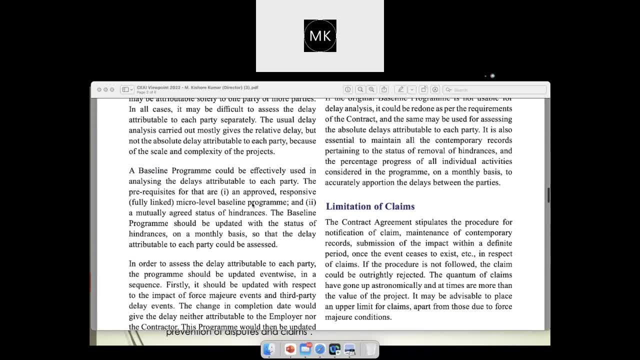 and an escrow account is opened. in fact, this account will be converted into an escrow account So that there is no default. So this planning has to be done. But they don't do planning. They are in fact comfortable having a different account. 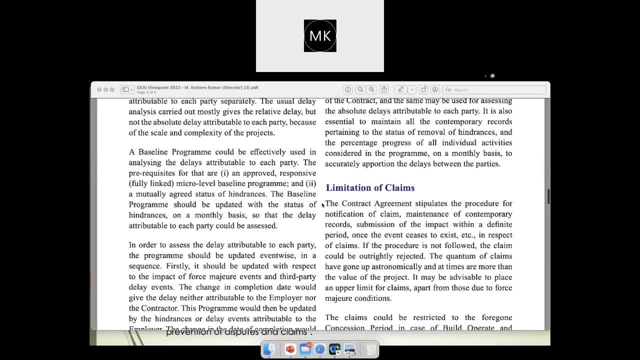 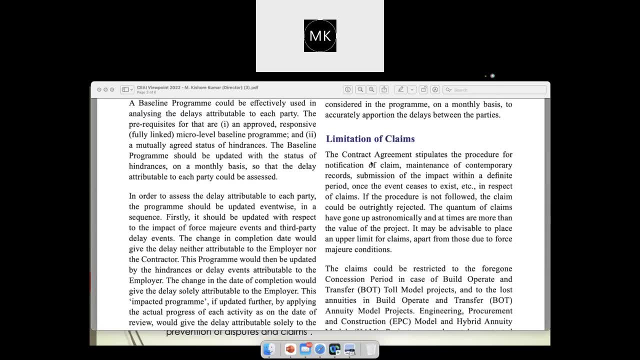 because they can do some funny things. They can withdraw the mobilization advance, They can withdraw many things into that and then route it to somewhere else. Then we have to identify that it is an escrow default And also periodically he is supposed to submit balance sheets. 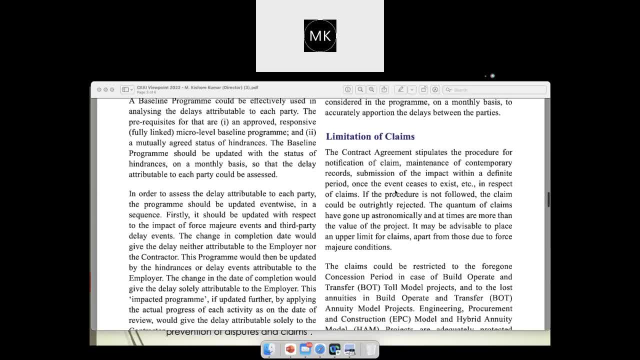 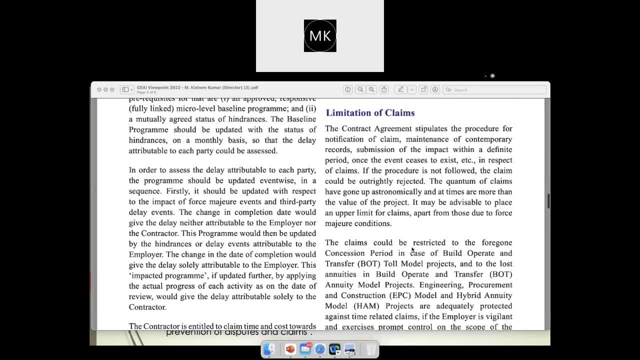 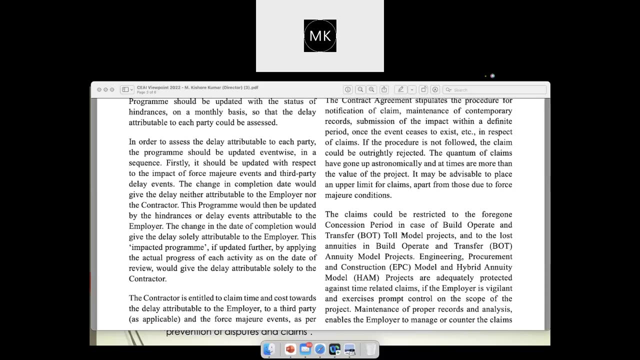 profit and loss account, cash flow statements and statutory certificate. Of course he is supposed to submit every time when he has to prove his percentage Percentage progress, See if this milestone is to be completed. So towards that he is supposed to submit the statutory certificate. 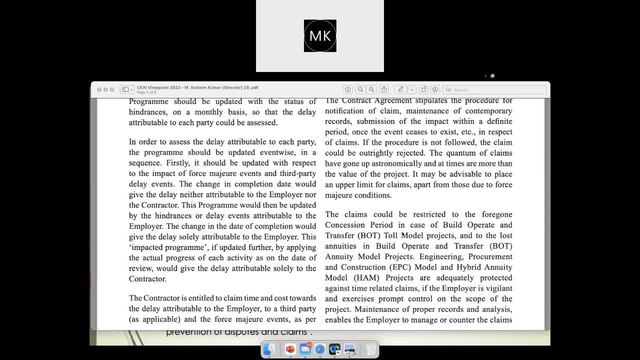 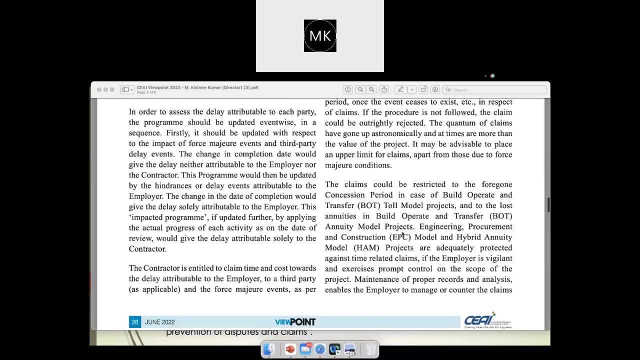 So these are the things, also quarterly, we have to see. You may not understand, but by studying these things I have given escrow default notices to a couple of concessionaires and they were put into a serious situation. So we will be able to identify. 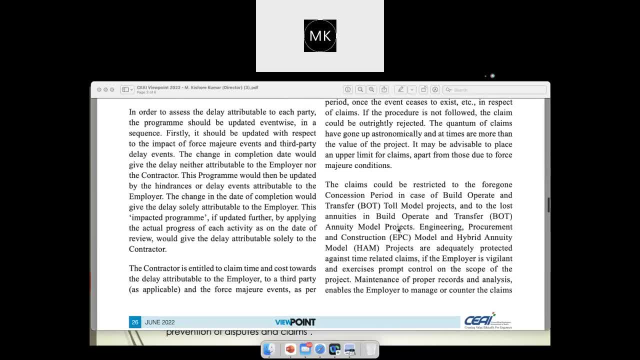 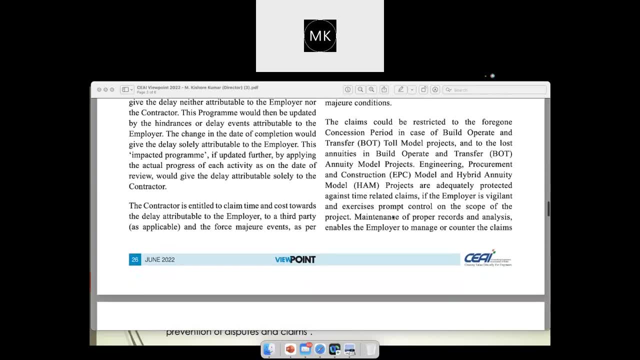 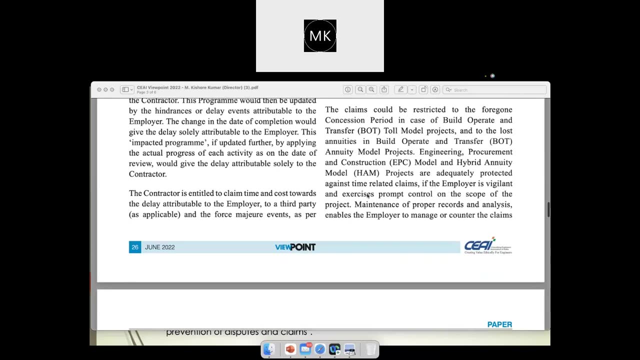 We can watch the advances, We can watch investments and diversion of funds, if any from these statements. Now the claims- And this is mainly prevention of claims: Time overrun, cost overrun. These are the primary reasons because when there is a delay in completion, 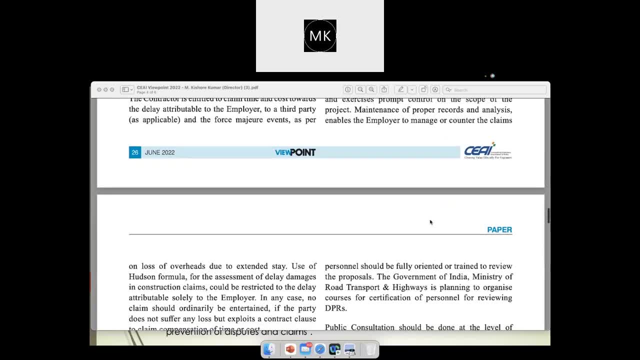 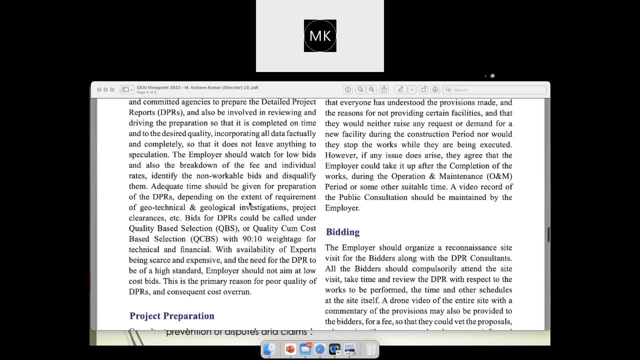 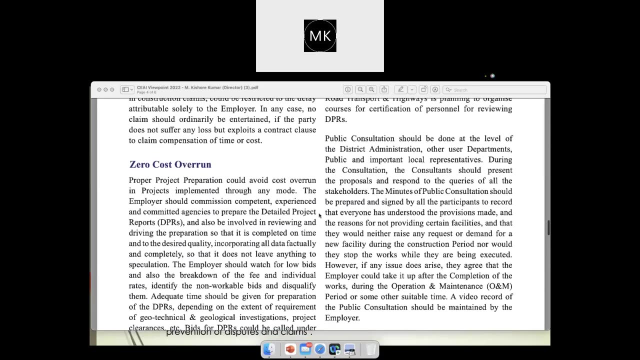 there will be a time overrun. When there is an increase in cost, there is a cost overrun and they result into claims. Best method is to avoid claims. Now there are three slides over here. We have to freeze the scope at the time of commencement. 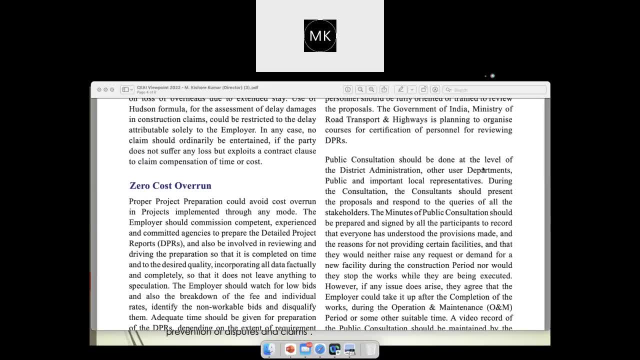 If all the parties single-mindedly work on freezing the scope of work at the time of commencement and completing the work on time, then most of the time related claims would be avoided. If you remember, I was telling you that up to 80 plus 180, whatever is given. 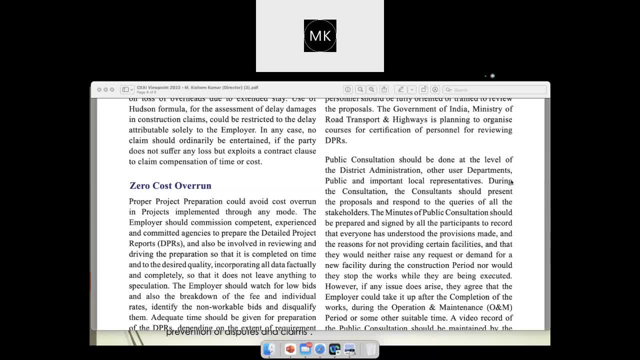 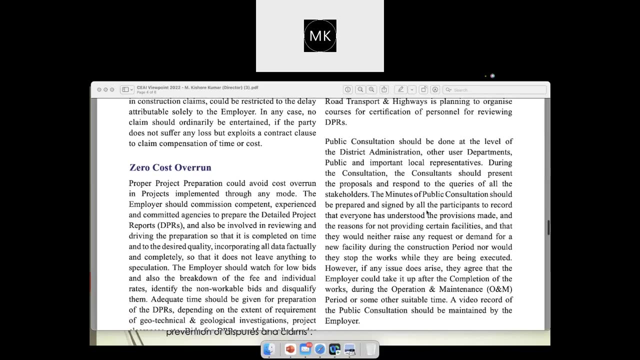 that is agreed as scope. after that rest of the time rest of the items or works are either de-scoped or de-linked for completion. Then he has to complete these things in time by SPCD. He cannot claim anything The moment it is abstracted. 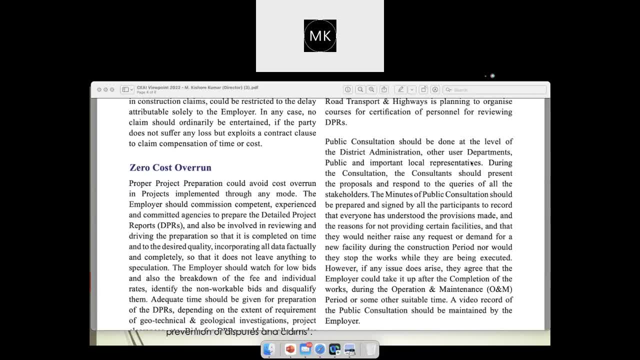 or the moment it is not handed over, it is already either de-scoped or de-linked, So there will not be any time related claim on this. Now, when you come to cost related, this is very important. I have put certain things in one of my paper. 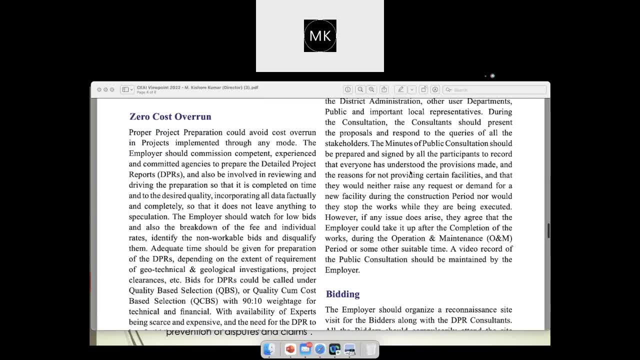 I have asked the organizers to give a PDF of that paper to all the people in this group. Please go through the paper for cost related claims. how to handle the DPR. I tried to put something there and if you can do it, kindly do it at your own level. 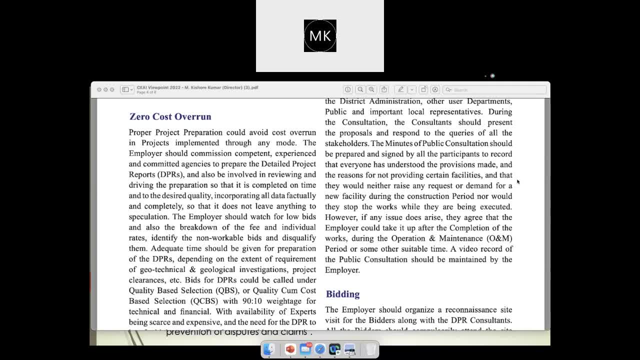 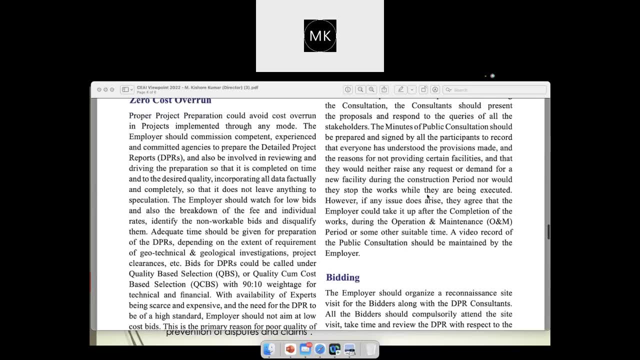 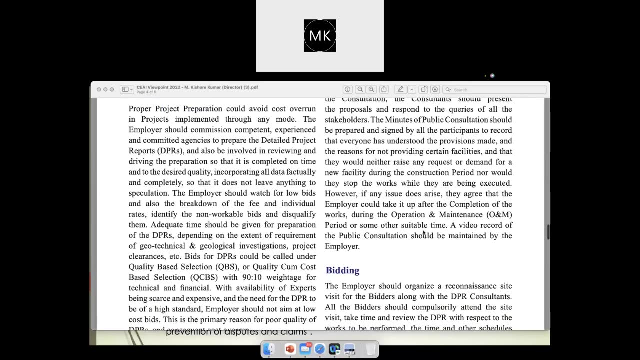 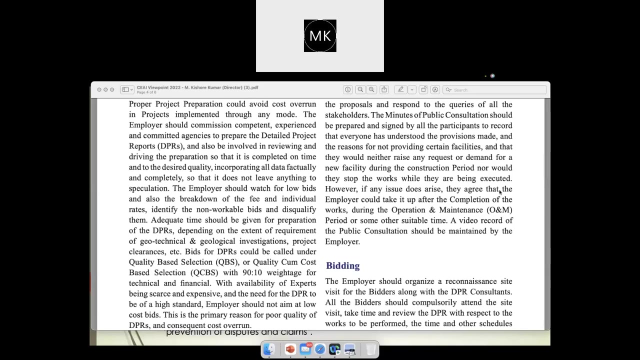 instead of waiting for a policy for that, then it can be done. So if the employer, DPR, consultants and bidders, and finally successful bidder, in that order, focus on achieving absolute clarity in the scope of work, there should not be any ambiguity and omission in the contract documents. 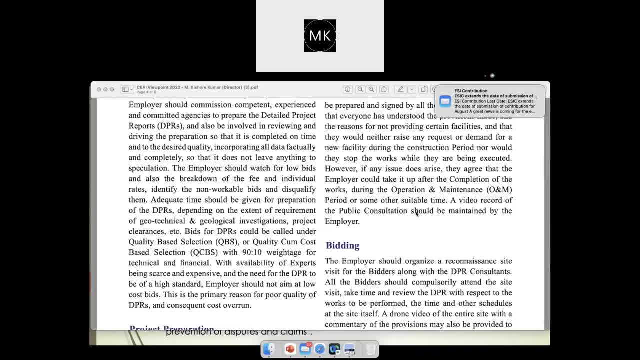 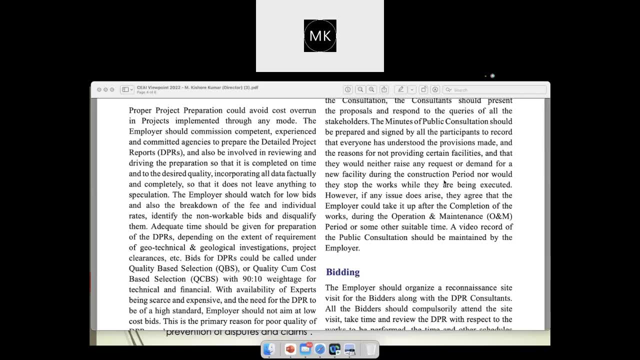 before signing the contract. We are always in a hurry to sign the contract and you know some reasons. somebody might be after us, so we have to sign the contract. We don't give clear replies to the pre-bid queries. we always say as per RFP. 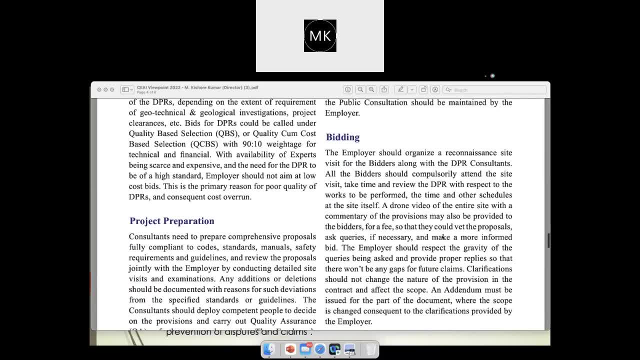 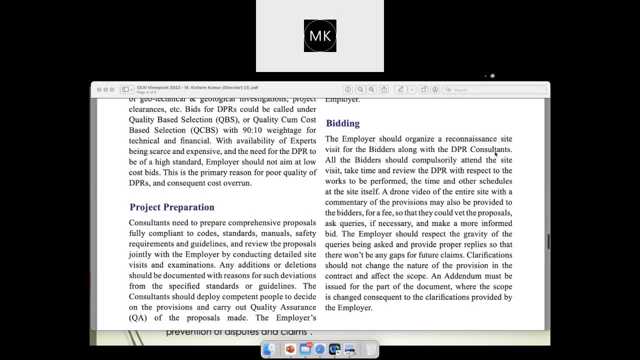 because if we want to give something, either it has to be approved by the committee, or sometimes it may have to go to the ministry, or sometimes it may have to go even above the ministry. So we are worried. But if you spend time there, 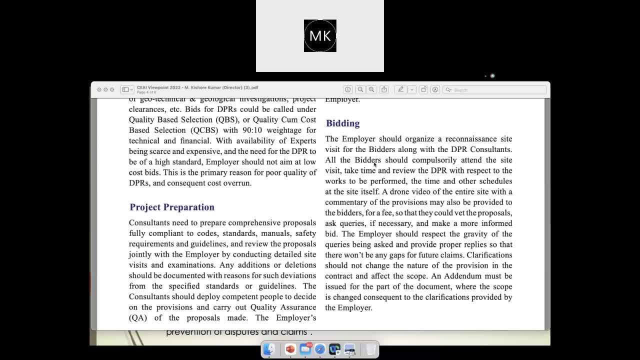 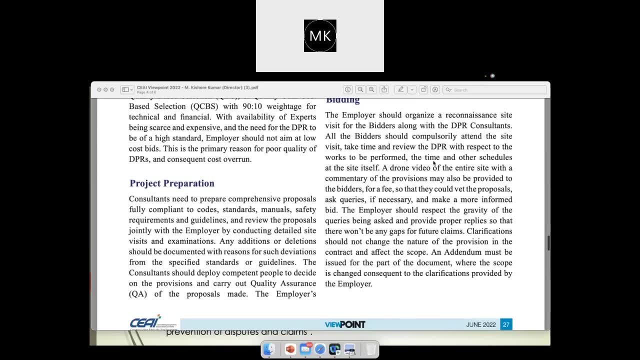 then certain problems can be sorted out once for all. So pre-bid queries have to be properly handled. I have more suggestions. In fact, if time permits, we will go over the paper and I will tell you what exactly I have presented over there. 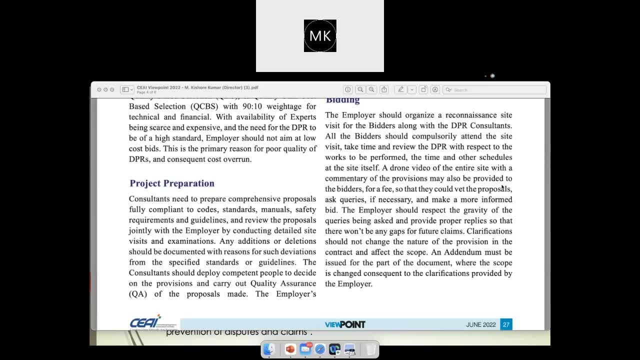 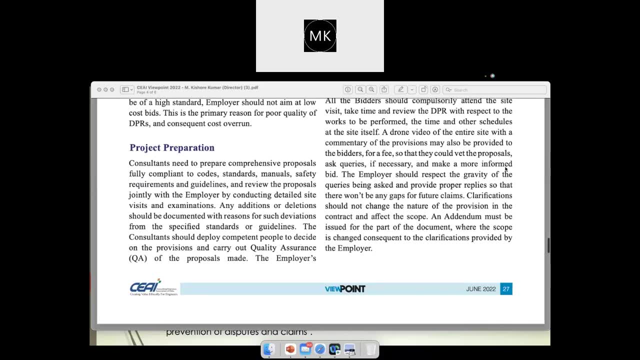 And, end of the day, before signing the contract, the contractor sits, stays for three days, four days, and studies all the documents and he compares the whole thing with a drone video. In fact, I suggest that a drone video should be given with commentary. 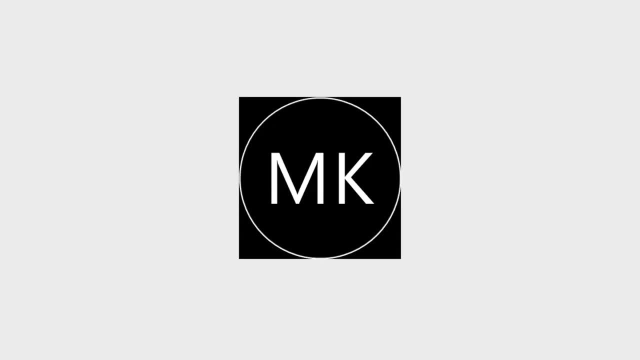 to the bidders. It should be available in the website So they can go over the drone video and comments are being given that here it is widened to the left side, here it is widened to the right side and here VUP is provided, and here we were supposed to provide. 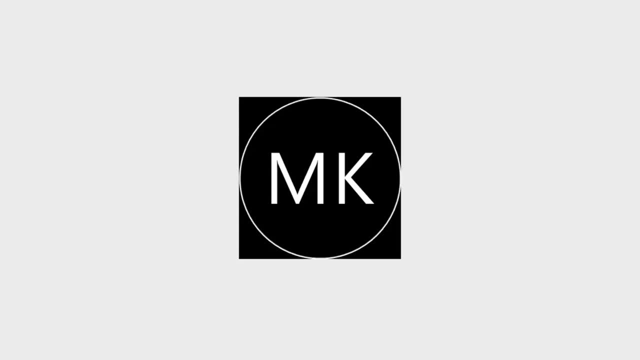 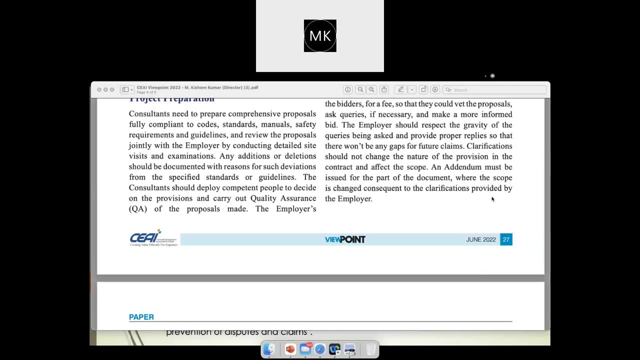 a VUP, but people have objected, So we are not giving the VUP, because that is also important Tomorrow. if there is a public representation, then we should know why it was not provided. We should not write a letter to DPR consultant as to why he has missed out. 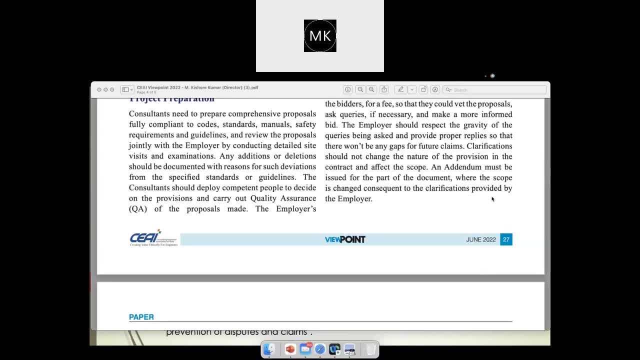 and we will take action. show cause all that. Instead of that, we should know why certain thing is not provided, And he may- actually he means the sense DPR consultant. he should give certain comments. commentary Commentary along with the drone video. 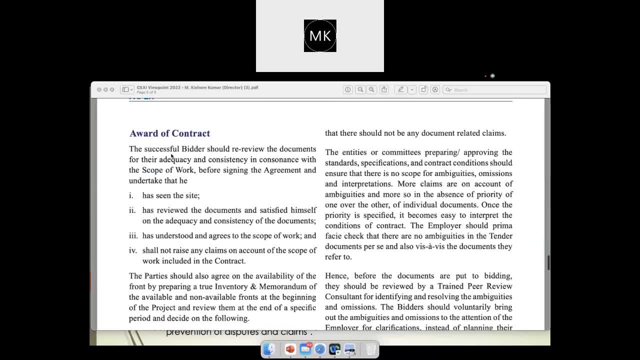 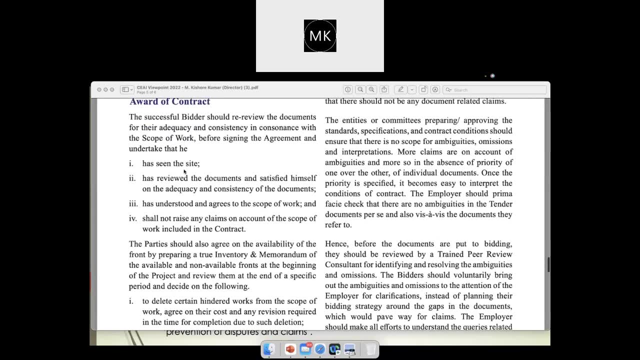 and the bidders can go over it over and over again and find out whether things are in order, whether the scope is clear to him, And before the bid date itself the scope is clear, And before signing of the contract. he does all these things. 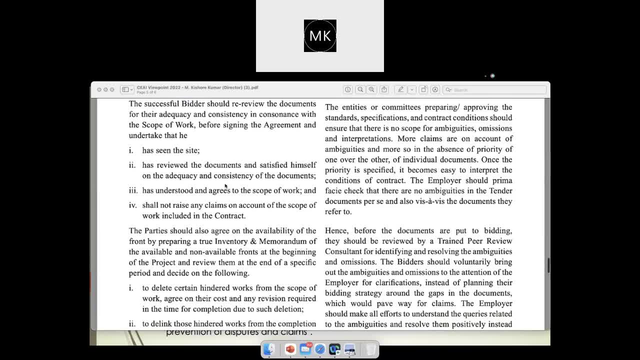 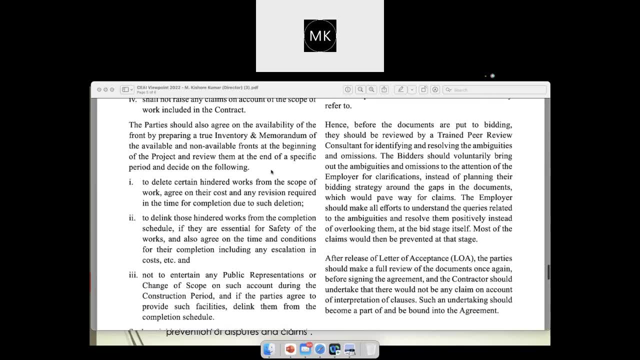 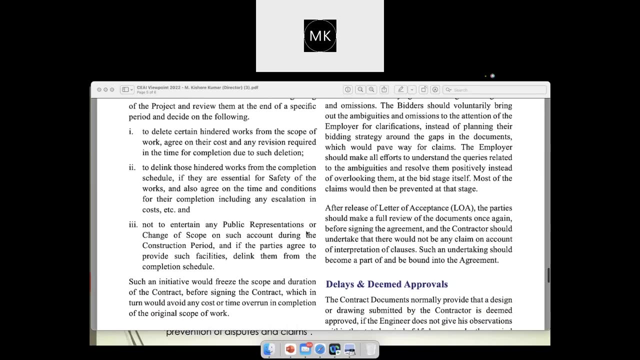 and says: I am not. I understand the scope and I am not going to raise any claim on you for the scope written in this contract. If he does that, he will not raise any cost related claim. The third one is document related claims. 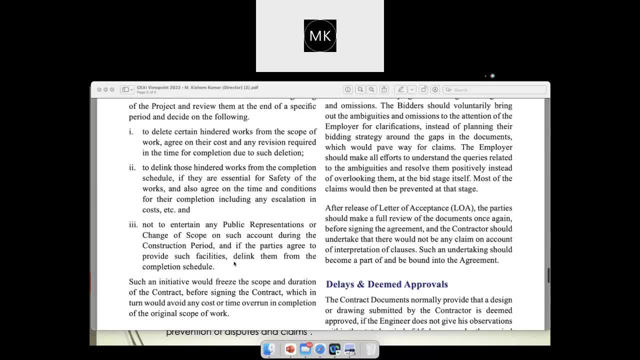 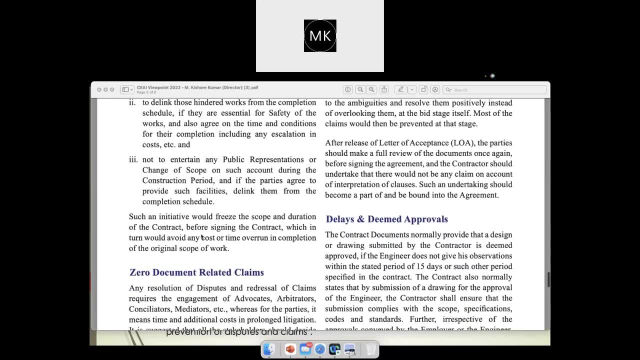 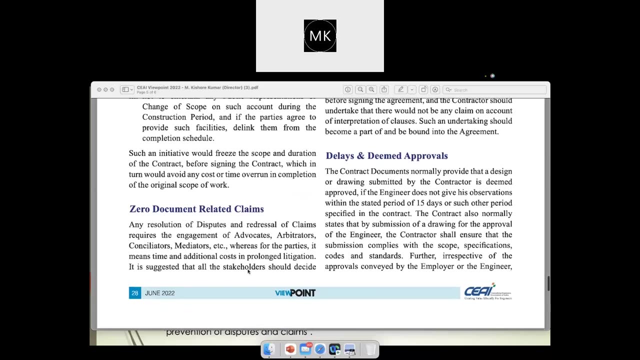 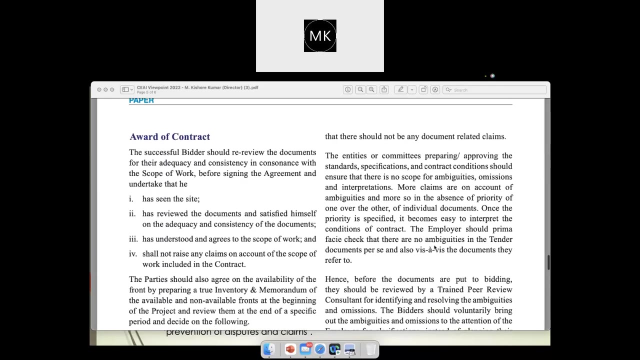 You know there are certain grey areas in the contract. Those grey areas, even though contractor knows he does not tell us, He keeps it with them so that he would exploit those gaps and then claim So if the parties decide not to exploit the gaps in the document. 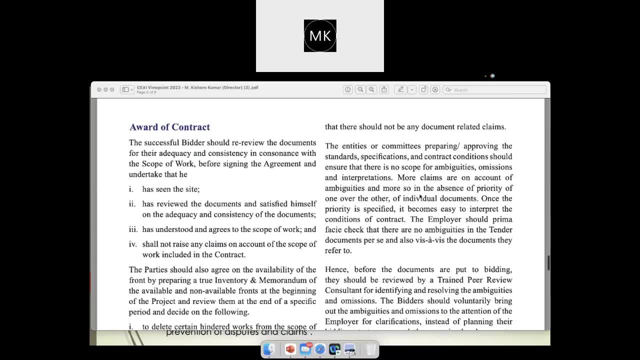 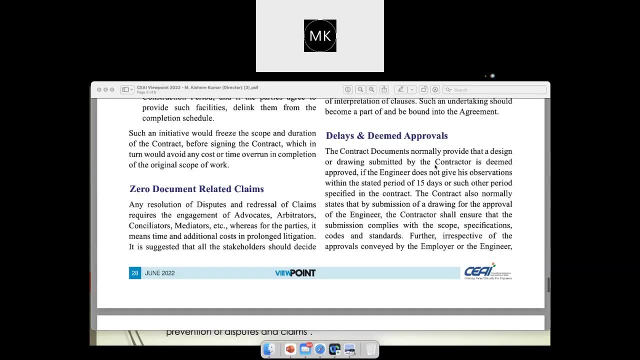 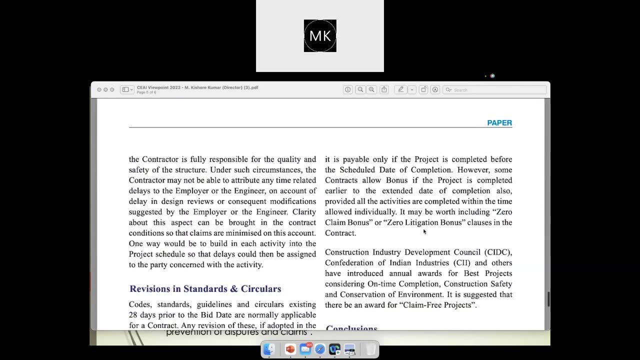 more so when they do not suffer any loss- they don't suffer any loss, but still they want to exploit the gaps- then interpretation claims also could be minimized. In fact these things should be handled even before signing the contract. But if something is still left out, 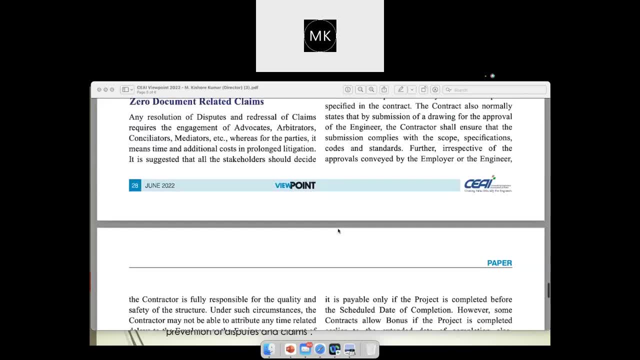 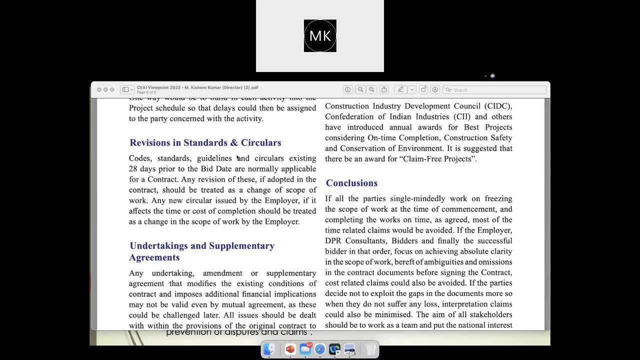 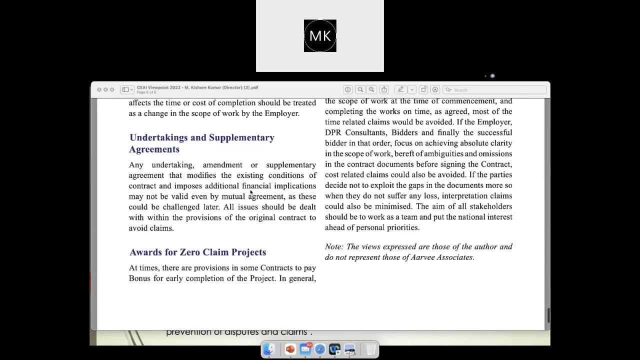 that should be minimized. So the aim of all the stakeholders should be to work as a team and put the national interest ahead of personal priorities, And gaps should be identified and ironed out before signing of the agreement itself. So this is. 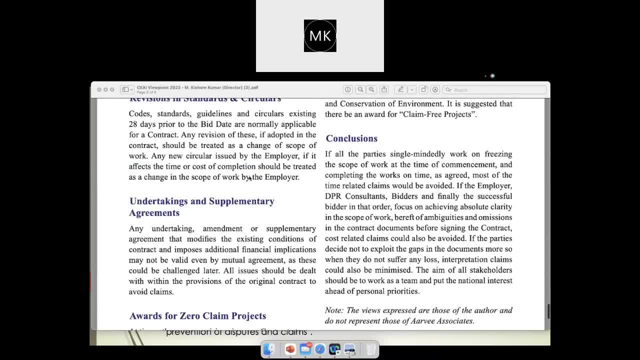 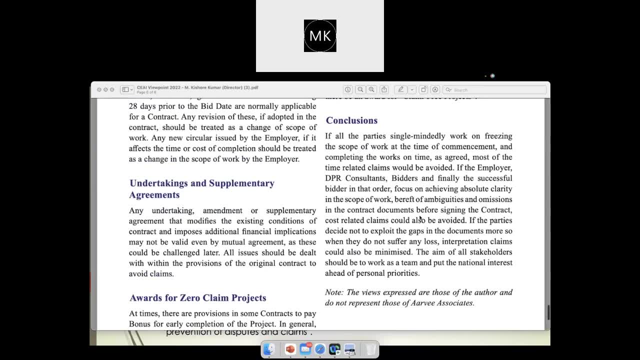 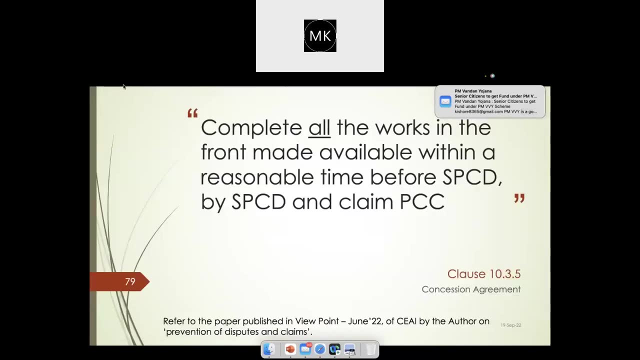 with this, I think we will be able to prevent the document related claims also. So the clue is simple: Complete all the works with the front made available within a reasonable time before SPCD, In the sense six months before SPCD. 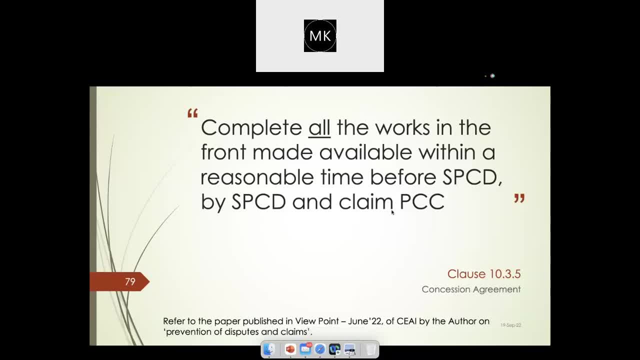 we have given certain works, not only AD plus 180.. Beyond AD plus 180, also six months before SPCD, certain front was made available to him. If the contractor completes them by SPCD and he claims PCC, whether you are able to put it on commercial operations or not, 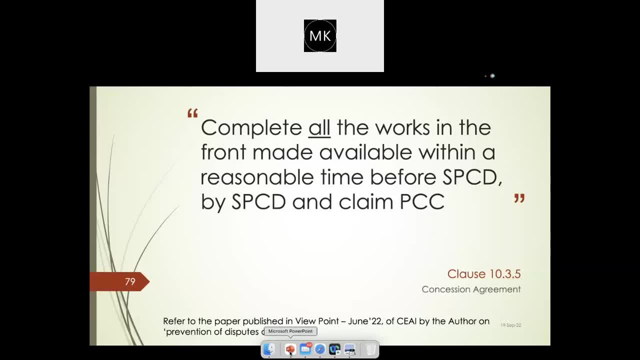 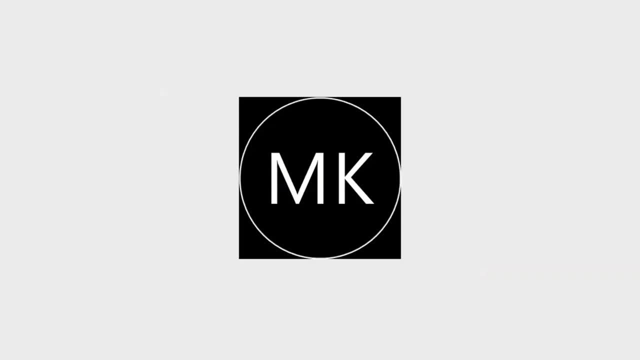 if he does that, there will not be any contractual issue because his annuities will be intact. Now in Tamil Nadu there is one project: 45 kilometers out of 50 kilometers is greenfield And there are many problems in the greenfield. 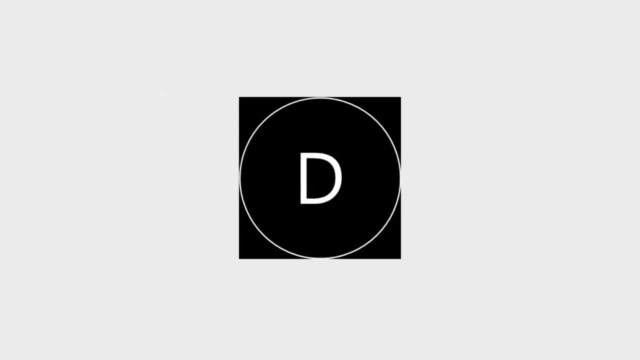 The contractor is planning to complete everything except the gaps in that 45 kilometers. So even after that traffic will not be able to use that greenfield. But we have to give PCC to him and make him eligible for claiming annuities. 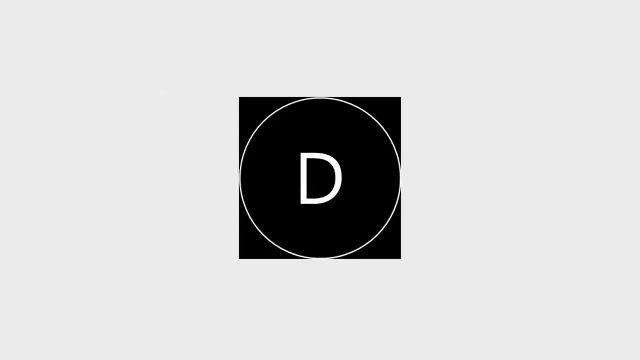 Then only contract related problems will not be there, Right? So we have to just watch the date. When is SPCD and all In the other program where actually I personally give training in IAHE? there I give at least. 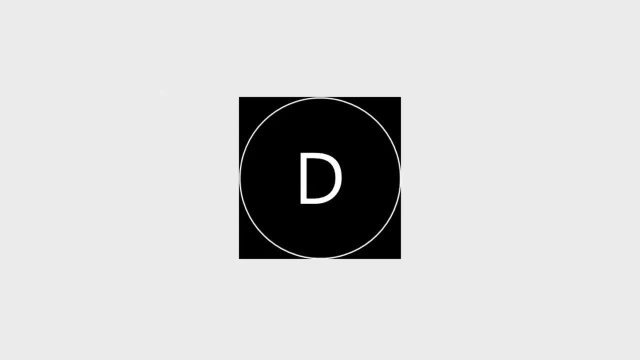 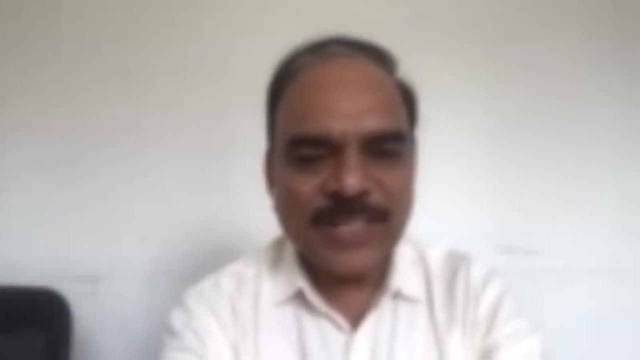 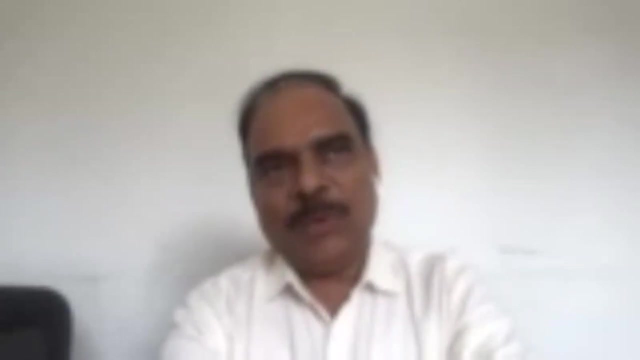 10-15 case studies In one of the projects. those people have written the date of completion at every place: In canteens, in offices, on the road, everywhere they have written and they have marked it as NISJM. 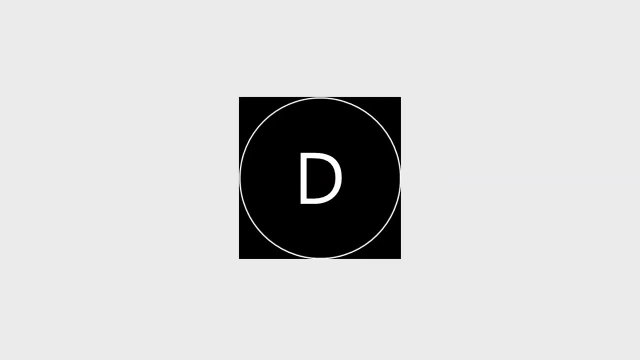 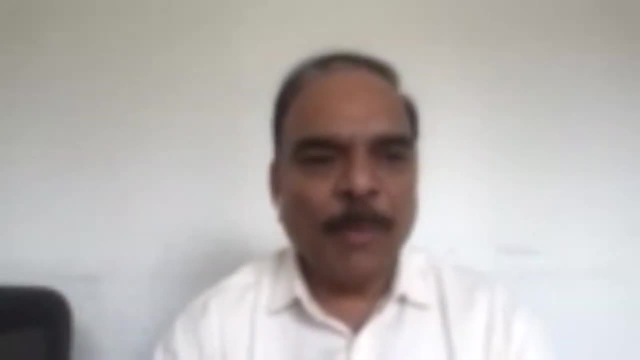 I mean, we have decided that we are going to complete this on this date. They have written this on commencement date And they have completed the project 100 days ahead of that NISJM. So once we decide that we will be completing on that date, 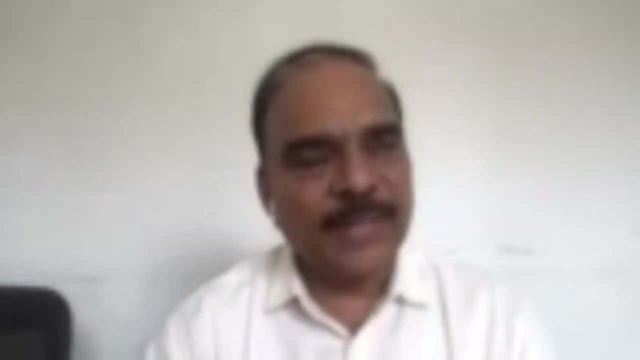 everybody will means all energies will flow towards that. Similarly, I know another contractor who actually floods the site with equipment, with materials, with resources during the development period itself. He knows that he is going to achieve the financial goals and he is going to commence the project. 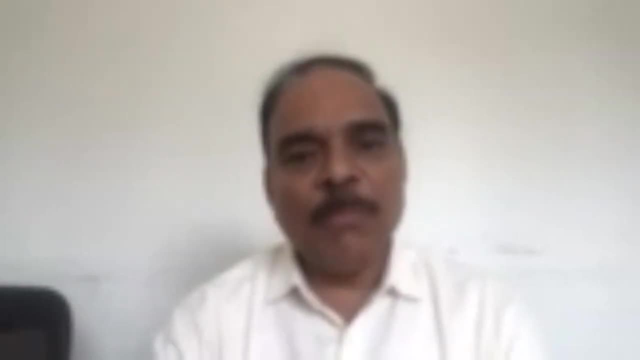 on appointed date. He knows everything. So during the development period itself he will make everything ready. I know another contractor who does the designs even before signing of the agreement. I don't know how he knows The moment he is declared as a. 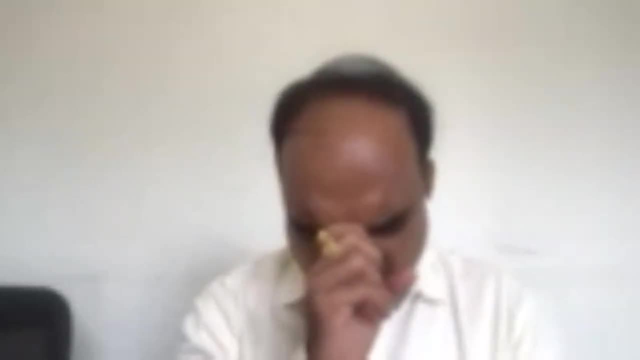 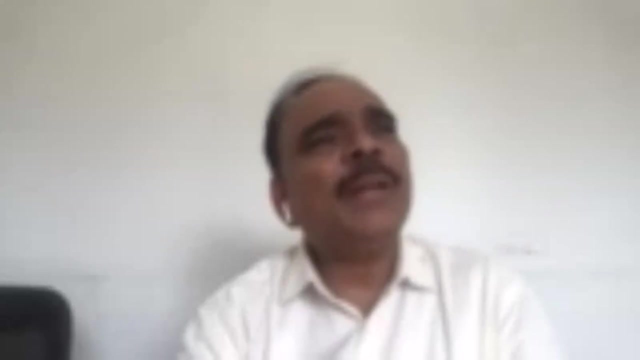 least I mean lowest bidder. he starts the designs: AE is not there, IE is not there, nobody is there. And he also commences works during the development, during the development period, And he is far ahead when the appointed date is signed. 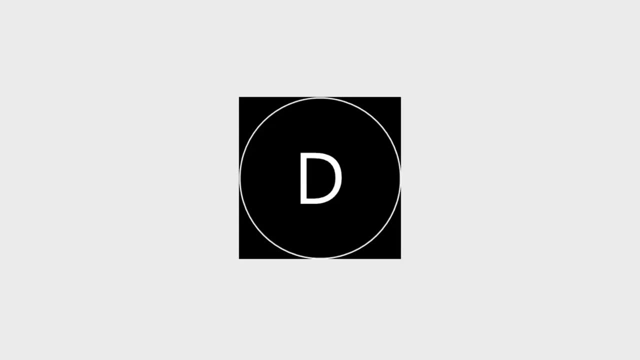 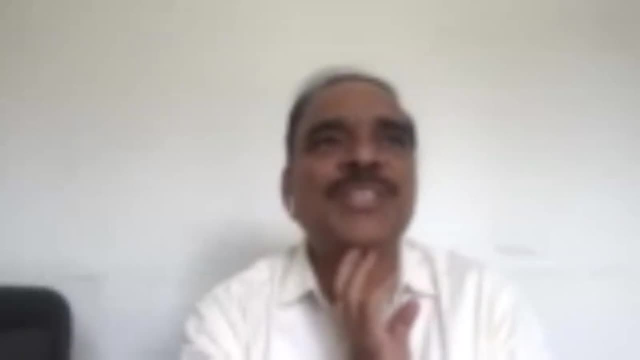 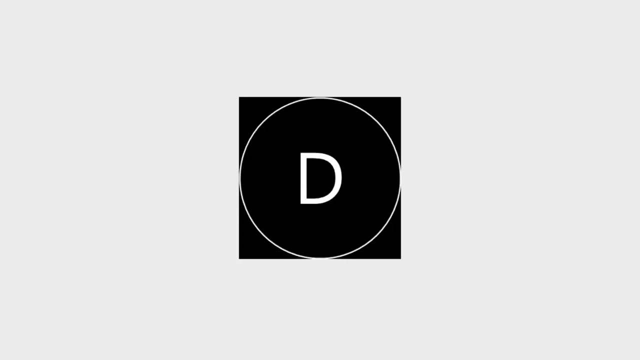 I don't know whether it is legally correct or not, But those people have completed the project one year ahead of schedule- One year, And they almost claimed 50 crores of bonus. It took time to clear that bonus, But after all the 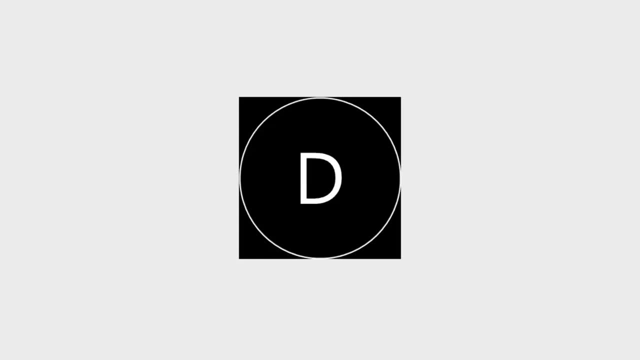 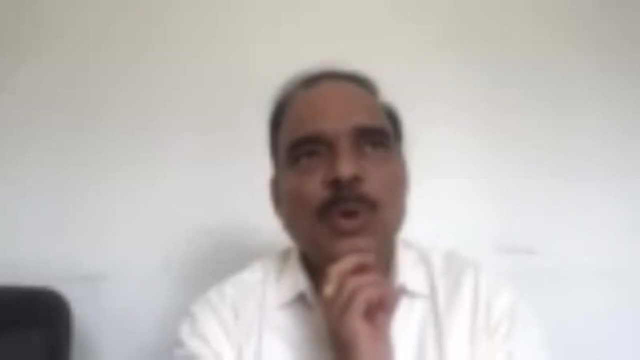 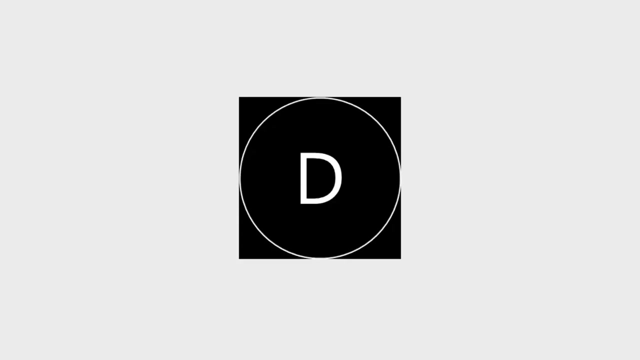 scrutiny and all that. that bonus was paid. And the other project person? he has completed eight months ahead of schedule And he commenced tolling, So it is basically the contractor. What are we supposed to do? We are supposed to only give. 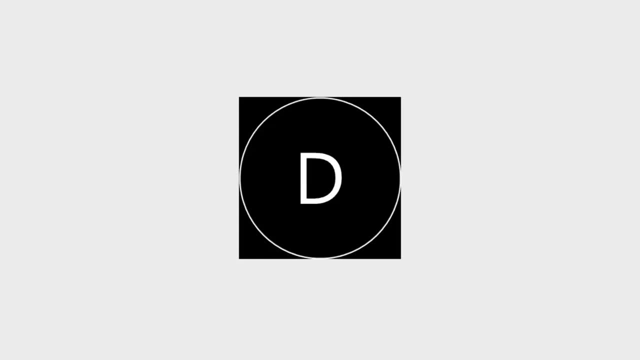 clearances decisions. And we should not stop him. We should not try to twist the arms. Some of the clients means they are very less in number. They don't want to give clearances, They don't want to pay on time. 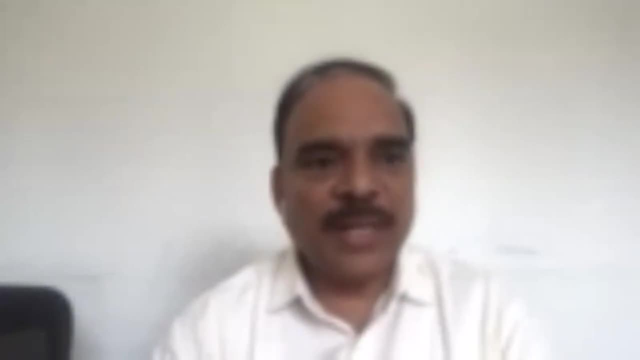 They will twist the arms In the sense, if you want payment, then you have to do this work, You have to do that work, It is okay. It is project work only. But why? So we have to be with the contractor? 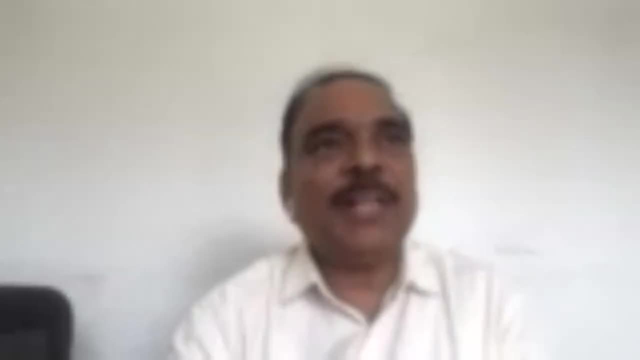 We have to be with the consultant And to see that things are done within the time. So more or less I have completed. It is 12.35.. It depends on how people. people want to post questions. now I will open it for questions. 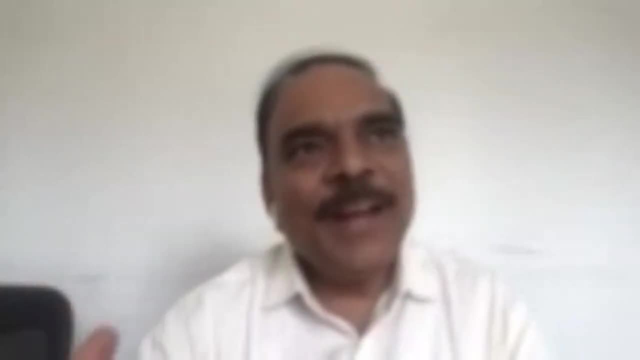 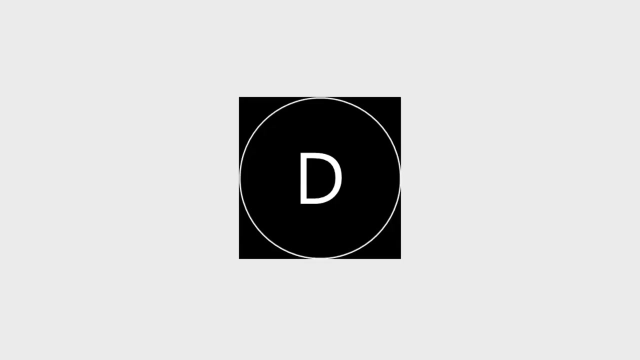 Thank you, Any questions? Hello, Yes, we already did some questions. It is, I believe, the last question. We will now get the questions from the audience. Did we get the questions? Yes, we did. The question is: 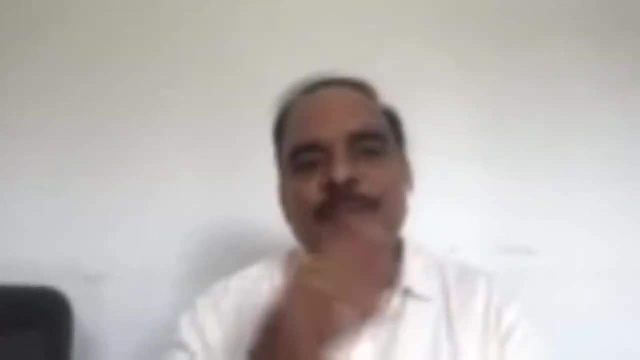 did we get the questions from the audience? Were they correct? Yes, they did. Yes, There was an initial question a few minutes ago. Oh, you know, I was looking at the information, Sir. you told that minimum basis will be considered as change in law as per some direction of. 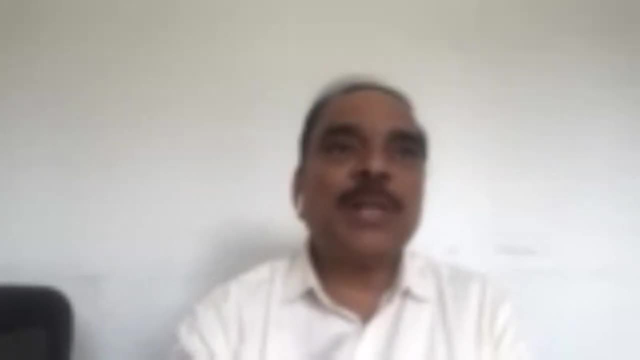 court. We already have a speculation formulas in our EPC and other contracts, So how it can can be accommodated in other items. Concessionaire may also demand for change. Your voice is not audible, sir. I'm so sorry. See, I have not told that, I am admitting it. I have only told that the 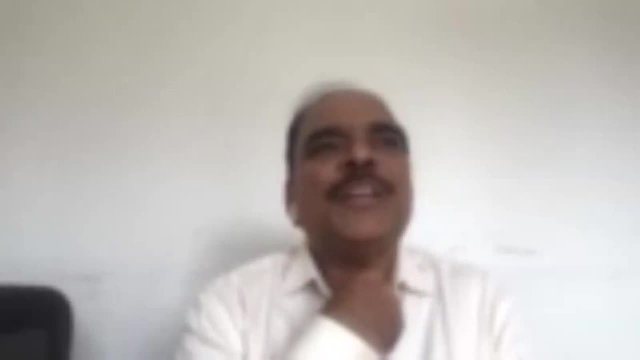 court's verdict should be explicit. It should state that minimum wages increasing minimum wages changes shall be changed in law. It should be so explicit. There should not be any scope for interpretation while reading the Supreme Court verdicts or judgments. That is what. 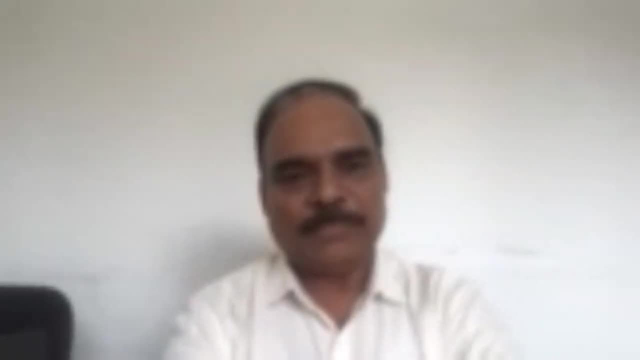 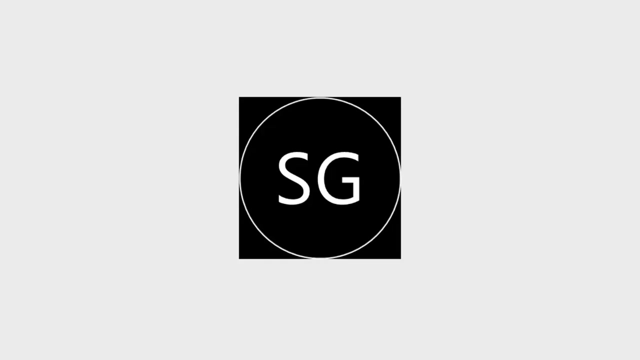 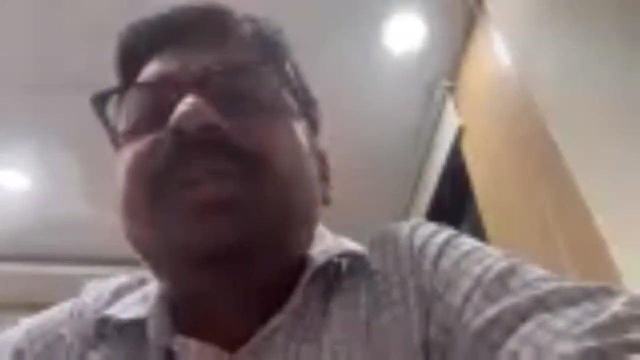 I have told, So I am not admitting it. It is in case of this thing, See, because anyway, go for more questions. Then I will deal one important aspect of prolongation damages, or what is that Prolongation claims. I will discuss on that. 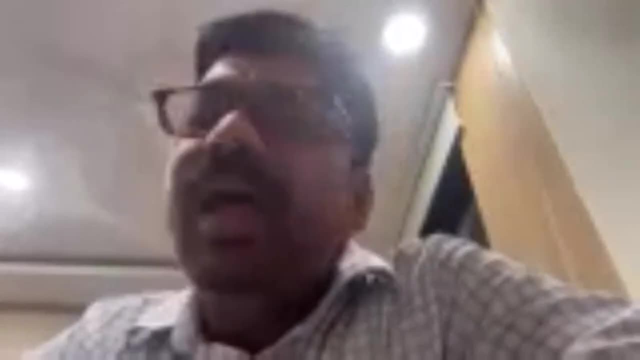 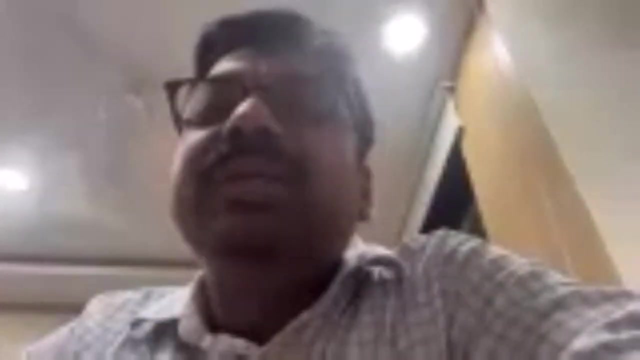 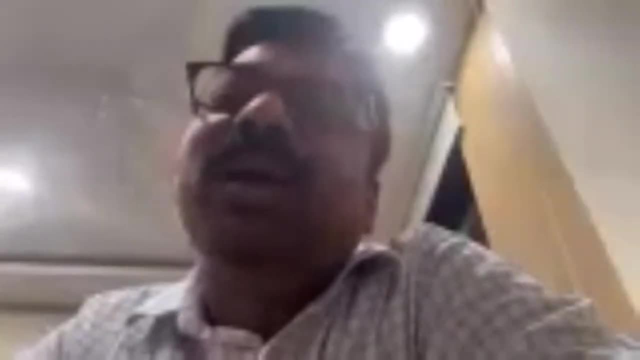 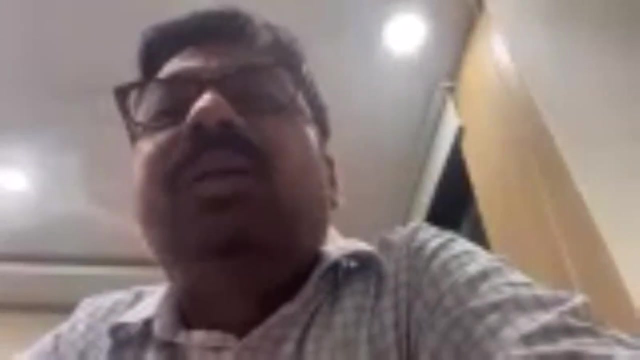 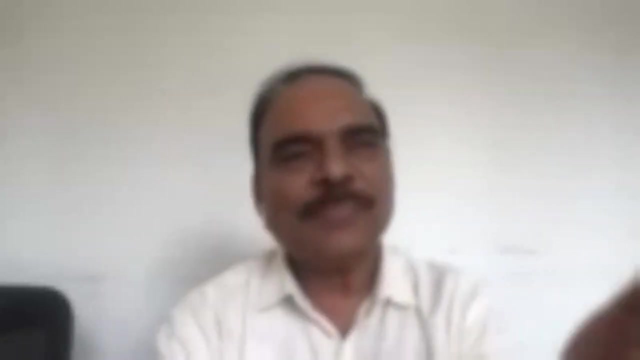 that part only which has not been given uh after 90 days of 80, 80, yeah, so what? what i wanted to say there was only in epc contract we have uh extension of time for the affected works, whereas in ham it is not written like that. it is for the whole of the project. that is what i meant. 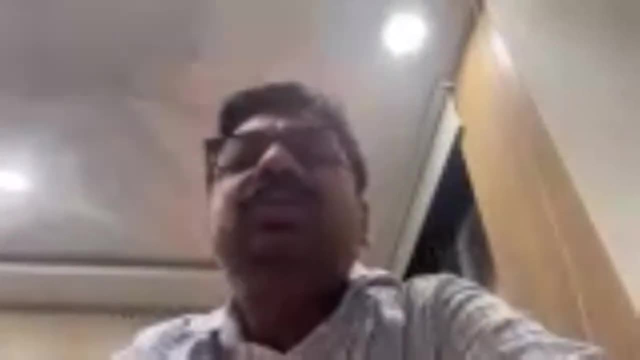 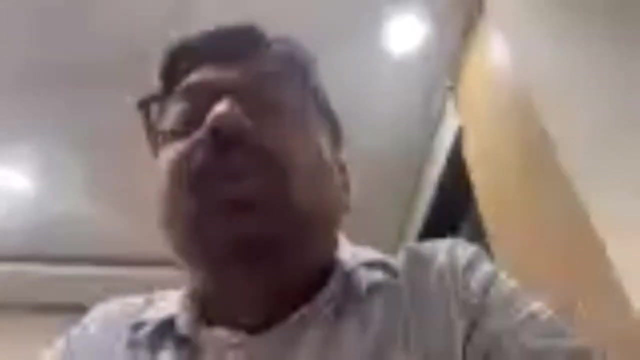 by saying globally ot, it is for the entire project. whenever we are giving only in epc it is for affected works and in other type of projects it is becoming global. but if you understand what i said about de-scoping and de-linking and all, there is no question of uot. 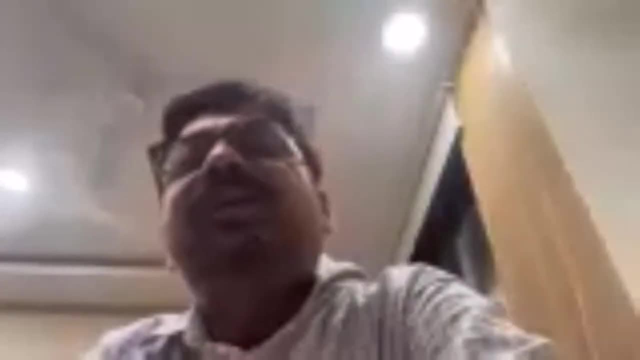 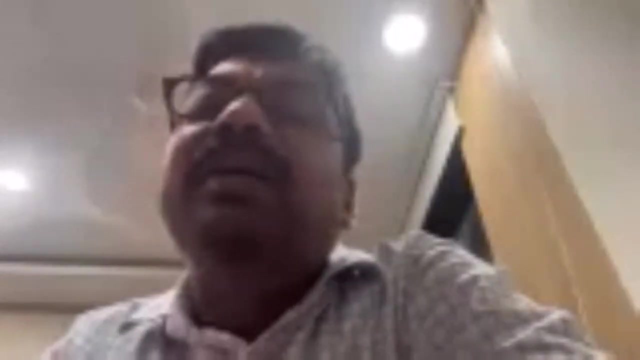 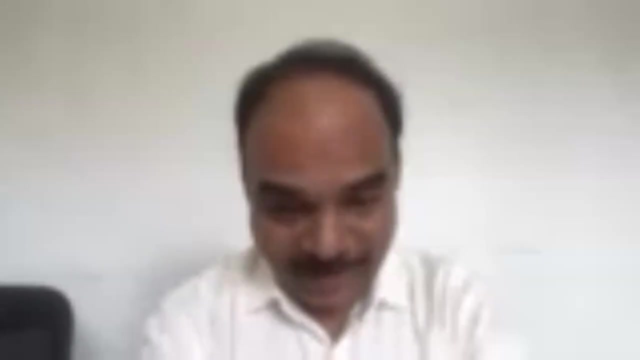 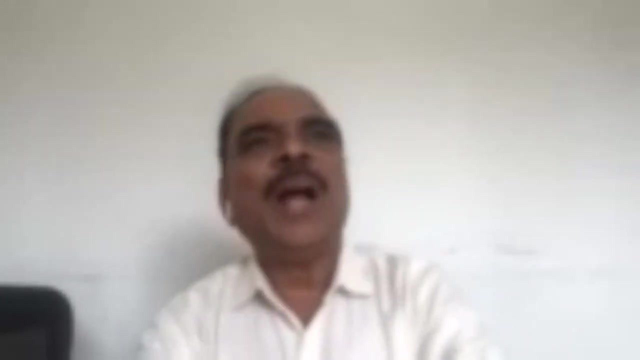 for whole of the project. in fact, many clients, they are telling me there is no question of uot for a ham project. i am not going to give and uh, okay, i. i will take you through the paper which i have published in one of the magazine here: 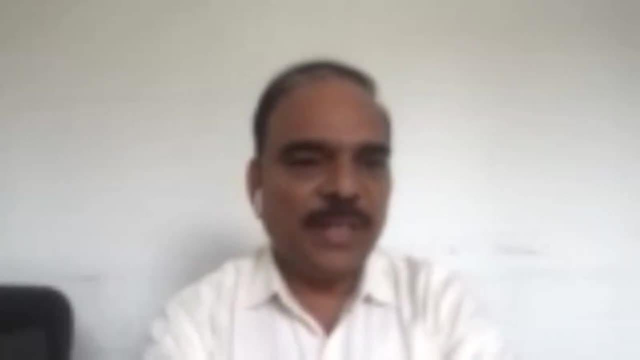 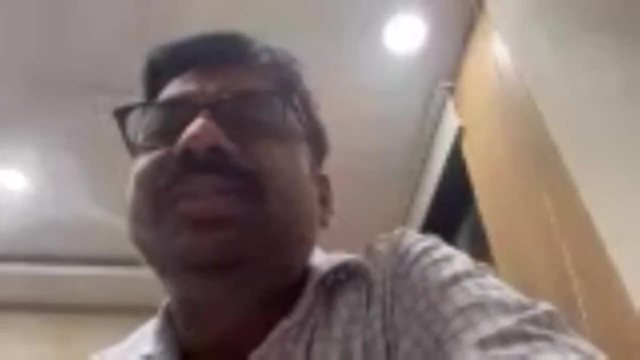 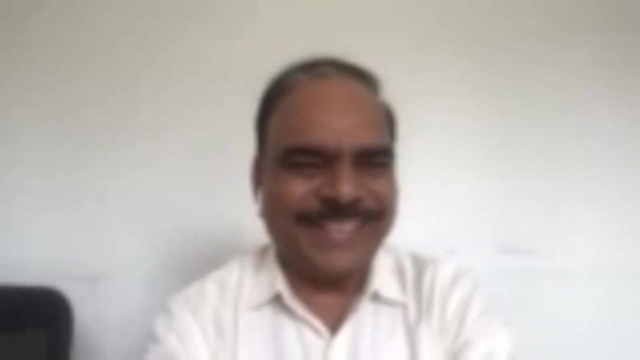 this is about prevention of disputes and claims. i requested iahe to give a copy in whatsapp. i told here: zero time overrun, this is the objective, how we should go here: zero time overrun and micro level construction program. i tried to tell here how it is supposed to be done. then delay: delay analysis. 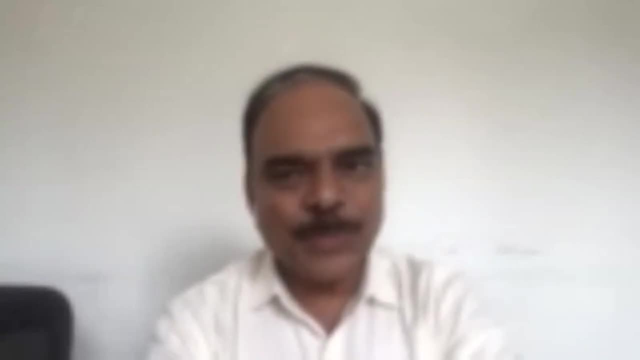 using construction program, how to do it, whatever i have told you about. impact program, revised program, absolute delay to authority of authority, absolute delay due to contractor, whatever is there i have tried to explain in this program, in this paper. then, limitation of claims. limitation of claims in the sense a project is cost only, say, 100 crores or 150 crores. claims come up to 300 crores. 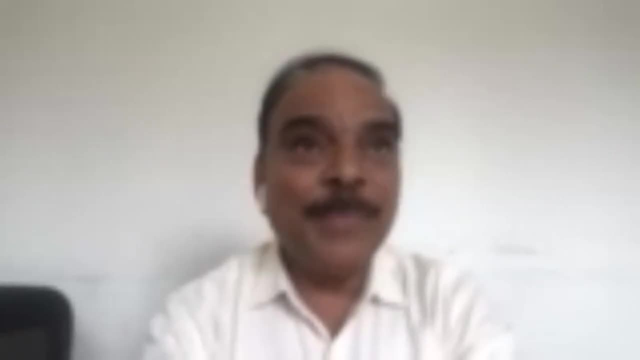 so there is no, there is no comparison, comparison. and another thing: what i mean by limitation of claims is claim should be restricted to the foregone concession period. in this sense, the project delays by 100 days, 100 delays, 100 days and daily, say, 30 lakhs. 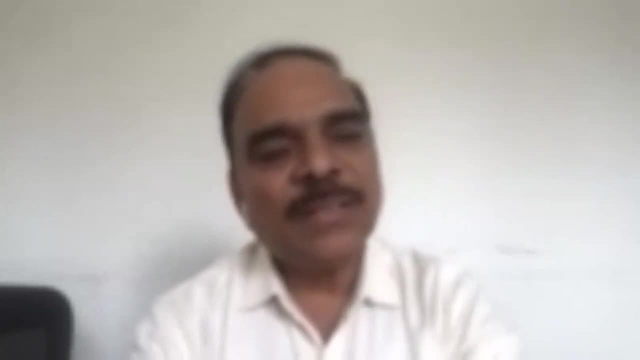 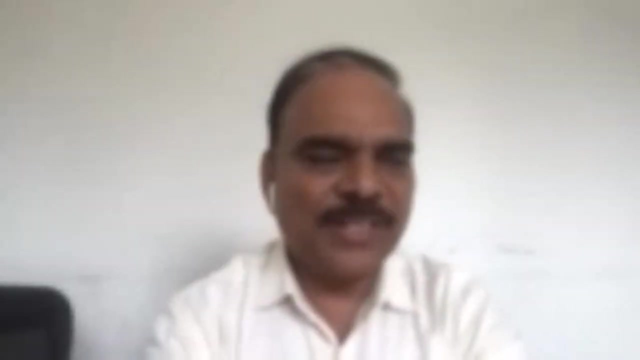 30 into 100 lakhs is 30 lakhs into 100 days is 30 crore. he should not claim 100 crores claim okay. so it should be restricted to foregone concession period in case of this and to the last annuities in case of build operate, bot annuity model projects. 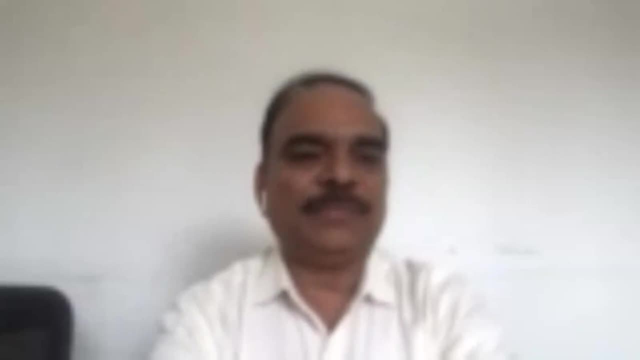 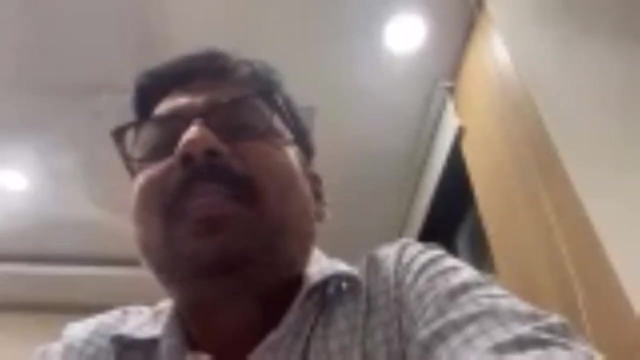 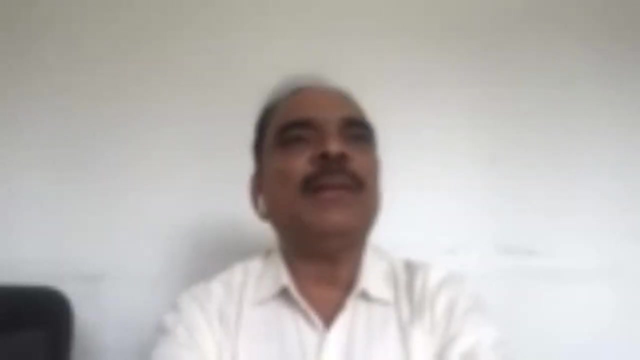 okay, so otherwise, epc and ham projects are adequately protected against time related claims if the employer is resilient and exercises prompt control on the scope of the project and, of course, maintenance of proper records and analysis enables the employer to manage, manage or counter the claims. okay now, zero cost overrun. uh, i in fact project preparation if it is done. 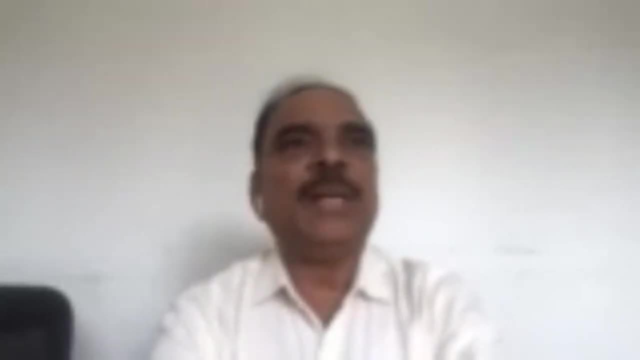 by a proper consultant, things would be okay, but uh, public consultation. i will give you an example of a project where we have prepared the entire proposal, all the schedules, and we made it. we prepared a presentation, then we called the local representatives- local representatives in the sense, including the party people who are heading the state. 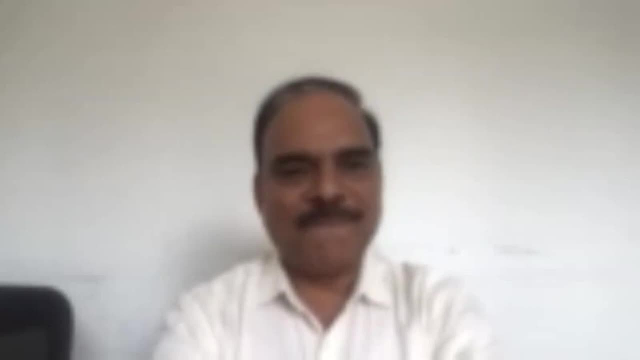 so that gentleman has come and district administration has come and other departments of public and important local representatives they have come and we have presented the whole thing. so this is the. these are the villages at this location. we have provided like this: here it goes to left, here it goes. 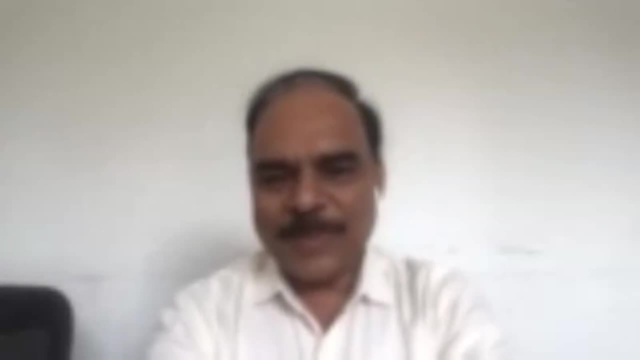 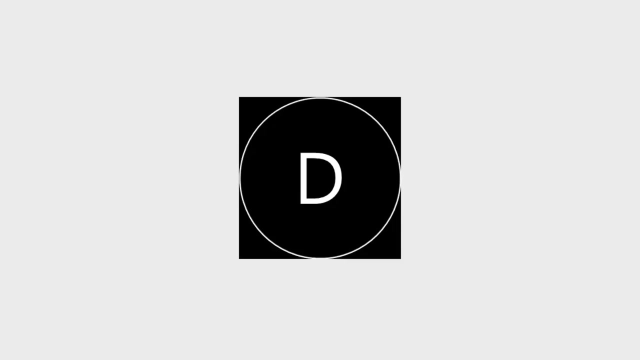 to right and all those, and then we have given they. they have questioned us there itself, but after that we have given time to the local rnb and other departments. they have told you should provide something here. we have planning like this: you are only providing a two-lane rov, whereas we 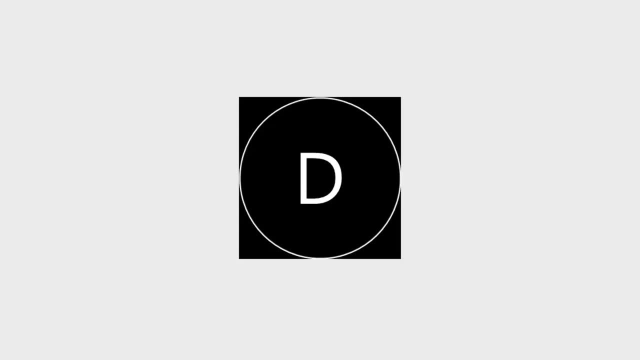 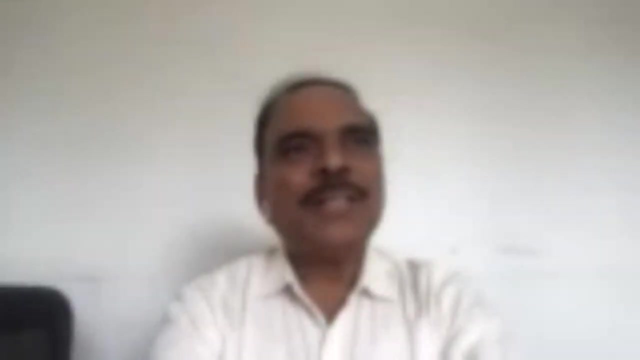 are going to two-lane underpass, whereas we are going to four-lane it within next four years. so please provide a four-lane underpass, something like that. so when that thing is done- and after that we should- we should see that the minutes are signed and they should sign that everyone has. 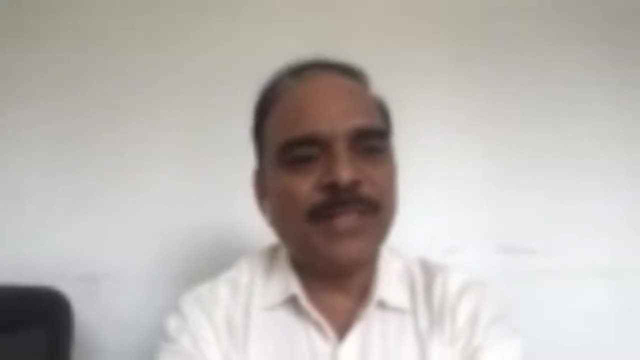 understood the provisions made and the reasons for not providing certain facilities, why we have not provided. they also understood that and that they would neither raise any request or demand for a new facility during the construction period, nor would they stop the works while they are being executed during the public consultation, if such. 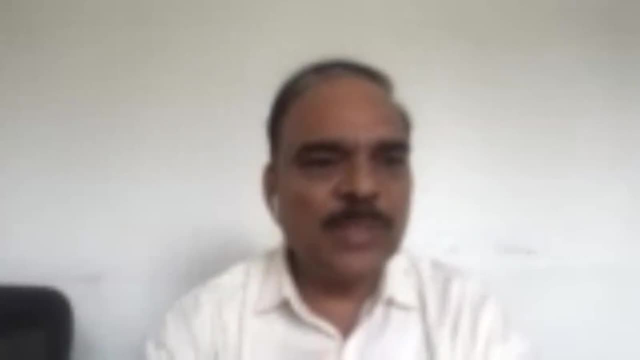 is organized in in front of the district administration, then there won't be a problem. and if, if at all, such an issue rises during the construction, they agree that the employer would take it up after completion of the works during one and period and all and a video record of the 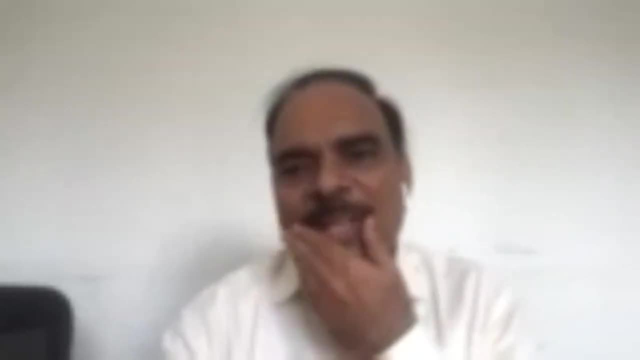 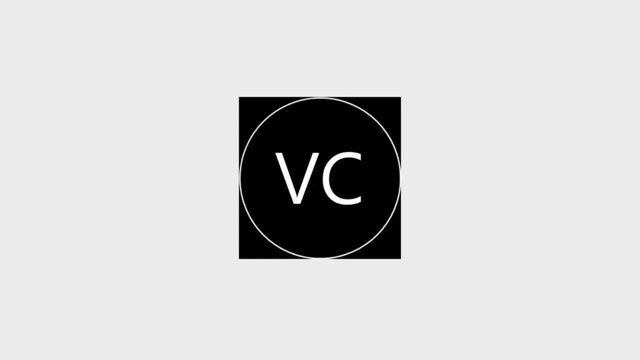 public consultation should be maintained by the employer. if such thing is done, at least completion will be done. project will be completed on time after that. okay, you need, uh, an underpass and we'll provide that during one and period there will not be any contract claims. now, bidding, bidding. employer should organize a reconnaissance site visit for the 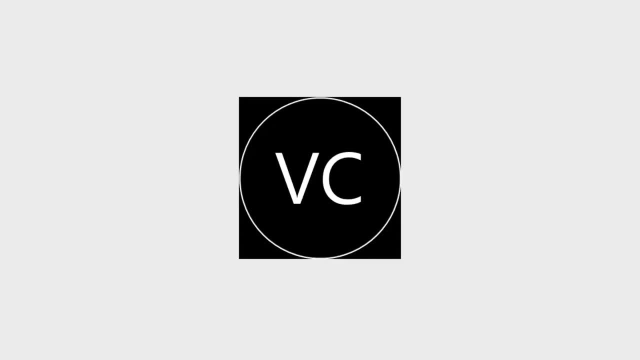 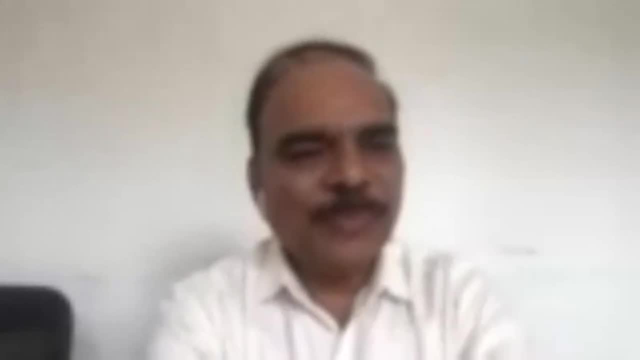 bidders along with the dpr consultants. now bidders are not coming and pd won't visit also, so all the bidders should go. all the bidders should compulsorily attend the site visit, take time and review the dpr with respect to the works to be performed, the time and other. 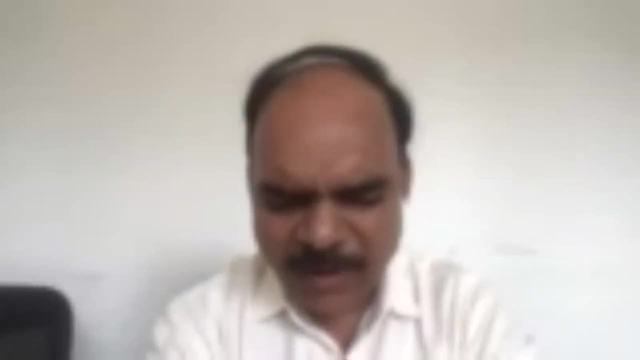 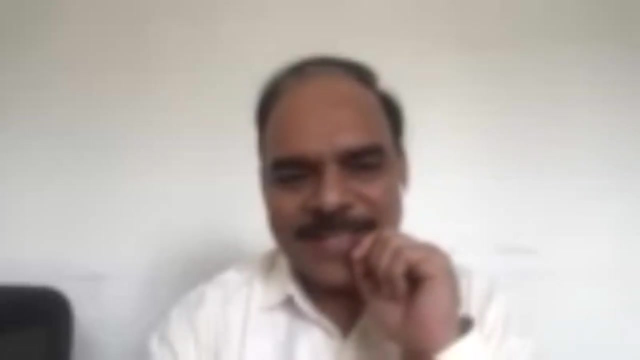 schedules at the site itself, so they should provide the inputs at the site itself so that the documents are modified if it is required. a drone video of the entire site with commentary of the provisions may also be provided to the bidders for a fee, if you want, so that they could vet the. 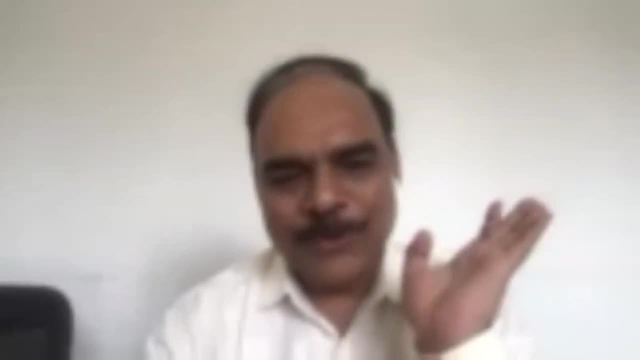 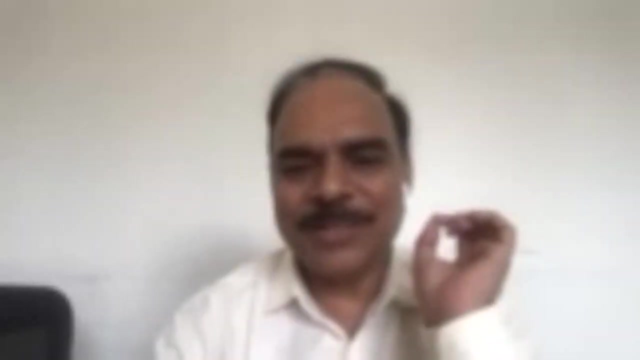 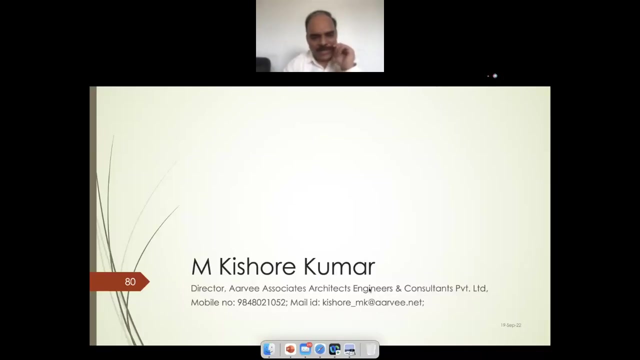 proposals, ask queries if necessary and make more informed bid submission. employer should respect the gravity of the queries being asked and provide proper replies so that they won't okay. and an identity must be part of the doc where the scope changed. consequent to clarify this: suppose the tooling has to be modified to four lane. then employer says: 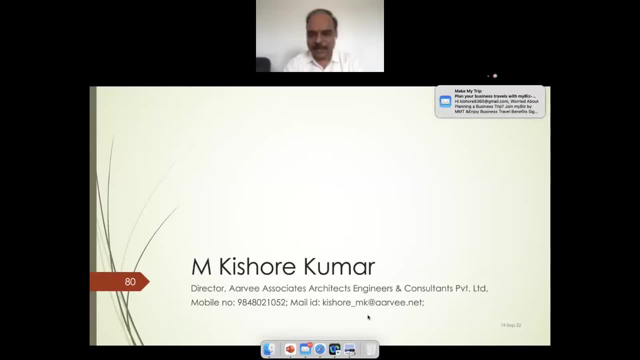 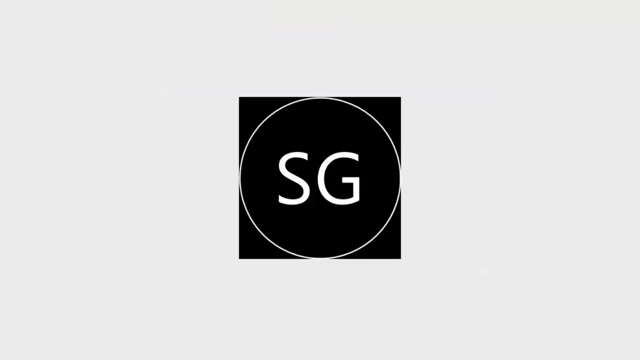 yes, schedule of addendum and clarification should be understood. clarification to don't only clarify what is written over there. it cannot change the scope of the document by clarification. so when there is an award of contract, successful bidder should re-review the documents for the adequacy and consistency in consonance with the scope of work before signing the agreement undertake. 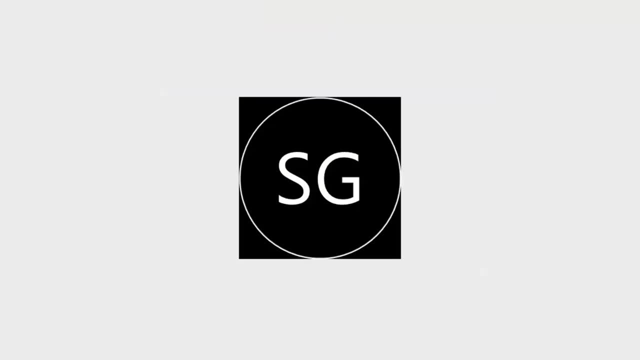 that he had seen the site. he has reviewed the documents and satisfied himself on the adequacy and consistency of the documents. manually: the writing something, schedule is writing something, so there is no inconsistency. we have changed, has understood and agrees the scope of work and shall not raise any claims on account of the scope. 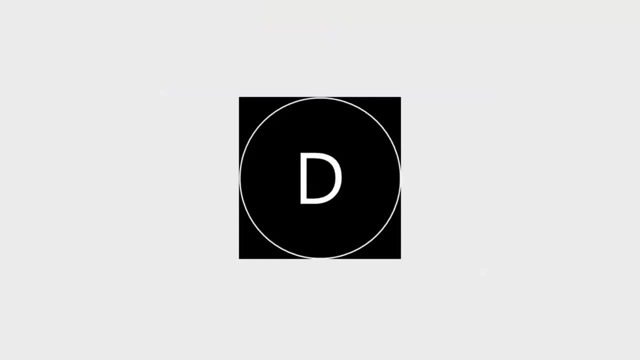 of work included in the contract. okay, and, of course, deletion of the thing and dealing that. what that's, what uh we have written and uh also that not to entertain any public representations or change of scope on such account during the construction period and if the parties agree. 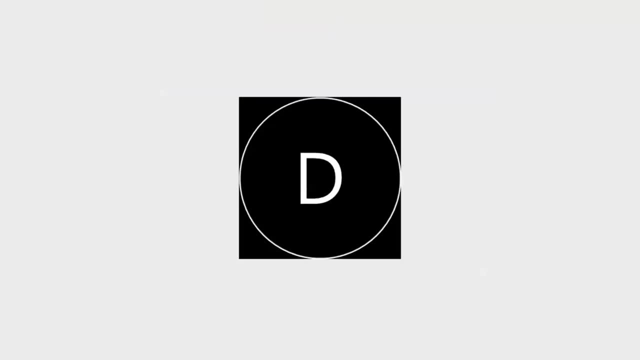 to provide such facilities, dealing them from the completion schedule. all seo should be dealing with it. so such an initiative would freeze the scope and duration of the contract before signing with the contract, which in turn would avoid any cost related claims, document related claims. uh, in fact, during the before signing the contract itself, they should discuss on these. 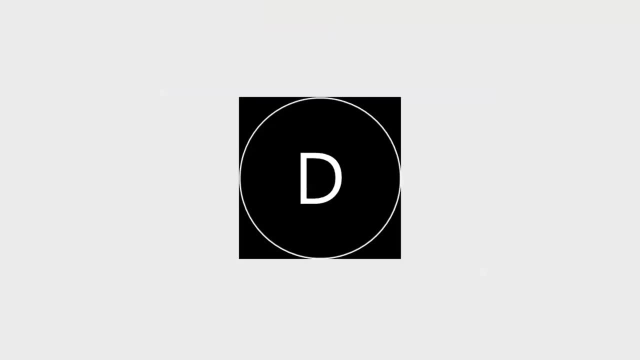 ambiguities, omissions and interpretations. they should be removed. so see, there is one aspect here that is delays and deemed approvals. uh, i'll leave it to you. i'll leave it to you then. revisions in circulars. a circular is issued, but it is not supposed to be. 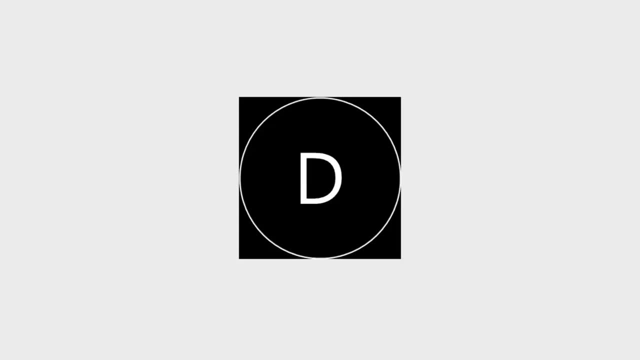 part of the contract, so when we apply it to the contract then it becomes a claim for him. undertakings and supplementary agreements- whether they are legal or not- it was addressed here- and awards for anyway i have given and whatever i have put in the last three slides is picked from. 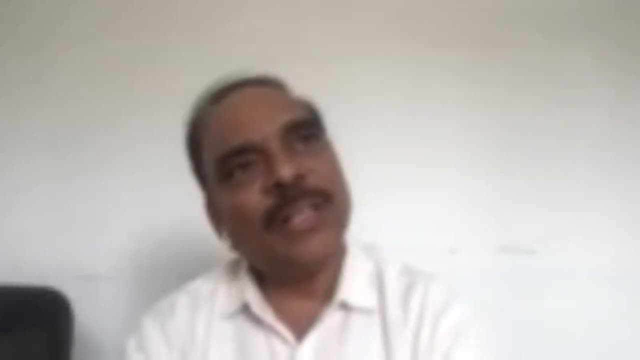 here. okay, so that's it. so more questions. so good afternoon. my name is dilip patil hello, i have been seeing that you are going off and coming back quite often. yeah, yes, sir, yes sir, actually the network issues were there. i know that's the reason earlier. 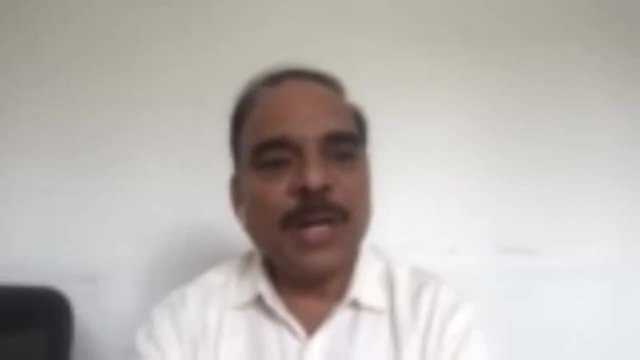 i was having a feeling that people are not interested in my session and they are leaving. no, no, no, it was very right actually, and this, this kind of minute study you have done that is very fabulous. but the issue is that how much we are able to implement in our- uh, particularly ham. 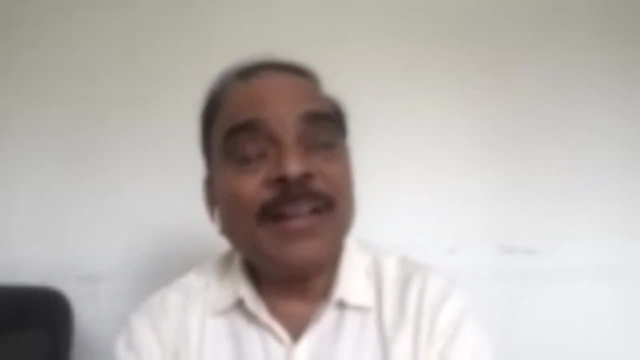 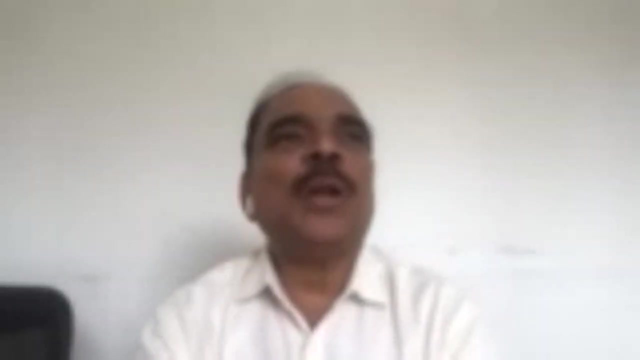 mechanism, because this eye is there and all these things. so that is one issue and, sir, another question was that in the, this ham, the financial models are given and then in financial model they are quoting the epc cost. so is it some kind of benchmark for us to see that their epc costs are limited to the financial model epc cost? 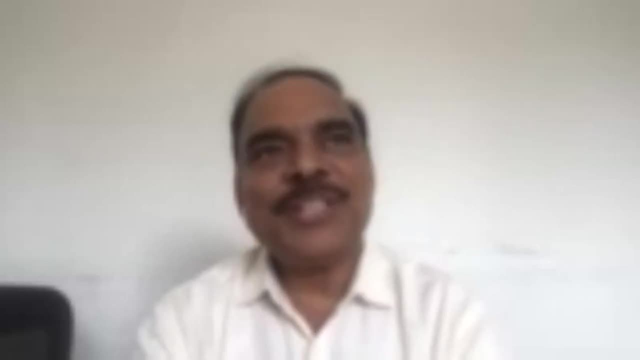 that was another query. and third was: is there any kind of uh private of the agreement between uh authority concessionaire and his epc? quantitative priority is always the main contract, see. another thing that we have to address which i have not told you is there is no priority set between schedule b, c and d. 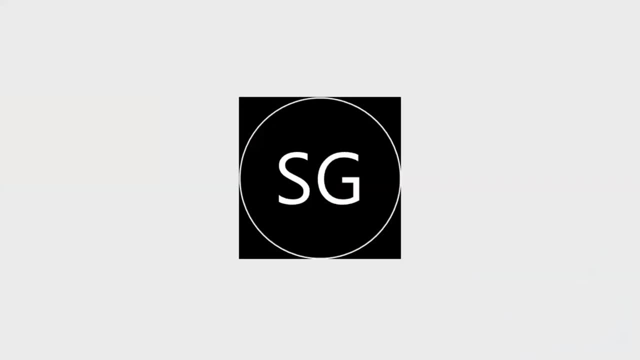 i have answered you directly. the main agreement is top and then we are not here to interpret what is below that. they don't form part of our agreement, so we are not here to interpret them and take it as a priority in deciding things. we only see that they are reasonable, they are correct. 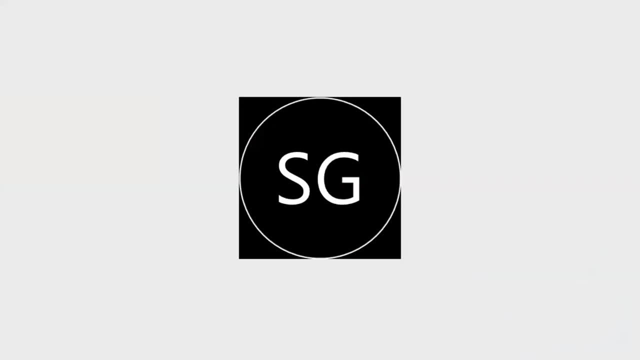 the epc document and o and m document, but they don't form part of the contract between the authority and the concessionaire or the contractor. so that is. priority is over. i was only trying to mention that there is no priority between b, c and d. suppose in d something is. 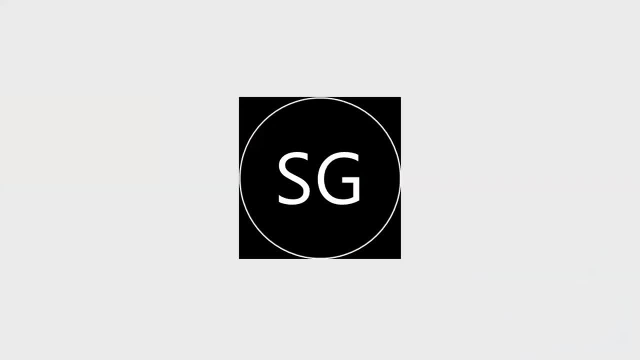 written and b nothing. nothing is written. but the d cannot form scope of work unless there is a link between p and d. so b and c are the primary scores. so, but our documents do not have that priority between schedule b and c and d. so that's what i and regarding uh, epc cost in ham, what? 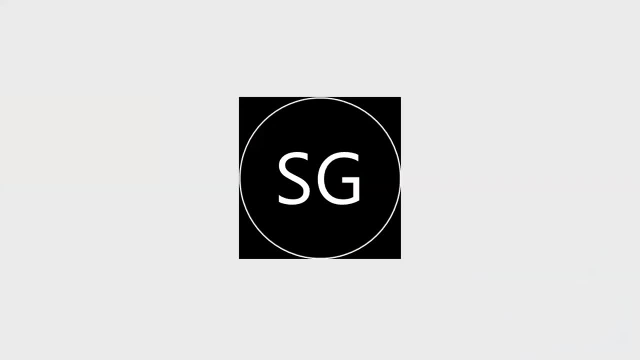 exactly is the problem? because i think in ham, what is the bit parameter? uh, the bid parameter is, uh, the cost, project cost as well as first year o and m. they have removed that. now what is the big parameter? big project cost and even maintenance cost. also know for the first year. 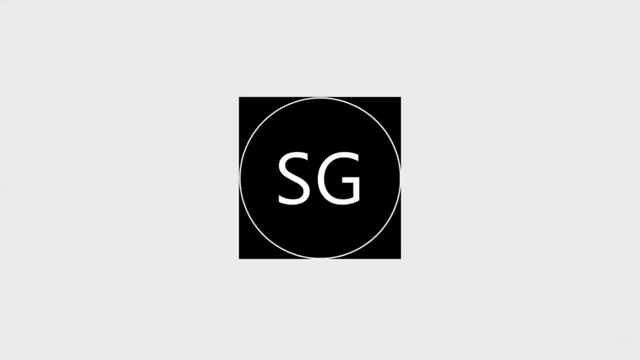 yeah, but uh, since last six months that has been deleted. so only now we are taking this bid project cost, not first year o and m cost, but then i am not giving first year o and m cost in the documents. they know it is a formula- is gay there, sir. and on that formula. 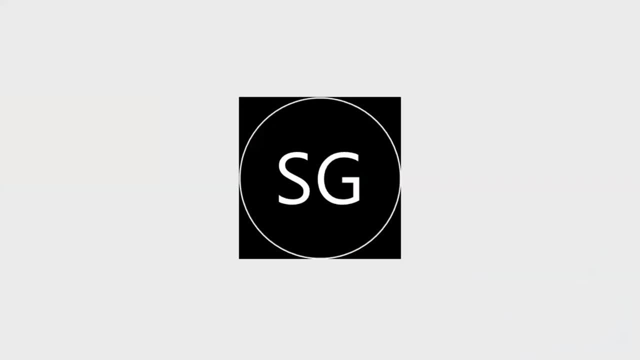 that will be project that is based on this bit. project cost, item cost are paid. okay, he does not have to quote a figure for that. first year. one name cost, yeah, okay. so now what is there to control? what is there to control? big project cost is quoted and, uh, whoever is quote. 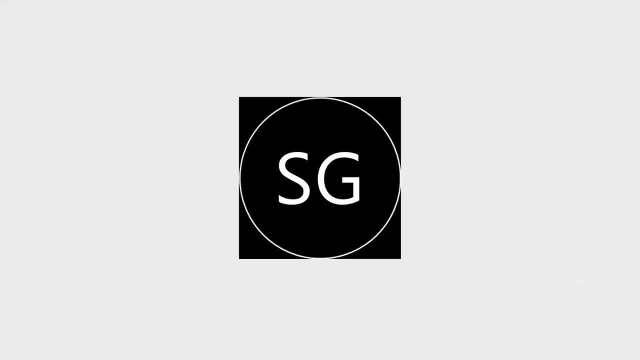 a reasonable cost that is to our advantage. we are agreeing to that and then we are going ahead. so what is there to control in that cost in? in one of the cases i will tell you- i think i have answered the question. but, connected to that, i will tell you something in one project in west. 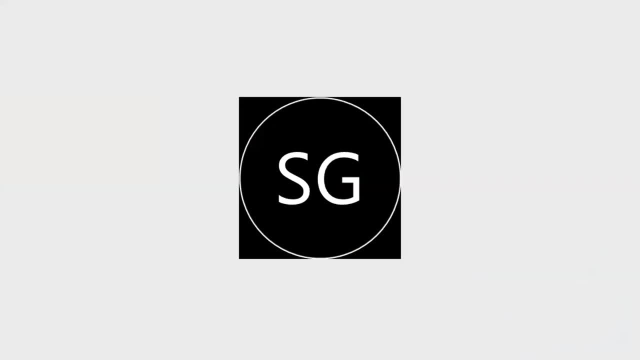 a request has come to me to change the flexible pavement to the rigid pavement, so now it's a ham project. i have estimated the flexible cost and i have estimated the rigid cost and then i have seen that around 60 crores is the variation, so which has to be given as a 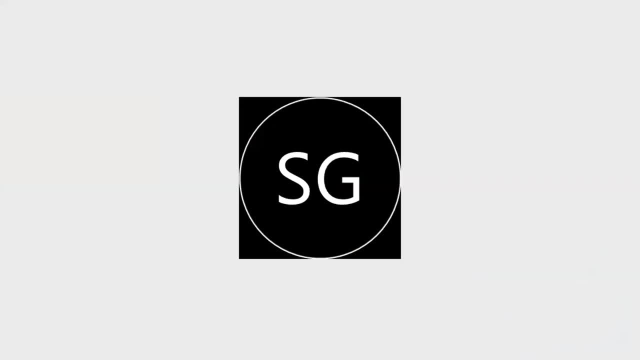 change of scope. suddenly, i have understood that the maintenance component of the flexible pavement, every five years we are supposed to put the means overlay and each each is around 25 crores, i believe. so it's about 75 crores and if i and rigid pavement maintenance. 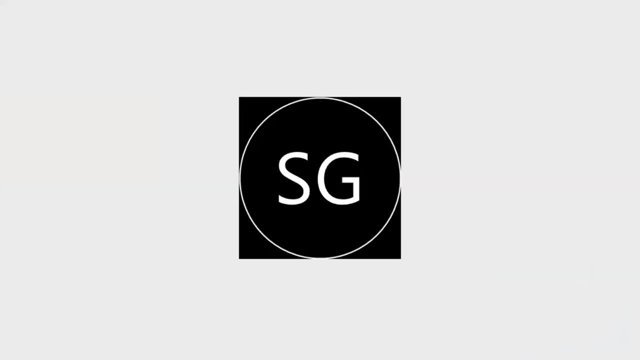 basically life cycle cost. yeah, but there it is. i'm only talking about see. if you see the routine maintenance cost, i think rigid pavement is only four lakhs per kilometer. for four lane that means one lakh per lane kilometer and if you see the flexible pavement it's about 3.5 lakhs. per four kilometers. that means around 90- 90 lakhs per lane kilometer. so there is not much difference between the routine maintenance. but there is no periodic maintenance in the rigid pavement and there is a periodic maintenance in flexible pavement, and that is almost 75 crores. 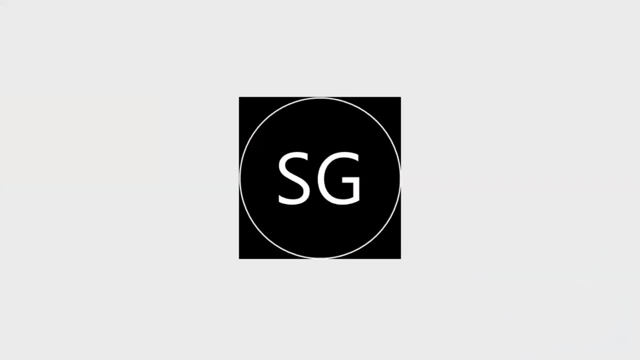 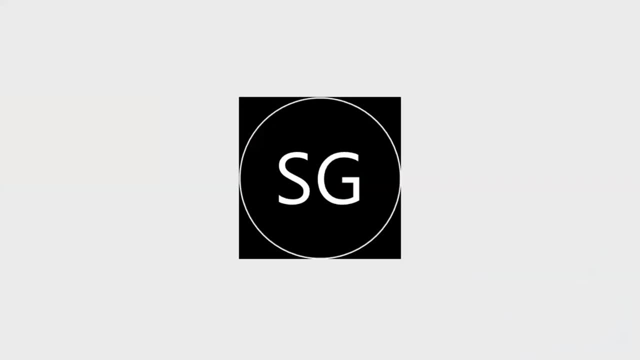 provided. the maintenance cost provided is around 10, 10 crores per annum, that in the ham. so now the 10 into 15 is about 150 crores. so now that 150 minus 75, whether it is- and i have seen my dprs in the dprs i am not providing the periodic overlay, i am only giving 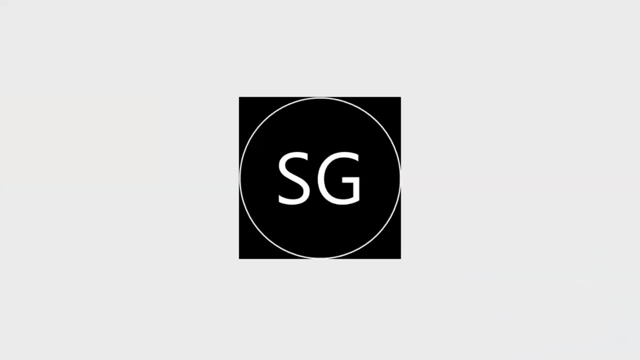 the civil cost. i am not giving a periodic overlay. so where is it? and he is giving a bit project cost. that budget bit project cost doesn't have maintenance included, periodic maintenance included. so with all this i was literally confused. anyway, i told the contractor: it is better that you. 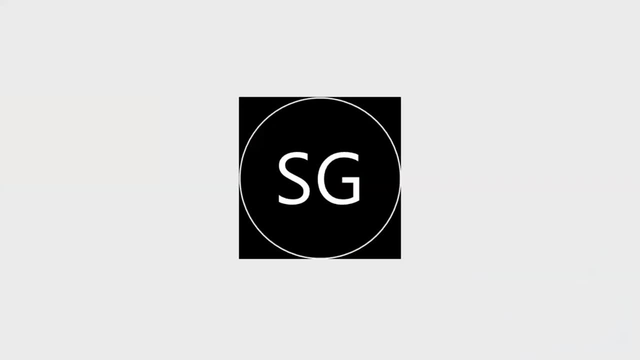 construct only flexible payment and don't ask me any cos for rigid payment. don't go for it. so this is one one thing that i wanted to share with you. so maintenance is required. i will just go over it as to why they have removed and how it is going to help the concessionaire or the authority. 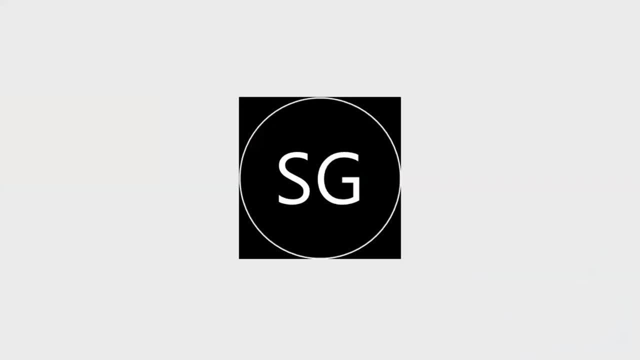 thank you for asking those questions. thank you, sir. uh, other participants are also requested. if they have any questions, please ask your questions. sir, i wanted to know is there any provision of sectional completion, because you said: sir, i wanted to know is there any provision of sectional completion because you said that, uh, after 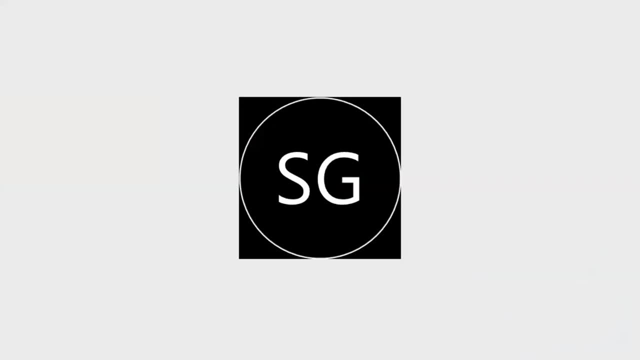 issuing funds list. 10 years was elapsed, but the work was not completed in all sense. so is there any provision of sectional completion? and second question is, as we came to know, that authorities engineer only review the design and the final responsibility of design lies with the contractor. so is this make any sense? 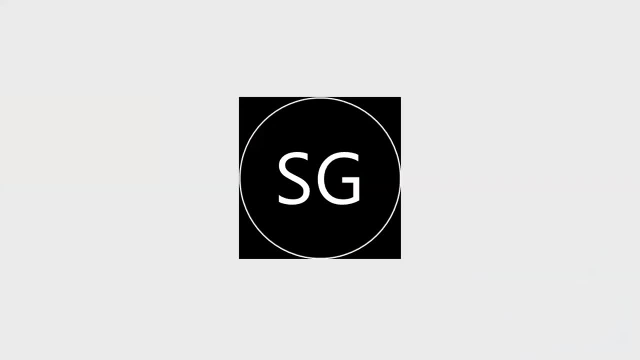 because if a is not given his review and the project was carried on, carried upon the design of the contractor. and third question is: you said that deletion of the scope, delivery as per SOR or mid time of SOR, of that a period, construction period and schedule H was defined during the agreement. so if after 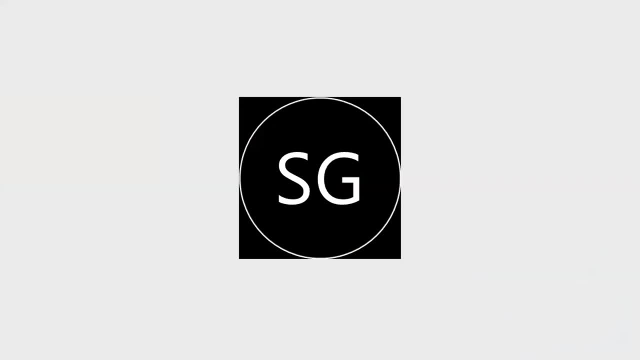 designing some component, the weightage of that particular component get reduced or enhanced, so schedule H may be adjusted accordingly. so does it make any sense that deletion will be a deletion will be as per the H, as per schedule H. any modification will be as per SOR, sir. yeah, yeah, thank you. thank you for those questions. see, I try. 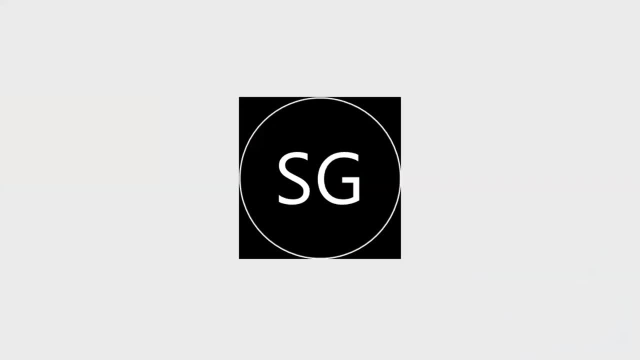 to remember the questions. so the number one was whether there was any sense of sectional completion, see, when we have given the provisional completion certificate, the main carriageway was complete and the service roads were complete and whatever was not complete was hindered at that point, and some more. 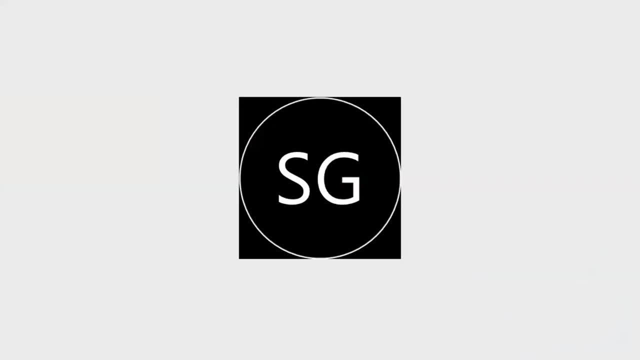 items were there which was supposed to be completed. for whatever reason there was a change of ownership and all that stuff. they could not complete those. and then now it's. it was also a BOT project, so in BOT project there is nothing like a sectional completion. the whole project has to be given right. so there was not. 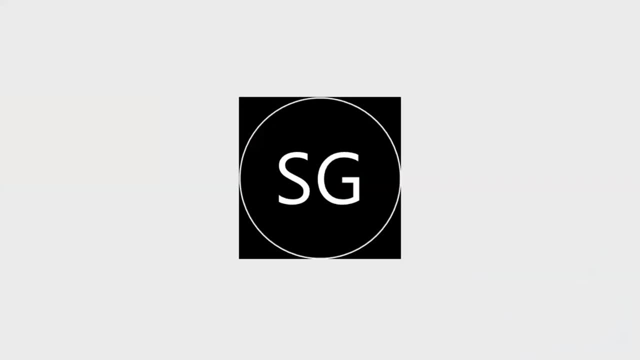 nothing like a sectional completion. then. second question was: I'm so sorry about the review of design. yeah, yeah see, between the authority and the consultant there is nothing like concessionaire is responsible between the authority and the authority. engineer authority is responsible. other engineer is responsible for accurate reviews, even if he. 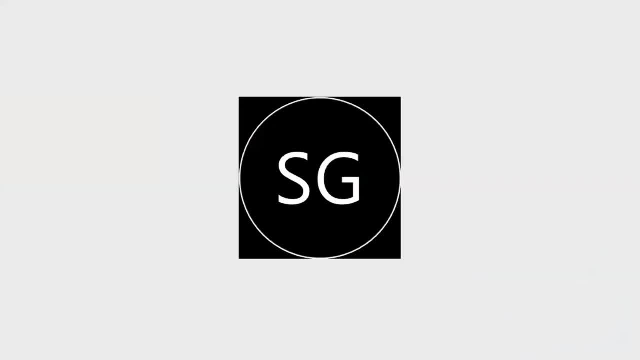 has. he is vested with some 25 percent responsibility and then there is nothing like a sectional completion, zero responsibility to review the RFS and all. he is 100 percent responsible or he is responsible for 100 percent equality between authority and authority. there is nothing but. 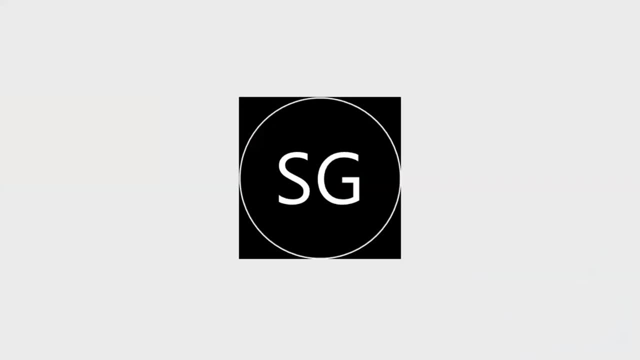 between authority and the concessionaire. the concessionaire is fully responsible for the accuracy of the designs. that is what. if you see the paper in there, there is deemed approval and all go through that it will be. it will be sent to you today itself. so go through that part deemed. 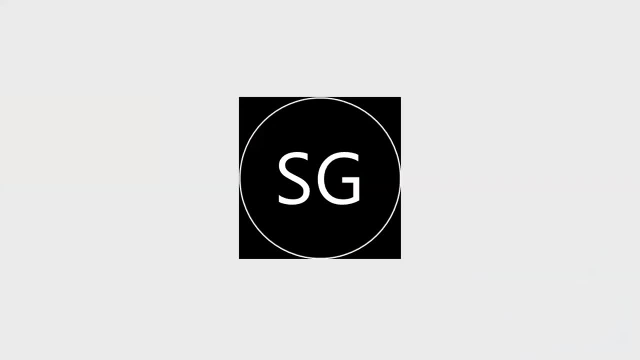 approval there. I have dealt it. so between the see there is a clause in bot if you remember that the contractor submits the designs to the authority also and authority may review them and comment them within 30 days. even if he doesn't give any component a comment, then it is the concessionaire's responsibility to go ahead. 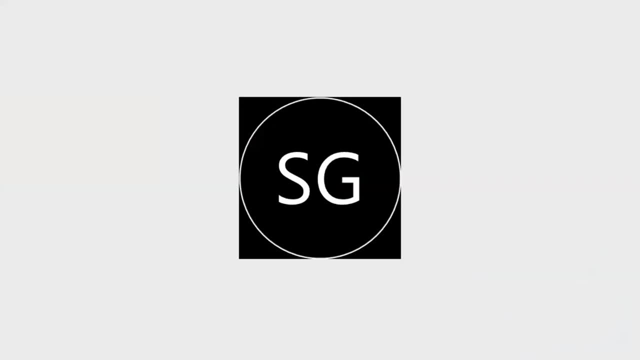 with that. so that's kind of a deemed approval from authority side or other team inside. so you read that particular para where i have written delays and deemed approvals, then you will be able to appreciate it. but but the answer for your question is: authority engineer and independent engineer are fully responsible for accuracy of the designs, whatever they have reviewed. 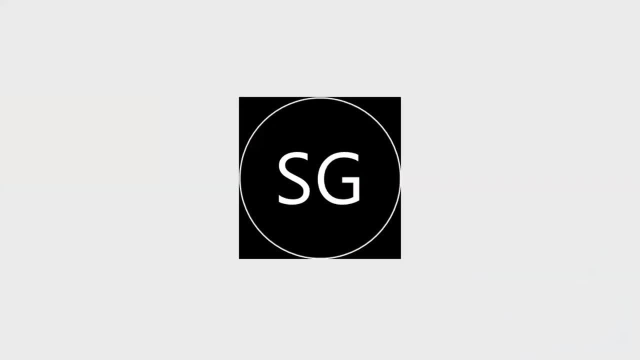 to the authority. right, that is the second question, and the third question was, uh, of the revision of schedule h. yeah, see, it is written on the epc document, if i remember correctly, that if at all authority is not able to review the design of the design of the design. 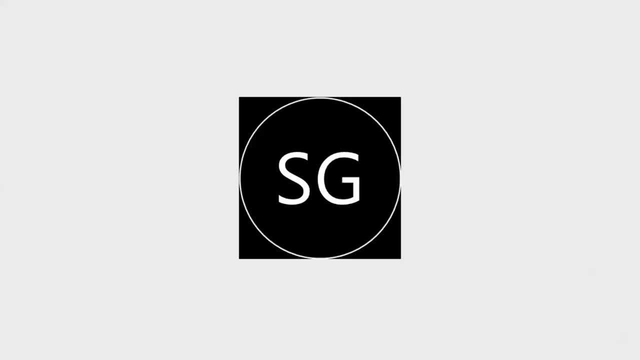 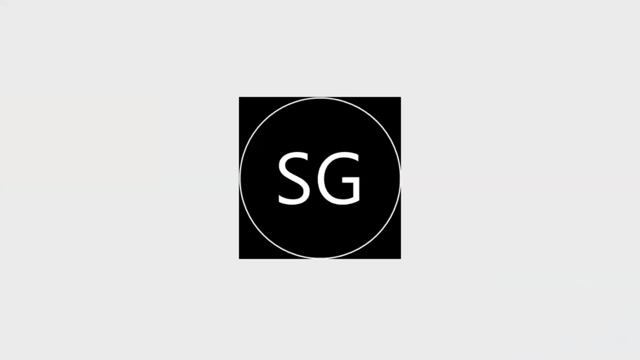 now as a practice. whatever is being modified, we are trying to do it with current sor because if at all the contractor does not agree to do this and if we have to get it done through somebody else, then it should be current so far. so the work will be. both the positive and negative will be. 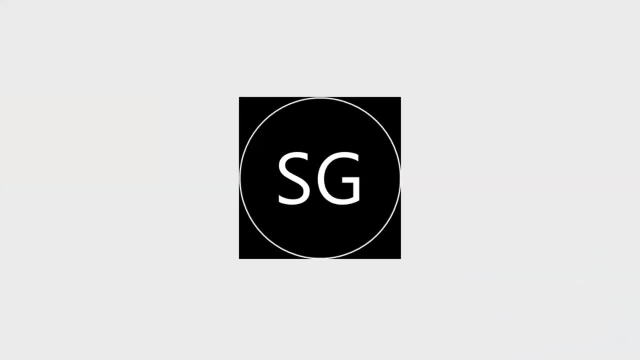 evaluated as per the current SOR and that will be given to him. He may deny to do so. He may deny the change of scope. That is the reason why we do it like that. I hope I have addressed your query, Thank you. 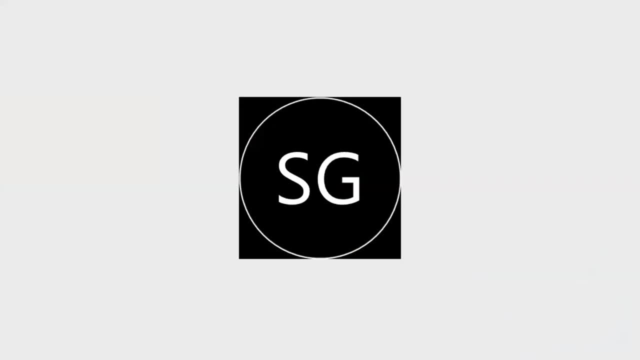 Anything more, sir, All our learned engineers who are there. I have all respects for the people who are. One more query, sir. Suppose my shadow C use a certain number of state lights- 100 state lights- but afterwards I found out that I do require more state lights as per the code alarms as per this site requirements. See, I don't know whether you have completed the question, But schedule C never gives the number of poles. It only gives that lighting should be provided in urban areas. 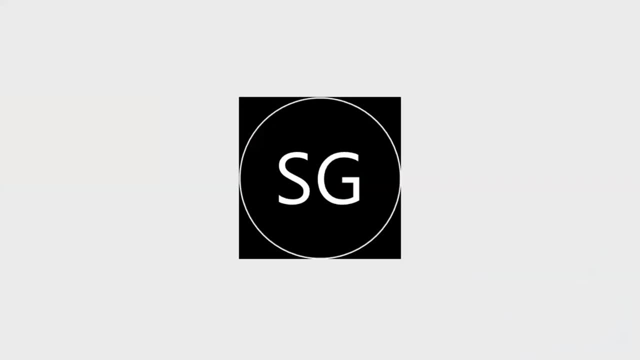 semi-urban areas, rural areas, habited areas or something like built-up areas and all. That is one Second thing. it also gives, probably on the structures it will give and it gives the lux requirement. So if there is a more length, in the sense it never gives even the 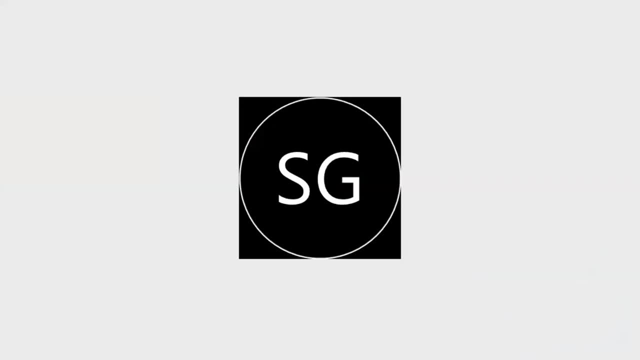 length. also, It only gives that you have to provide here Toll plazas like that. So there will not be a number. I have never seen an agreement where it is these numbers are given. It is only where it is supposed to be given. 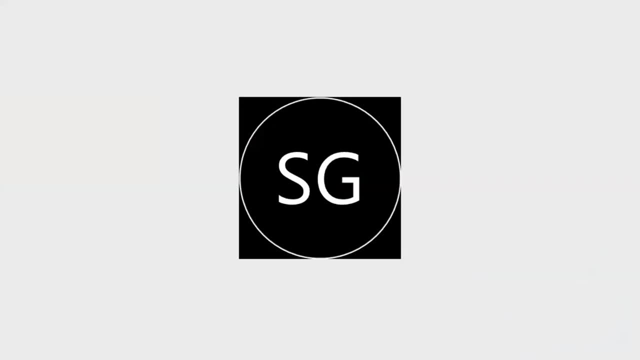 Yes, Thank you, sir. Anything more? sirs, It is one o'clock, Sir. one doubt, sir, Can you tell me? Tell me, Sir, regarding this is base date. sir, Base date and change of law. 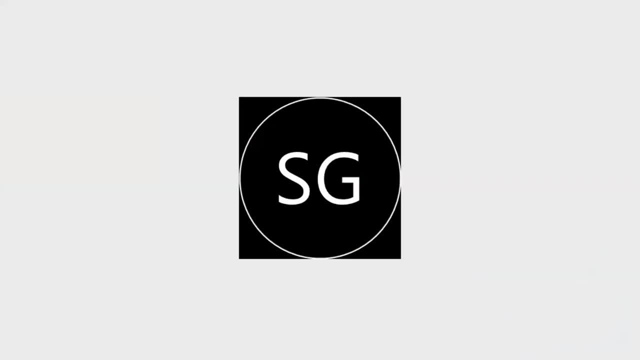 I am having difficulty in listening to you, Sir, regarding base date and change of law. Change of law, Okay, Change in law. I think we have a difficulty. What I suggest? please note down my email ID: kishor, underscore mk, at rv dot net. 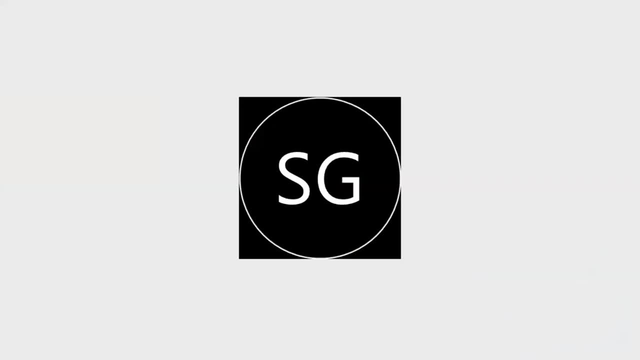 Any of you. if you have any, if you any time in your project, you can write to me and I promise you that I will give a prompt reply the moment I see it. Vijay Kumar ji, aap isme nishiyega. 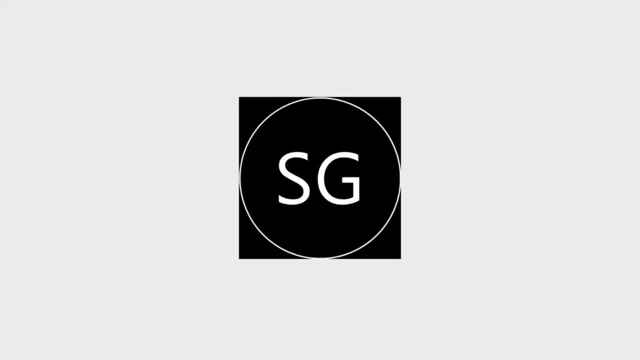 Because I am really not able to listen to you. I am so sorry, Thank you. Thank you, Please share the email. I think I have not shared it, So I will share this. Sir, we have already shared your email ID. 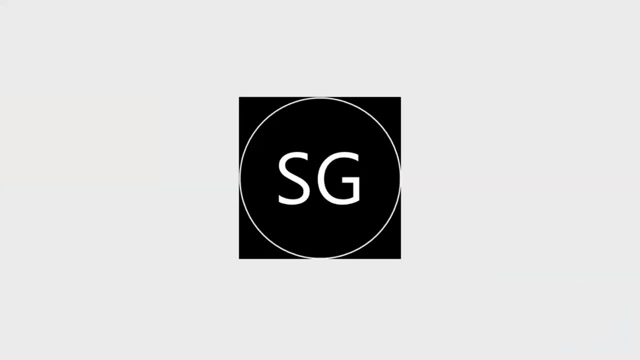 with the participants. See, I am always. I have been giving these sessions across the country in some other CII conferences and all other things. I want to be involved in these issues. You can always send me a line on this mail ID. You can always even call me also. 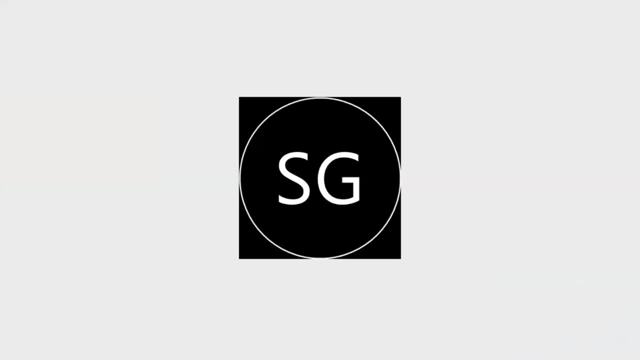 I have received calls from many people many times in the last 4-5 years. Okay, sir, Thank you very much, sir, for sharing your presentation, as well as your knowledge, with the participants, And thank you to also the participants to listen. 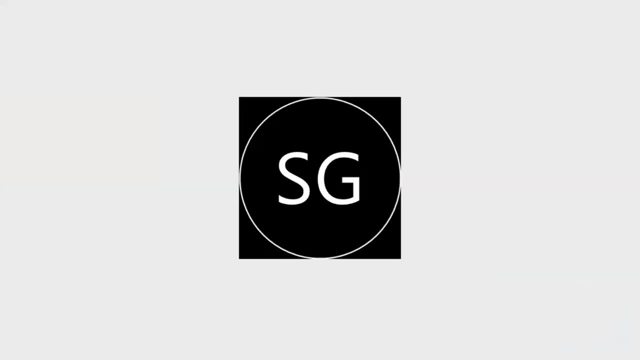 carefully. One last query, please. Yeah, Sir, actually some of our BOT projects are quite old. They were constructed when codes were prevalent codes. Now, with the subsequent revision in the codes, safety norms are changed. Now we are not providing. 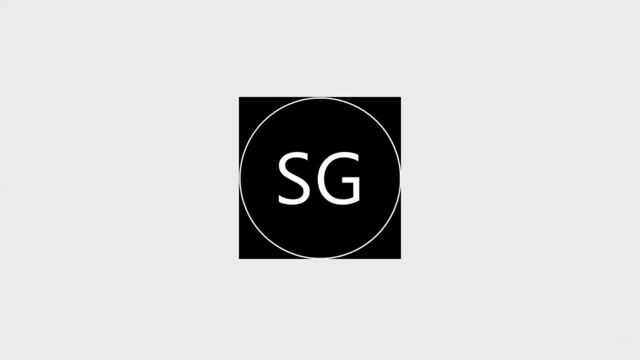 these RCC railings. It is being crash barrier New Jersey type crash barriers. One recent tragedy also is testimonial to this need for the upgradation in the safety requirements due to this revision in the code and norms. But our construction always says that. 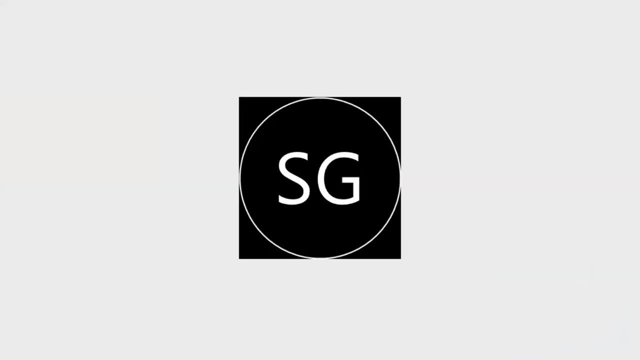 when we constructed this, built this project, the prevalent norms were according to prevalent norms we have constructed. And now if you are asking for revision in these codes and this revision in the facility, then it is tantamount to change of scope And whereas our version is that 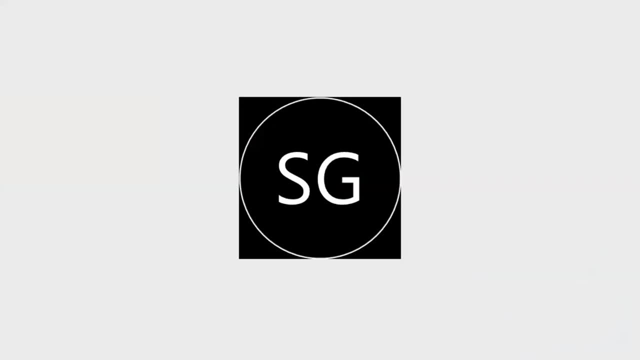 to be this, because this total revision is there We are. you are collecting the tool which is again link with the price escalation and WPI, So it is your safety obligations like that. So what should be our correct to stand? Your argument may not stand. 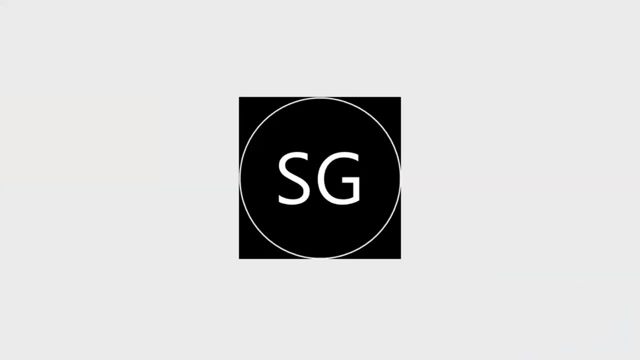 That our argument, I would say, may not stand. So if it actually tantamounts to expenditure, then it is better that we give: see signboards. Signboards: 2001 is different, 2012 is different. There is a cost difference. 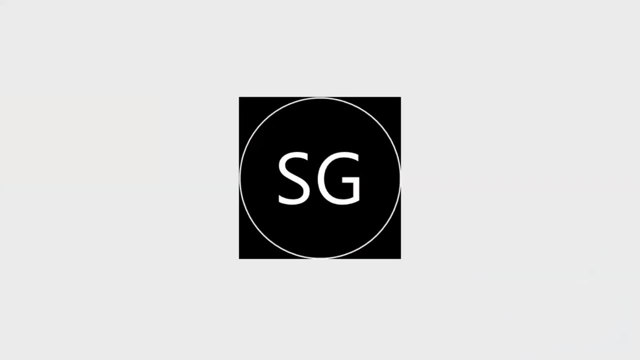 One or two crores Of change of scope It is good to give. then even you know what is happening in crash barriers: MBCBs. MBCBs also have to be crash tested. We have a test track in Indore. Now we are able to do that there. 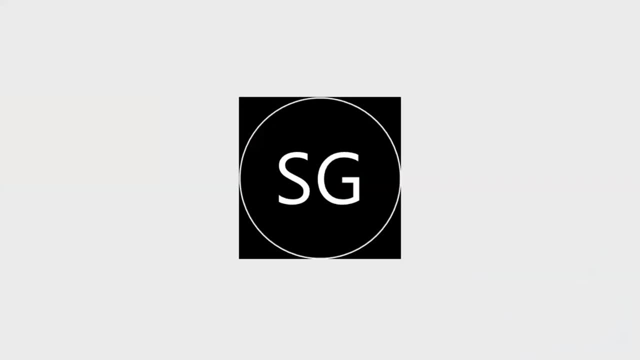 But none of the people are doing the crash testing. On top of that, they're reducing the interval, They are reducing the depth of the stem, They're removing the spaces between the horizontal beam and the vertical post. all that And they are putting it just like that. 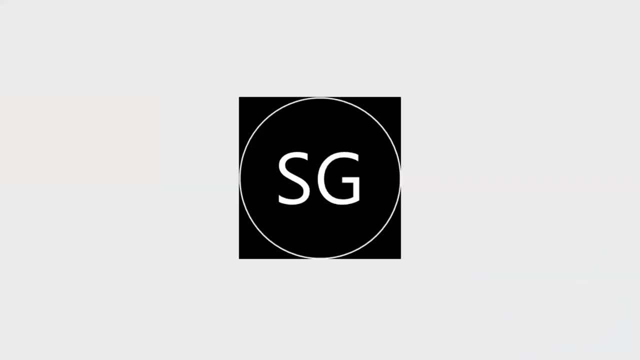 And they say that you have to clear it And we have approved there, We have, we got it approved here and all So, whereas NHIA or anybody has not cleared anything like that. So look at the design that they are submitting for MBCBs. 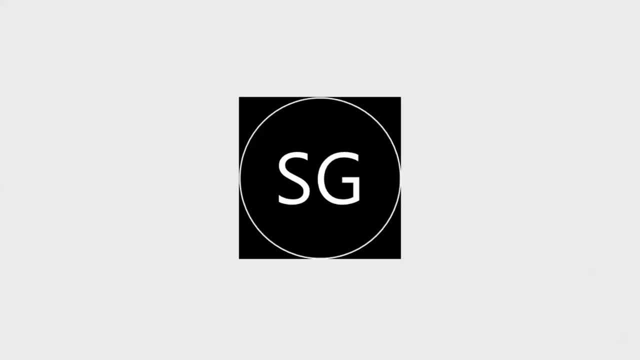 and whether it is as per the agreement and whether they are crash tested because it is written. So now, primarily coming back to the question, if there is any change in the code and if you want that a better provision has to be provided, it will be change of scope. 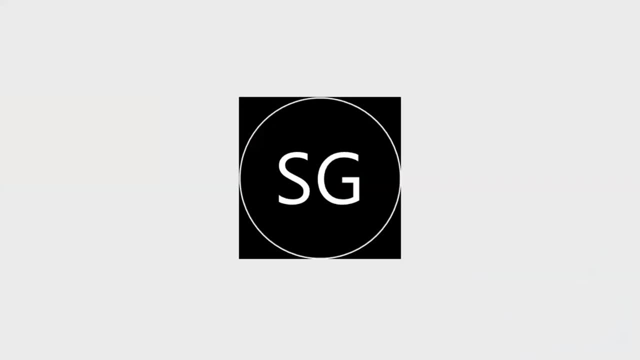 And see, be kind to him, Be reasonable to him. If he has to spend money, then we have to give him a change of scope, because your financial model will not cover all these things. So you can always rely on the financial model. 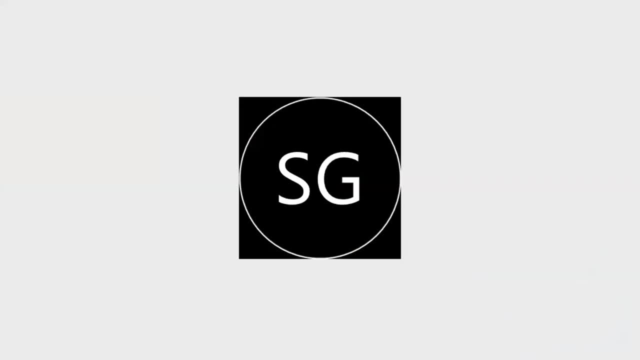 If we had time, we would have seen those also, Where all I am asking that they should go back to the financial model and tell me whether it is really affecting them. So give them changes. Let's go, please, Yeah, yeah. 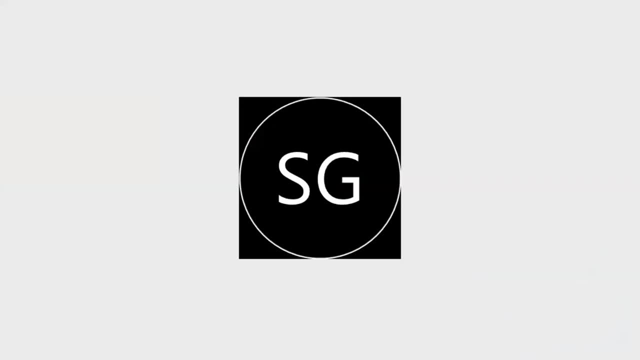 Yes, sir, Thank you, OK sir. Thank you very much, sir. Now I think we can conclude this session. Thank you very much to the participants also. OK, Neeraji now. please finish the meeting now. Yes, sir.